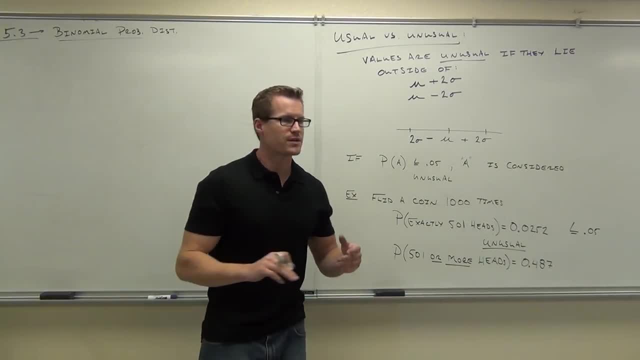 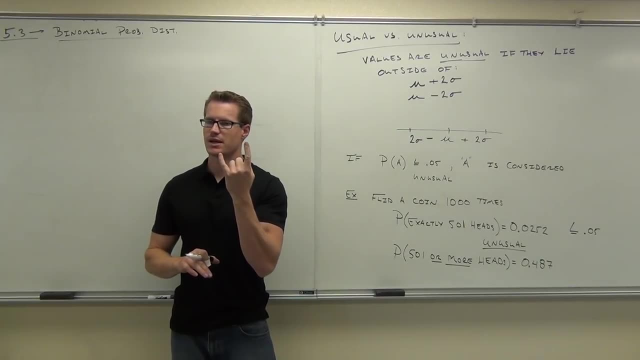 Something like name term outcome. For us it means outcome. What this is is a probability distribution where there are only two outcomes. Two outcomes: Something considered a success and something considered a failure. Okay, something considered a success and something considered a failure. 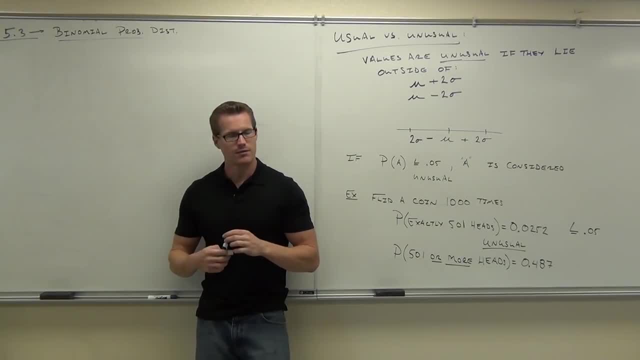 Now, let me warn you ahead of time. You can make a lot of things into a binomial distribution. Remember rolling the die. Don't roll the die And you have Actually six outcomes there. right, But if you say this, if you say my success is rolling a four, everything else would be a failure. 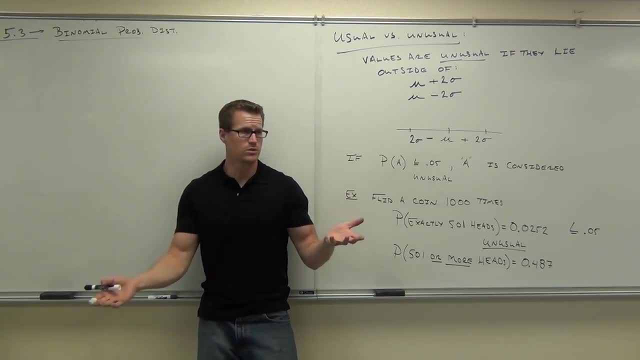 Doesn't that only have two outcomes? You either get the four or you don't. Does that make sense to you? So we can make things into binomial distributions. even if they have more than that number of number outcomes, we qualify them. 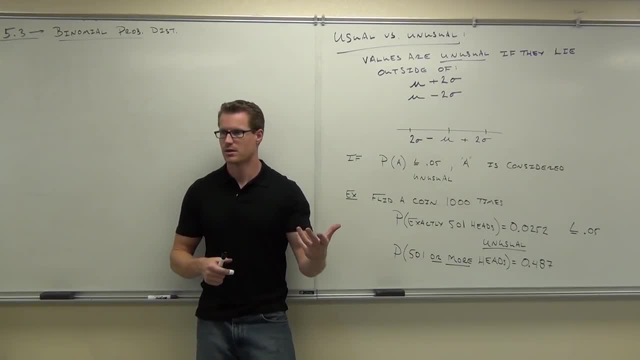 One would be a success and one would be a failure. Nudge your hip if you're with me, Okay. so that's what this means. We categorize our two outcomes as four. We categorize our two outcomes as a success or a failure. 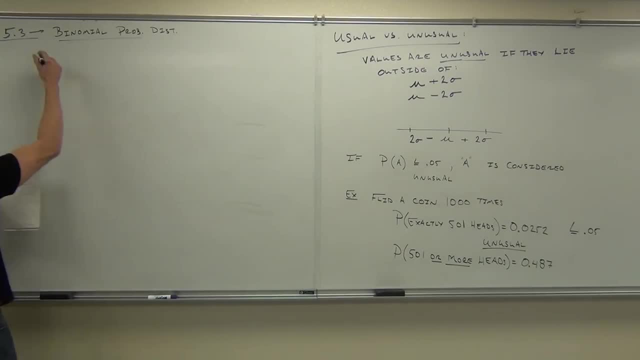 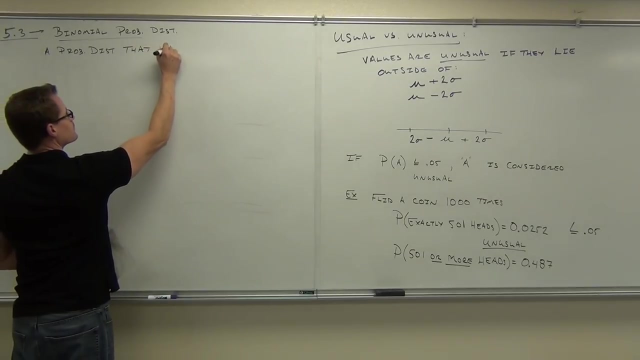 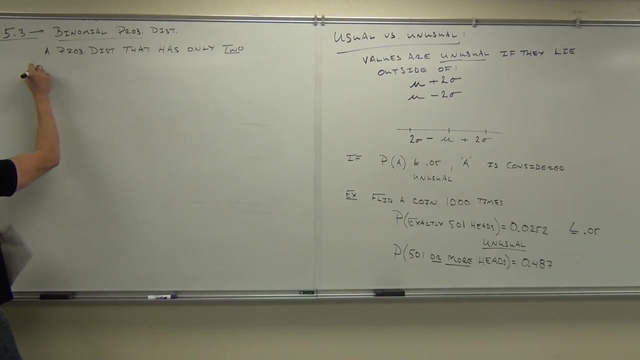 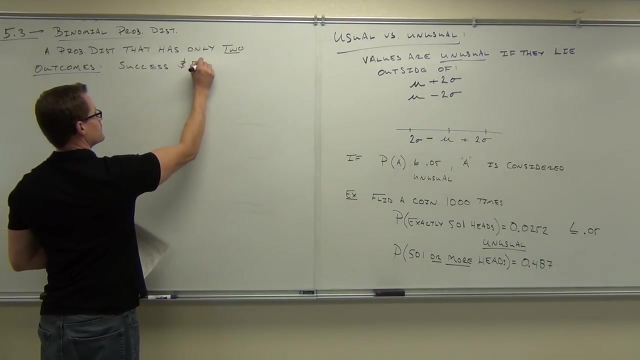 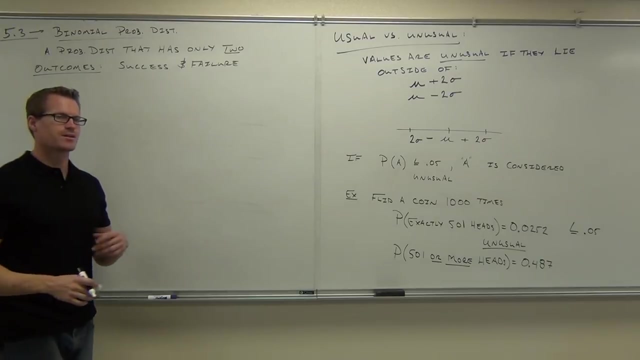 That way there's only two of them binomially, So a type of probability distribution where there are only two outcomes. Subtitles by the Amaraorg community: Success and failure. Now there's a few things you need to know about a binomial probability distribution before we actually go and do any examples. 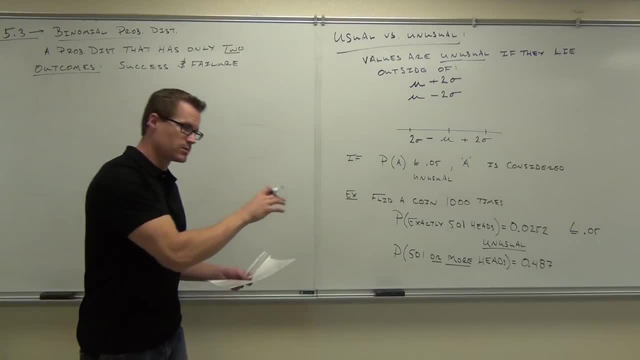 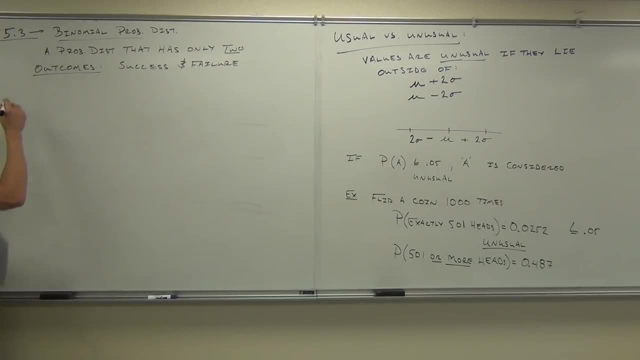 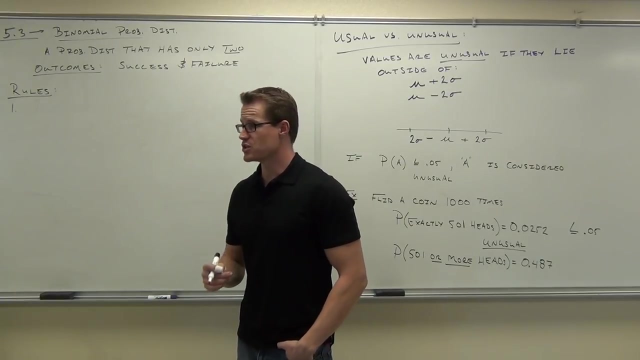 And that's some vocabulary, some simple civilization notation Subtitles by the Amaraorg community And what it takes to even have this binomial distribution here. So here's the rules for this thing. First rule: You have to have a fixed number of trials, which means you can't go and do this procedure for eternity. 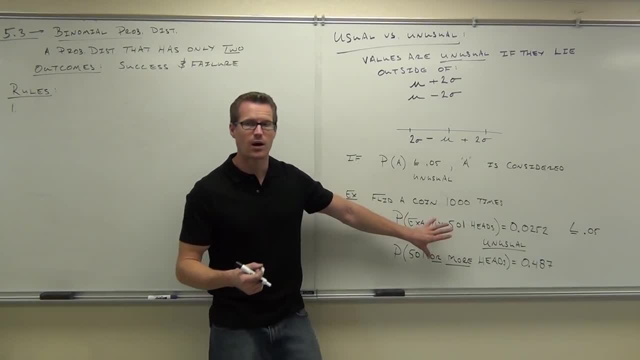 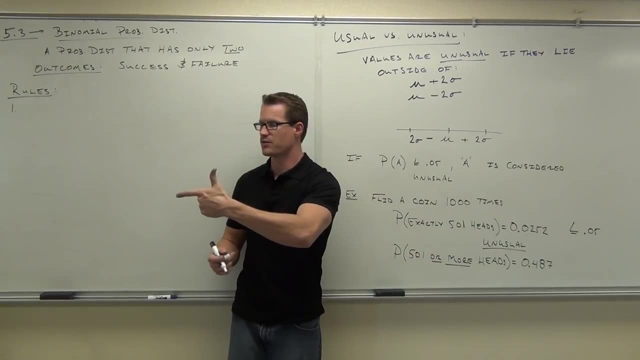 It's got to end somewhere. For instance, you're going to find out that this was a binomial distribution idea. You're flipping a coin. You're looking for heads. Heads would be a success, Tails would be a failure. Does that make sense? 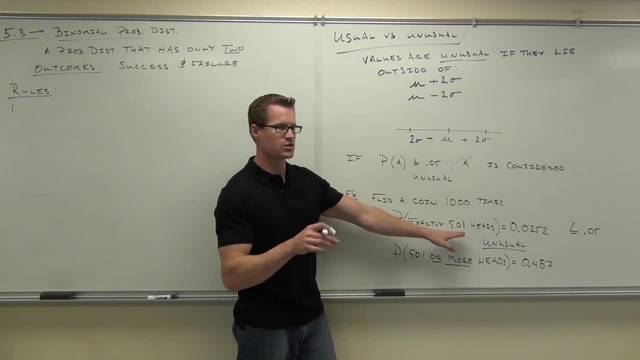 In this case, we were looking for exactly- hope- you listen to this terminology- exactly 501 successes. Does this make sense? In this case, we were looking for 501 or more successes, But it was out of how many tries That would be our trials. 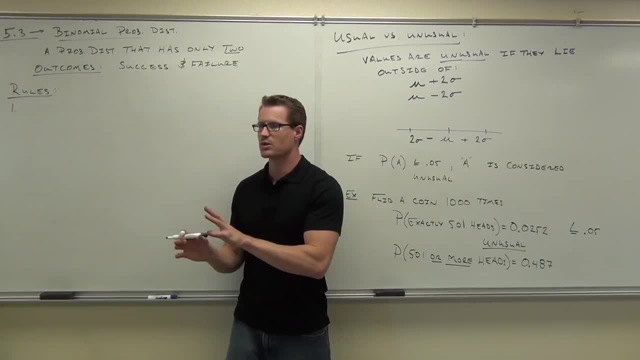 So we fixed that. We had to fix that somewhere so that we can work with our problem. So, number one, you have to have a fixed number of trials, You can't just flip the coin forever. Subtitles by the Amaraorg community. 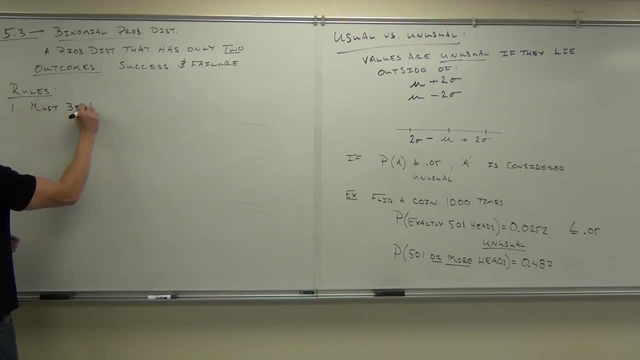 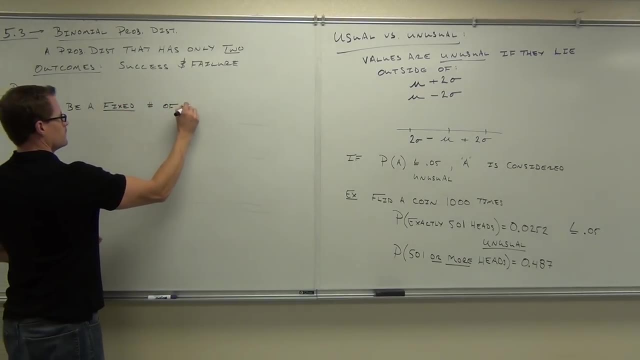 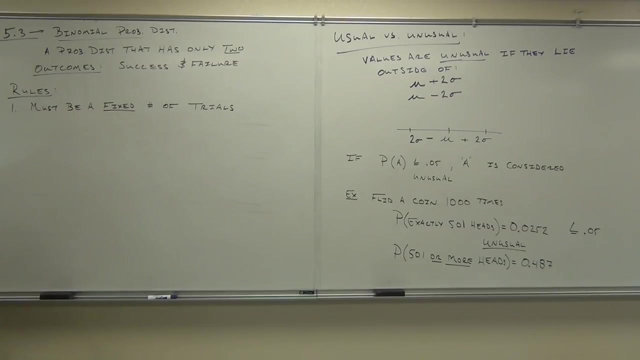 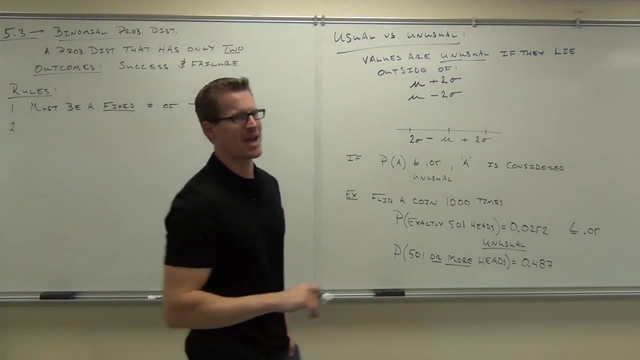 It must be a fixed number of trials. Number two: oh, this one's got to be there And you're going to be happy about this one, Trust me. Do you remember? well, you don't remember the distribution rule. We just found that out, right. 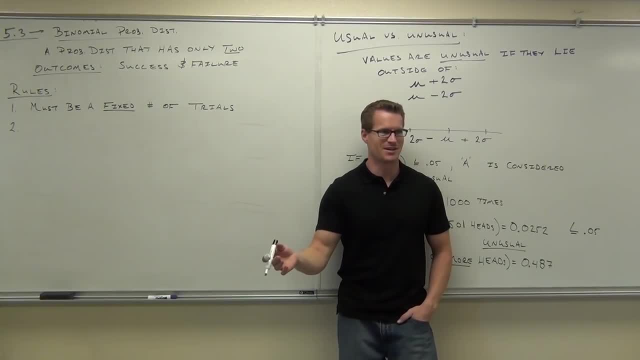 You're all going to be looking at the video. I'm going to have like 1,000 views tonight on that video for the distribution rule. But if you remember anything about the distribution rule now you've looked back at your notes, which you should do occasionally, I hope. 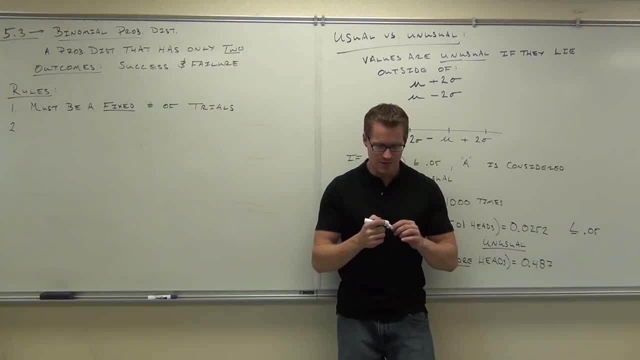 There's a long time between tests. When you look back at there you notice there was really. it mattered whether one probability depended on the other one, didn't it? It matters sometimes And we had to have it so that those things were independent. 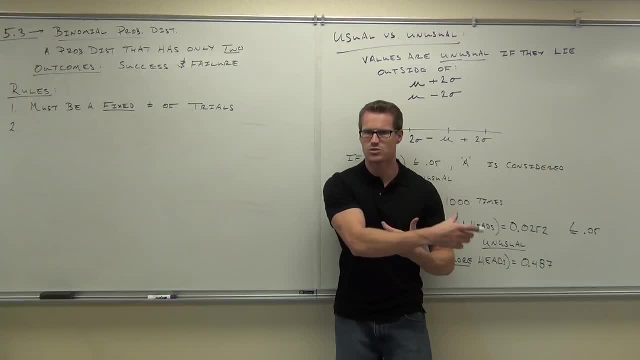 Otherwise, we had a carryover, We had a crossover. We had to subtract that out. Remember that When they could both occur at the same time, Or where one probability affected the other one, That would make a big difference if we were having several probabilities in a row. 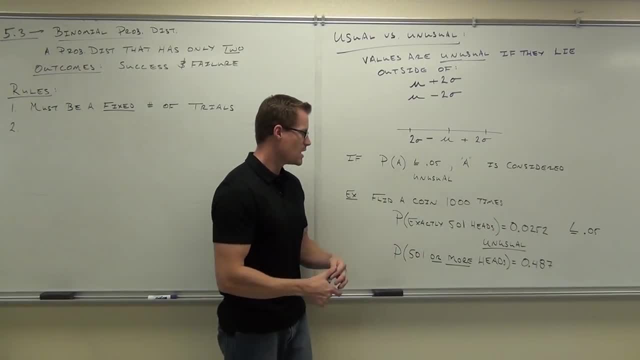 That would make a difference. For instance, let me explain it according to this: This one not so much Exactly 501, that was just one probability, But this one 501 or more. If you are flipping a coin and what you get the first time affects what you get the next time. 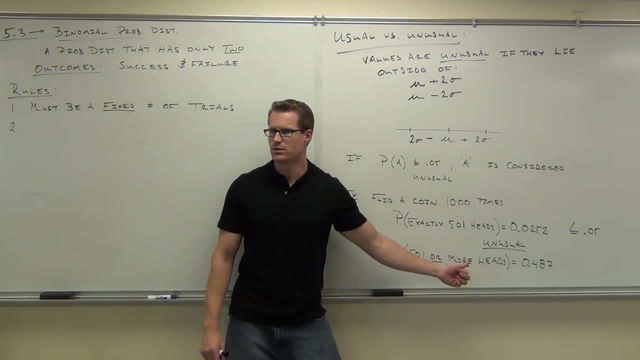 adding all these probabilities up would be extremely hard to do Right, Because 501, getting that head would affect the 502nd or the 503rd or the 504th And you would have a huge, massive thing to deal with. 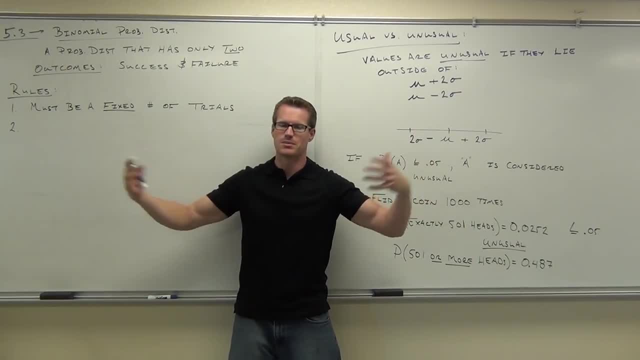 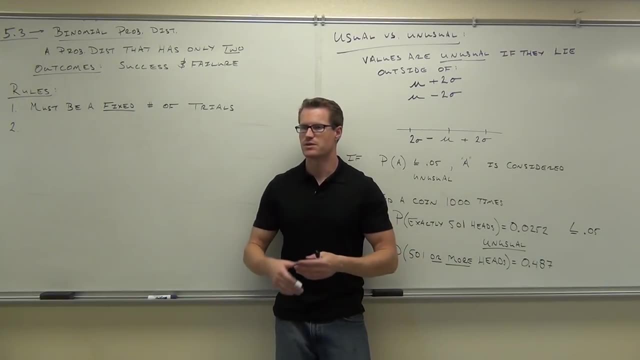 Do you see what I'm talking about? So these probabilities have to be completely independent, not based on each other. Which means: I flip a coin, everything resets. I flip a coin, everything resets Back to 50-50.. Every single time. 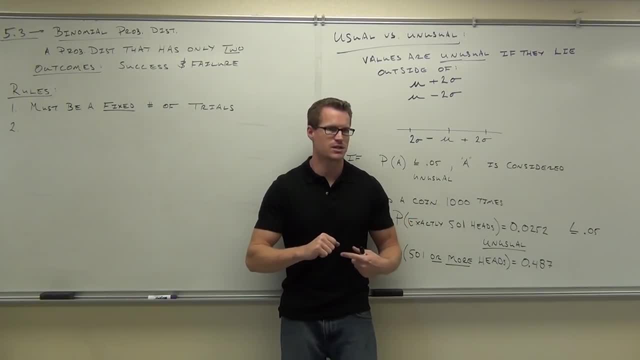 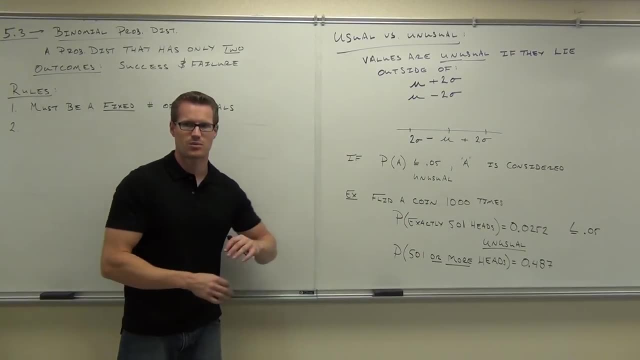 I roll a die, I pick it up Back to one-sixth chance for all those sides. Are you with me on this, folks? They've got to be independent. They cannot. the probability of one outcome cannot affect the probability of another. 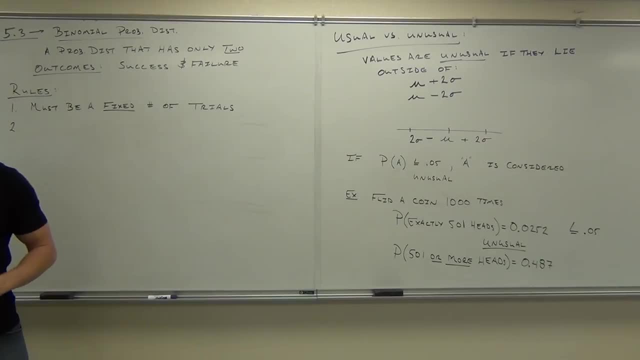 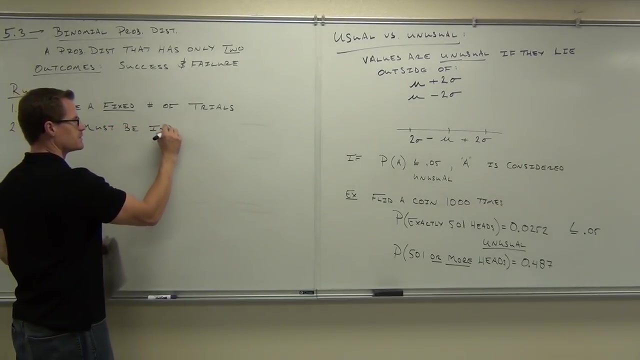 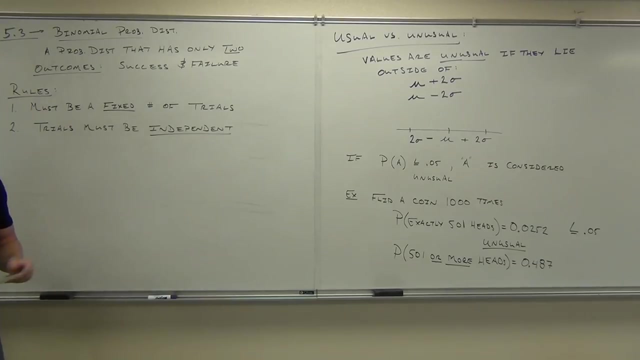 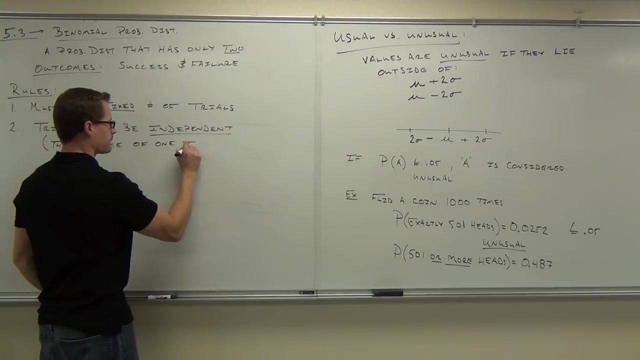 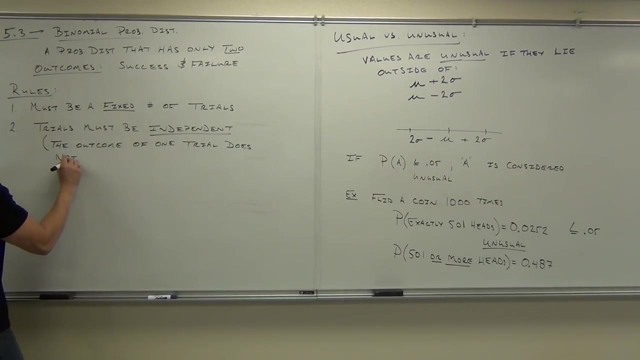 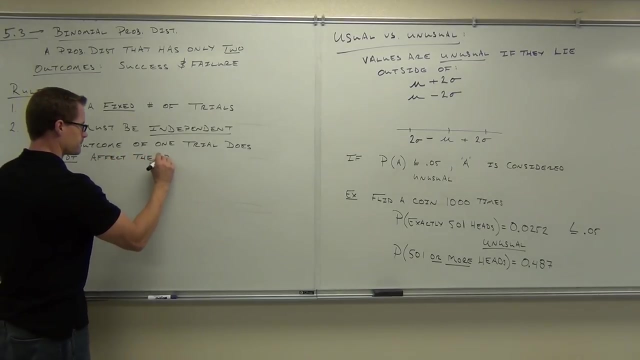 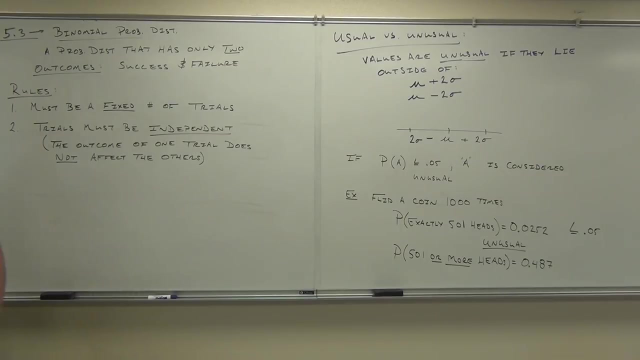 Or I should say the occurrence of one outcome does not affect the others. Trials must be independent. That means the outcome of one trial does not affect any of the others. That means the outcome of one trial does not affect any of the others. 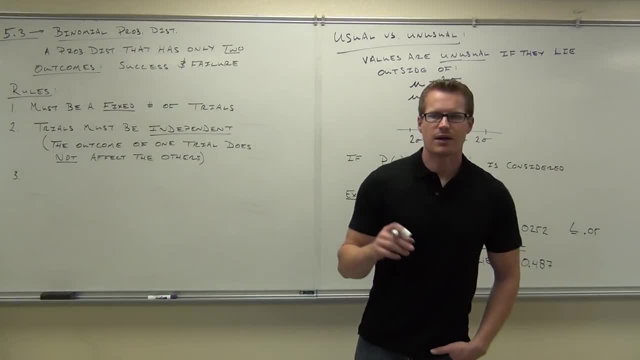 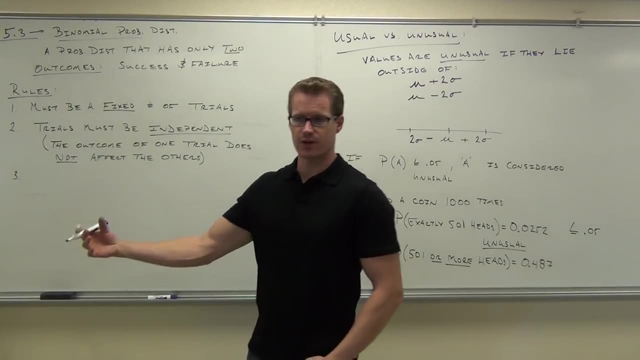 Third, this is where we get the binomial part. We just spoke about this. Each trial has to have only two outcomes: Either a success or a failure, Or once you qualify a success, once you categorize a failure. So each trial has only two outcomes. 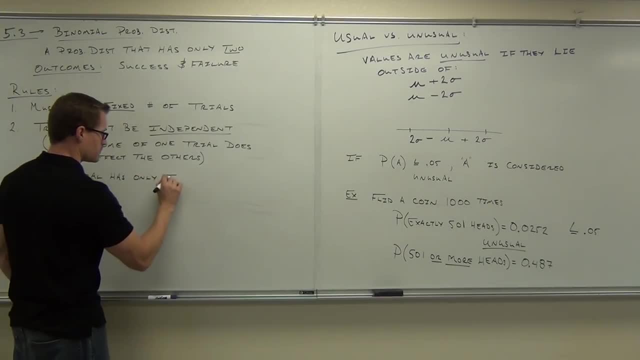 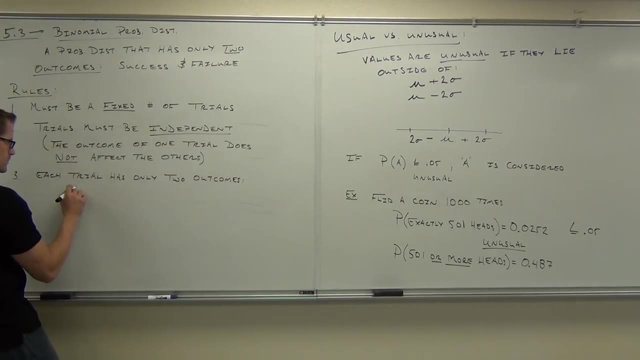 So the problem is which one of the two outcomes is the point, Either one or the other? Let's see. I have a bunch of results here. They all look pretty good as a result, but you can't set up a good one for this one. 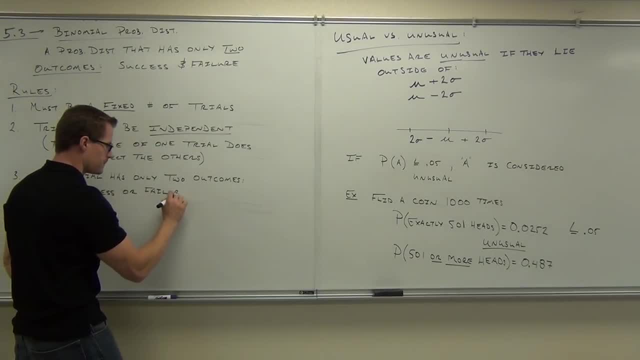 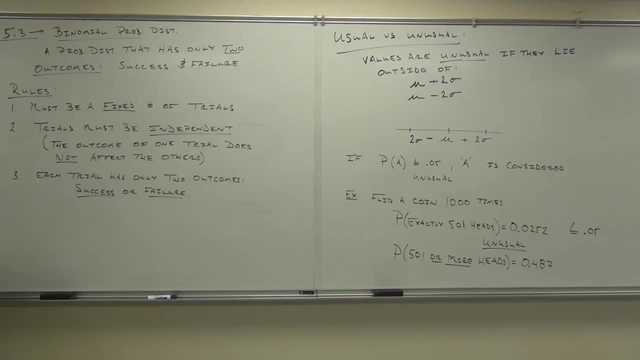 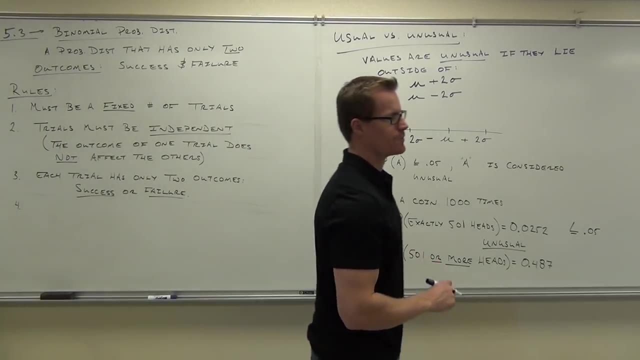 What do you do? You just kind of get good results, don't you? And there you go. You don't get pretty good results, don't you? No, Okay, I think I'm doing all right. And number four: the probability of a success has to say the same for each trial that you 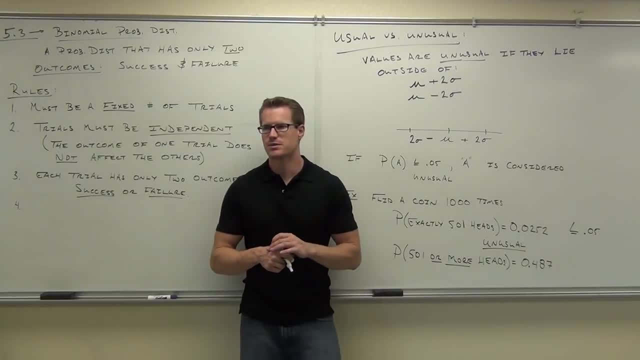 do. For instance, if we're flipping a coin a thousand times, we're not going to go halfway through and say, oh, we're going to switch coins and this one has more of a chance of beating heads. That wouldn't work so well for us. 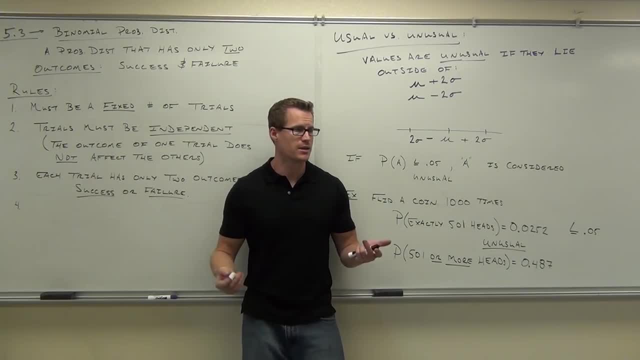 So the probability of getting a head has to be the same every time. If we're rolling a die. the probability of rolling a three- if that was our success- would have to be the same every single time. it can't change. So we could do this with a way to die. it would just have to be that the probabilities 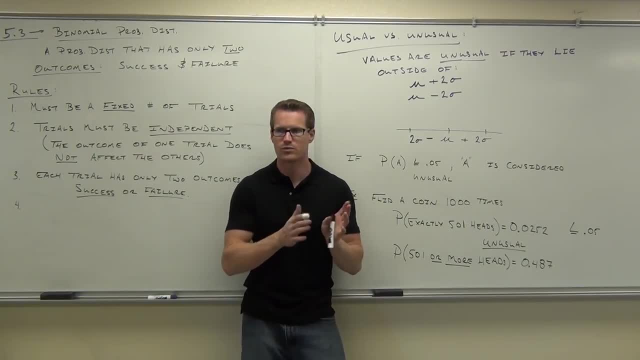 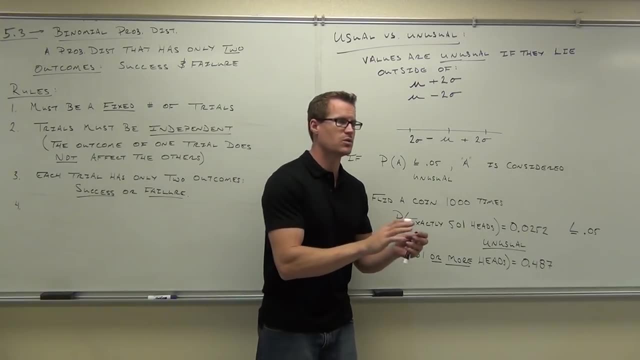 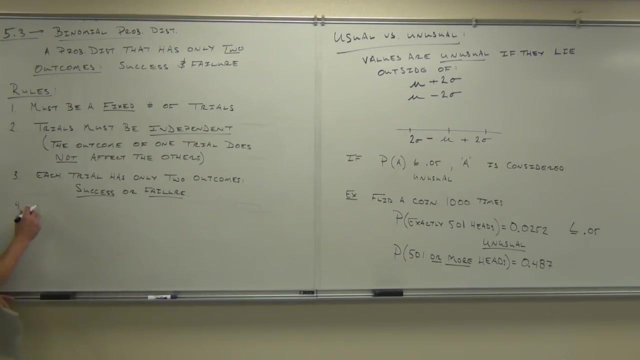 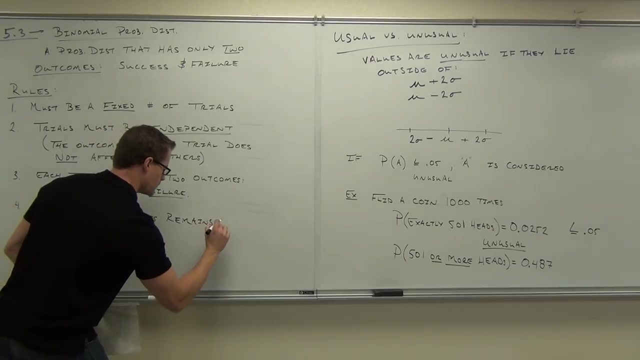 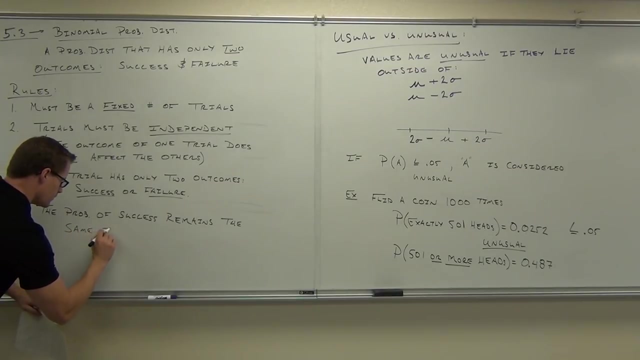 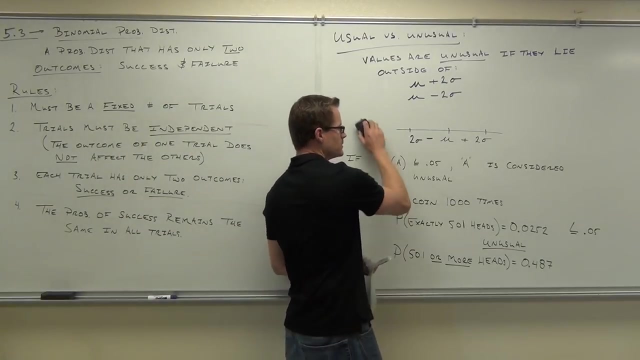 don't change halfway through my experiment or a quarter of the way through, or vary by trial by trial. Are you with me on that? Yes, So every time you repeat the trial, the probability of a success is the same. Okay, there is some notation that I've got to give you. 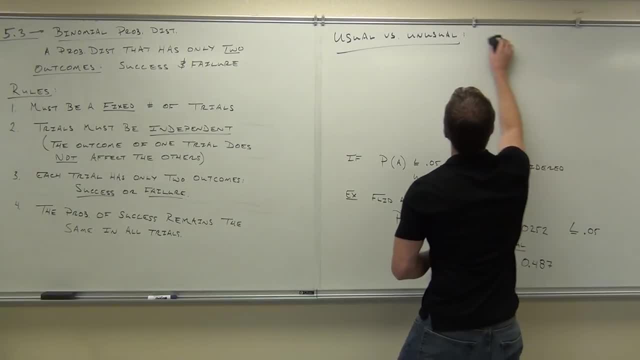 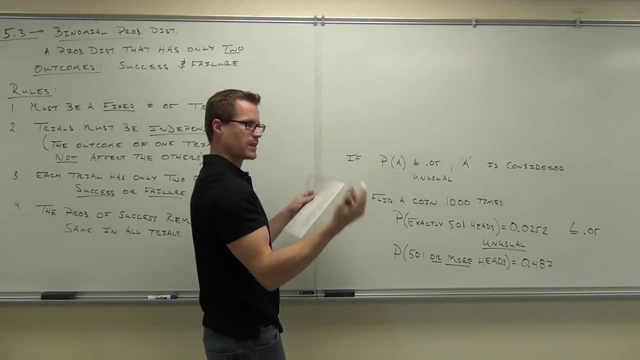 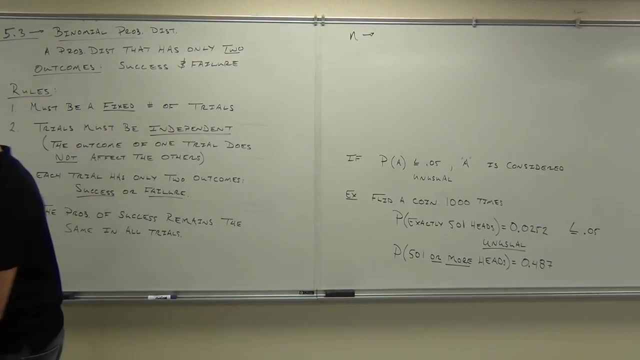 Okay, Okay, When we're dealing at a binomial probability distribution, we've got some letters we've got to deal with. First one is n little n. Little n usually stands for the number of things right, The number in a sample. 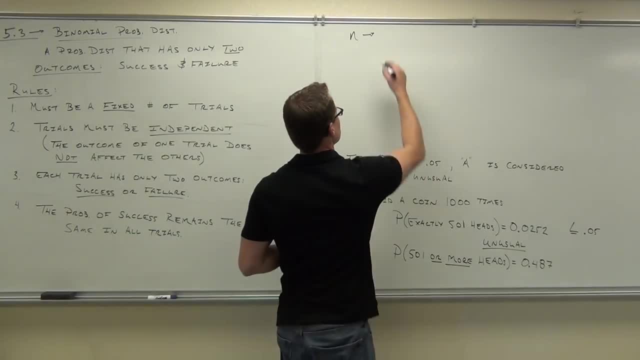 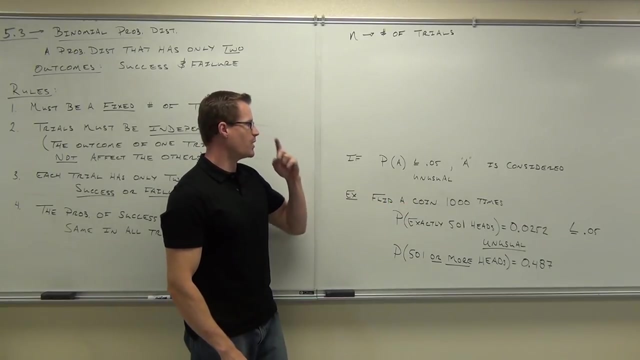 In our case, n stands for the number of trials we're repeating- I'm going to do this down here as well- kind of refer you back to this example. that's what I left on the board. But if we're doing this example, what is our n in this case? 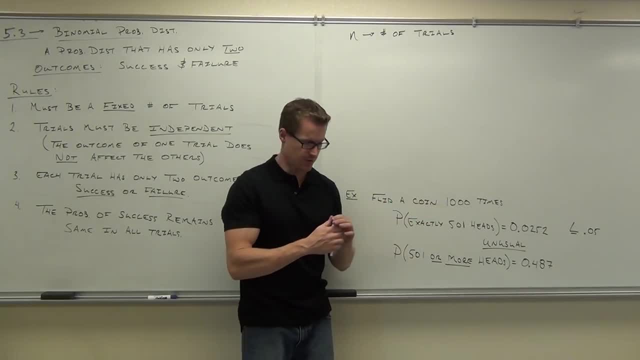 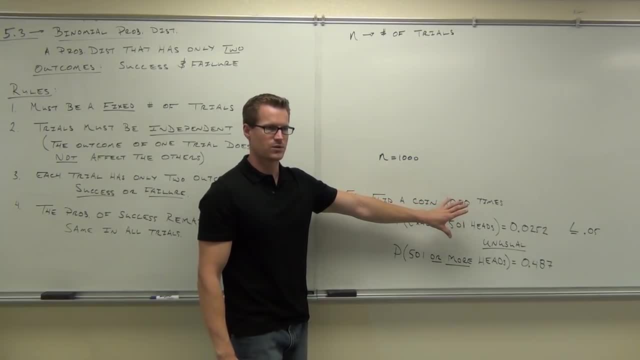 Don't get those two confused. just rewrite that, Or we're going to do several more examples. so just kind of keep this one in your mind right now. okay, Trust me, we'll do more examples. I don't want you going back, because that was not the idea at the end of section 5.2. 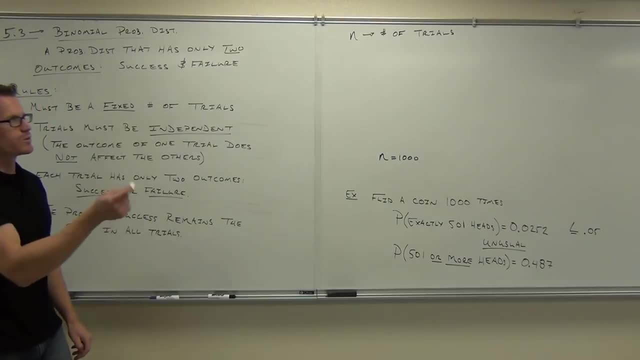 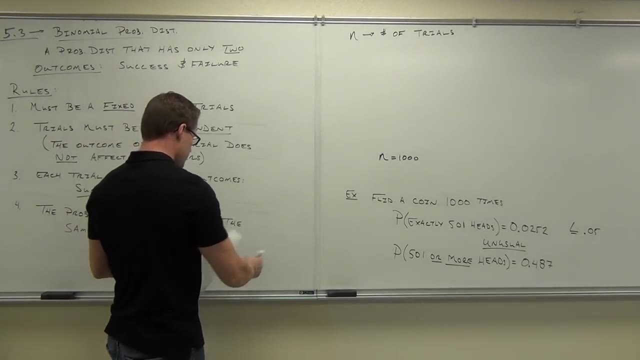 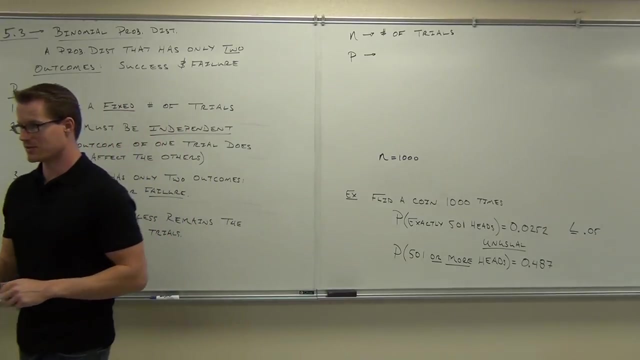 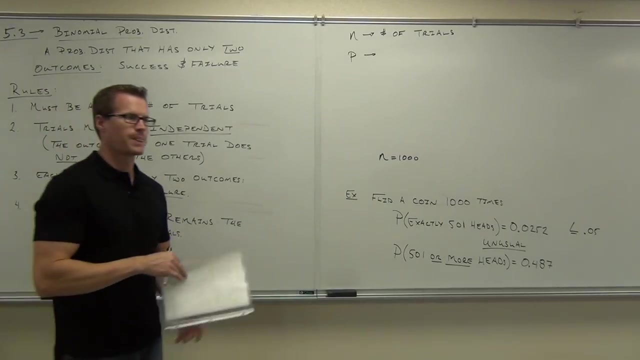 It was a 5.3 idea, So number of trials n would be 1,000 in this case. that's how many times we're repeating that procedure. There's a couple of other letters. One of them is p little p, not big. P little p- lower case. 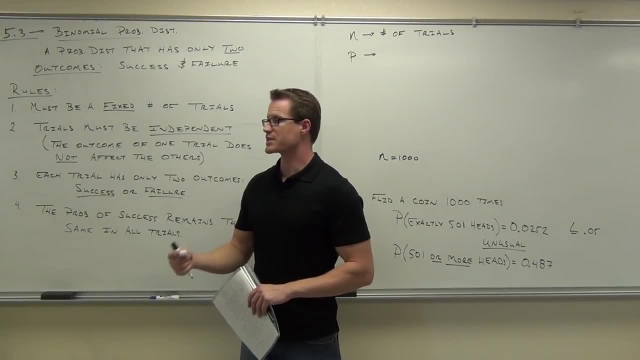 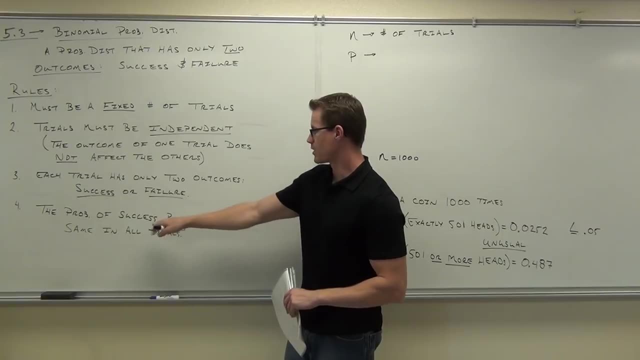 Little p stands for the probability that you are going to get a successful trial. Is little p going to change throughout your procedure? No, that's what we said right here. Little p is going to be the probability of getting a successful outcome in each individual. 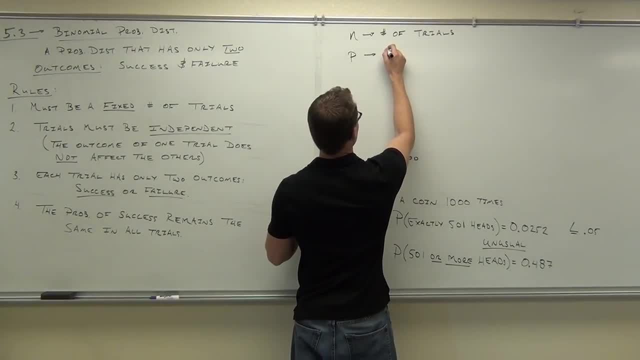 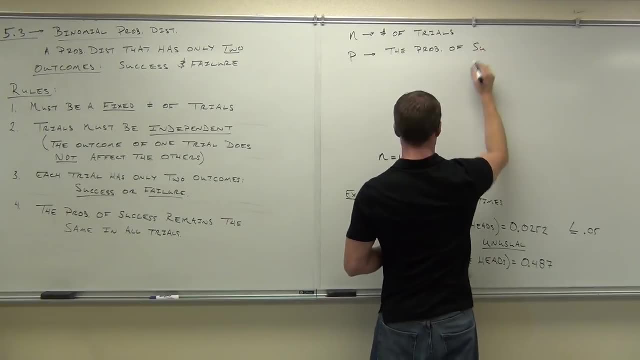 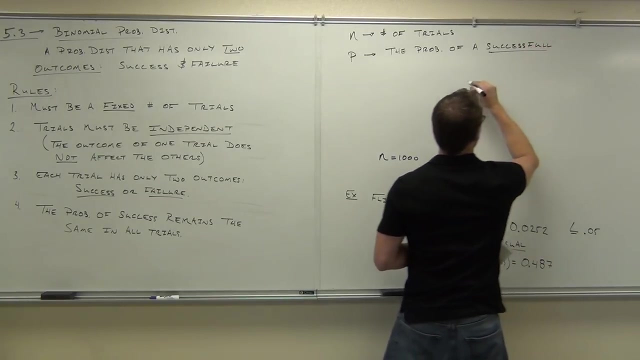 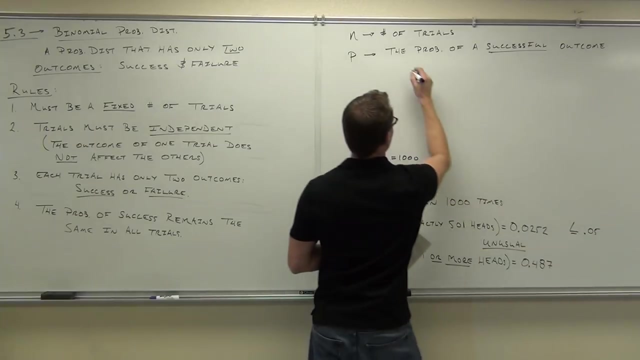 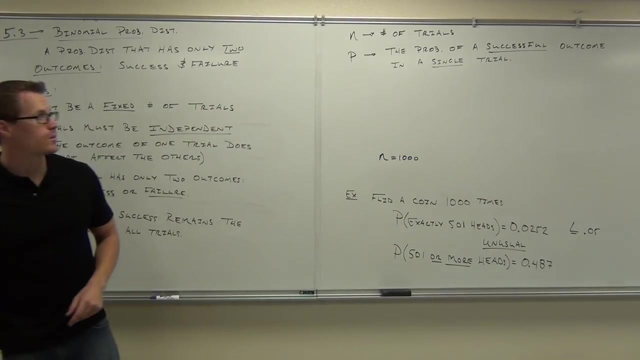 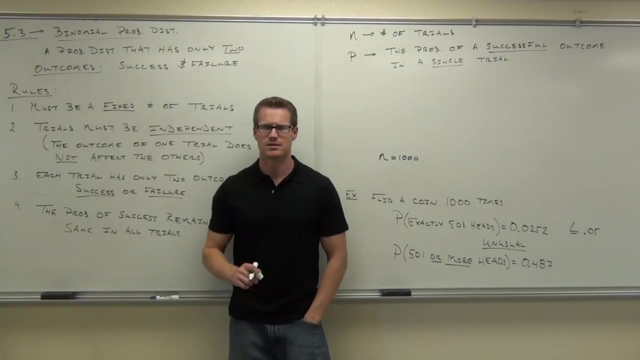 trial: The probability of a successful outcome for each trial. Okay, So put in a single trial the probability of a successful outcome in a single trial. Okay, what's the opposite of the letter p, Q, Q? Well, obviously it's written backwards right, so Q. that makes sense. 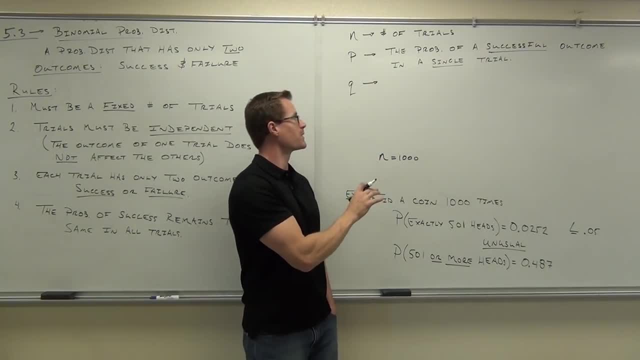 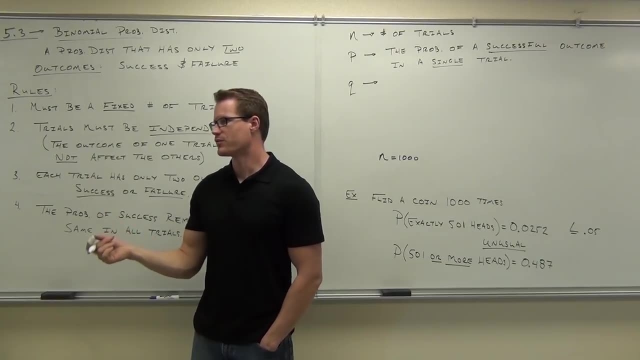 If little p stands for the probability of a successful trial, the probability of a successful outcome in a single trial, the probability of Q stands for what do you think? the probability of failure, Failure, Failure, Mm-hmm. This is the probability of a failure. 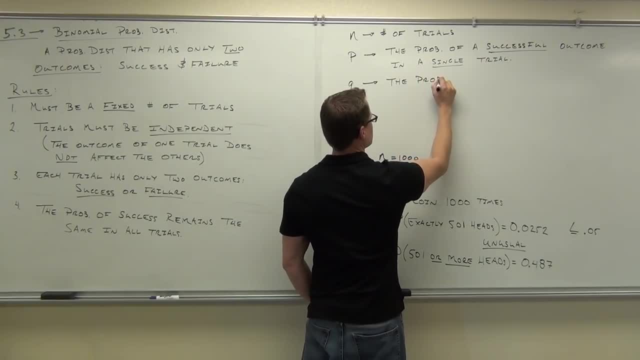 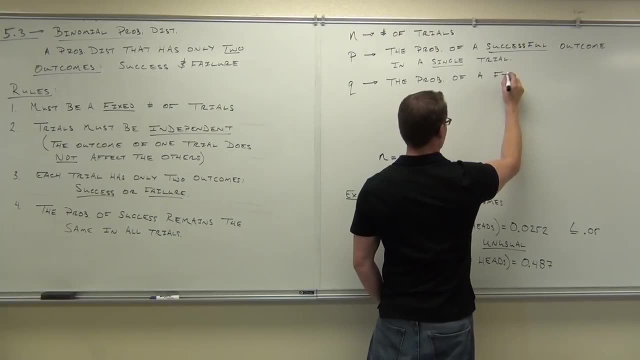 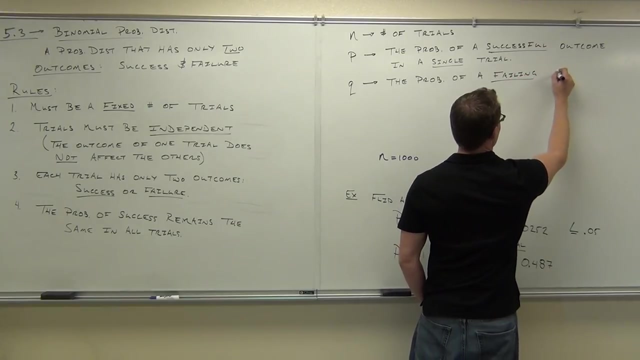 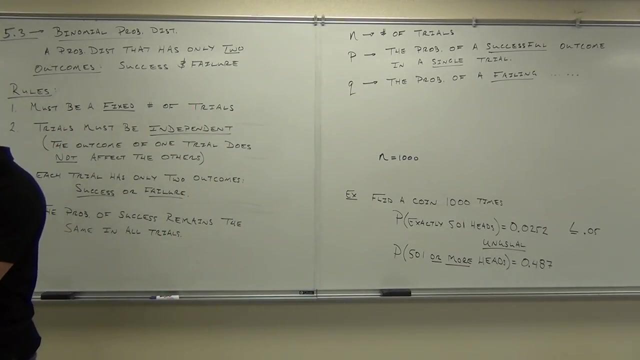 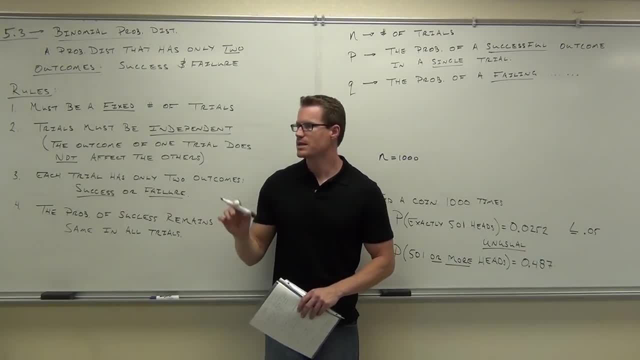 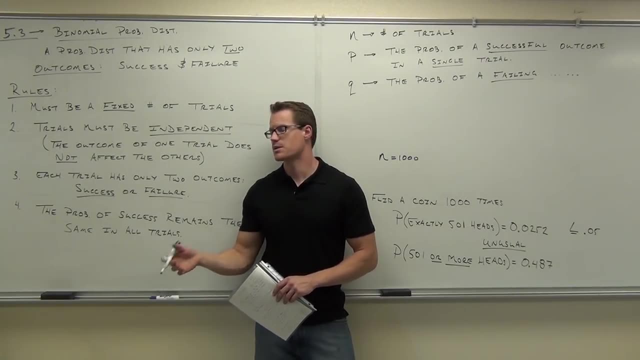 Failed Failure, The un grooming Samsung. I think that suchenger doesn't have to Talk about it in English, right, Your child will talk. It'll just Talk about it is a probability of a successful trial. you'll also be given that. the same with Q. 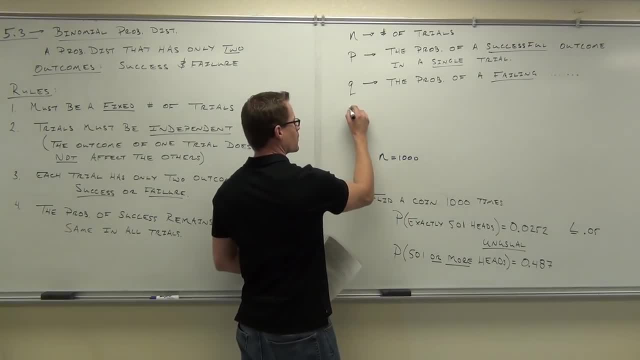 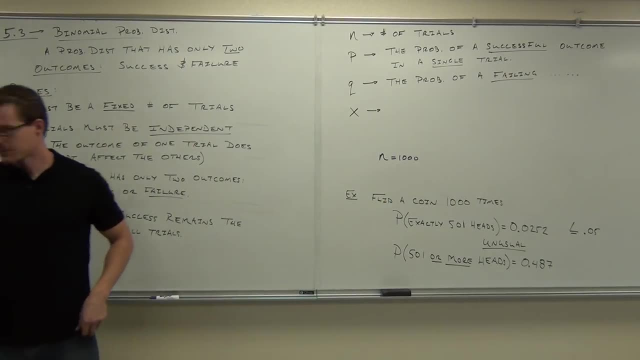 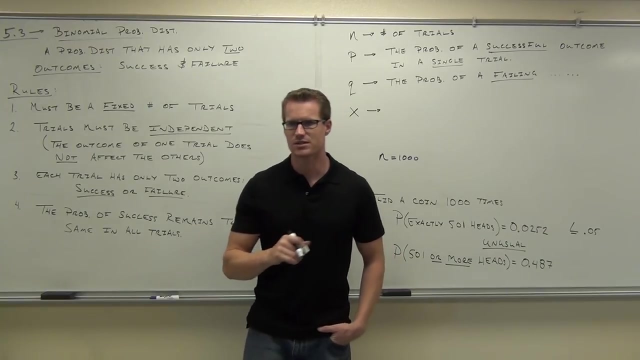 You have to be given those things Also. what you're looking for is the X. In our case, the X is the number of successes that you're looking for. Okay, the number of successes that you're looking for, Or the number of successes that occur in the end trials. 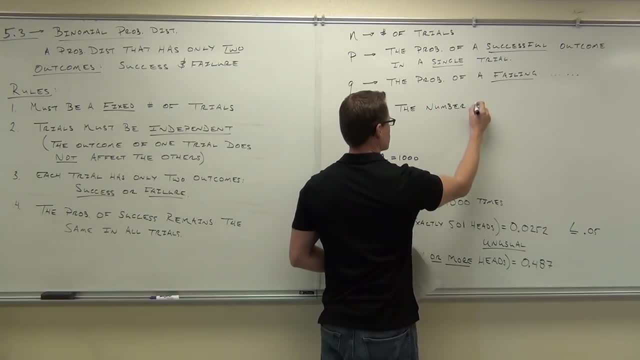 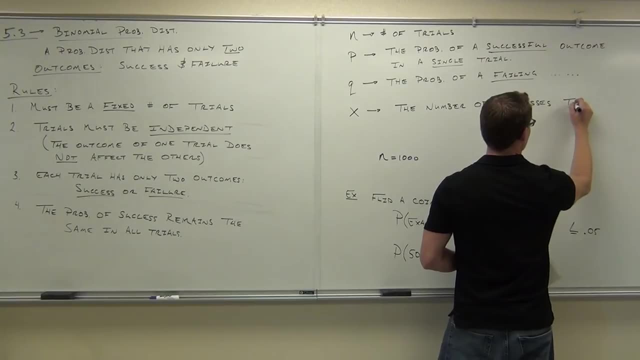 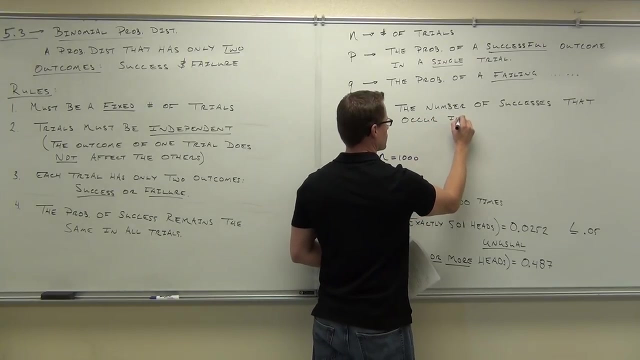 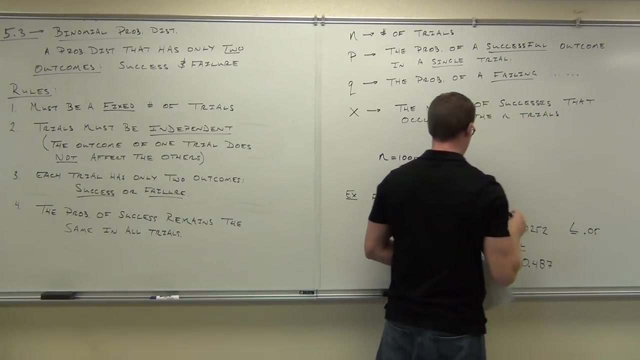 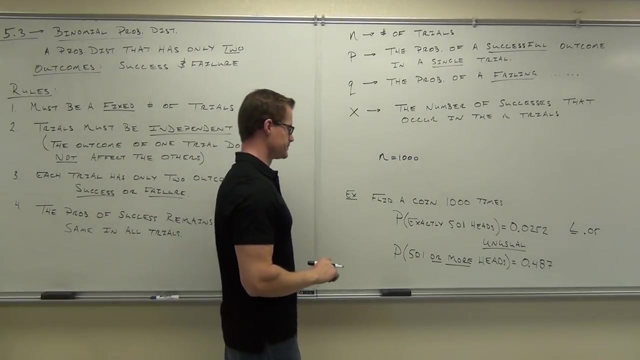 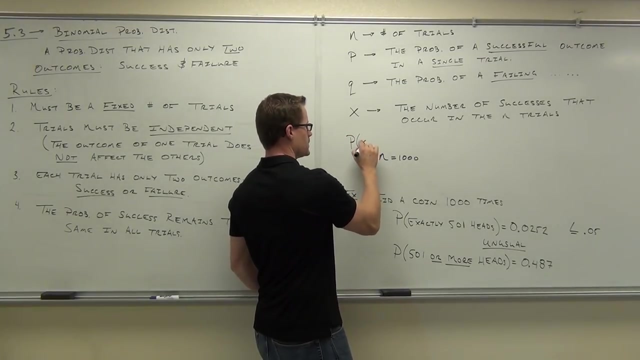 Okay so the number of successes that occur in the end trials. Okay, so the number of successes that occur in the end trials. Okay, so the number of successes that occur in the end trials. One last, one big letter: P. It's always with the of X, P of X. 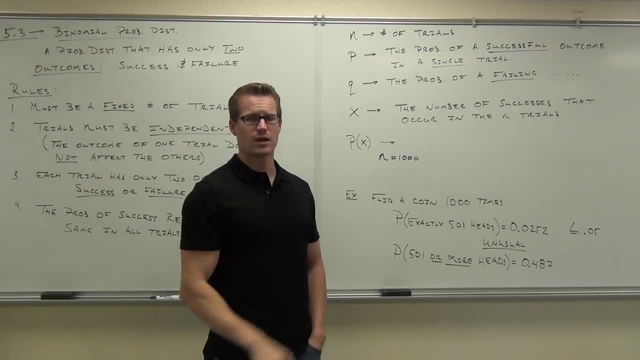 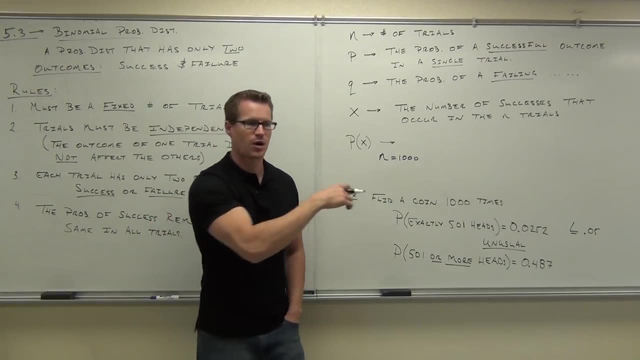 What's that big letter P stand for Probability? It's probability. What's the X stand for, again, Number of successes? It's the probability of getting that exact number of successes. okay, This is the probability of getting this many successes. 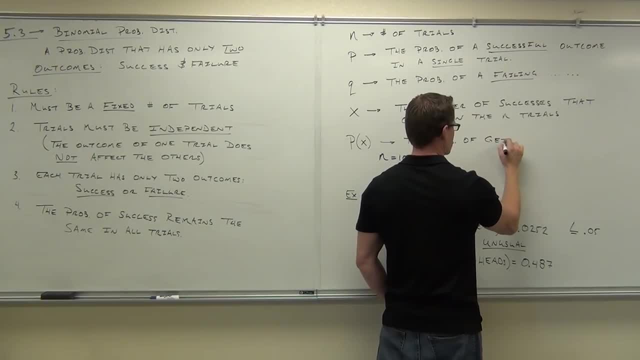 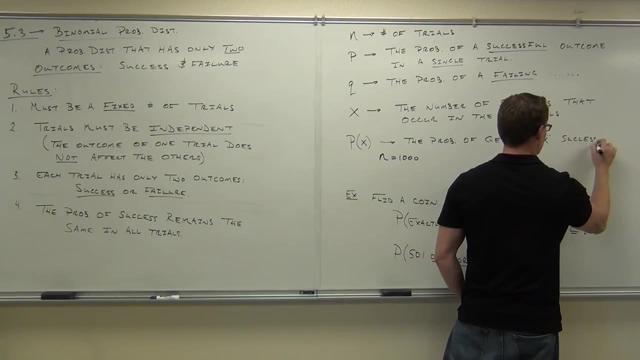 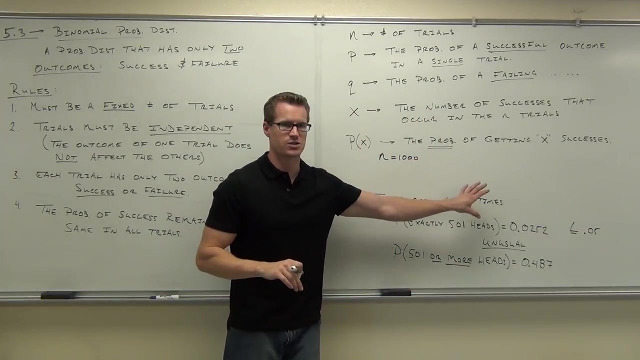 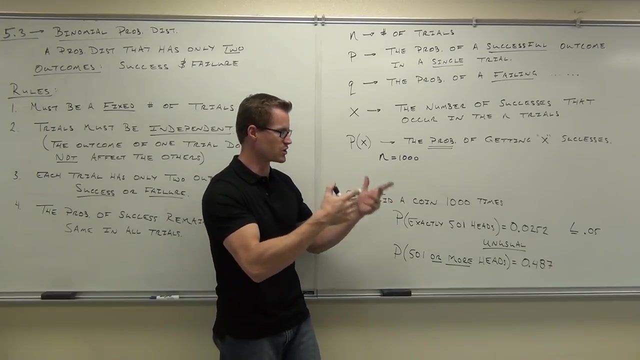 Okay, we're going to fill all the rest of this out. We're going to identify these items in just a second, But before we do, I need to make a couple things really, really clear for you. So put your pencils down or just stop, or pause for a second and just listen. 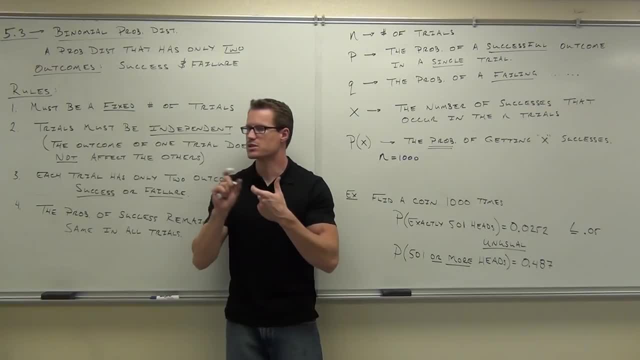 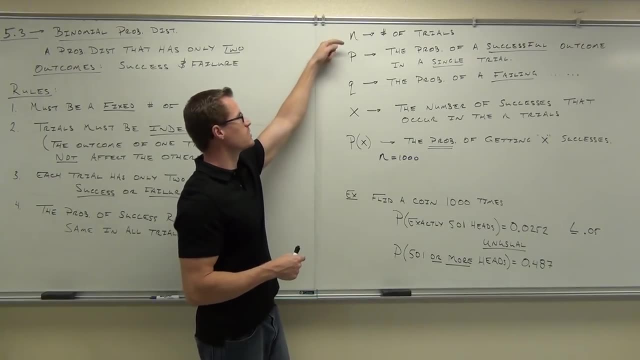 When we're doing these things. a lot of students get really confused with some of this terminology And usually people are pretty good with the N? N's- just a number of times you're repeating something, But they get really confused between this one, this one and this one. 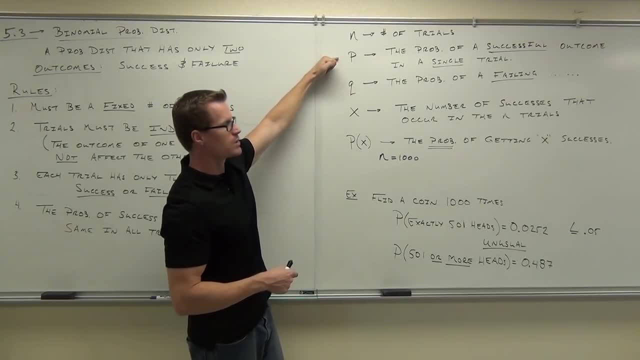 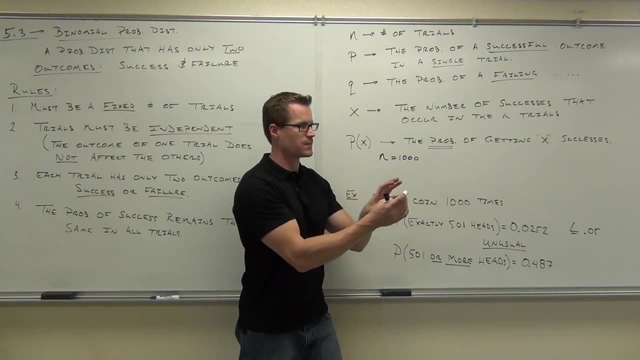 Okay, these are tied together. This is a probability, sure, but this is just a number. Okay, here's the difference between these. X is the number of successes you want, P, lower case letter. P is the probability of each. 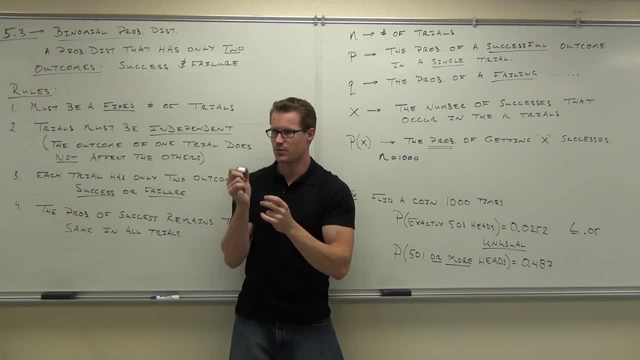 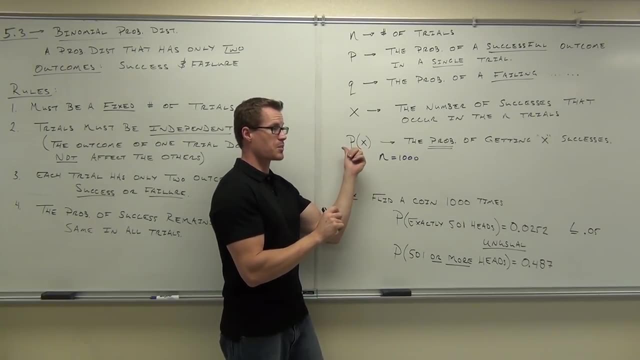 of those successes happening, The probability of one single success occurring in your trial. That's what that means. What this probability means is the probability of getting that many successes. So is X a probability? Is X a probability? X is just the number of successes you're looking for, whatever that happens to be. 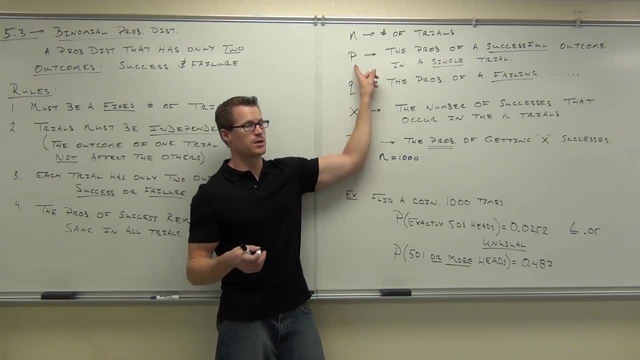 X is the number of successes you're looking for. Is this a probability? Yes, That's the probability of each one of those successes is happening. successes: is each one of those successes is happening? okay, over and over and over and over again. 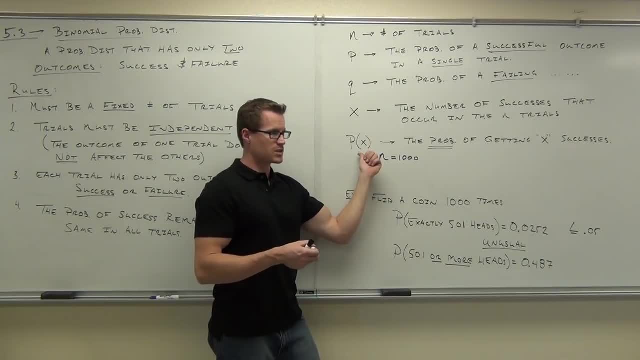 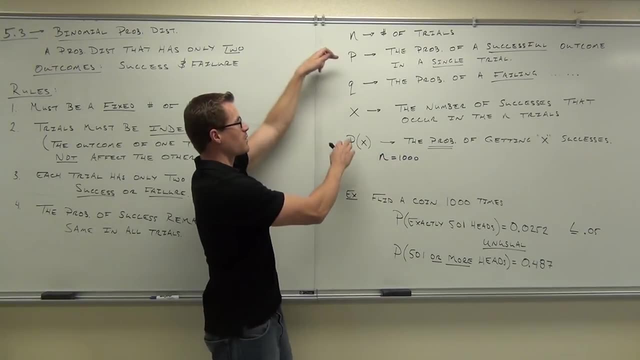 This? is this a probability, Definitely? This is the probability that you're going to get all of these successes, exactly that amount of successes. Do you see the interplay between them? These are both probabilities. This is trial by trial. This is overall, which is based on your number. 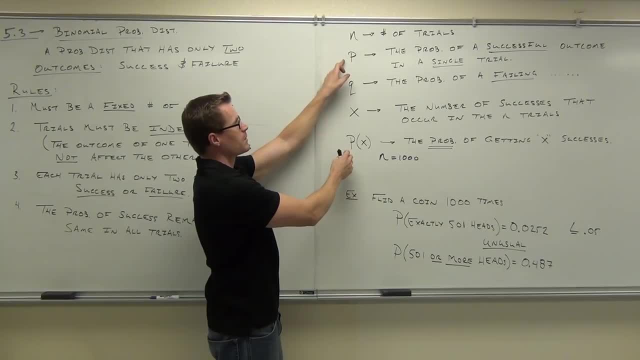 of successes you're looking for. Okay, so this probability of each success that you get, This the number of successes you're looking for, This the probability of getting that number of successes. So let's go ahead and fill out the rest of the stuff. 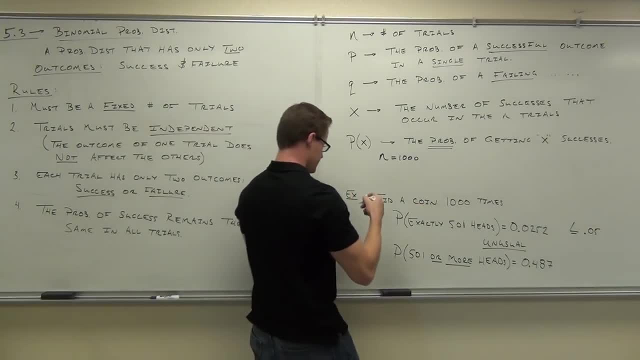 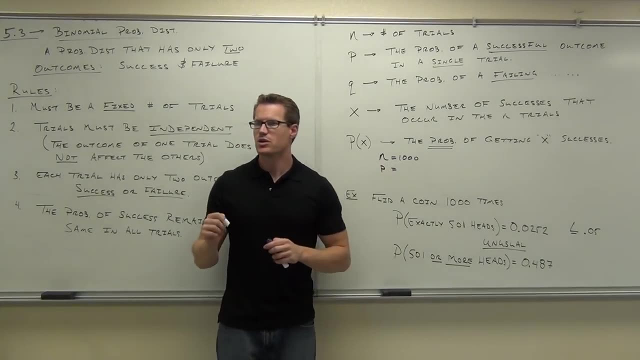 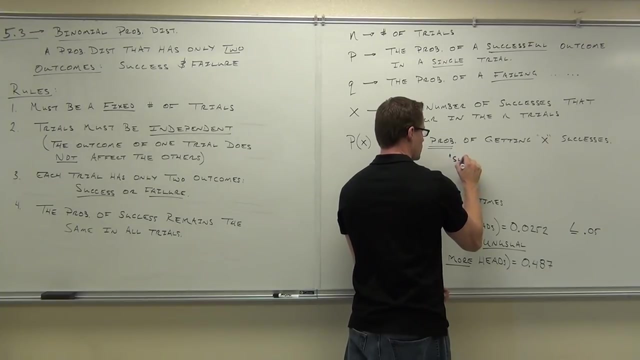 We knew N was 1,000. We're going to look for P little p. Little p is the probability you're going to get a successful outcome. Now, in our case, what is our success? in our case, Head, What was it? 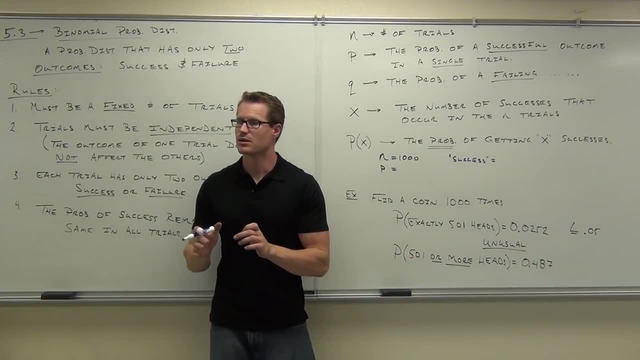 Head, Head, yeah, getting a head. And then I list a success. please listen carefully to this. a success is not getting a head, Okay, Okay. A success is not getting 501 heads. A success is not getting 501 heads. 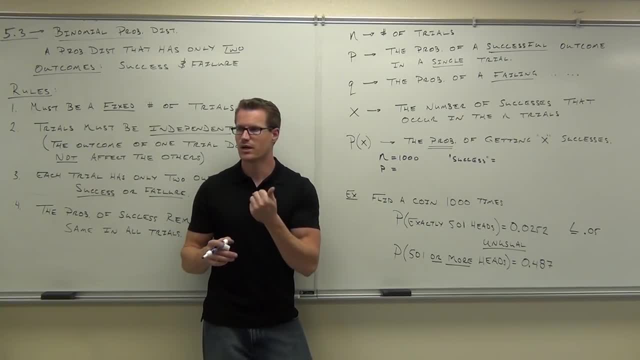 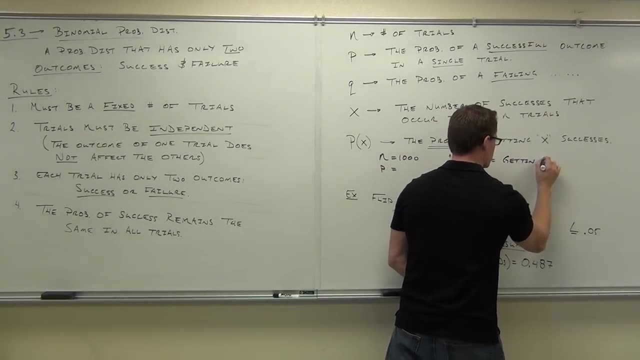 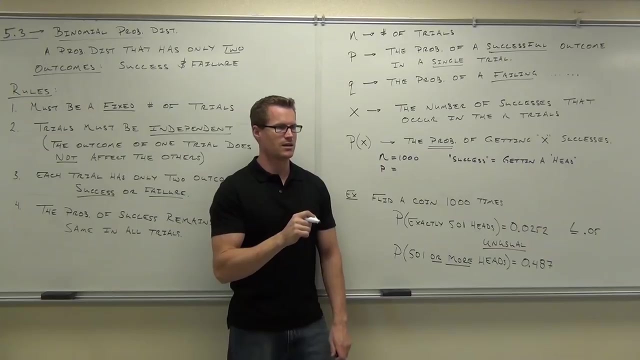 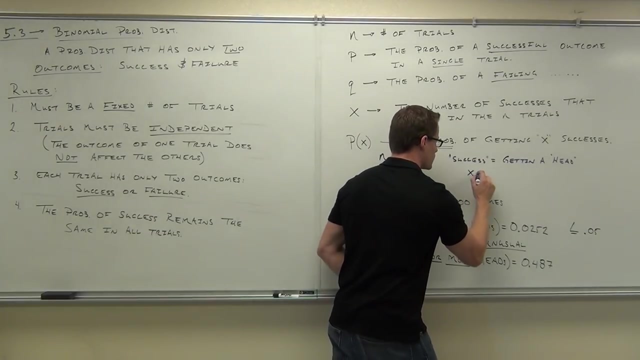 A success in this procedure is getting a single head. That is a success. Success is getting a head, just one. Why do I say that? Well, it's because when we look at X- X counts up- notice the difference here. 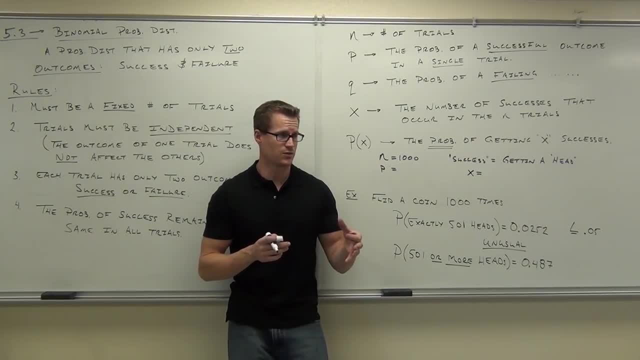 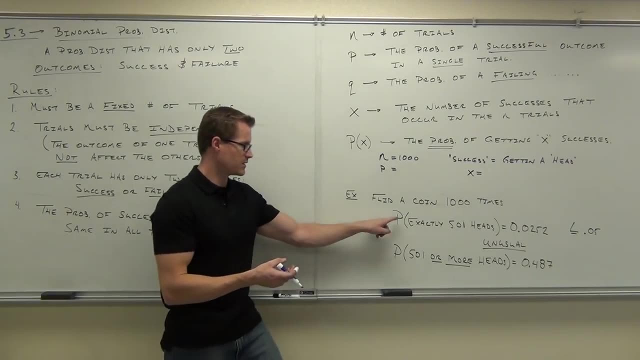 X counts up the number of successes we're looking for. The number of successes we're looking for. How many successes are we looking for in this example? How many successes right here are we looking for? 501.. That's what we're looking for. 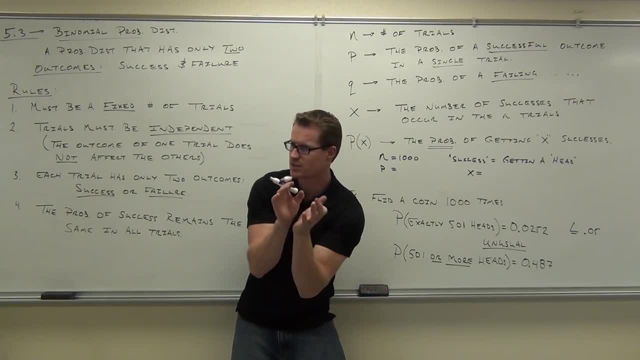 Notice the difference. The success isn't getting 501 heads. The success is getting one head. We're just looking for that to happen. How many times? 501 times? That's where X comes in. So success is getting a head. 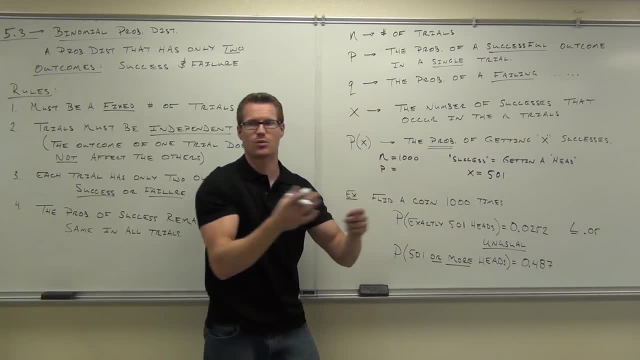 X. we're looking for 501 successes. That's how that plays in there. We're looking for 501 successes. What's the probability of getting one success? Flipping a coin- assume it's a standard coin. Flipping a coin is. 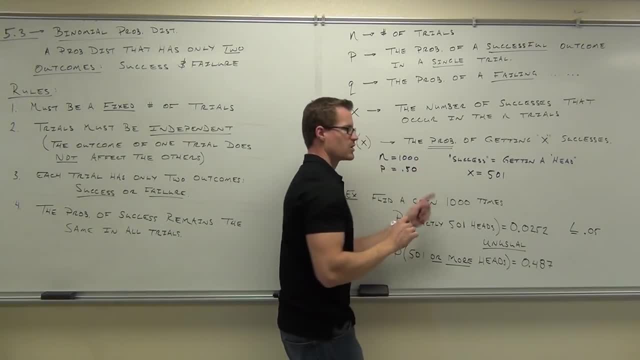 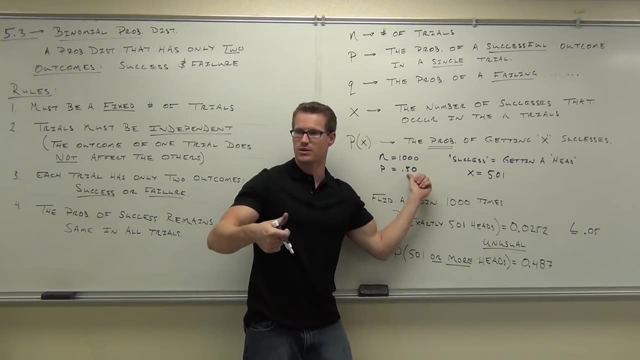 Notice how you have to identify a success as a single. Look at the board. Notice how you have to identify the success as a single, because it's a probability. It's based on one single outcome. You have to do that. X is yeah, that's the number of successes you're looking for. 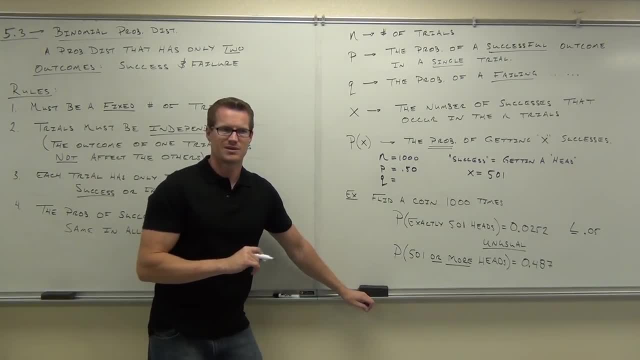 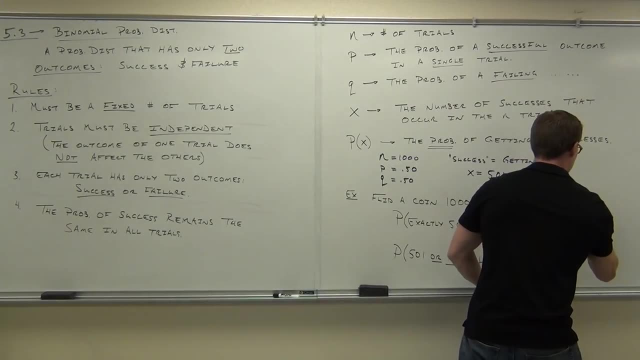 If P is .50,, how much is Q? Yeah, Why? One more thing, The last thing we'll talk about: How much does P plus Q have to equal? For sure, Probability of success or failure. you only have two outcomes, right. 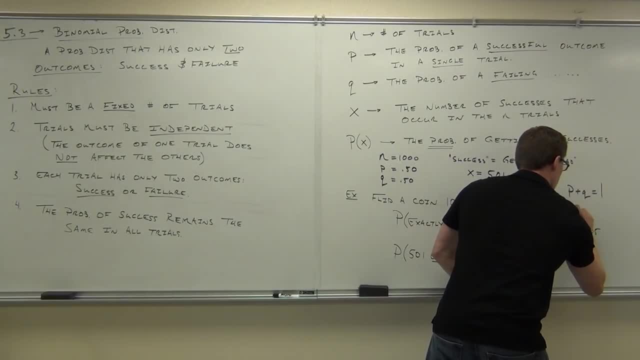 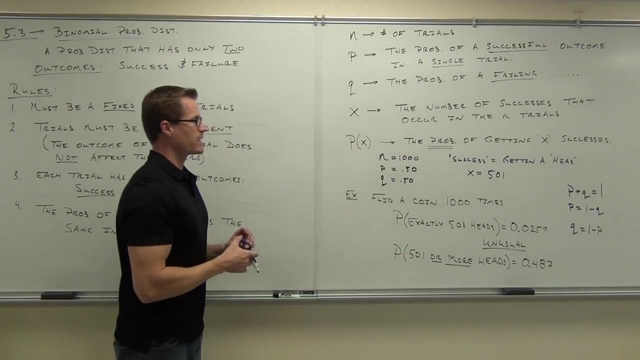 It's got to be one. This also leads to P equals 1 minus Q, P subtracted, Or Q equals 1 minus P. The only thing we haven't done is figure out this, but we're going to go ahead and figure that one out next time. 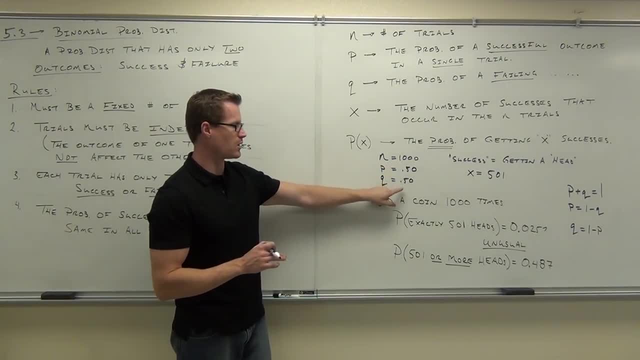 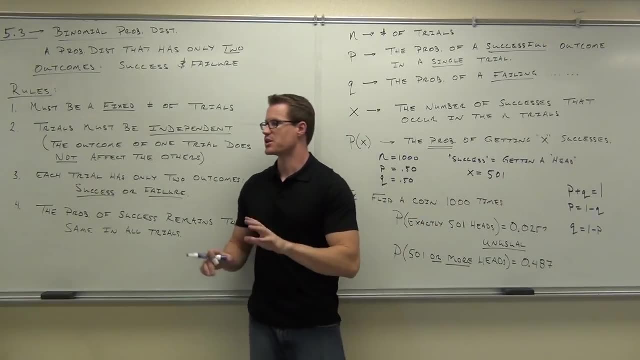 So we now know N. We know probability of success for a single trial, probability of failure for a single trial. A success is a single outcome. It's a single outcome. X gives you the number of successes that you were looking for. How many would feel OK with what we talked about so far? 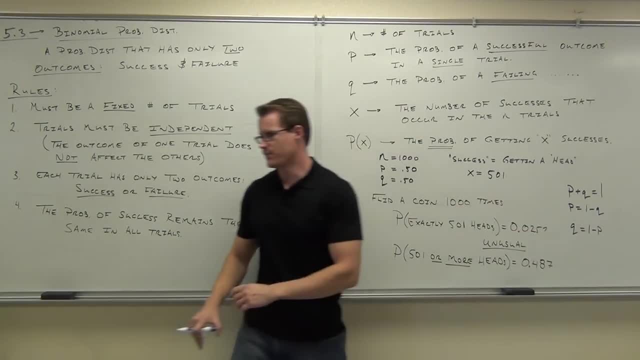 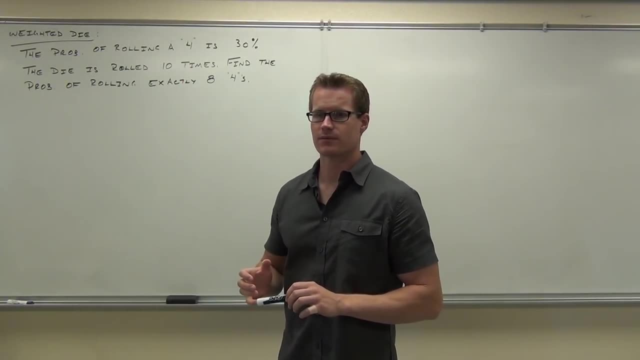 Do you all feel OK with this stuff that we did Very good. Can you put up the formula like? I know there's going to be a formula, but I'd like to see the formula like I'll put it up there in a minute. 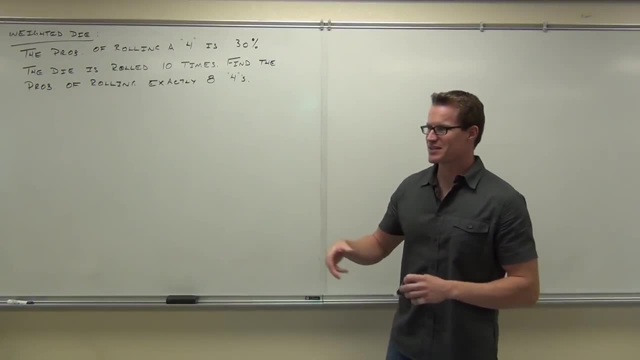 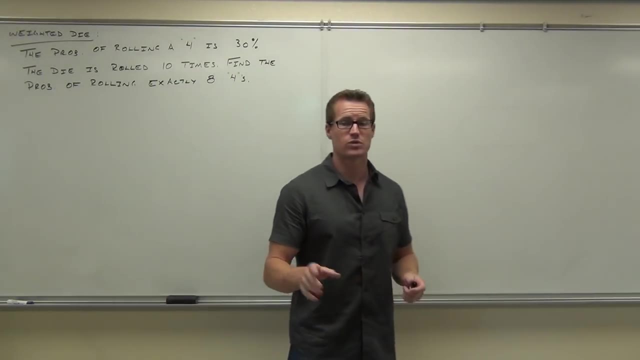 Don't worry about it. So we're trying to figure out these binomial terms Basically. this is what I want you to understand right now. What is our N, our lowercase P, our Q, our X? The probability of X we'll deal with in just a second. 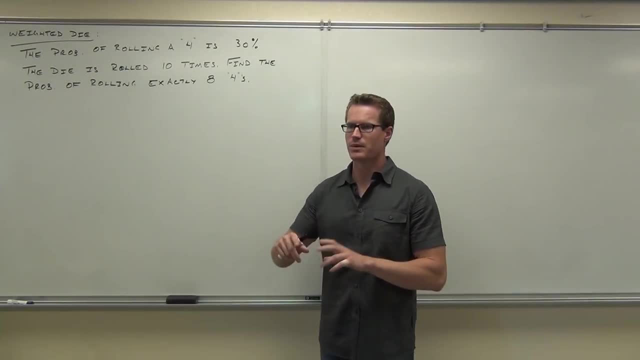 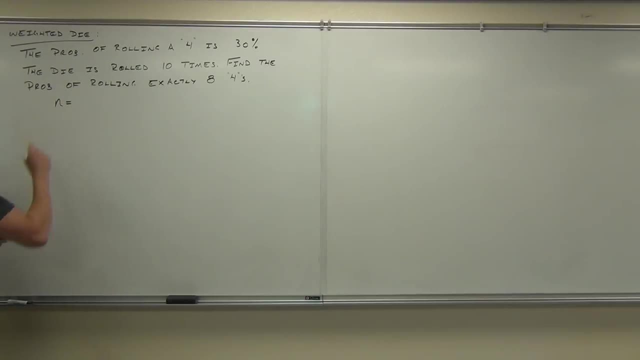 So we're looking at binomial probabilities, We're realizing that binomial means either success or a failure and we need to identify all of these letters. So N, which we just talked about, was the number of trials that we're having to occur in our whole entire procedure here. 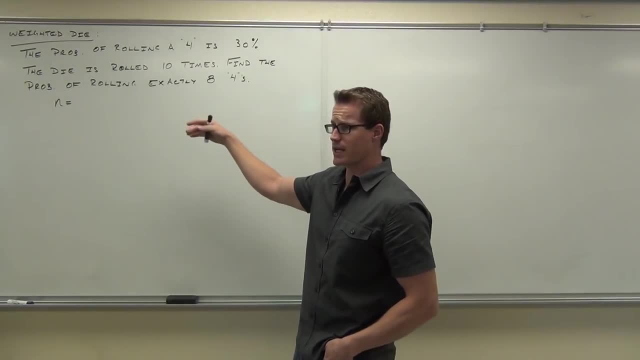 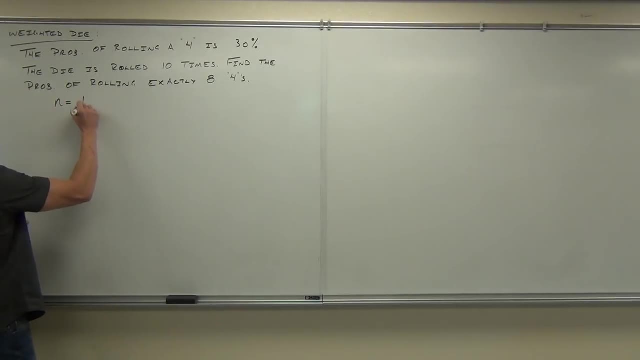 So how many trials are we dealing with in this particular weighted die problem? 10.. Yeah, we're rolling the die 10 times, So this trial is being repeated 10 times. So, yeah, N is 10,, for sure N is 10.. 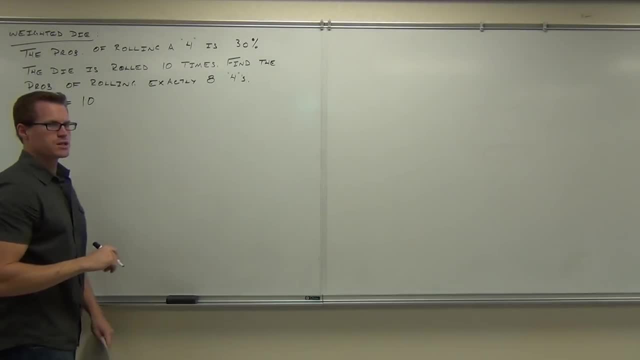 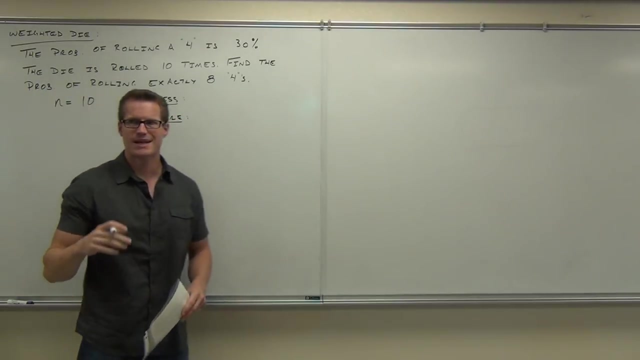 Let's go ahead and let's look for the probability of N. Well, firstly, we need to identify something. We need to identify what is our success and what we're considering to be a failure. I want you to identify these, Even if your problem doesn't ask you for it. 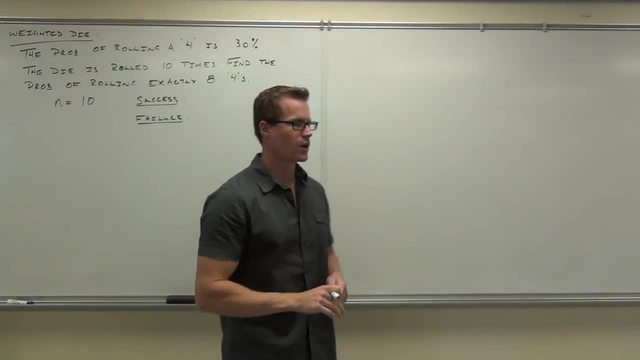 identify those on your problems on the test or on your homework. Be identifying that. I'll ask you for it. on a test, I want you to understand what a success is in this case and what a failure is in this case. So let's look at this. 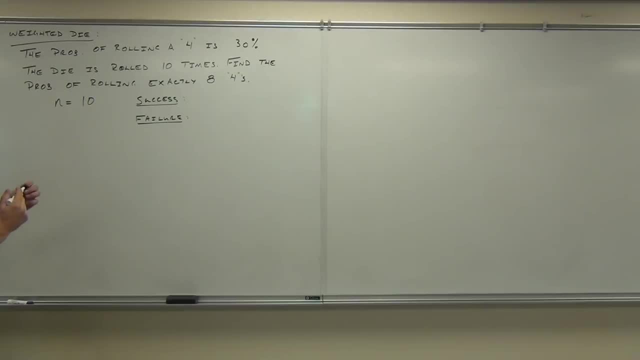 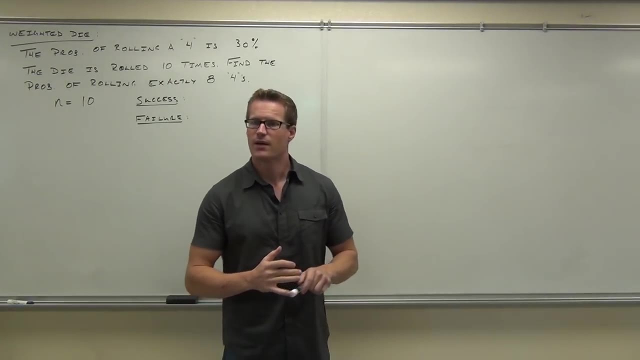 The probability of rolling a 4 is 35.. The die is rolled 10 times. Find the probability of rolling exactly 8 4s. What is a success in this Rolling 4s? OK, a lot of people get confused here. 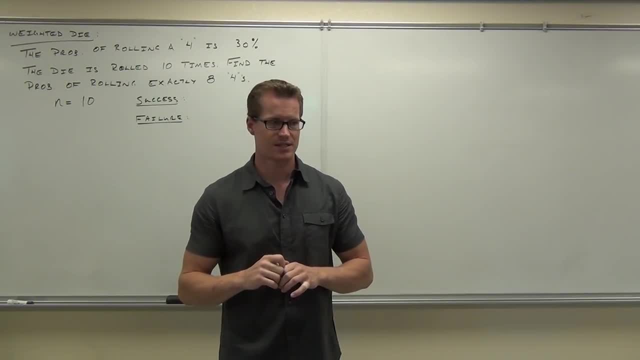 Is the success rolling 8: 4s or is a success rolling A4? A4.. A success has to be trial by trial based, Otherwise you cannot find your lowercase letter P. It's got to be for one trial. So you know you can't find the whole idea is going to be. 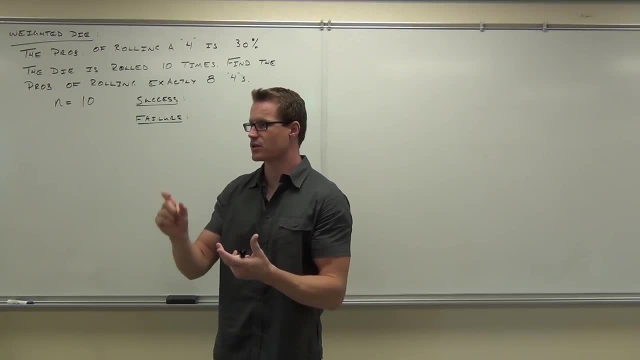 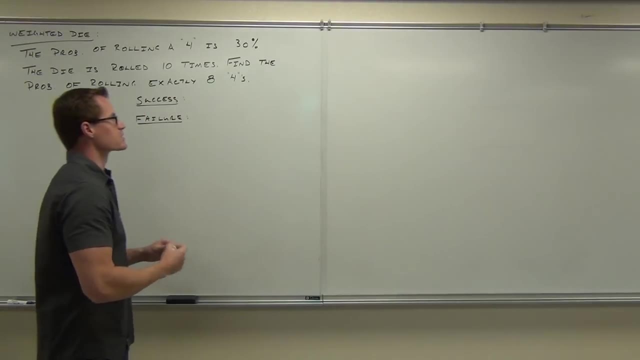 to find the probability of a certain number of success is that's based on lowercase letter P, which is an individual, by individual trial success rate or probability of success. So in our case, a success isn't rolling 8: 4s, It's rolling just one, 4.. 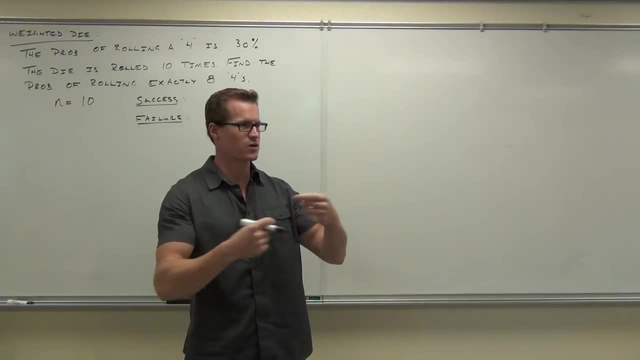 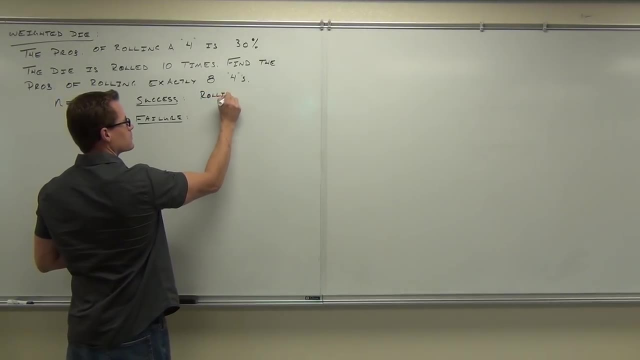 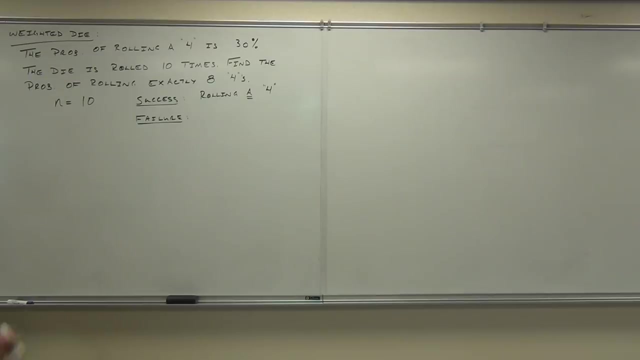 We're going to be looking for a certain number of successes. Do you see the interplay there? So in our case, a success is just rolling a 4, rolling A4, singular OK. OK, what's a failure? What would that be? 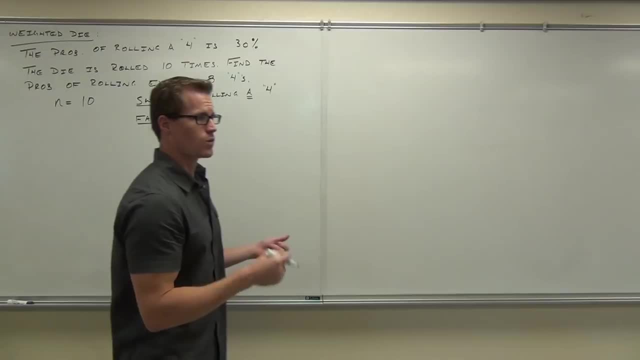 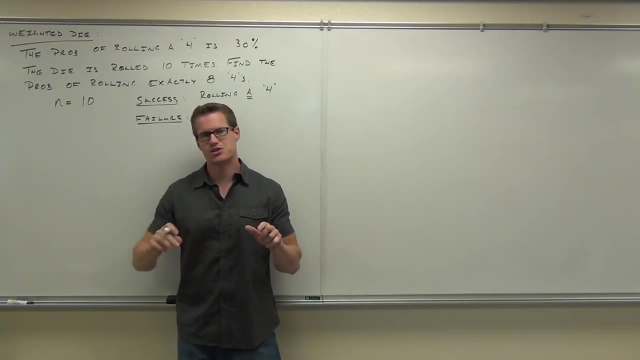 Sure, we have our six outcomes that are possible. So if you roll a 1,, 2,, 3,, 5, or 6, even though those are all different outcomes, right, There's six possible outcomes. Notice that this is still a binomial probability. 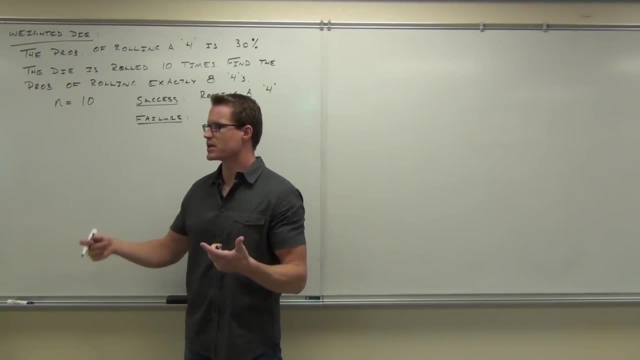 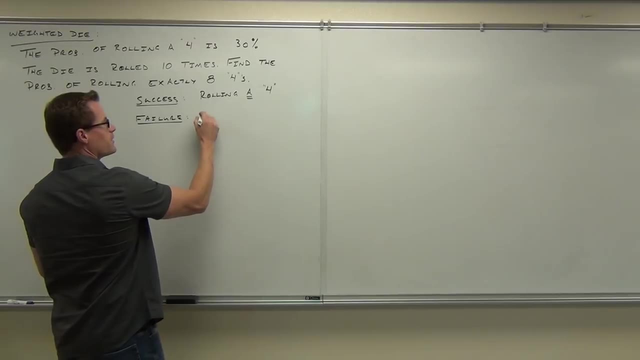 because we have only one success and the rest are failures. We say 4 is our success. That's why we have this rule in A single 4, that's a success. Everything else would be a failure. So in our case, failure is rolling. anything else? 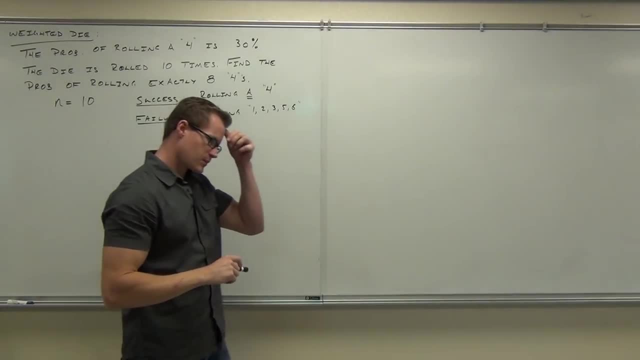 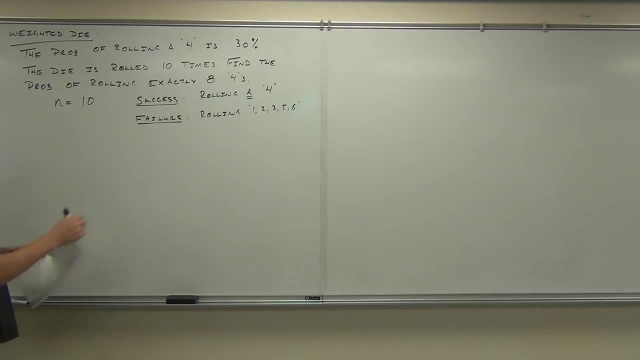 Rolling 1,, 2,, 3,, 5, and 6.. Feel OK with N, the success and the failures. OK, I want you to be identifying all that stuff on your own as well. Let's go ahead and let's look for the probability of success. 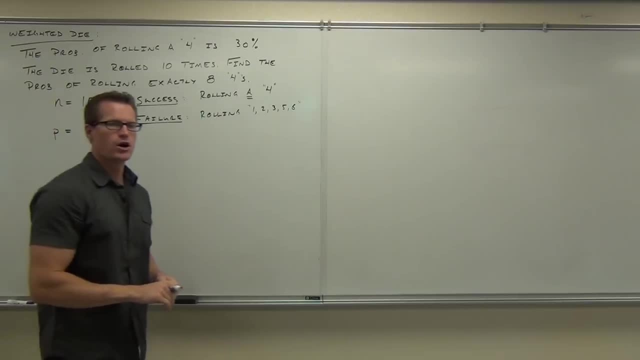 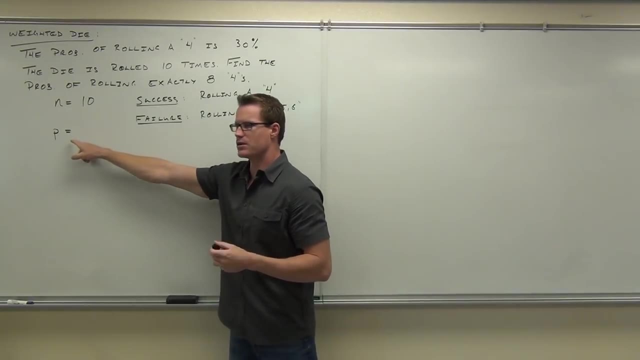 That's our lowercase letter P: the probability of success. Notice how, if I have, the success is rolling 8, 4s. I can't even find that right now. You have no idea. That's what the question is actually asking you. 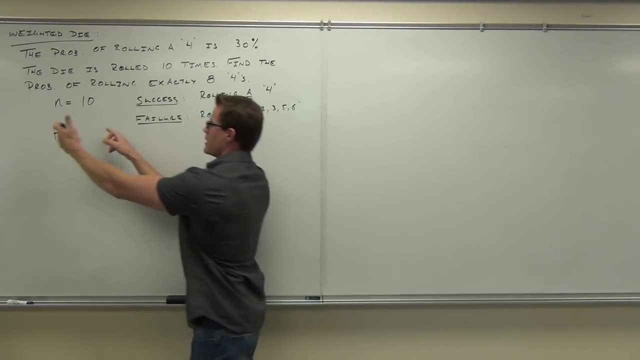 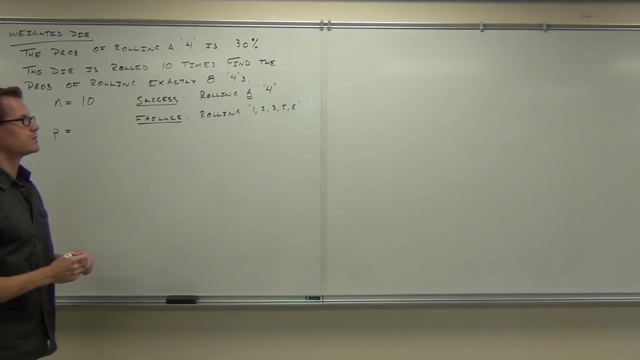 So these things have to work together. A success should be probability of A success right here. So what's the probability of A single success, A rolling a 4? 1 out of 6.. Nope, 30%, Nope. it says up there at the very beginning. 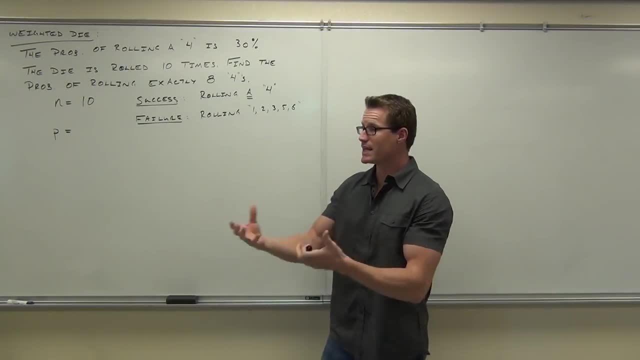 probability of rolling a 4 is 30%. Oh, so this is a way to die. So it's not just automatically 1 out of 6.. You've got to read for what. For what the probability of success actually is. 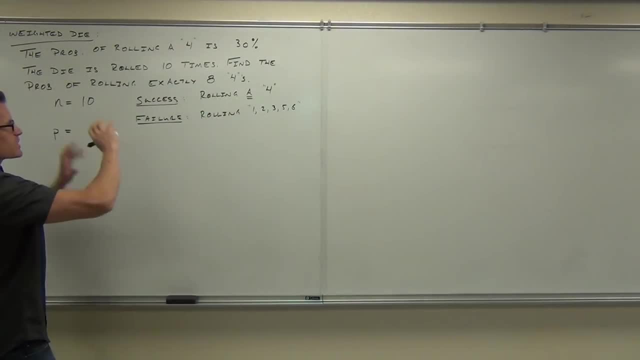 So if our success is rolling a 4, we should say up there somewhere, It should be given to you in some way, what the probability of success actually is. So, probability of rolling a 4, 30%- Am I going to put 30?? 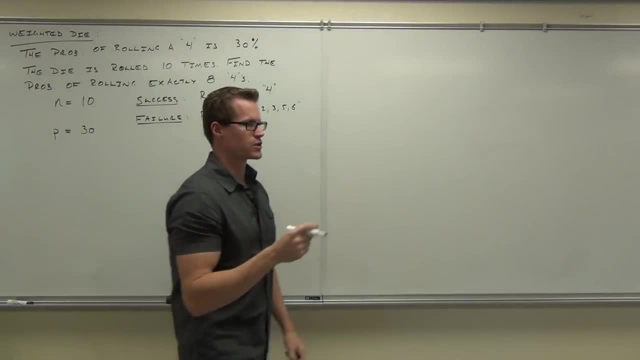 No 0. What am I going to put? 0. Good, We know probabilities are between 0 and 1.. So if I give you a percentage, we've got to translate that to a decimal. So we have that. 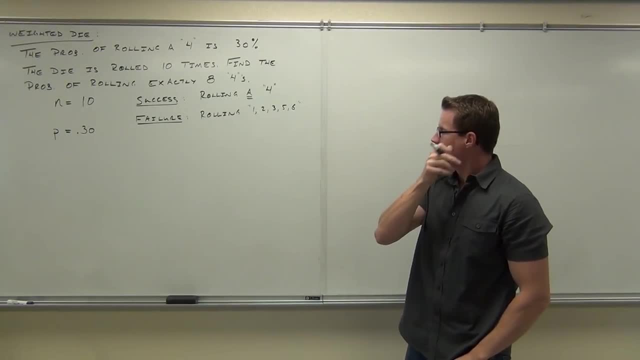 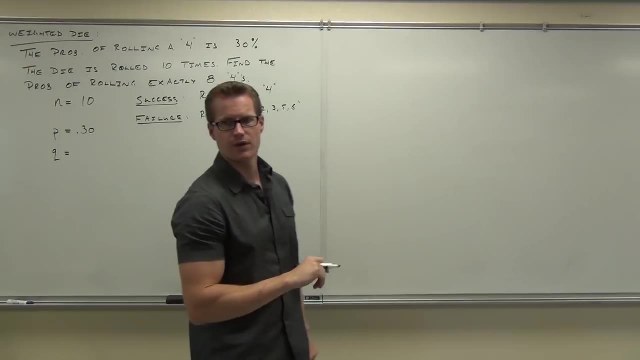 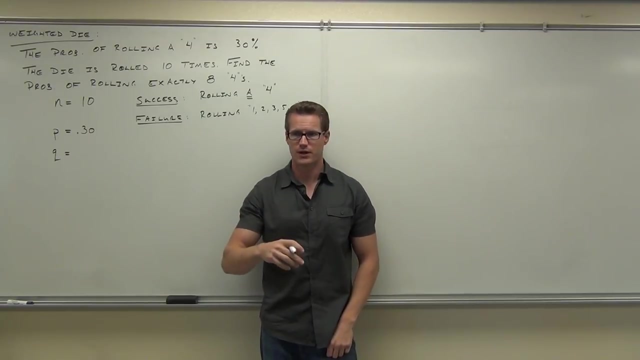 Let's show it off our cell phones, please, If P is 0.. P is 0.. Can you find Q? Can you find Q the probability of failure? Yes, These things are complementary. You're either a success or a failure. 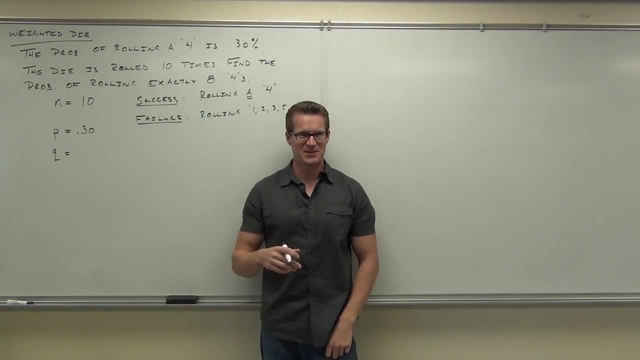 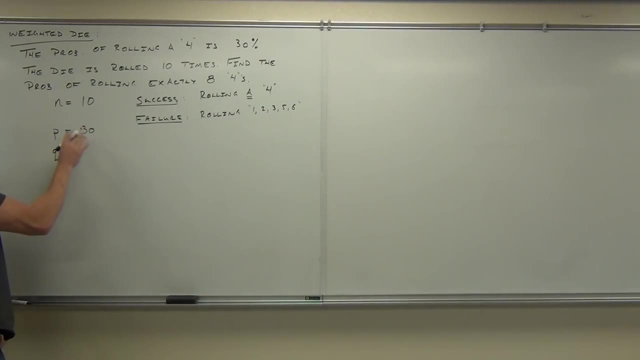 It's kind of harsh huh: You're successful or you're a failure. No middle ground. You're not just average. No, Well, if your probability of getting a success is 30% or 0.30,, the probability of failure is everything else. 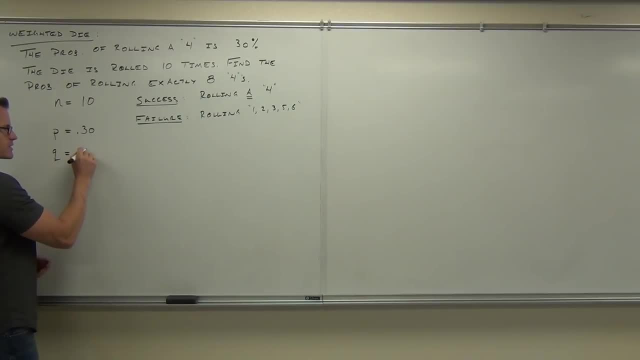 So what is that 70%? Yeah, The way we're figuring out the 0.70, we're taking 1 minus P. That's what that is. 1 minus the probability of success gives you the probability of failure. Those things have to add to 1.. 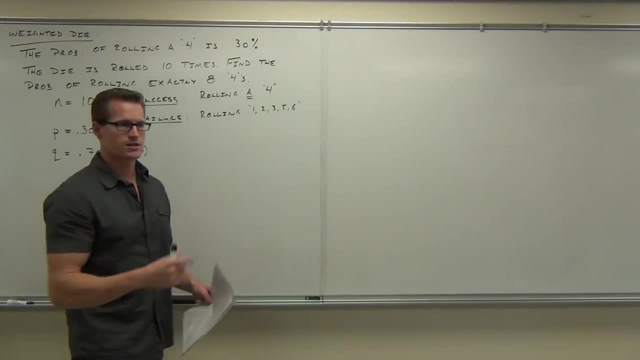 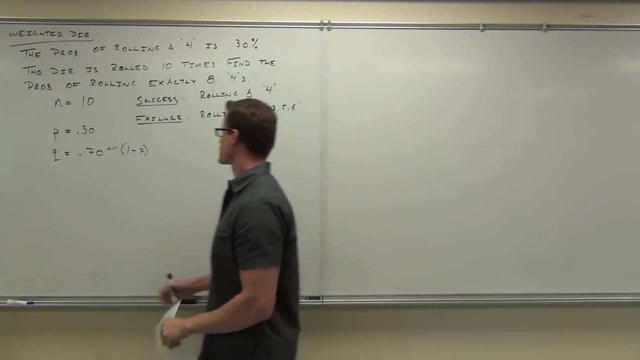 Therefore, the number 1 minus either the probability of success or the probability of failure will give you the alternate, the complement of that. What else we missed? Oh yeah, X, X, Yeah. What does X stand for? again, The number of successes we're looking for. 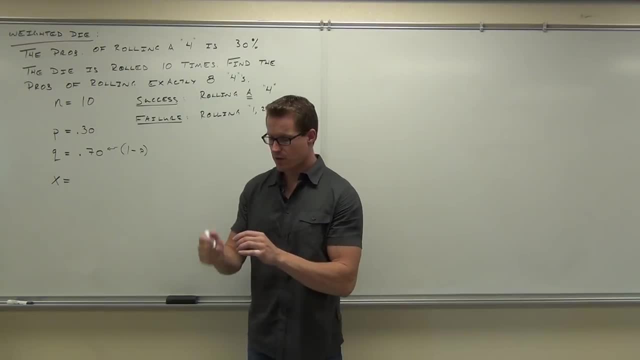 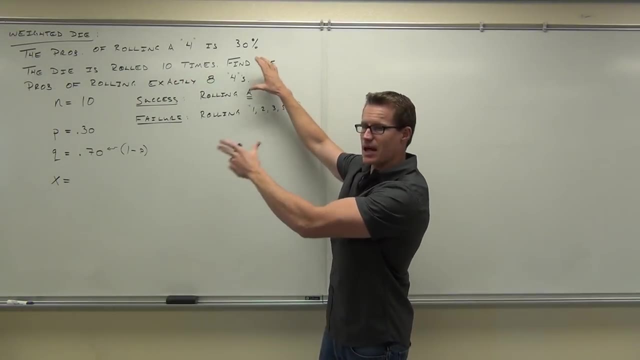 Cool Number of successes we're looking for. So notice how a success would be a single thing, The number of successes, how many of these things, how many successes I'm looking for in my whole entire procedure. So how many successes am I looking for? 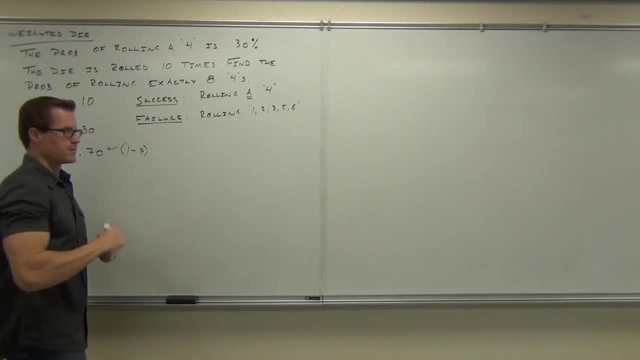 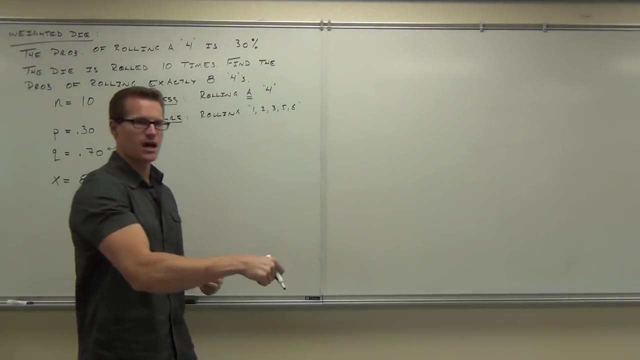 Basically, if a success is rolling forward, how many 4's am I looking for? 8. 8. Very good, Yeah, We're looking for 8.. We're looking for 8 times that we're successful. We're looking for exactly 8 times we've rolled that 4 in this case. 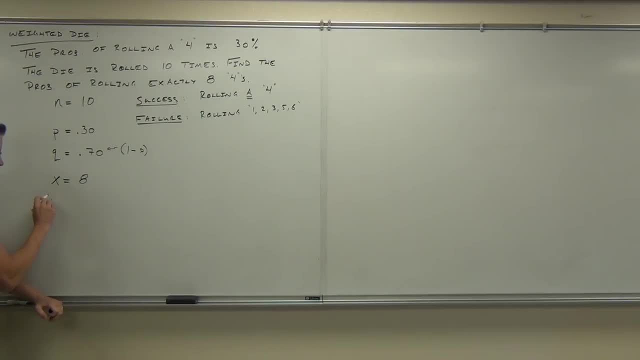 Last up now comes the question: how do we find the probability of exactly 8 successes? The probability of 8 successes? I want you to notice how the 4 is not here. We're not finding the probability of a 4.. 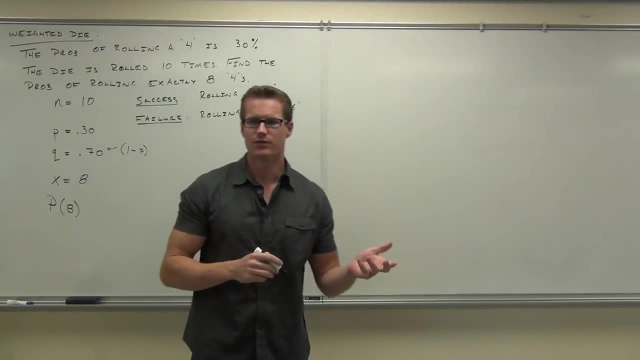 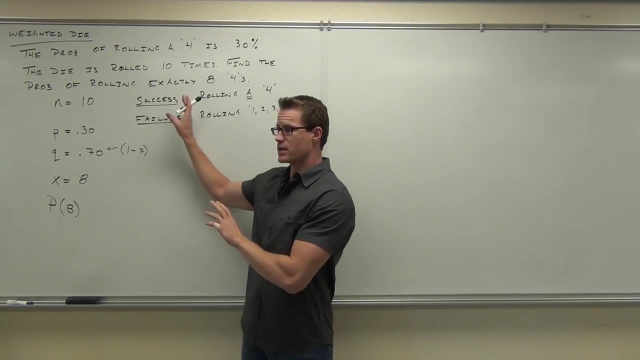 4, honestly, is kind of weird, but 4 is going to be irrelevant. What this comes down to is the number of successes you're looking for out of a certain number of trials. The fact that we're rolling 4's, that's all great. 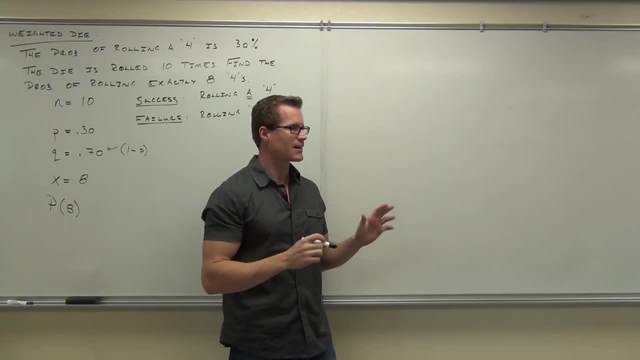 But we're actually just looking for the number of successes. We'd get exactly the same thing if we had like a weighted die And I said the probability of getting a head is 30%, The probability of getting a tail is 70%. We're looking to flip the coin 10 times and get 8 heads. 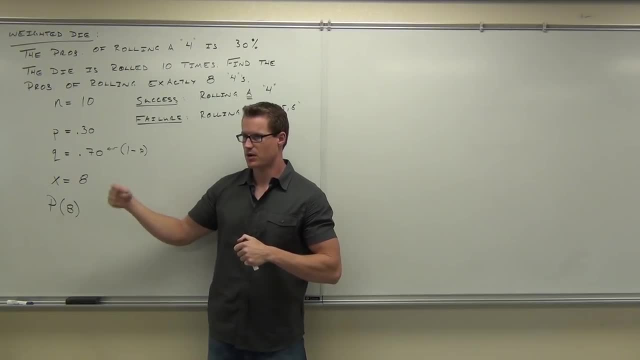 That's exactly the same problem. Exactly the same problem. So this is all based on the number of successes compared to the number of trials and considering the probability of success and failure for each trial. You're going to see what I mean in just a little bit okay. 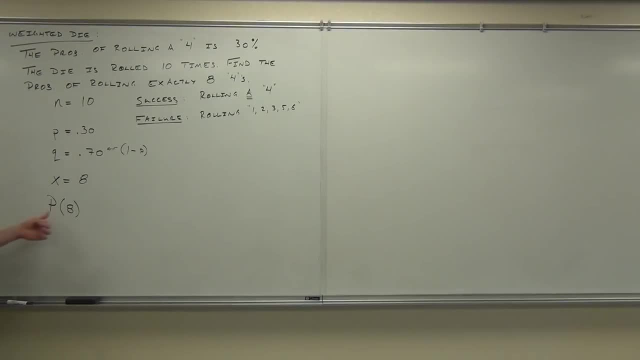 Just a little bit. So we're looking for the probability of exactly 8 successes. Oh my gosh, how in the world do we do that? Well, there's a formula. There's a formula for how to find probabilities. It's a binomial situation which we have here. 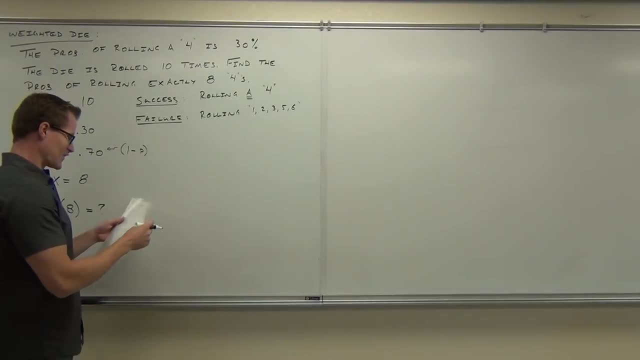 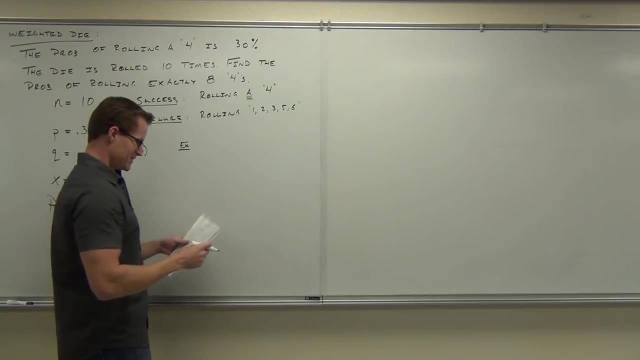 You ready for the formula? Yeah, Of course you are. I told you I'm on today. I told you about my math injury. So our formula. Here's the formula for the binomial probability formula, If you want to find the probability of a certain number of successes. 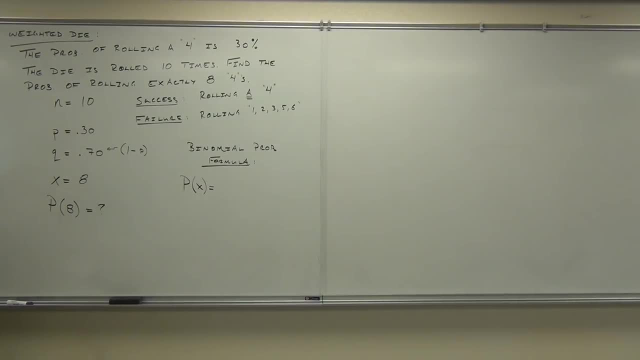 The probability of a certain number of successes. Here's how the formula looks. I'm going to give you the formula. Then I'm going to tell you why it works the way it does. Does that look familiar? I hope that looks familiar to you. 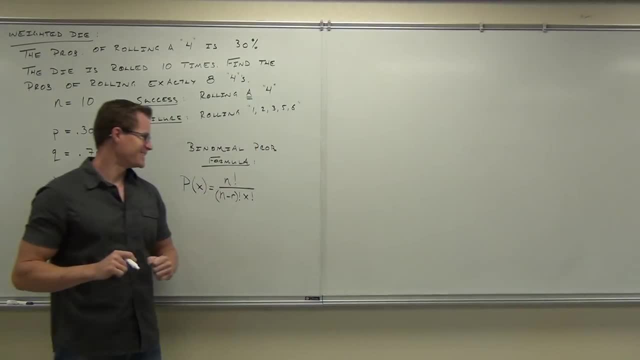 My back looks familiar. Does this look familiar to you? That should look familiar to you. You just did that in section 4.7.. What is this formula right now? Oh good, You all remember the formula. This is awesome. 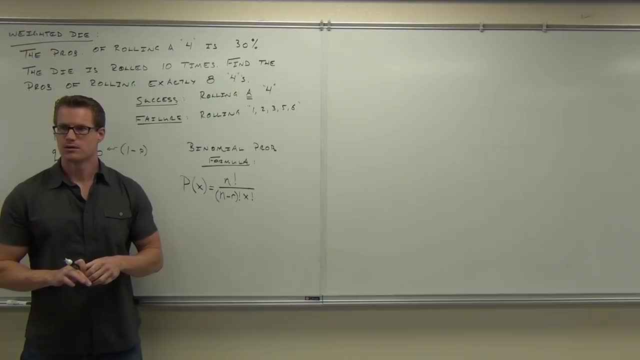 It's either a permutation or a combination. It's one or the other. It's really similar to the combination one. It is the combination one. Oh you know what? In fact, let me make that an X. And then it is the combination one. 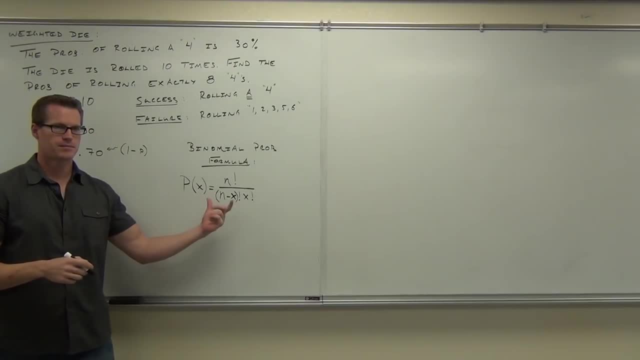 I think I accidentally put it in R. It should be an X. Oh yeah, Now it makes a whole lot more sense. Now, that did look familiar to you, didn't it? Not at all. I've never seen that before. 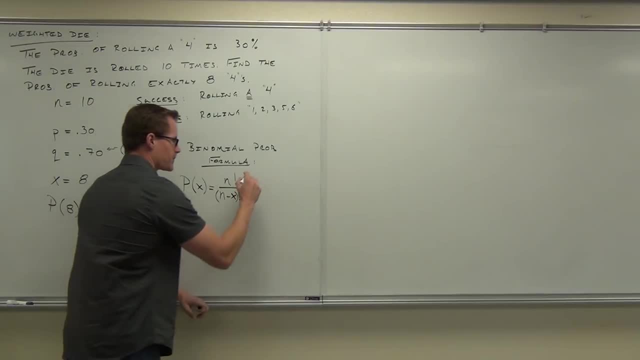 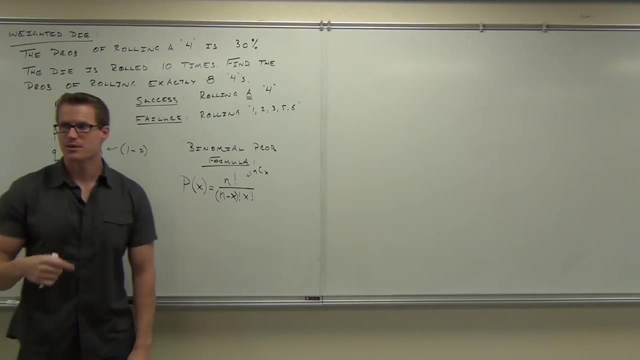 Yeah, So this is the combination formula. This would be NCX. That's what this is. That's what this section is. It's a number of combinations of ways that we can accomplish eight successes, or however many successes, out of ten trials. 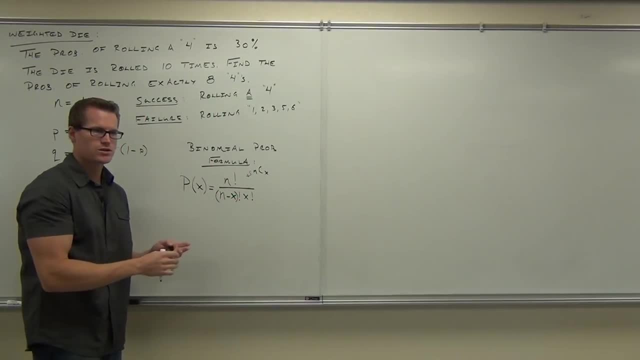 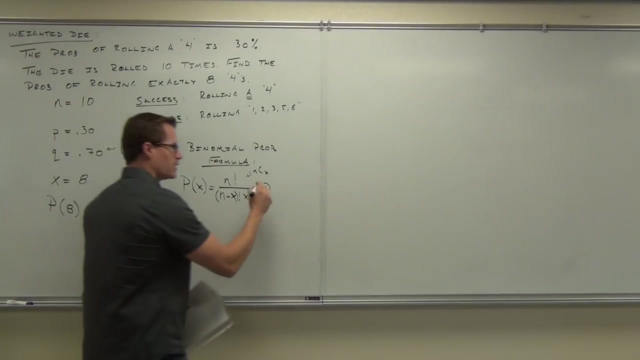 That many combinations is what we're looking for, So we're taking each of those combinations. We're not done with the formula, though. What we do now is multiply all those successes times the probability of success For each one. That means to the X power. 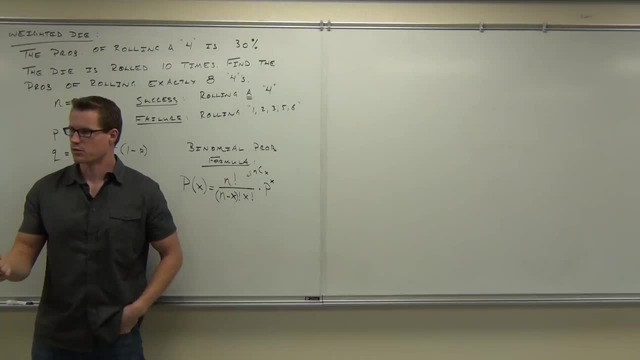 So X, right here, is the number of successes we're looking for. We identify this as the probability of X, That's the number of successes. This is: every time we have a success, we have to multiply that probability. That's what the P of X comes from. 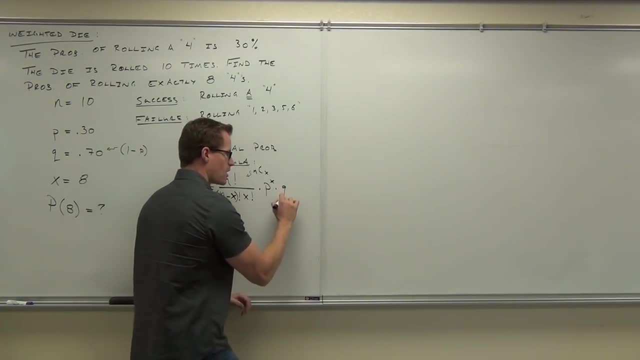 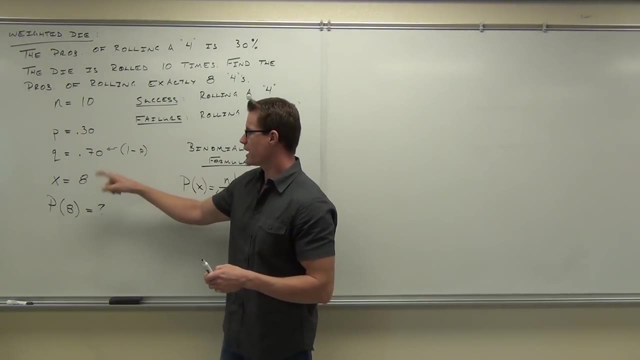 Now we also have to multiply every failure times the probability of failure, because we're looking for an exact number here. So this is kind of interesting to think about. In our situation, we actually want eight successes and we actually want how many failures. 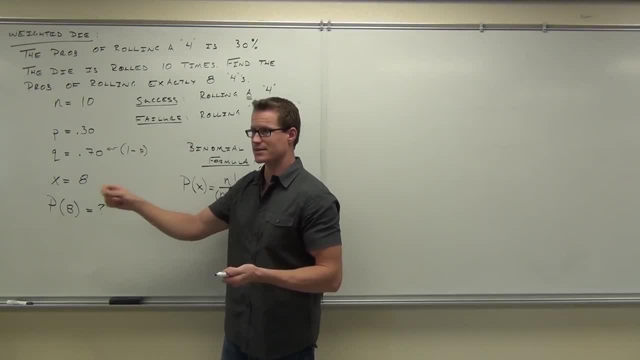 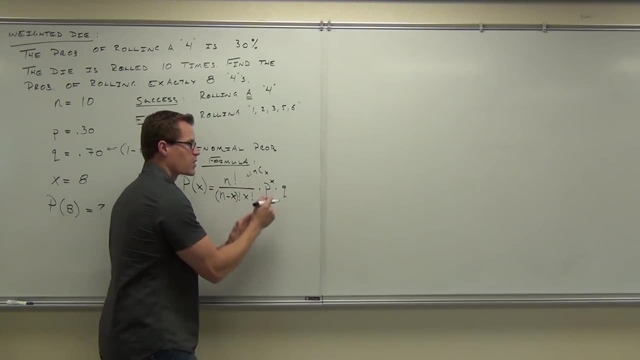 We want two failures. We want two failures in order to get those eight successes. Are you with me on that? So in our case, we have to multiply not only by the probability of success a certain number of times, we also want the probability of failure a certain number of times. 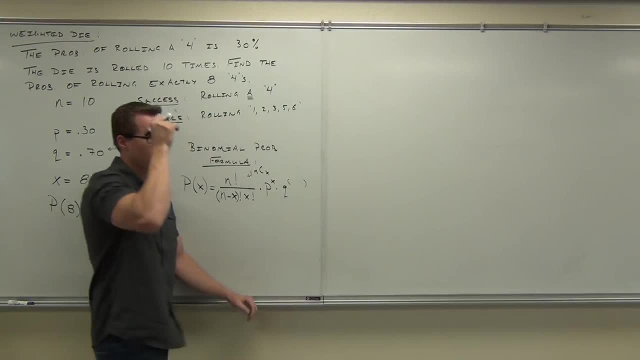 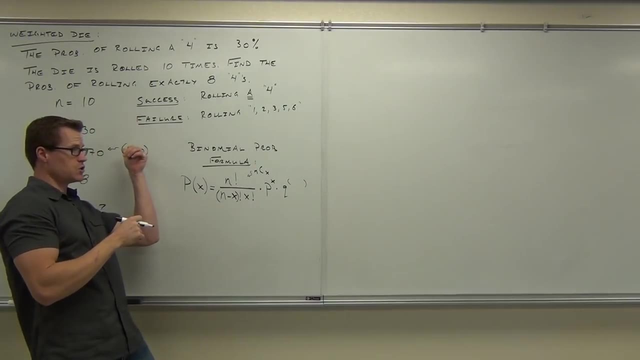 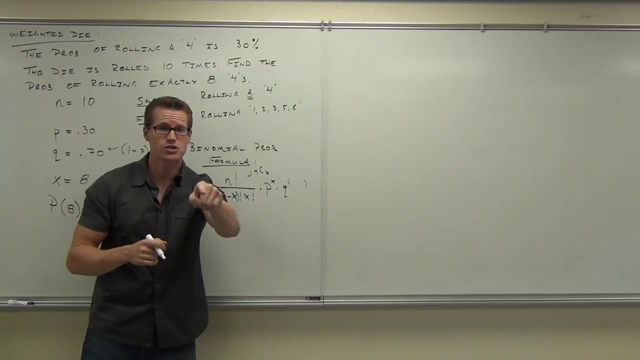 What does this have to be? do you think, If we have X successes, we want? how many failures? In this case, two failures, sure, But how about in variable form? Say that again: N minus 2 for this situation, sure. 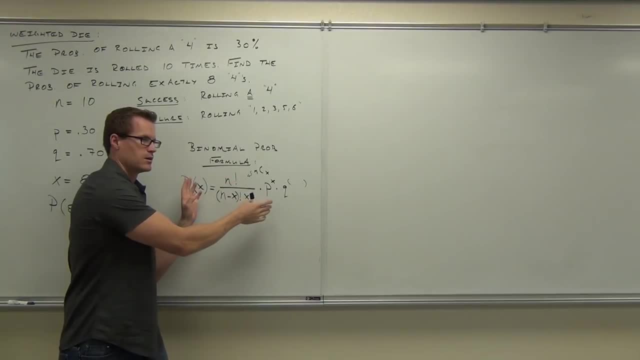 That would be 10 minus 2.. I don't have a 2 here. I have a. I'm sorry, not N minus 2.. We have N minus 8. actually, That would give you the number of failures: N minus what. 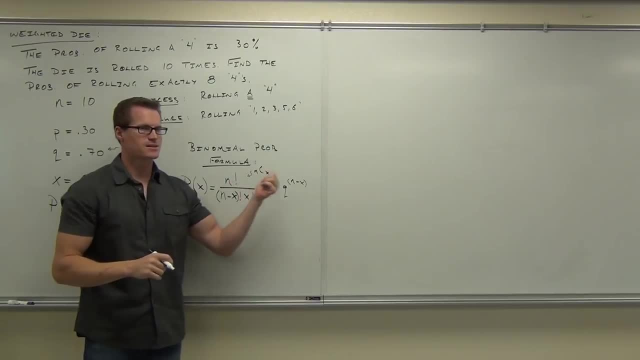 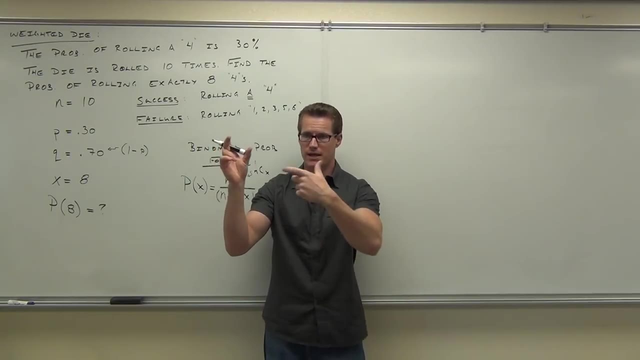 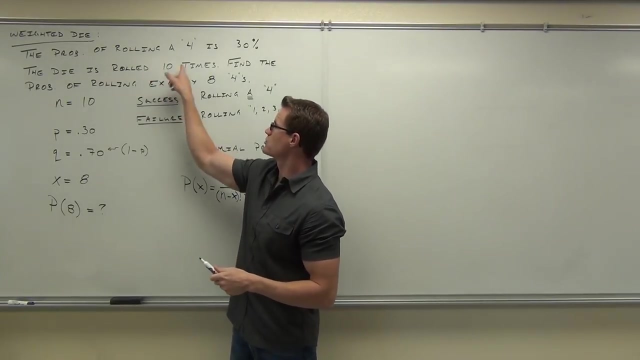 X. that's right. If you have X successes and you have N total trials, how many failures do you have? Well, you have the total number of trials minus the number of successes. That gives you your failures. If you have 8 successes out of 10 trials, 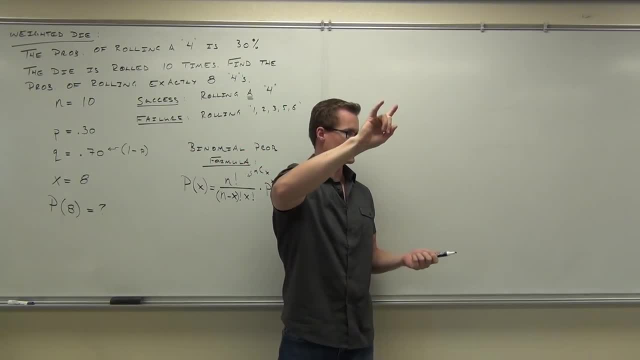 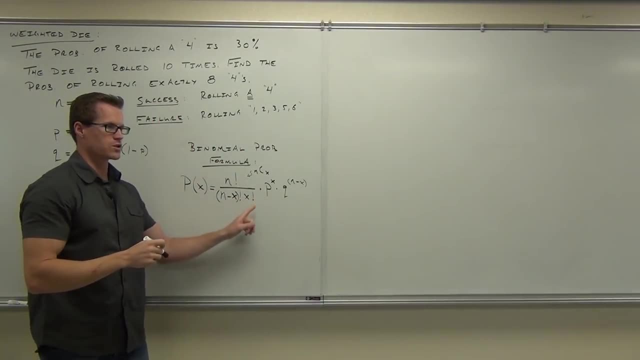 we want 2, or 10 minus 8, failures. Are you with me on this, folks? Yes or no? Yes, So this is the number of combinations that we can accomplish: X successes. This is the combinations of that happening. 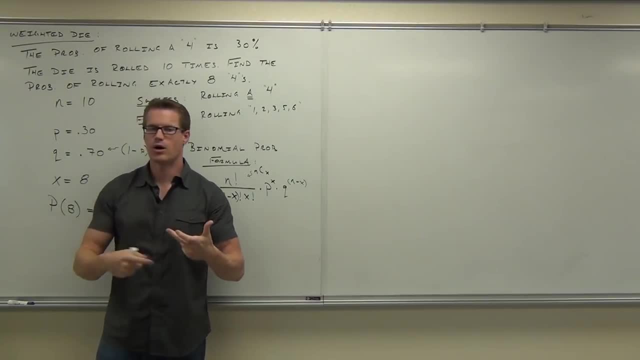 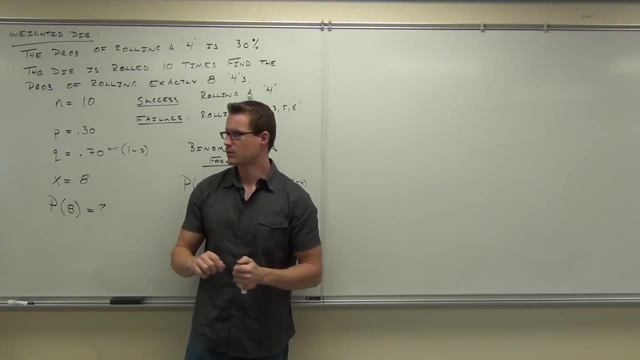 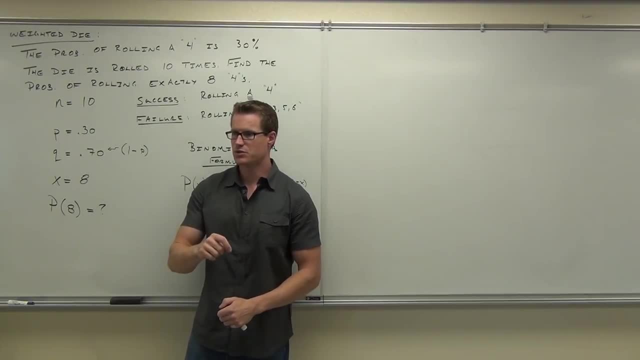 and then whatever else, the next 2.. We could roll a 4 and then a 2, and then a 4,, a 4, a 4, and then a 7.. Oh no, not a 7.. 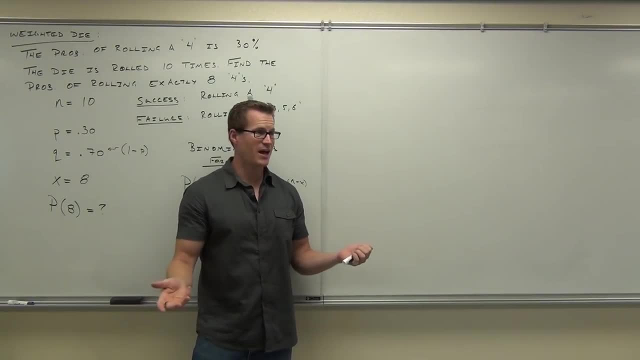 We can't roll a 7,, can we A 6, and then a couple more 4s? We could do that. Or we could roll a 4 and then a 3, and then some other ones, Or a 4 and then a 5,. 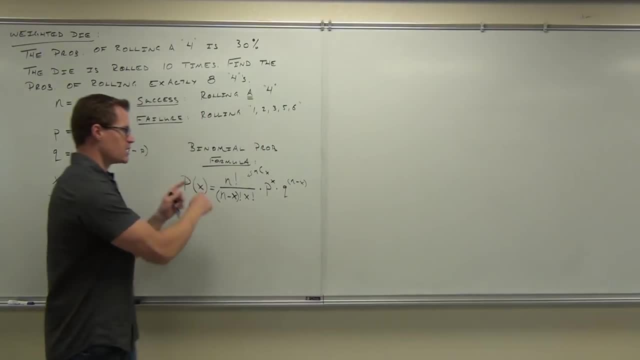 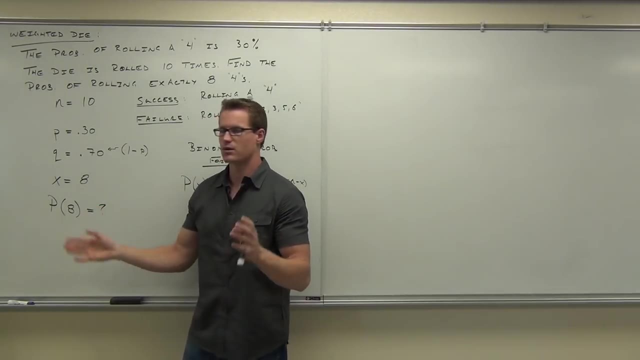 and then some other ones. We could do all those situations, all those playing to the number of ways we can get 8 4s and 2 something else's. Yes, 2 something else. whatever they are, We don't care. 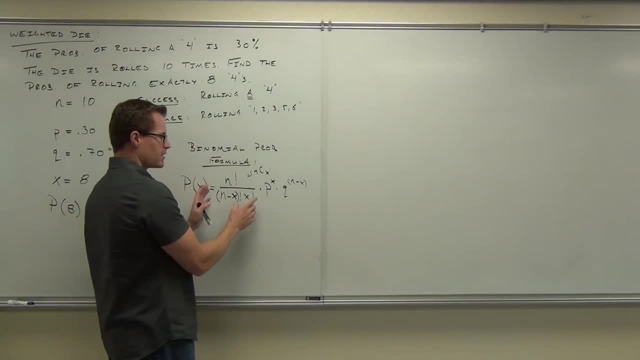 They're all in the same category of failure. We take each of those successes, we multiply that times the probability of P, the probability of those successes. That's where this P to the X is coming from. This is over and over again. 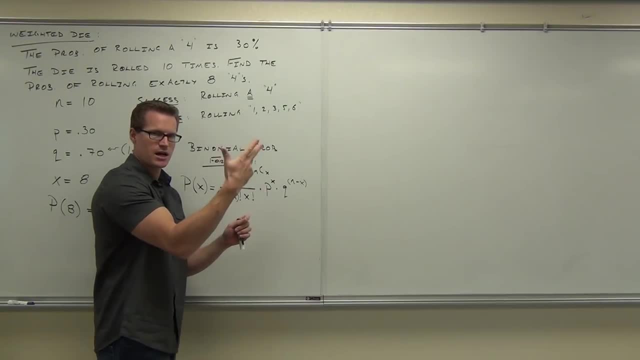 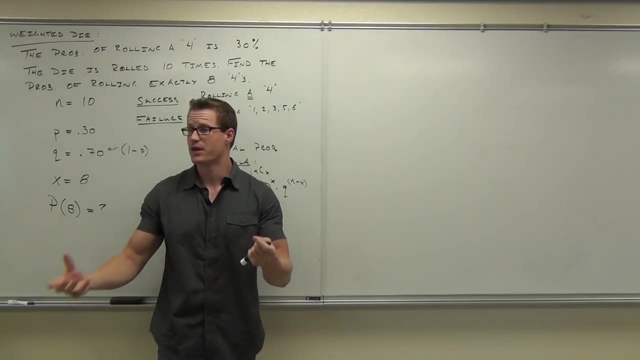 If we had 8 successes, we'd be doing probability of success 8 times. That's where we're getting that X going Probability of failure we're taking. well, the total number of trials minus that many successes gives us the number of failures. 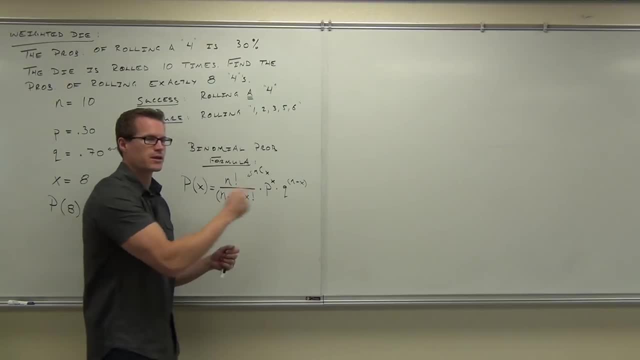 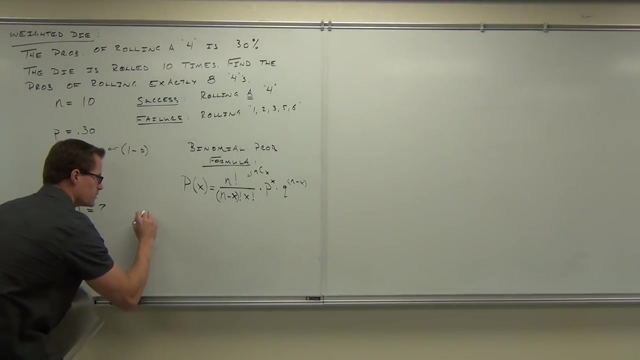 We want two failures. We multiply this twice times itself Probability of failure twice. That's where this formula is coming from. Now let's see if we can use this formula to find this probability. So we want the probability. Oh, by the way, 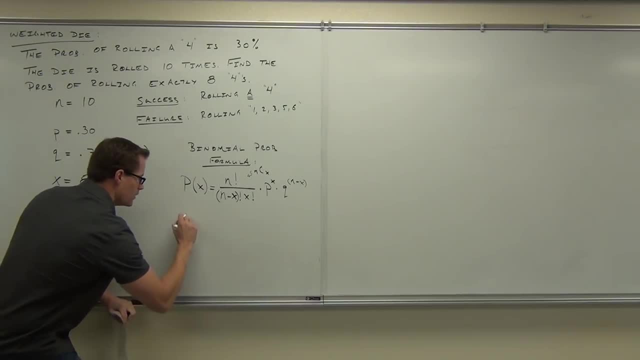 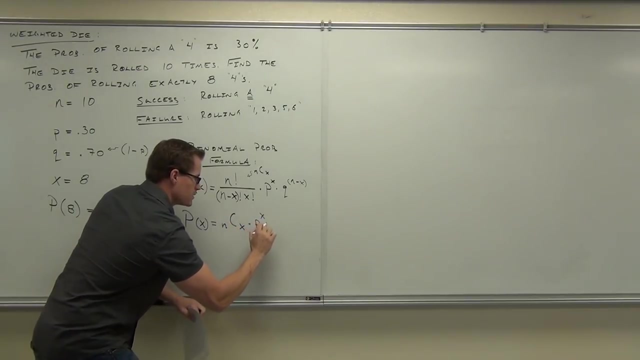 if you want to make this a little more concise, I'll let you. Why don't? because your calculator will actually do that, won't it? Let's just call it that. Let's do N C X times P of X times Q N minus X. 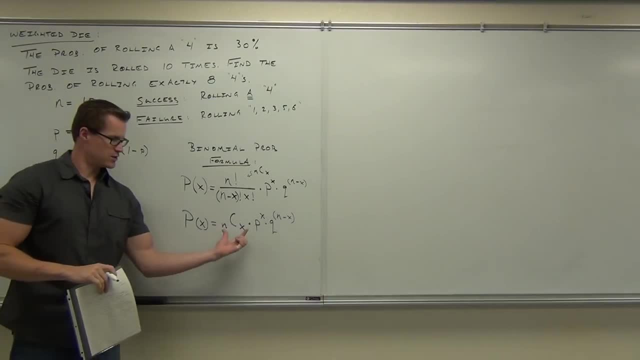 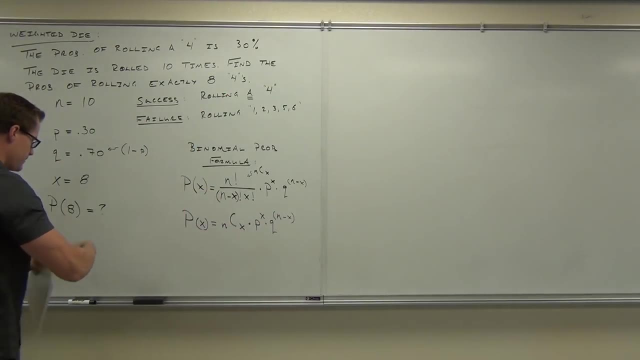 That's a little bit easier to accomplish on your calculator. We know how to do this. That's just an exponent. That's just an exponent. I'm going to do that over there so we can see it a little bit better Right now. 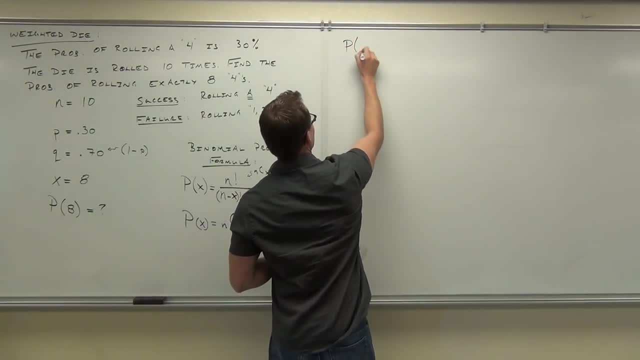 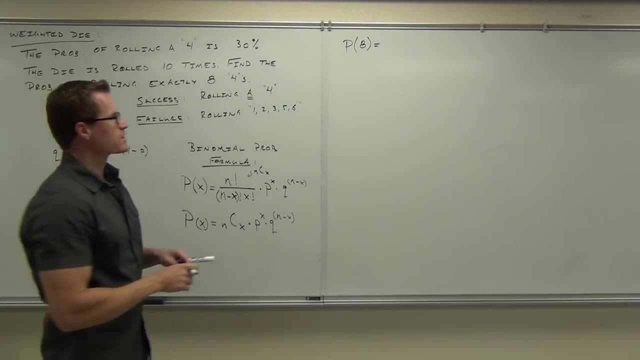 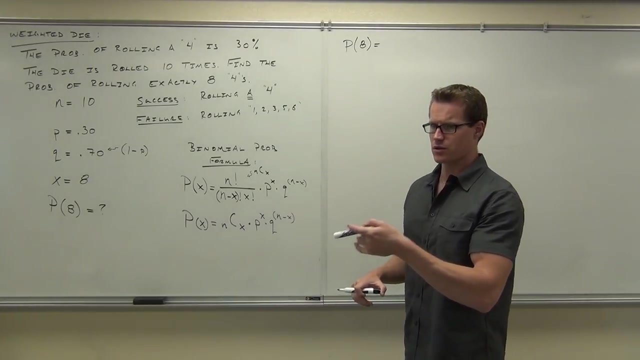 we're going to look for the probability of 8 successes. The probability of 8 successes. What this says to do is: first off, we're going to have N, C, X. What was our N in this case? You're also okay on that right. 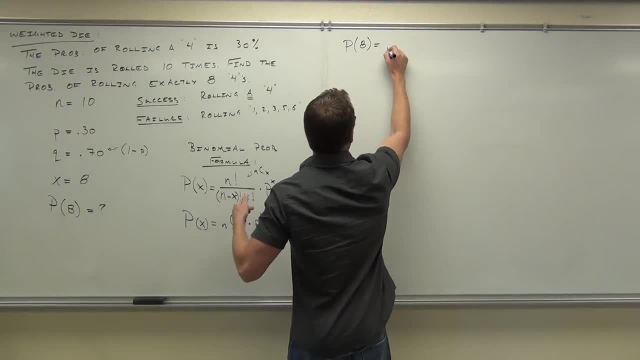 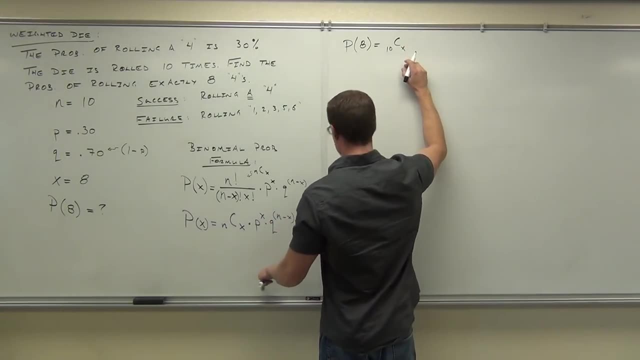 That we have 10?. Okay, Let's do this. We got 10 C. what was the X? 8. 8 successes? P of X is N, C, X. In our case, we have 10 trials, We're looking for 8,. 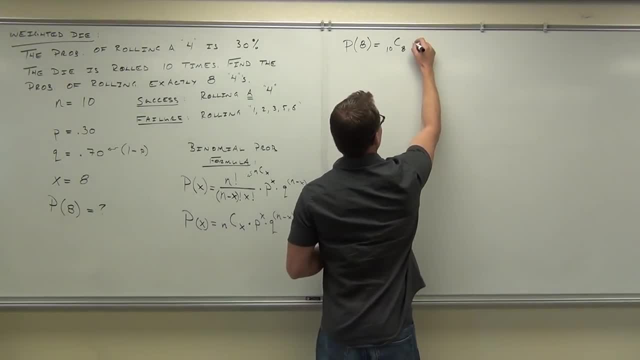 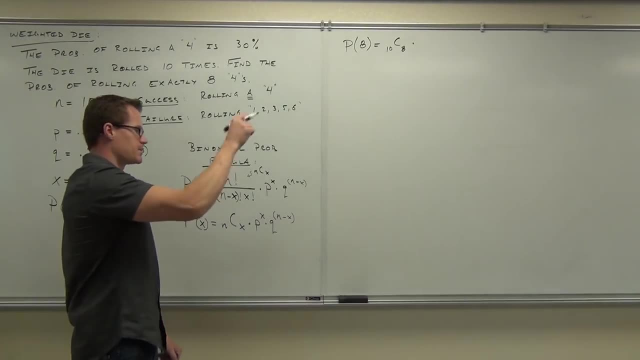 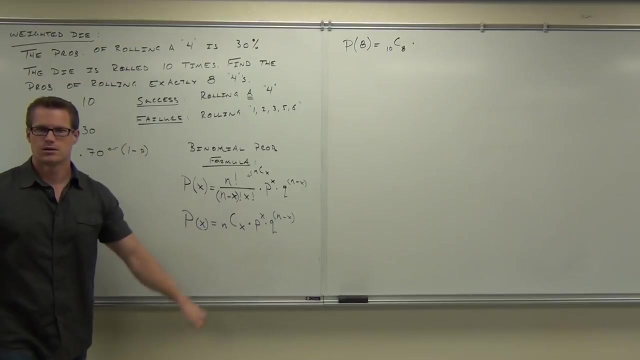 exactly 8 successes Times. We're going to take the probability of each of those successes to the power, which happens to also be the number of successes. So what's our lower case letter P? What would go right here? I'm going to put that in parentheses. 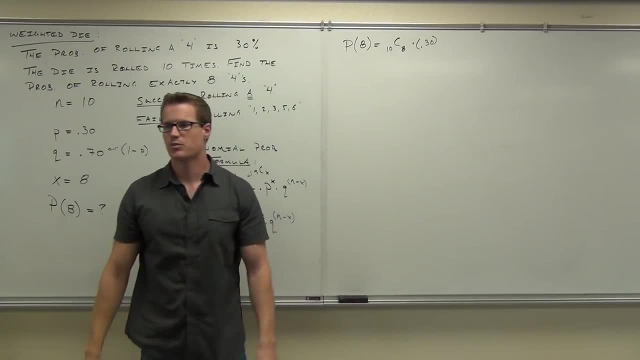 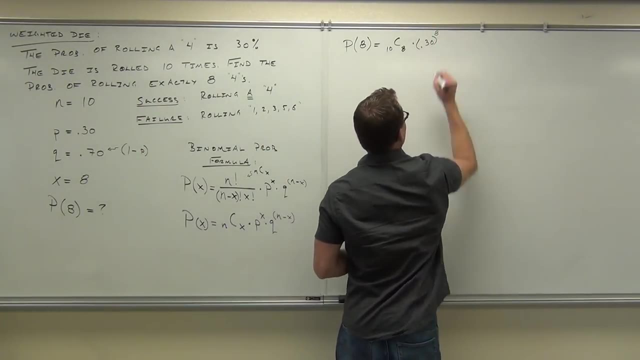 but it's a little bit more nice that way. so you know, that's a decimal in there: .30.. What power is that going to be raised to, ladies and gentlemen? Eight, Eight, Sure, Sure, Why? to the eighth power again. 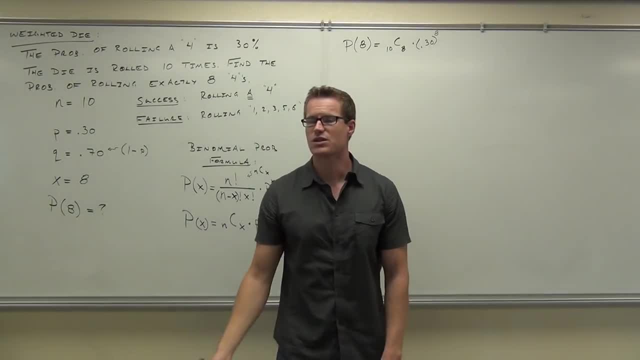 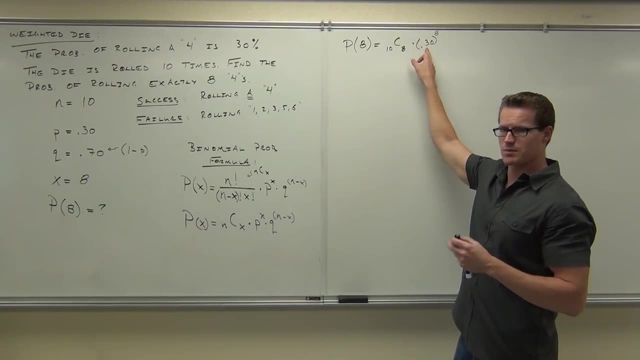 Complete the eighth power. That's our number of successes. I want you to think about what we're doing. Think about what you're doing. This is the probability of each success. Okay, We're multiplying the probability of each success times itself, for however many successes we want. 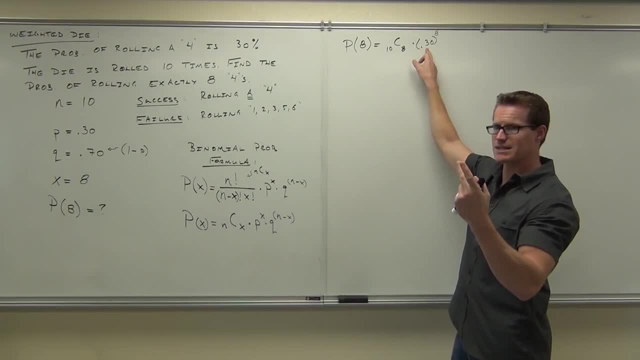 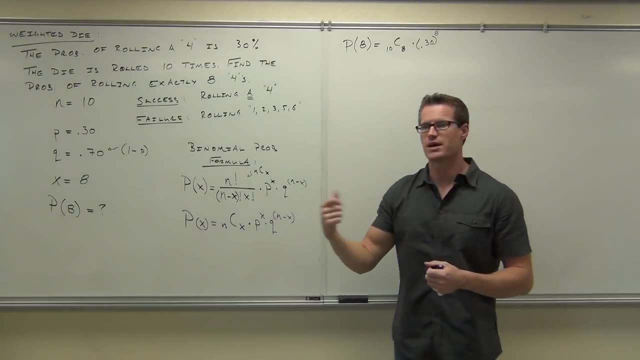 So .3 times .3 times .3, eight times. That's where that eight's coming from. We want eight successes. Multiply the probability of success times itself eight times. That's .30 to the eighth power in the case Next up. 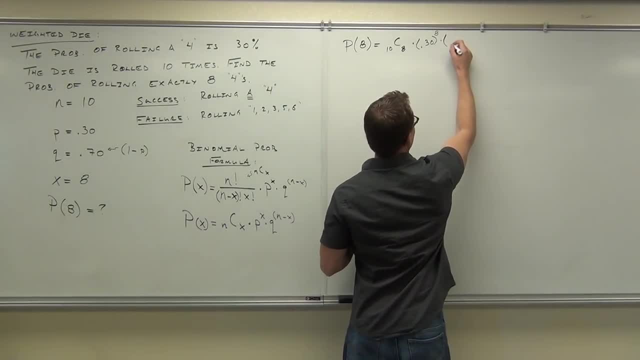 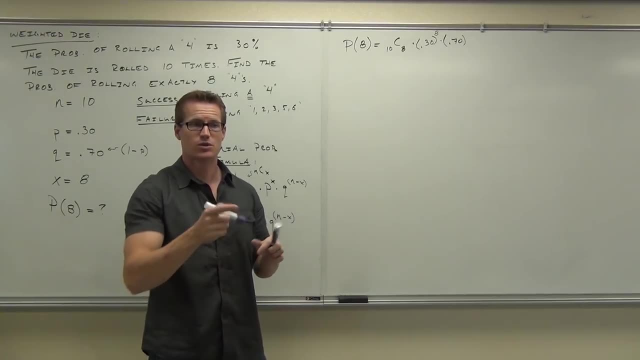 we take the probability of failing. What's that probability? .78.. Now we're going to take that to what power? in this case, Ten minus eight, Yeah, ten minus eight, which is going to give us that two. So n was ten. 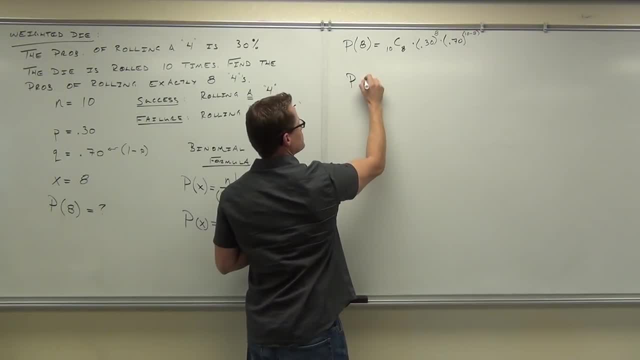 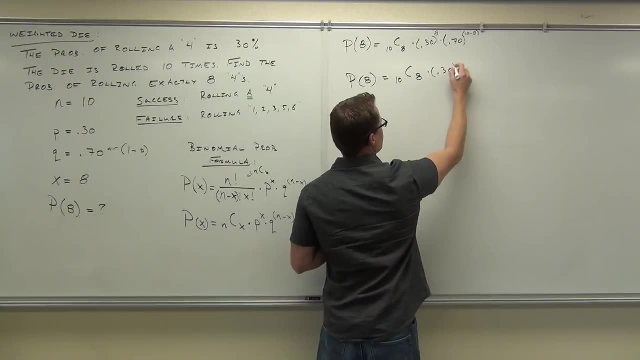 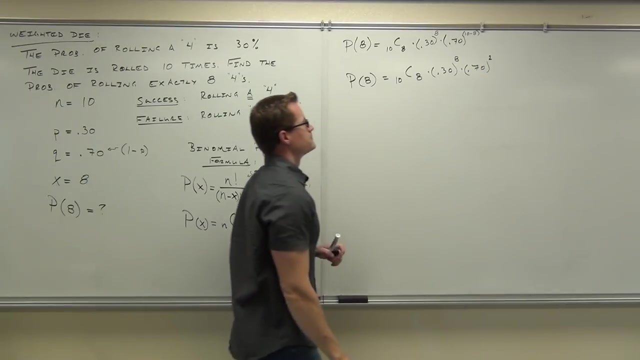 x was eight, So our probability is ten c. eight times .30 to the eighth power, times .70 to the second power. That will give us the probability of getting exactly exactly eight successes. Again, the reason why this formula works. this is every possible way. 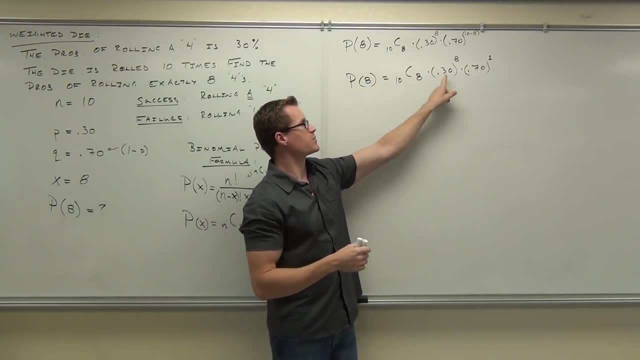 you could get eight successes out of ten rules. That's what that says. This is the probability of success. We want eight of them. This is the probability of failure. We want two of them. You multiply all those probabilities together: multiplication rule. 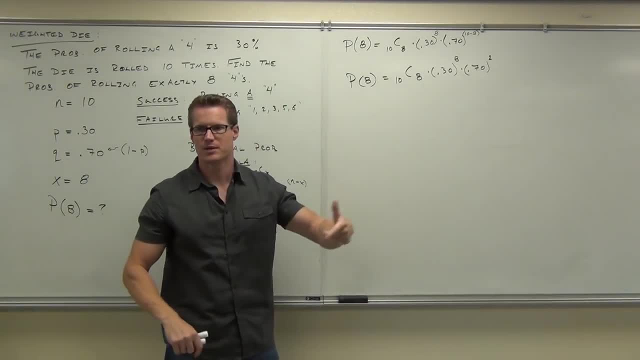 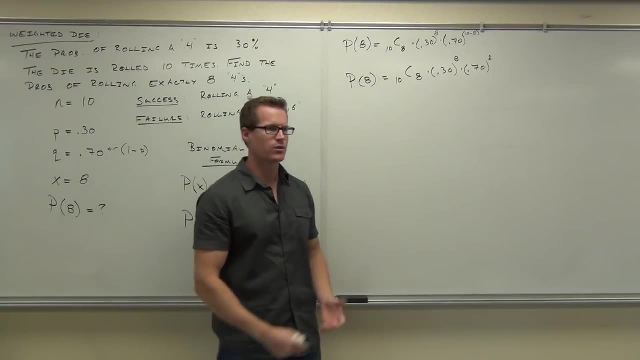 and you have this formula. So, based kind of on the multiplication rule, how this is derived, Let's do it. Find ten, c, eight for me. You should know how to do that on your calculator. We've done that a couple times. 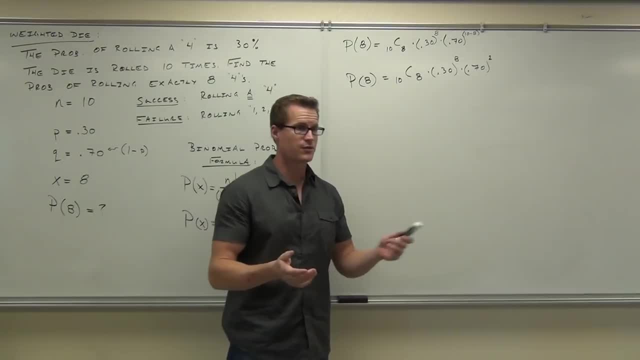 right before. What is it? Only 45. So there's 45 ways rolling a die, that I could roll it ten times and get exactly eight successes. So 45. Only five. Oh, by the way, I was going to mention this. 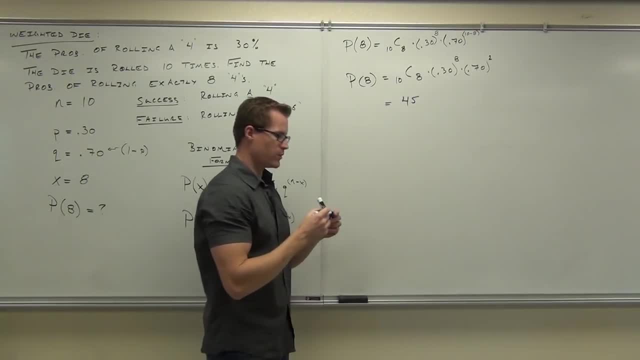 Look at the board here real quick. The number four was the number we were actually trying to roll, wasn't it? Did you use the number four at all? No, That's. what I'm trying to tell you is that this is not based. 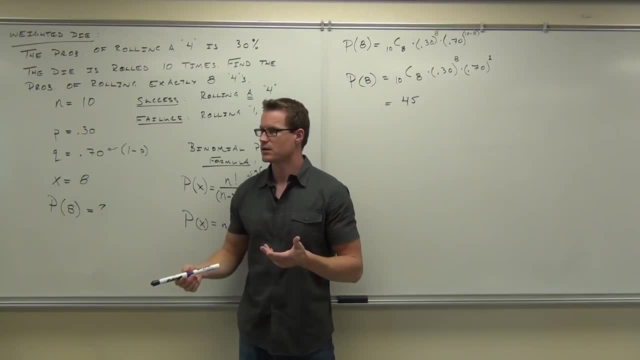 on the specific value that you're trying to get. What it's based on is the number of successes you're looking at, considering your probabilities. Do you see that I'm trying to get the number four? I'm trying to get the number four. 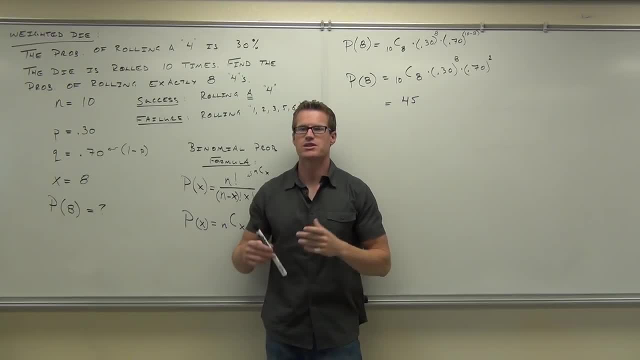 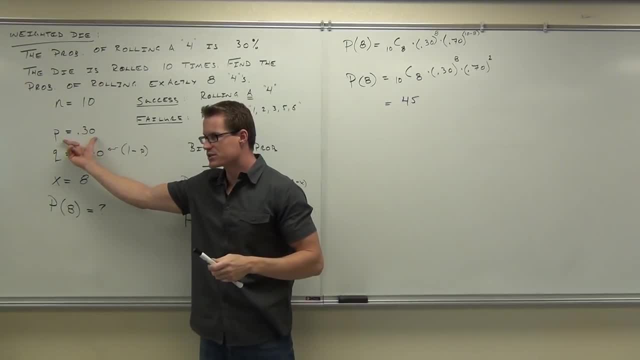 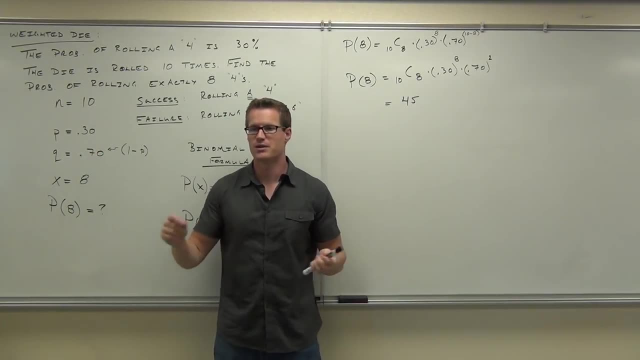 It's just about the number of successes compared to the probability of each success, the probability of each failure, the number of trials you have and the number of successes you're looking for. It doesn't even have to do with the four, It's all about. 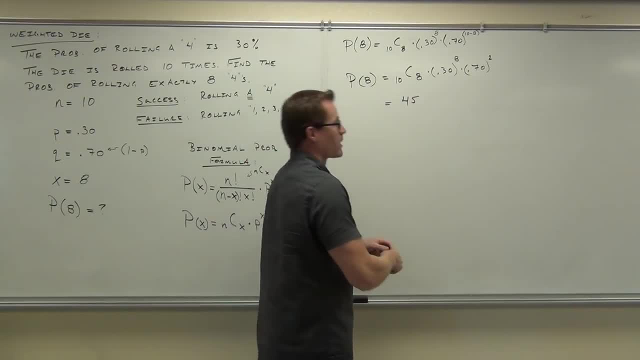 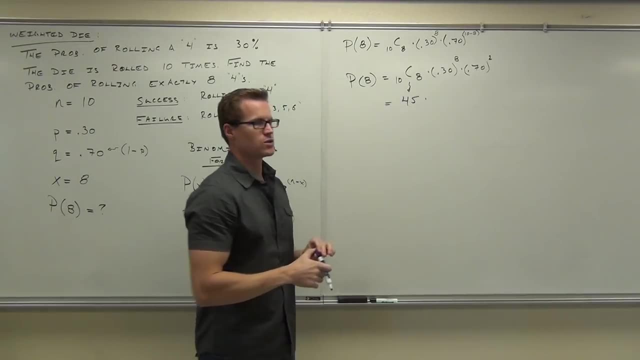 the number of successes. Yes, no, That's what I was trying to say earlier, or what I was saying earlier. So 45, that's this little part times. let's do .30 to the eighth power, .30 to the eighth power. 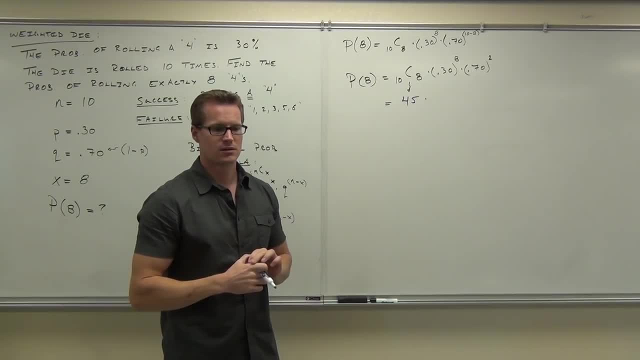 Six point five six. Six point five, six. One times 10 to the negative five. Okay times 10 to the negative five. Right, because when you multiply decimal times decimal you actually get a smaller decimal. So you put six point five six. 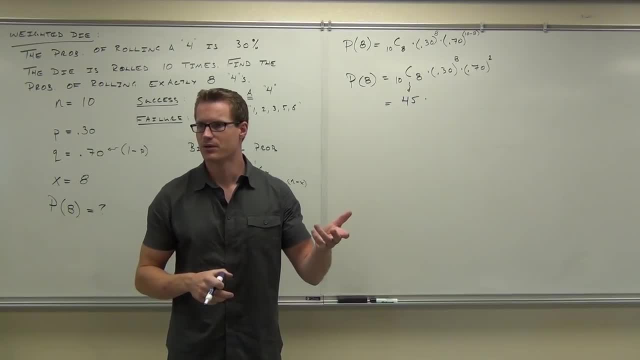 you're way off. Okay, you're way, way off. You're going to get a number bigger than one. you're going to have a probability of like- oh, I don't know- 250 or something. Now your probability. 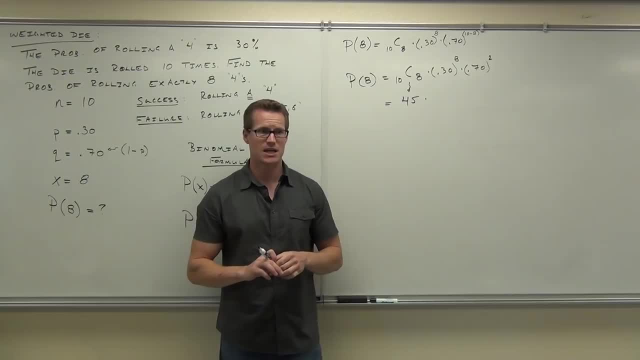 between 0 and 1,. so when you're reading your calculator and you get times 10 to the negative fifth, you have to know what to do with that. So tell me exactly what you got: 6.56, is that what it says in your calculator? 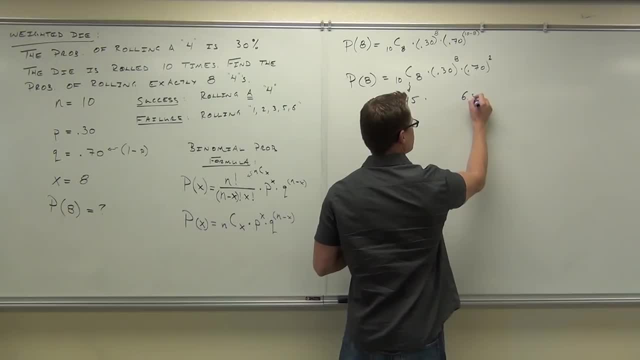 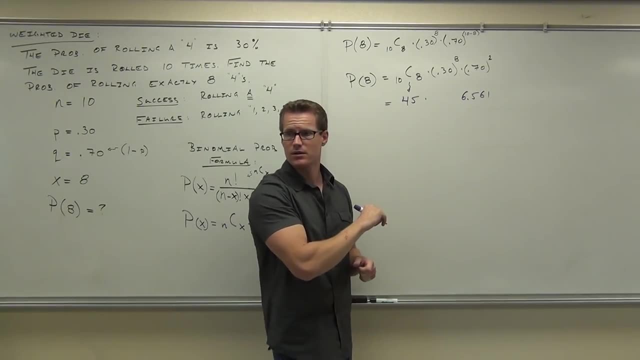 6.561.. Okay, 6.561.. Times 10 to the negative. Times 10 to the negative. Do you know what that means? Yes, That means you are one, two, three, four, five. decimal places this way. 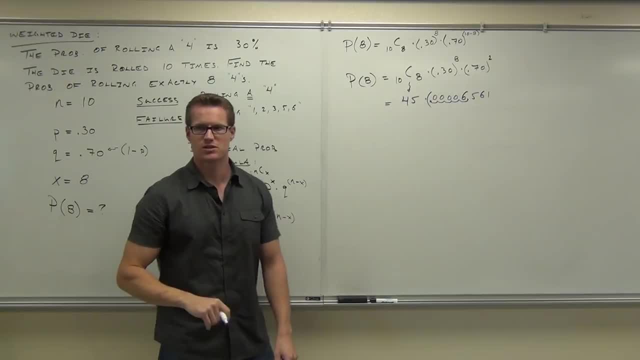 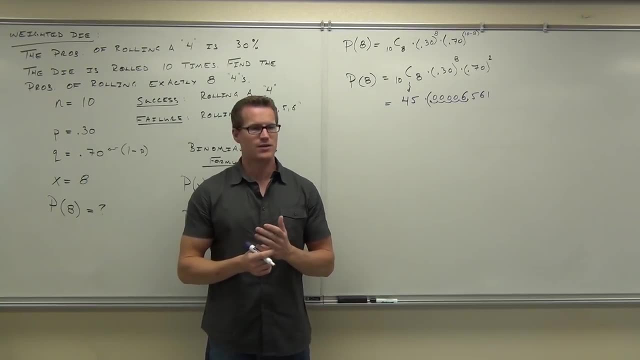 That's what that means. So you do not put 6.561.. You put .00006561.. Should you round these numbers? do you think, Man, they're so small? if you round them, you're going to be off, all right. 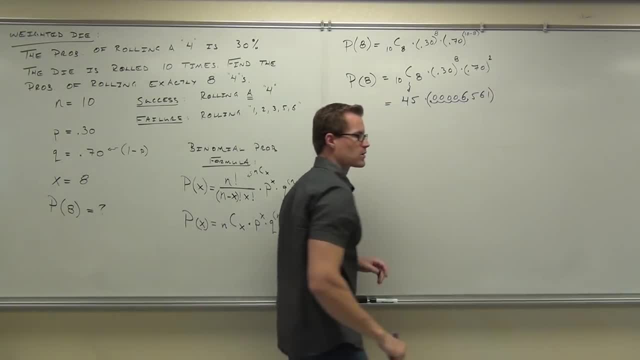 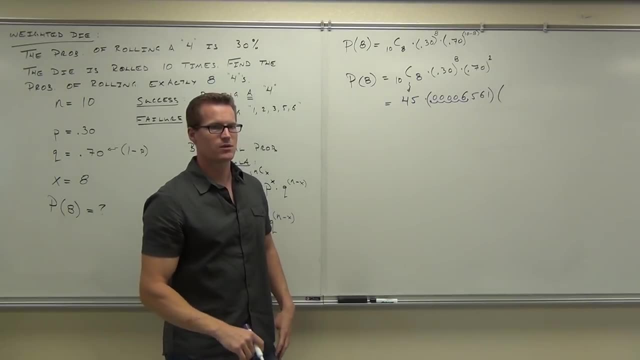 You're going to be pretty off on that, So we can't round them. We're going to put exactly what our calculator says to the end, to the very end, And we're going to do the same thing. .70 squared, That should give you .49.. 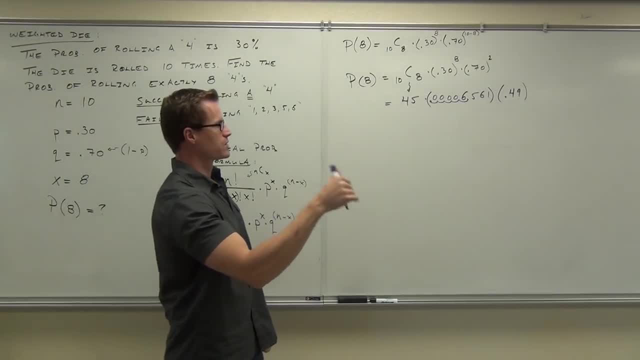 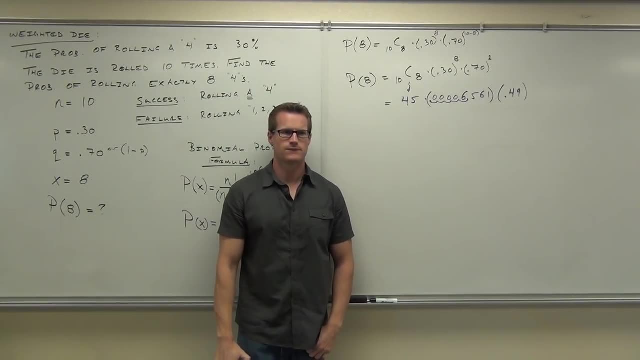 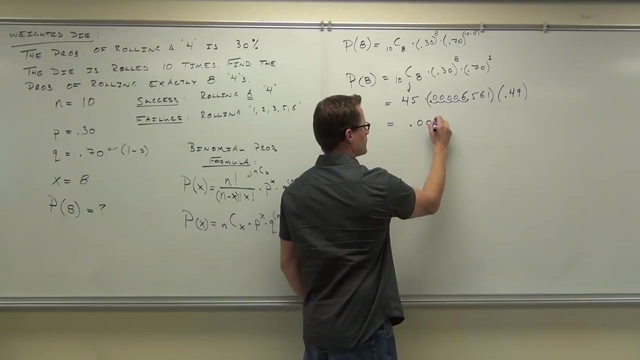 So 45 times, .00006561 times. .49.. .00144.. Okay, say that one more time. .001447.. Seven, Yeah, just round it. Six, sevens, It's probably 6666 forever. .001.. 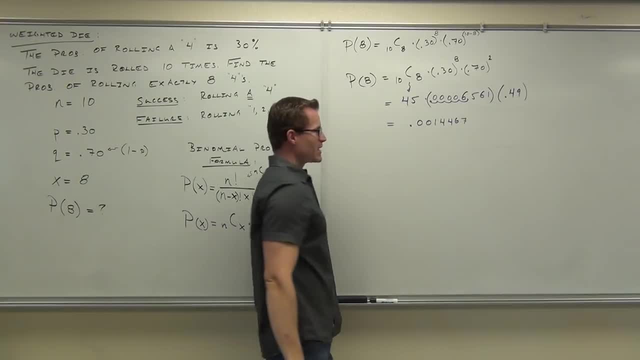 I'm wrong. I mean it's probably going to be .01, right? Yeah, okay, so that's good enough for us. In fact, most of the time we're going to end right about here, Most of the time we're going to end right about there, 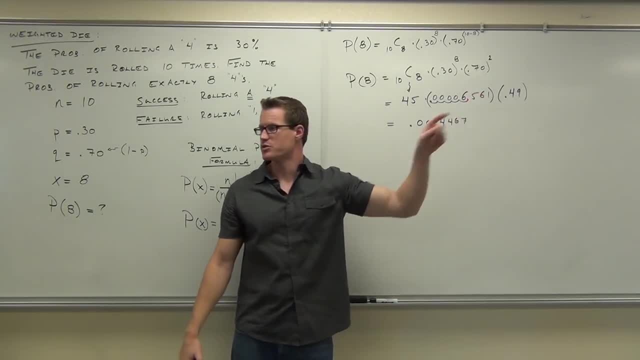 But to get right about here or here or here, you have to be very accurate with your numbers. You cannot round those things. Remember the rounding I told you about. Don't round until the very last step. That's what we're doing here. 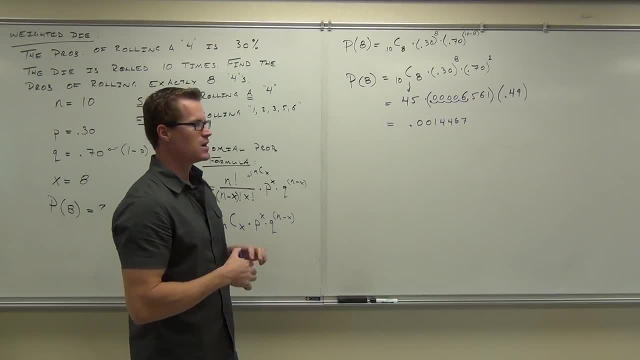 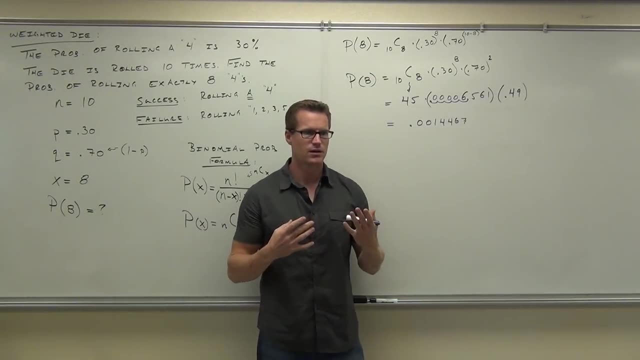 So what does that even mean? Oh my, If you roll a die ten times, what is the probability that you are going to get exactly eight number fours Using this information? Is it me? It's like .1%, .14%. 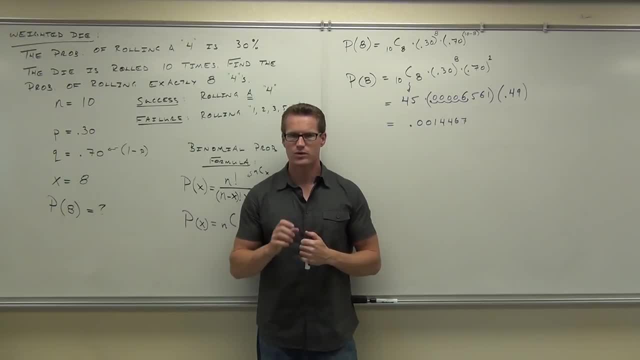 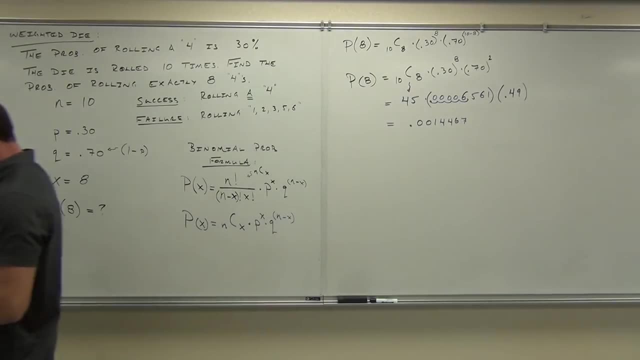 That's pretty rare, right, Pretty pretty rare that you're going to roll that die ten times and get eight, fours and then two of something else's. That's pretty rare, By the way. what distinguishes rare from unrare, or usual versus unusual? 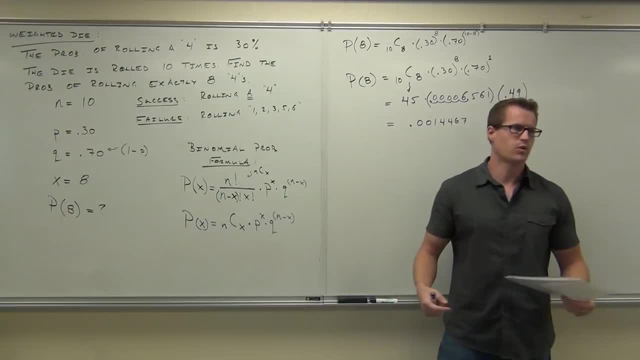 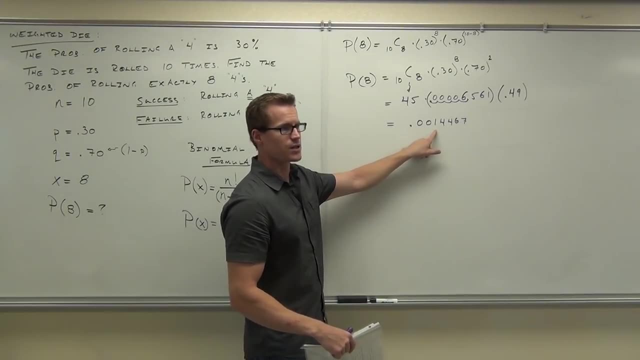 What number are we looking for? probability speaking wise: .05.. .05.. Not .5.. That would be 50%. Okay, .05, that's 5%. If this is less than 5%, which it definitely is, then this is considered an unusual event and this is very. 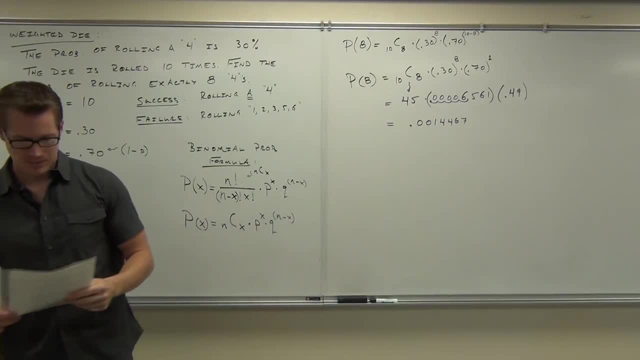 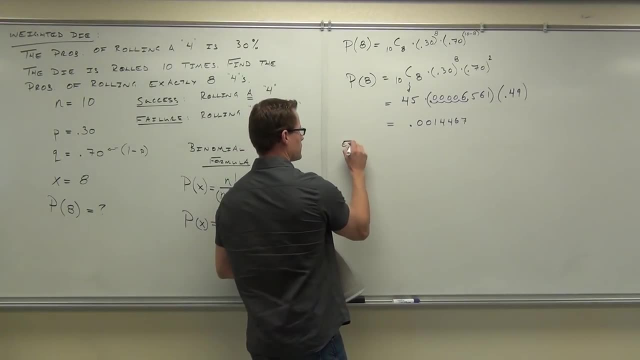 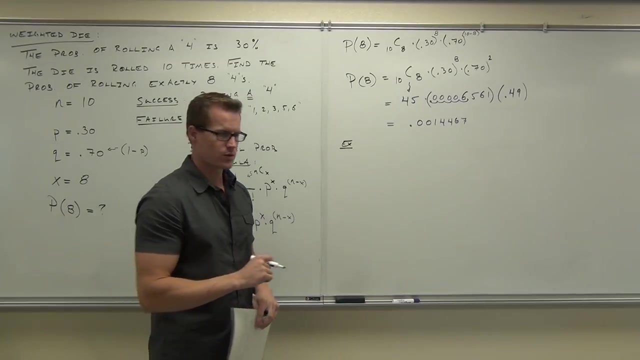 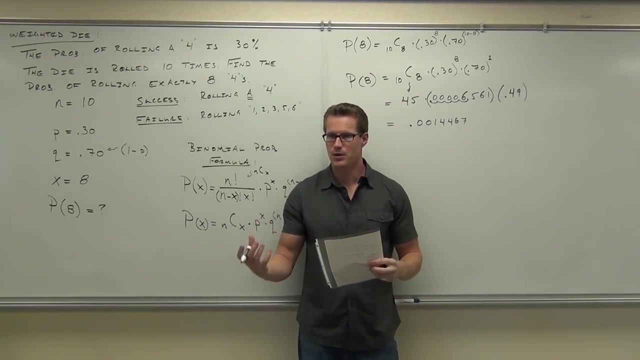 very unusual, very unusual there. Now let's consider: after we did this, how about the next question? The next question is: what's the probability of rolling at most eight fours? You got a 6.. So in this class you're going to feel very good. 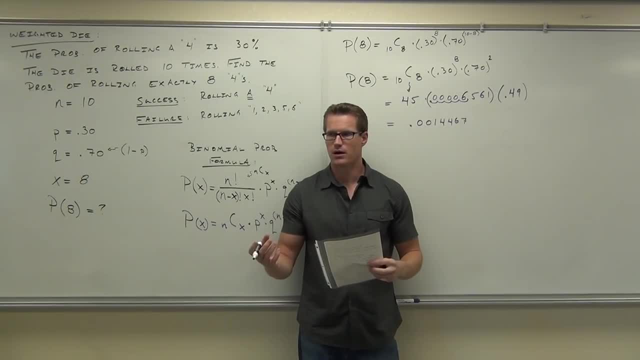 at knowing the interplay between, at most at least, more than or less than and none. Those four situations occur a lot More than less than, at most at least, and none. None's the easy one. None means zero. 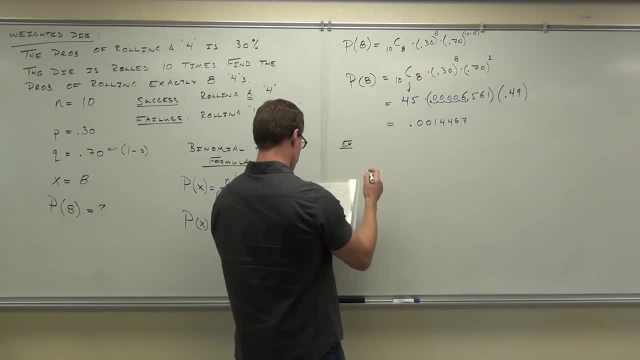 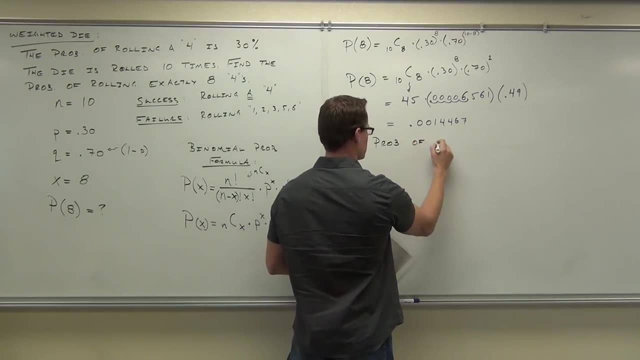 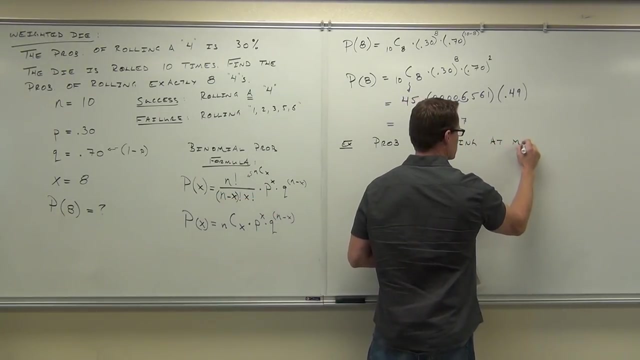 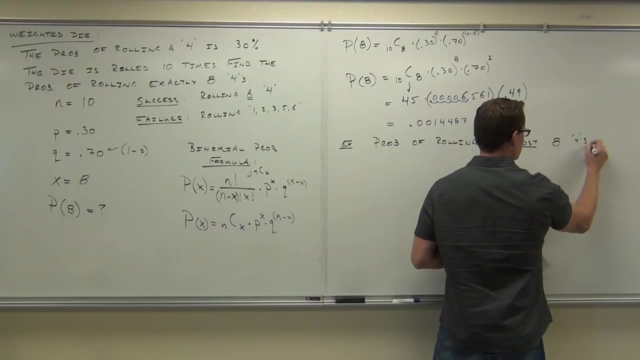 Okay, but the at most and at least, and more than and less than are all different situations. What about finding the probability, using the same information, of rolling at most eight fours? The probability of rolling at most eight fours. 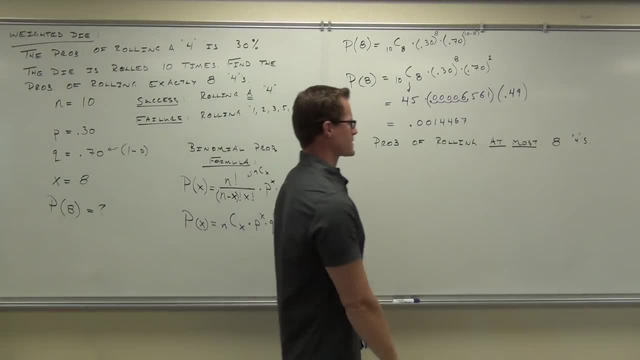 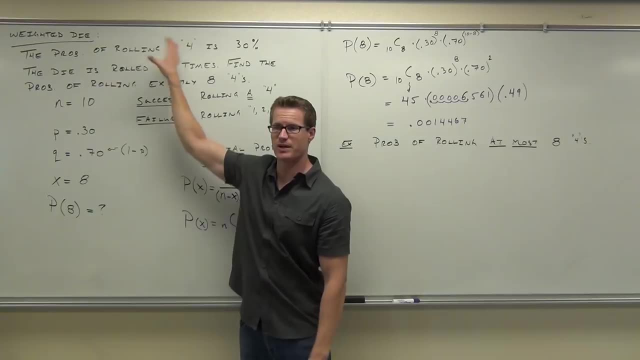 Oh, let's think about it. probability of rolling at most eight fours. we're going to pick up our die and we're going to roll it. we're still going to roll it ten times. okay, same exact information up here. same exact information. 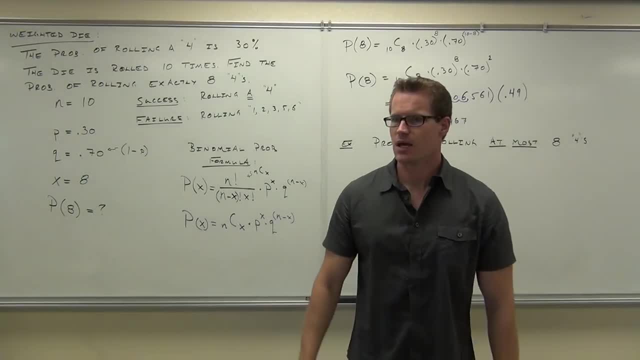 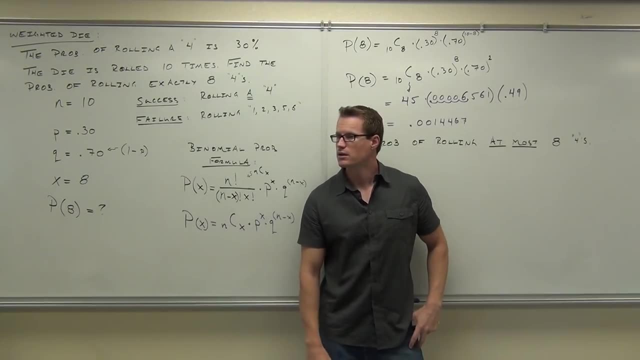 You kind of have to understand, though, what at most means. If you have at most eight dollars in your pocket, at most eight dollars, how much money could you potentially have in your pocket? Could you have eight dollars? Could you have nine dollars? 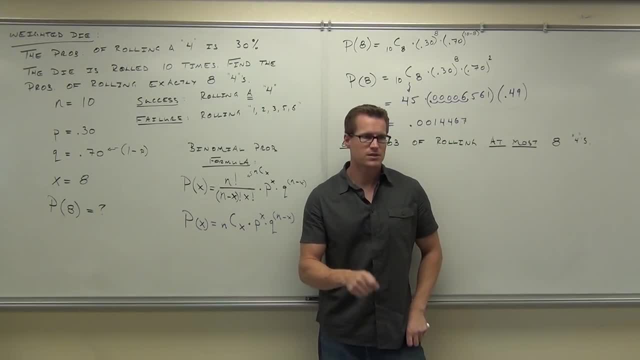 No, but you could have eight. right, Could you have seven, Six, Five, Four, Three, Two, One, Zero, Negative? No, your pockets can't be. this would be negative. right, Your pockets can't be. you won't let me out of state. but no, you can't have negative. 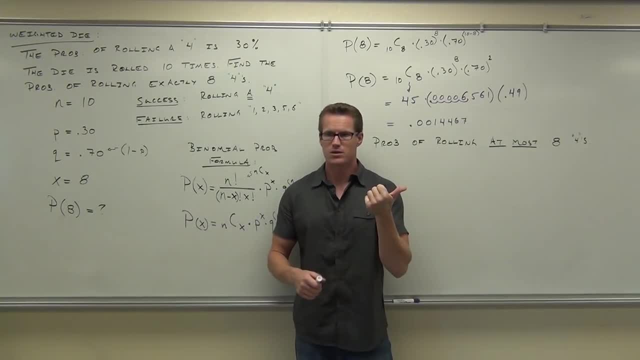 but you could have. in order to satisfy this zero, you could have zero dollars, right, That's at most. it's not even anything at one, two, three, four, five, six, seven, or you could have eight- somehow I got an eye on that- you could get up to eight, including. 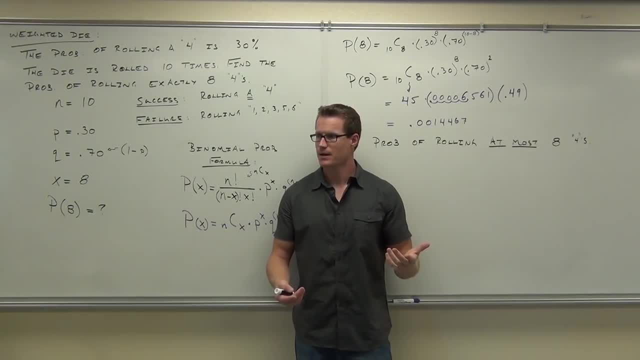 eight, You could satisfy at most. Does that make sense? Less than what if I had said less than eight? If I said less than eight, would eight be included in that? No, Then it would be seven, six, five, four, three, two, one or zero. 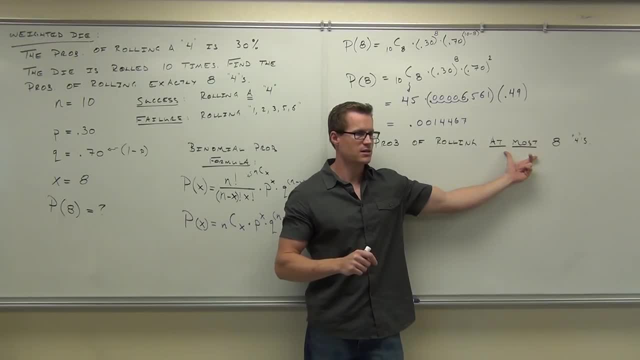 If I said at least eight, at least eight, that would be eight included. and then what? Nine, ten or more than that? If I said more than eight, more than eight, would that be included in. more than eight, Would eight be included in that. 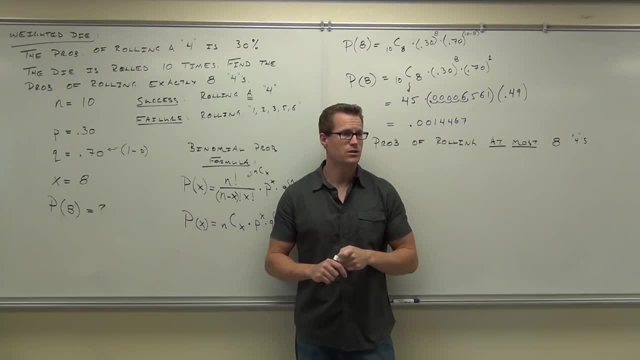 No, If you have more than eight dollars, do you have eight dollars? No, Then you have nine or ten or eleven or twelve or fifteen or fourteen. That's the interplay there between the, at most at least, more than less than, and. you need to know, you need to really know those in order to get these problems right. So we're looking at at most eight. At most eight means you could have zero, one or two or three or four or five or 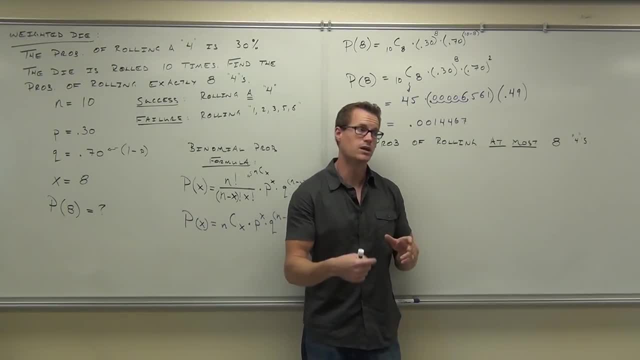 six or seven or eight, number fours that come up in your ten rolls. Are you with this? So this is kind of interesting. You could have zero, one or two or three or four or five or six or seven or eight. 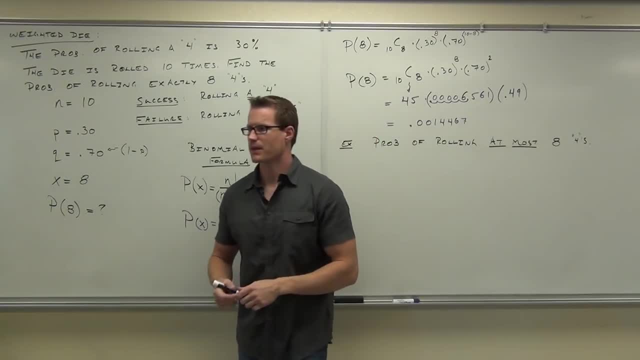 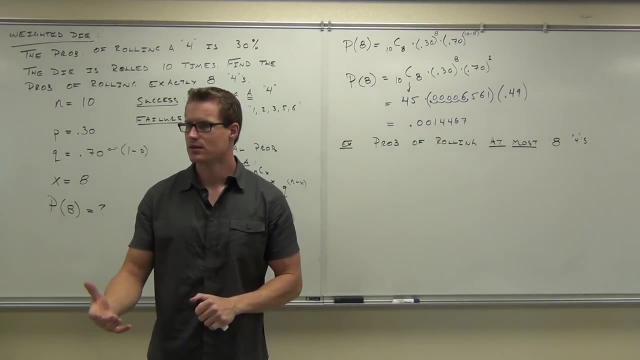 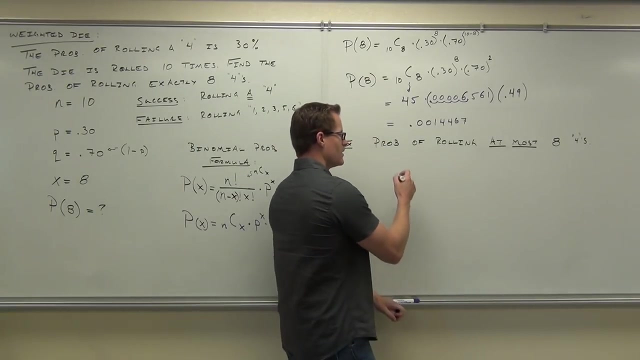 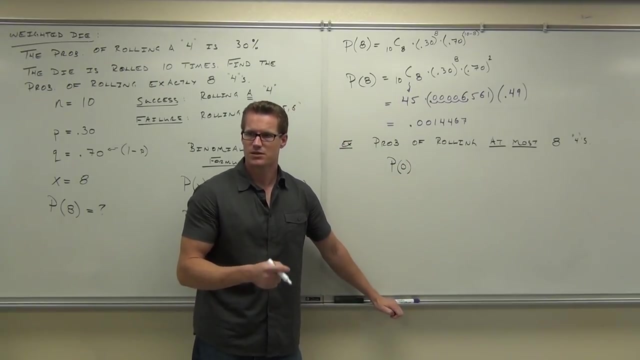 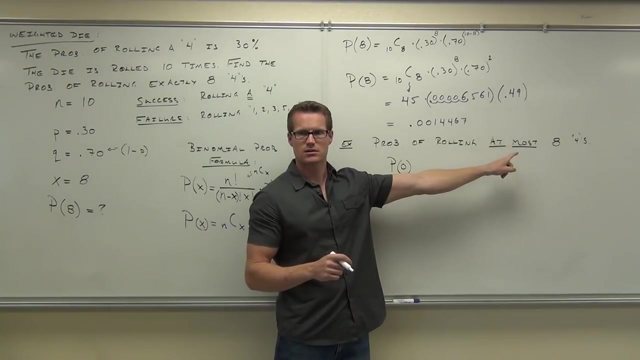 number fours that come up in your ten rolls. Are you with this? So this is kind of interesting. We just said that zero would satisfy this right. Zero successes, Zero successes would satisfy this. Remember successes here. If I get no fours, is that at most eight. 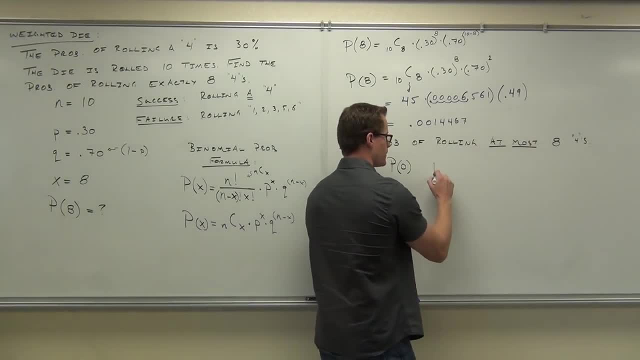 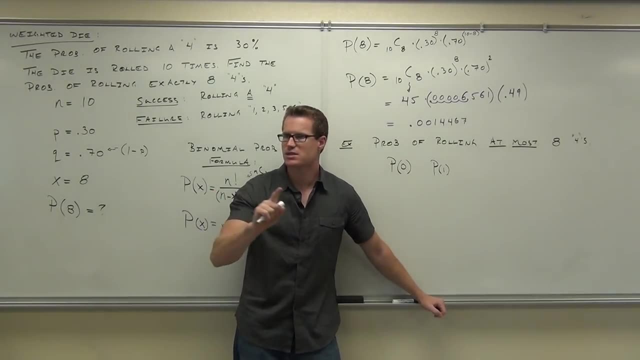 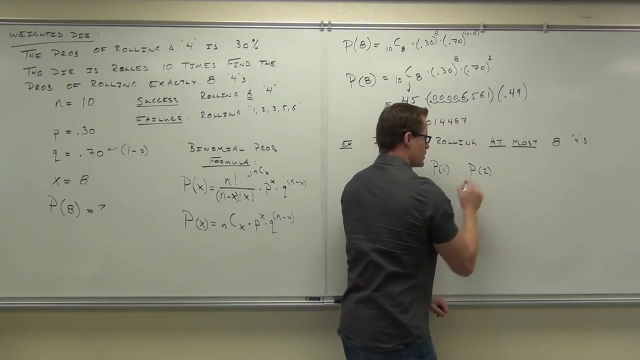 Yes, We also said: or you could get one four, Would one four one success? would one success, one four satisfy at most eight? Or you could have two successes. Would two successes, two fours satisfy at most eight? You with me on this. 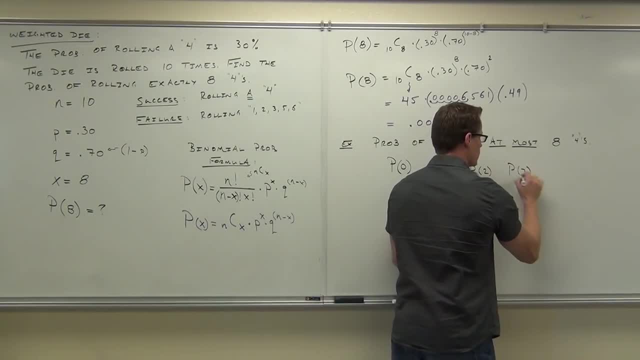 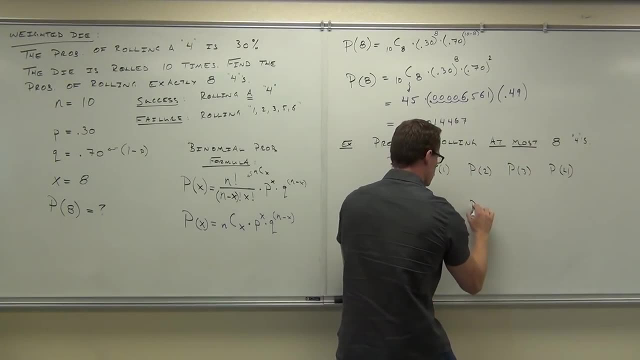 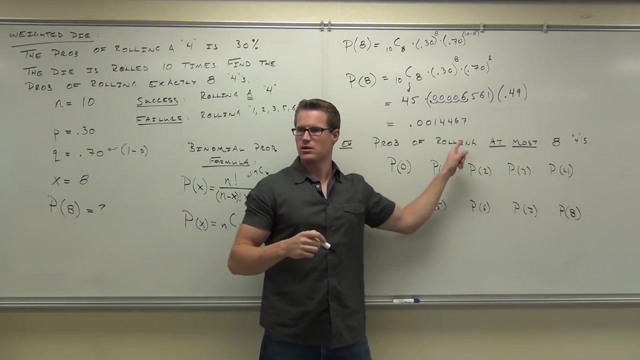 Or three or four or five or six or seven or eight? Do you agree with me that any of these situations would satisfy this situation, Either zero or one or two, or three or four or five? 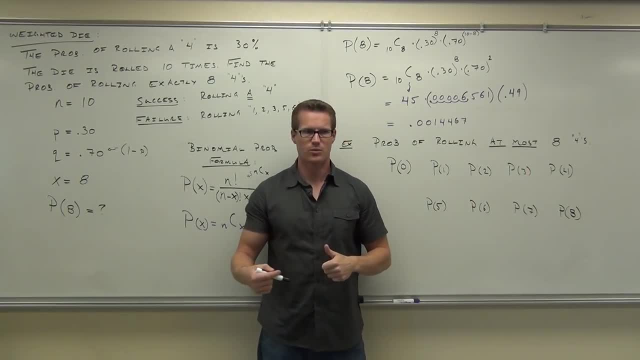 or six, or seven or eight? Do you remember? Do you remember the or? We talked about the or. Hopefully you did go back and refresh your memory on what or means. How do I calculate the probability of an or What do I do with those? 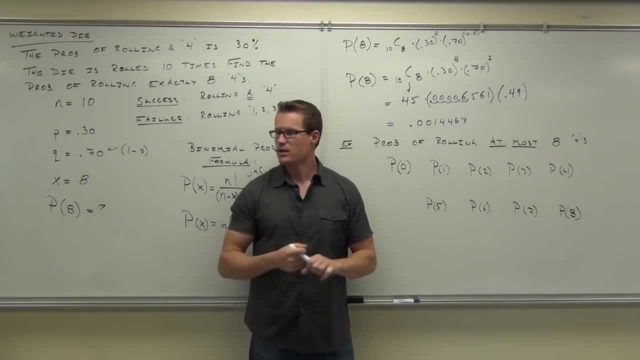 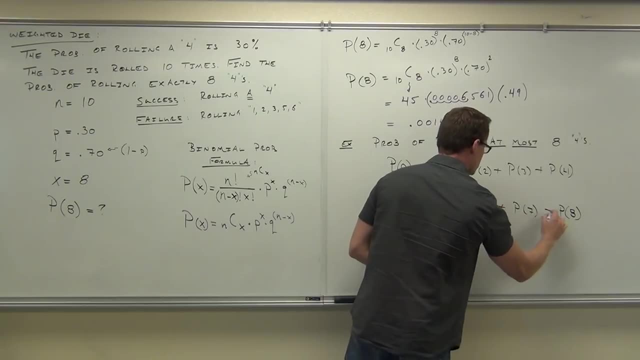 You add them. You add them. yeah, This is the probability of zero occurring, or one occurring, or two or three, or four or five, or six, or seven or eight. You add all those probabilities together because that's an addition rule. 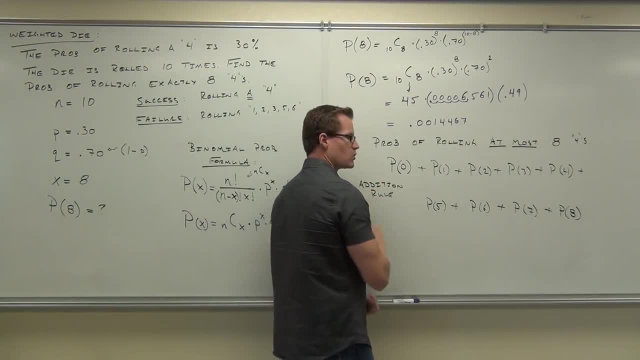 This is an addition rule for disjoint sets. You can't have both three successes and four successes, Can you? Can you get both three fours and four fours? when you're rolling the die ten times? Can you get a certain number of successes and a different number of successes? 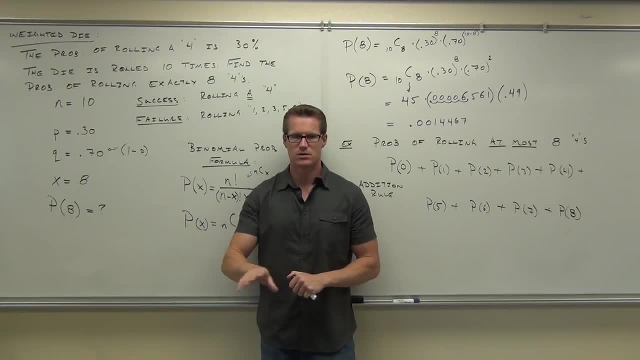 For instance, imagine your head. You're rolling the die ten times. okay, One, two. you're rolling the die. Can you get Out of your ten rolls? can you get both three fours, only exactly three fours and four fours at the same? 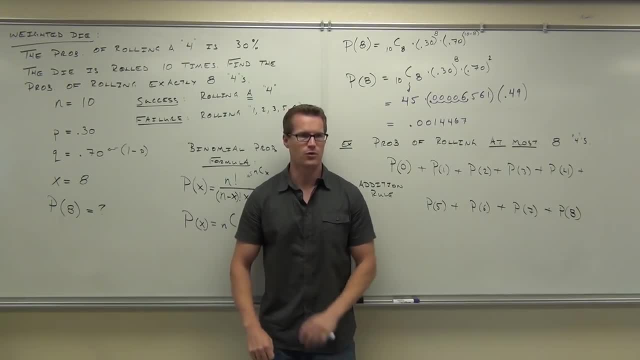 Can you get both of those? exactly three fours and exactly four fours. Those cannot happen at the same time. You can't get that. So here, when we're doing this, these are disjoint sets, disjoint outcomes. We add them all up. 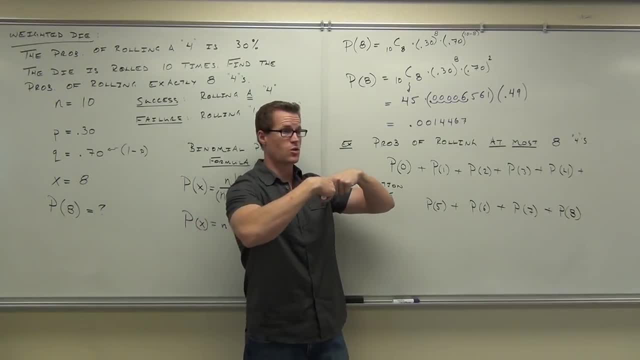 We don't have to worry about a crossover. That's what I'm trying to say here. There's no crossover, There's no and of them happening at the same time. We just add up each of those probabilities, So the probability of rolling at most eight fours comes. 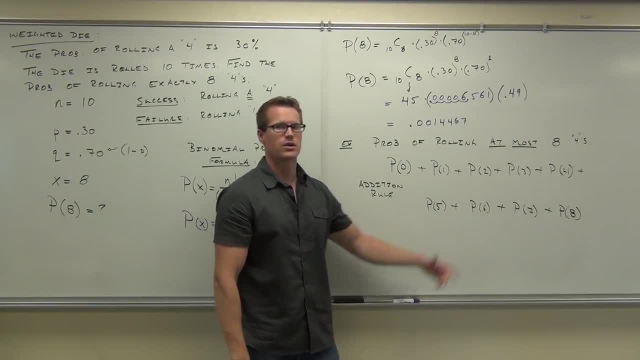 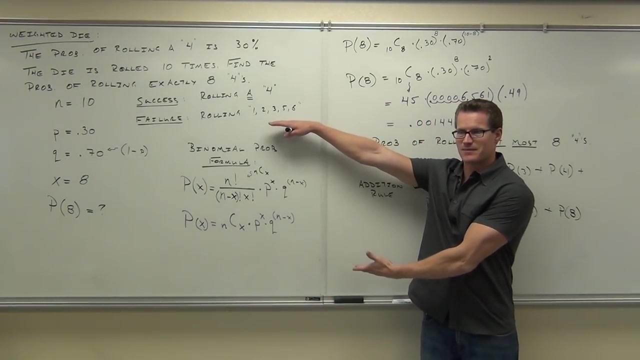 down to the probability of rolling zero, plus the probability of rolling one plus two plus three plus four, five, six, seven and eight. How do we find each of these probabilities? It's that right there? Can't you find the probability of zero? 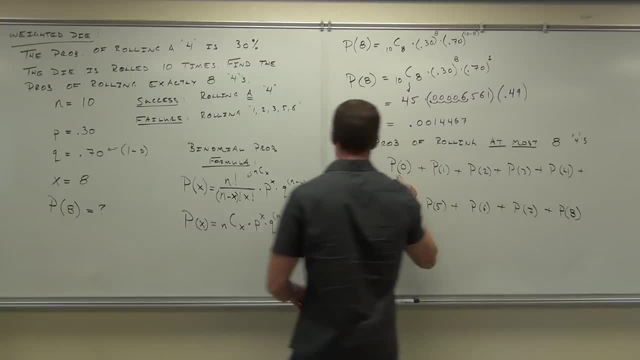 Let's do this real quick. Let's see what the probability of zero would be. Probability of zero: is that rolling a zero? Does that mean rolling a zero folks? What does probability of zero mean? No fours, No fours, It means you have zero successes. 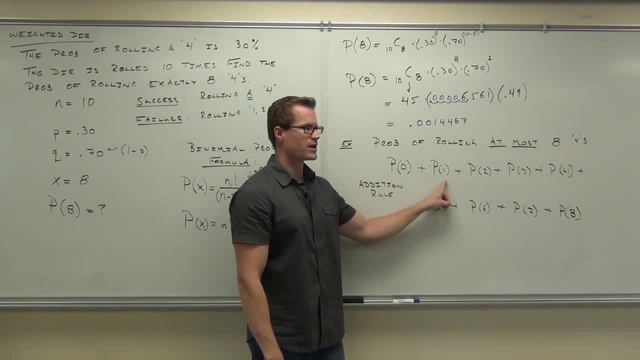 It's not the probability of rolling a one. I don't care about that. What I care about is one success: It wasn't the probability of rolling eight. That was definitely not an eight. We don't even, can't even, roll an eight. 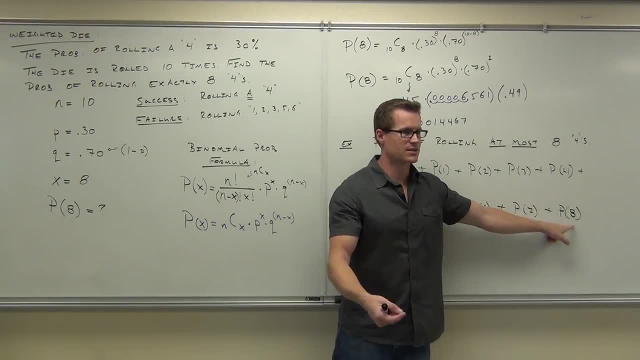 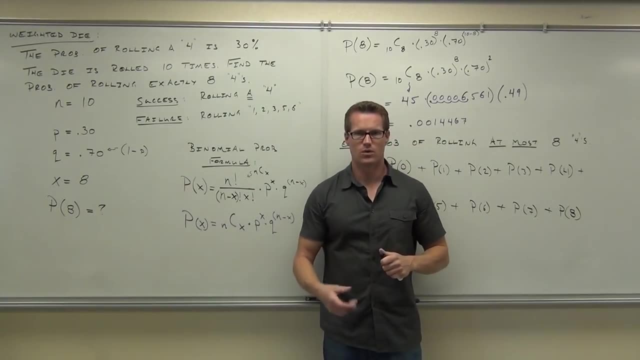 This was the probability of rolling eight fours or getting eight successes. How many people understand the difference between those things? You kind of have to to really get this stuff. Otherwise you should be able to do it. You should be asking a question or kind of think. 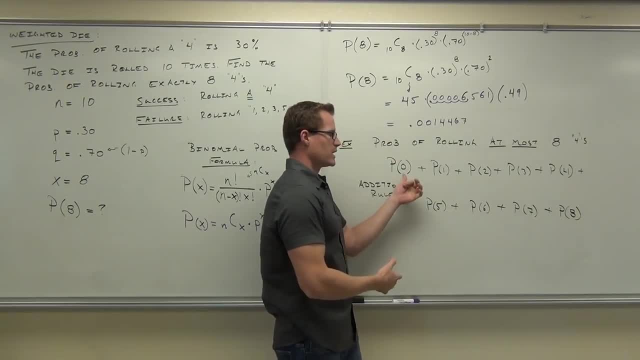 about this a little bit. So this is not the probability of rolling a zero. That can't even happen. All we can get is one through six. This is not the probability of rolling a one. We don't care about that. It's not the probability of rolling a four. 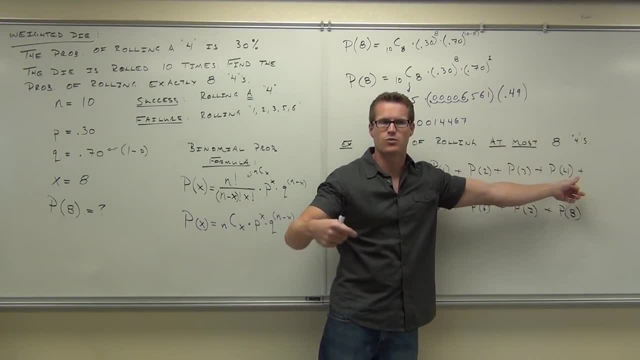 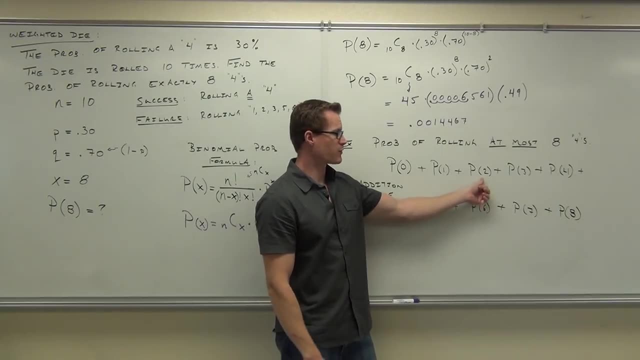 I don't, I don't, I care about how many fours I'm rolling. This is the probability of rolling zero fours out of ten. This is the probability of rolling one four out of ten. This is the probability of rolling two fours out of ten. 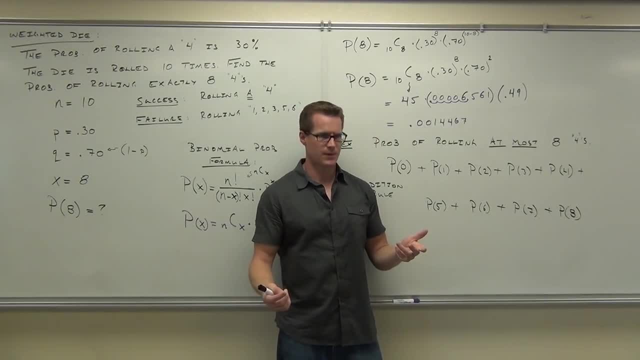 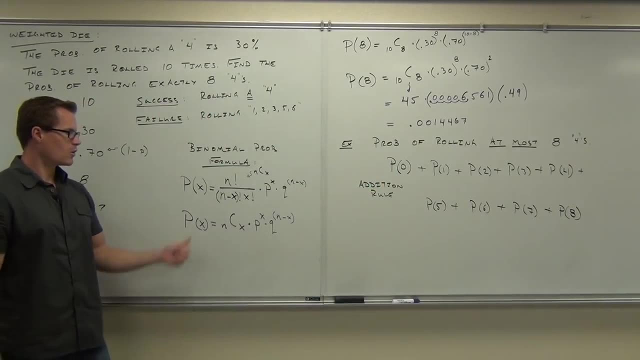 or eight fours out of ten. Do you see the difference there? imagine, if you. okay, that's, that's the big point here. so the probability of rolling zero fours out of ten or X become zero shit. when our n change what our n change what our X change, that would not become zero. 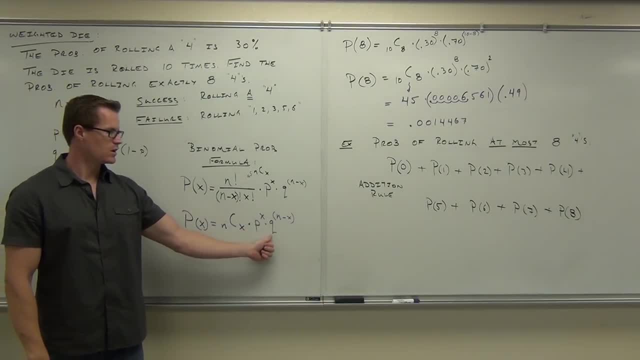 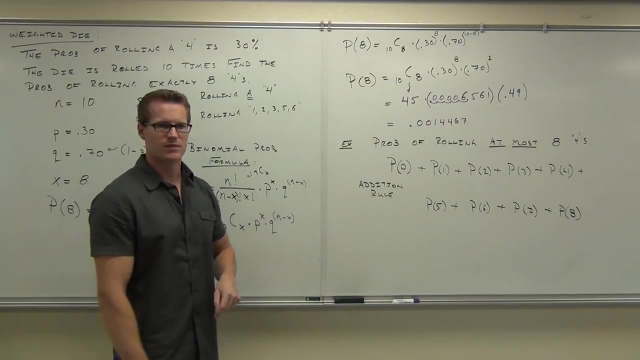 what our P change: X would become zero, Q would become would change and minus X, that would become ten. this would be zero, that would be ten, this would be zero. and choose zero would still be something that you need to calculate. it was still happening. calculator, so I can become zero. this probably does exist. you'd have. 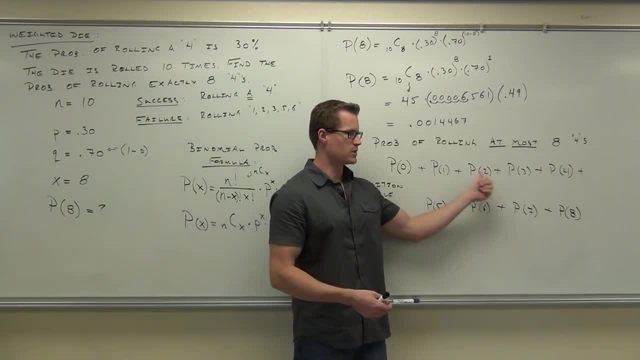 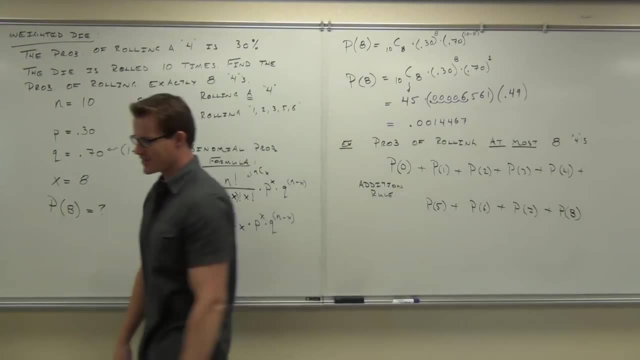 to do that for this one, then you'd have to do that for this one and do that eight times and add them all up. do you wanna do that? why not? super fun. yeah, it takes way too long, so you could do it though, couldn't you? you could do it though, couldn't you? 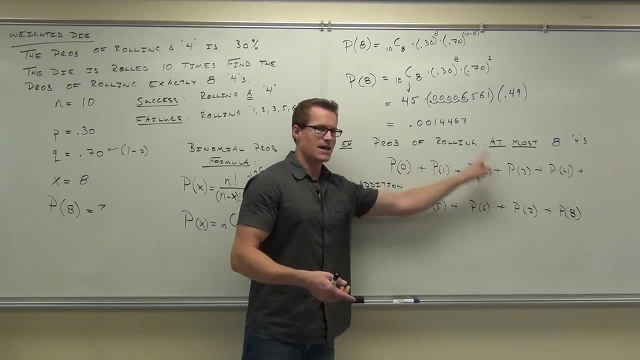 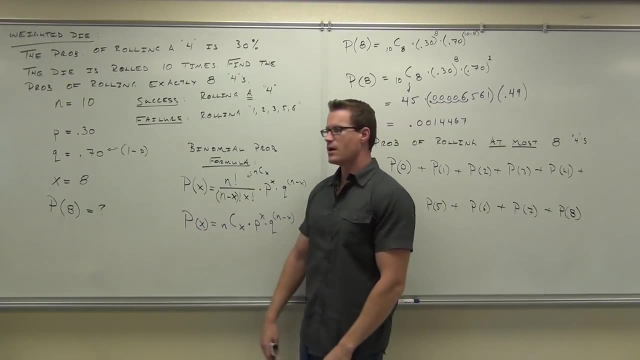 here's one. here's one, two, three, four, five, six, seven, eight, that's nine formulas that you would have to do nine times each time. the only thing that will be changing is X, and you can redo your formula. find out this number nine times and add them all. 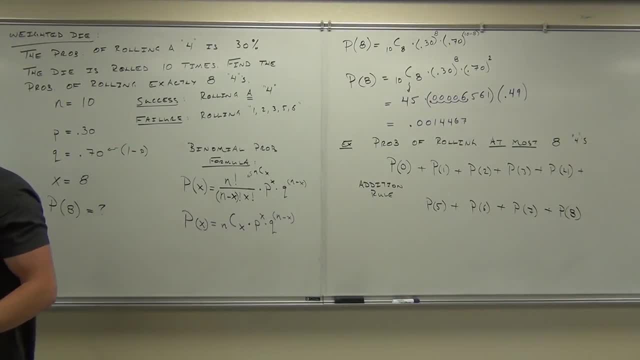 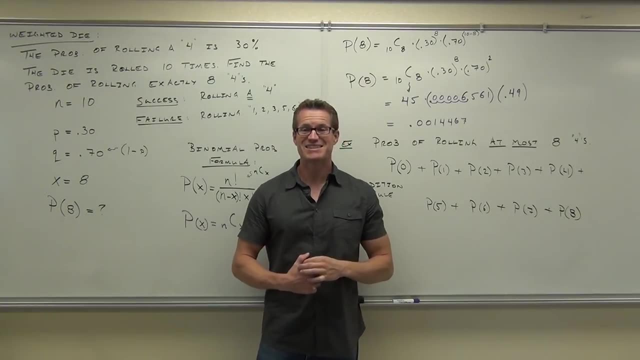 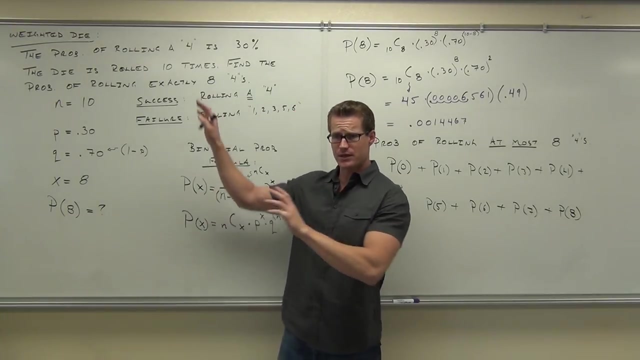 up, however, some guy had a lot of time on his hands. it was me- and has done this for you. you don't see what's done for you. it's kind of awesome. do you remember how I told you that this action, this whole act of doing this, really had nothing to do with the? 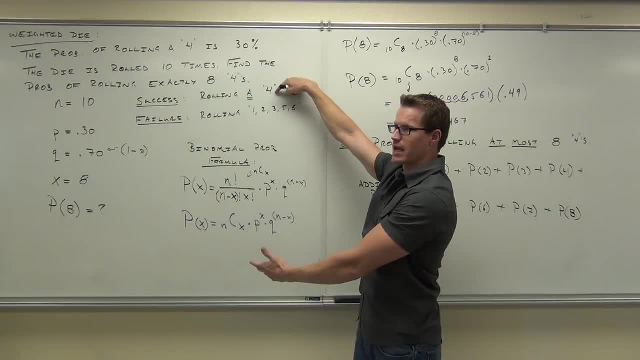 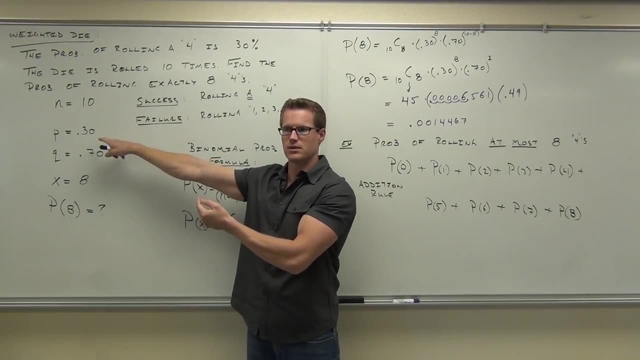 fact that we were rolling a four. it had to do with the fact that we had ten trials and we're trying to find eight successes with a certain probability, and you agree with that and you said, okay, yeah, it's really nothing to do before, it's all about the number of successes. some guy realized that and he made up a 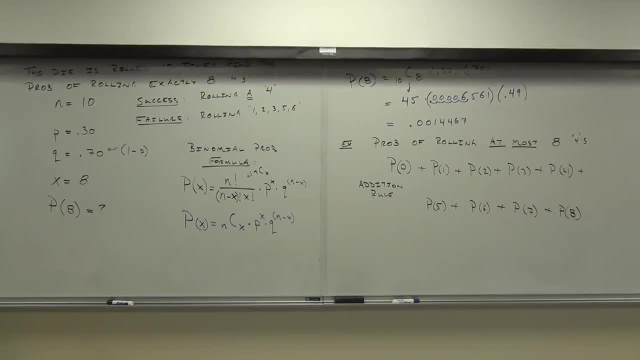 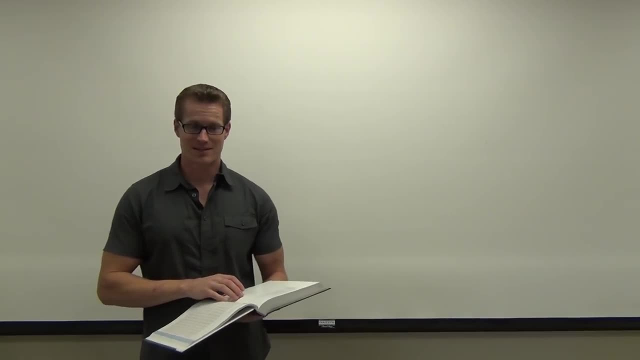 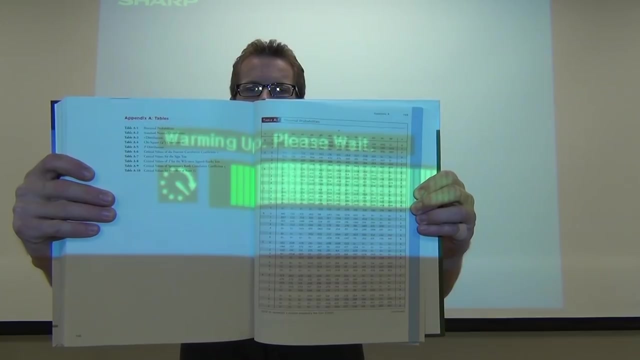 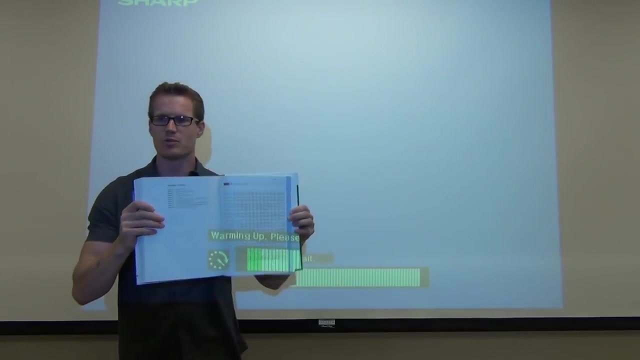 chart that basically does your work for you. so in the book that magically appeared in my hands, what you're gonna find on page, write this down: 749. see that, show and tell. 749. you get this nice table thing. looks like that. and listen, the very top is binomial probabilities- never, ever talking. 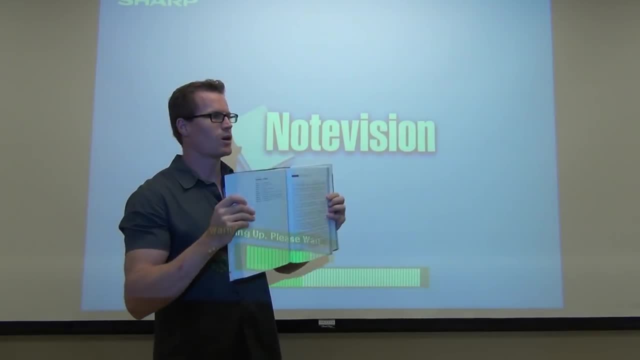 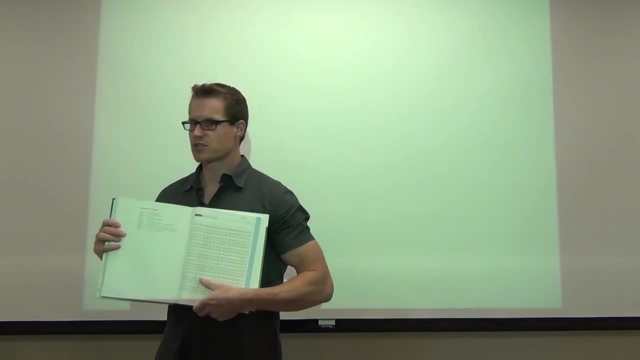 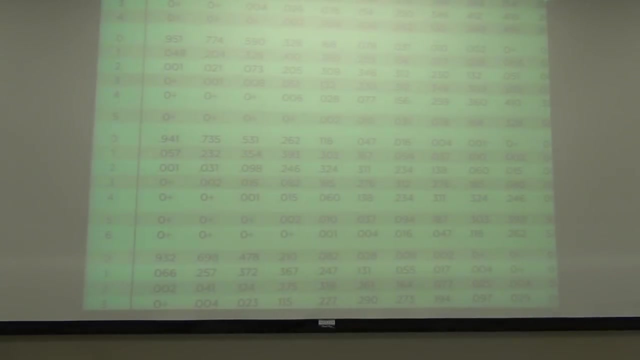 about binomial probabilities just right now. by no, we probably somebody did all your work for you. he found all the probabilities to the fourth decimal place. third decimal place. sorry of all the situations we'll accomplish or that we'll have to face in this. let's look. 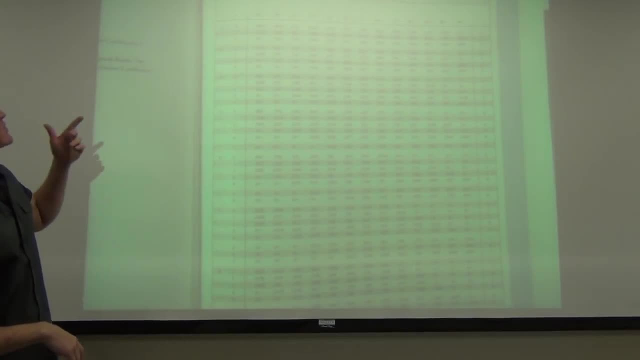 so here's how to read your table here. if you read your table says binomial probabilities on the top. I want you to notice. up at the top left hand it says some letters we should be kind of familiar with. what do you see? I see n? n stands for what number of x? 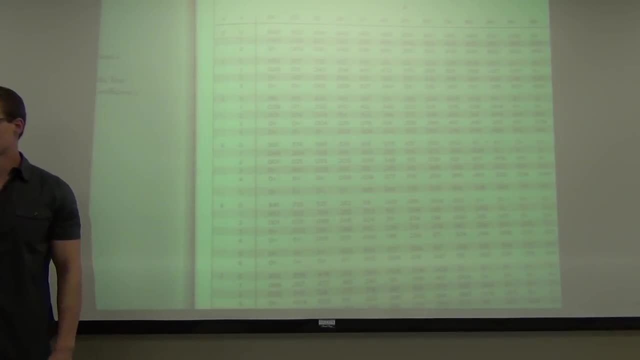 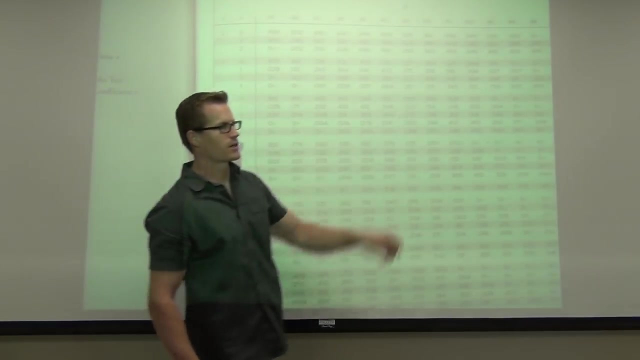 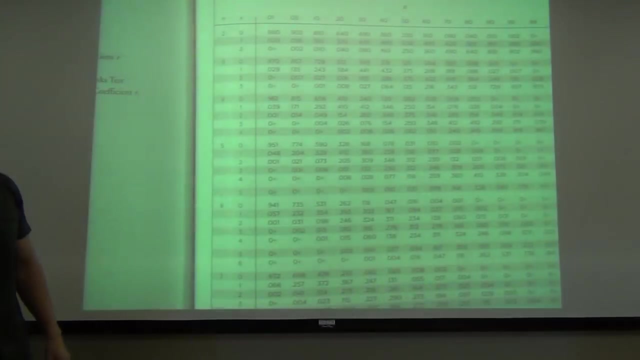 stands for successes, for sure. it's not based on the value you're trying to get. some number you're trying to get also is another. what's that letter can you read? that? is your eyesight that good? that's a, that's a P. once you turn those lights off, for me, would you? that's the P, that's a. 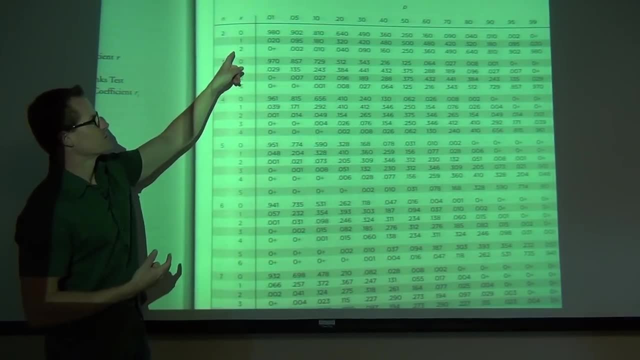 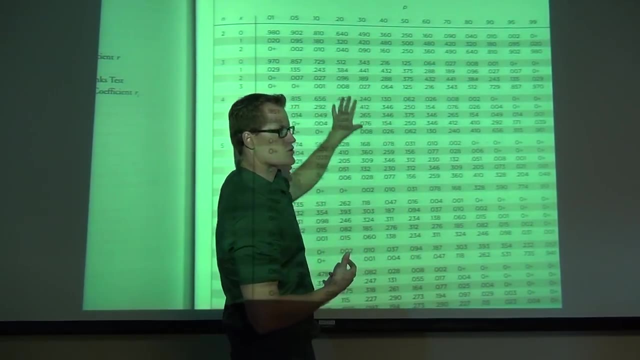 probability of getting. is this the probability of getting two successes, or is this the product of each individual success? right here, this: these are the probabilities of getting certain number of successes. that's kind of cool. it does the work for you. so this is the probability of getting each. 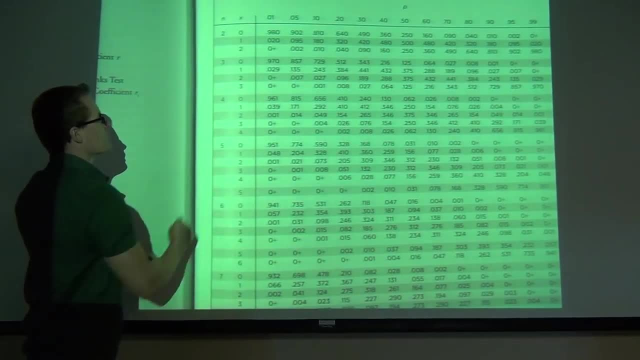 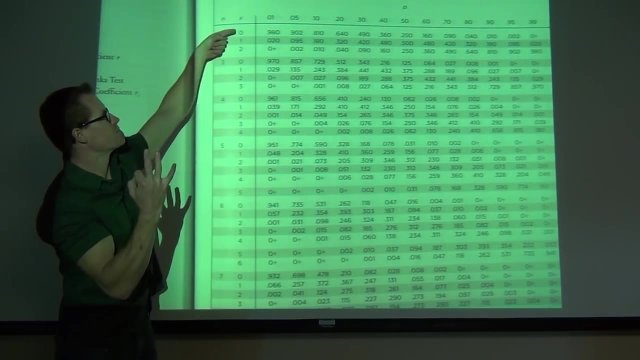 individual success based on this information. here's your n, here's the number of successes you're looking for. now. you'll notice that if you'll have two trials, there's only three situations. you could add zero successes. one success or two successes, that's it same thing. with three trials, you have zero one. 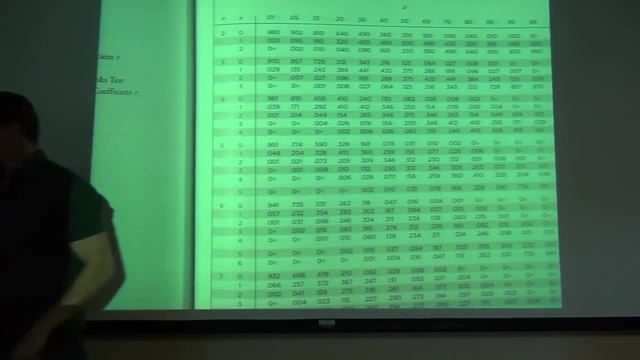 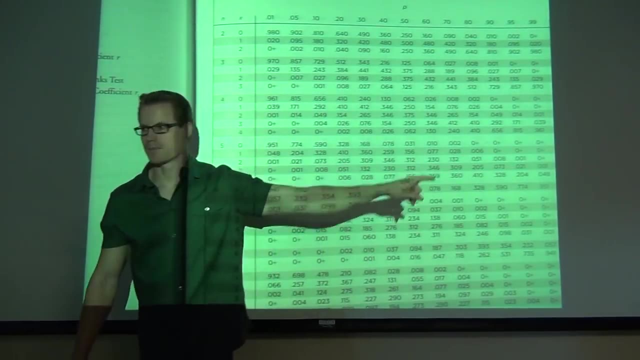 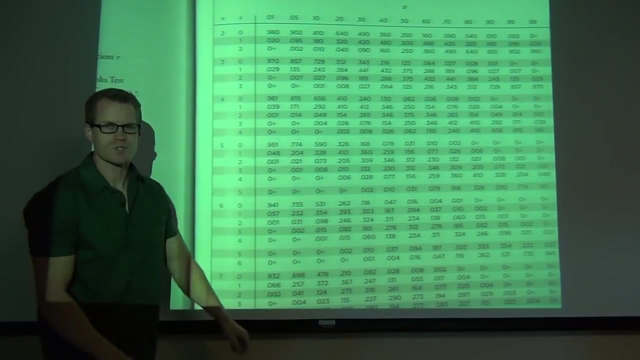 two or three. it builds as you keep going through and going through. so let's see if we can do our problem. I hope you remember the probability over here was point zero, zero, one, four, four. right, let's go ahead and try to find our situation on this on this table over here. what was our end in our 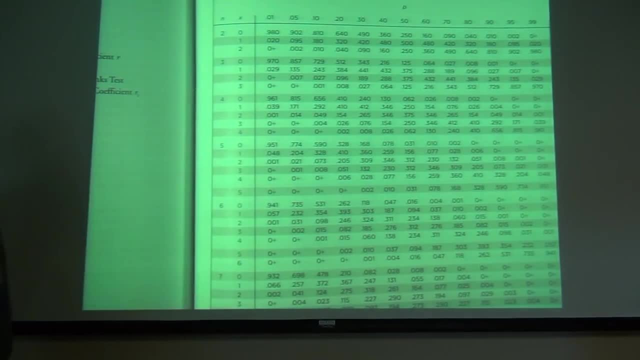 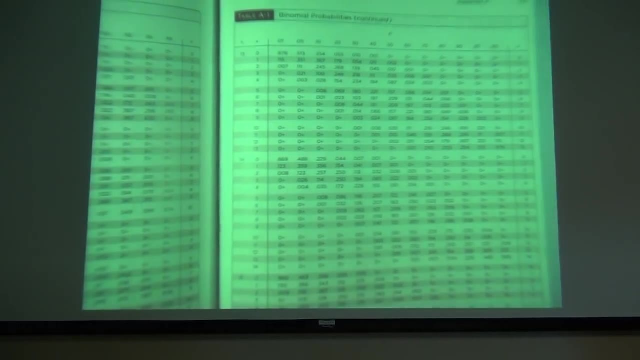 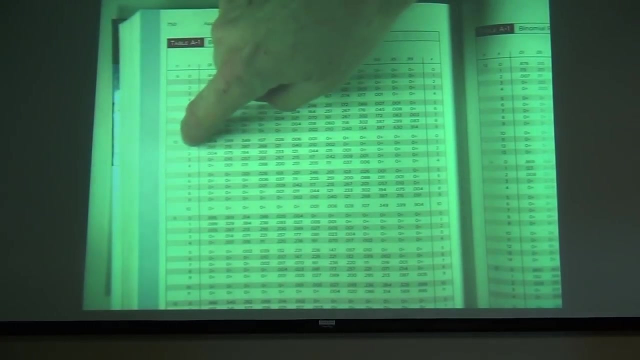 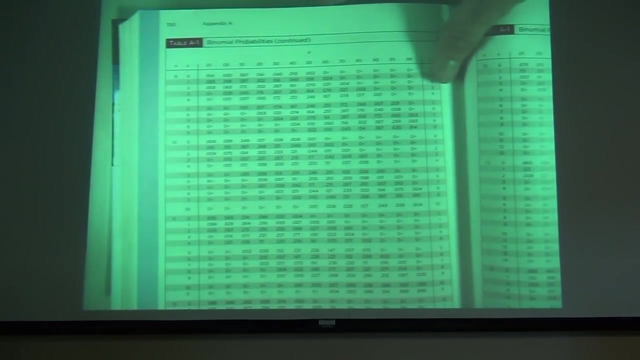 rolling the dice situation. let's keep going. we have- I'm seeing here's- n and is nine, right down here and is ten, so we should be in this, this segment right over here, where it is ten. are you with me, folks? next thing we're going to do is: 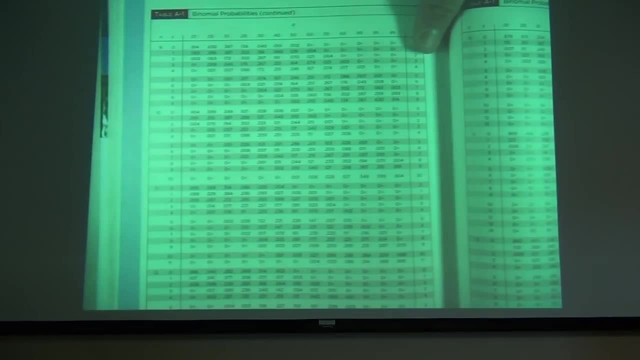 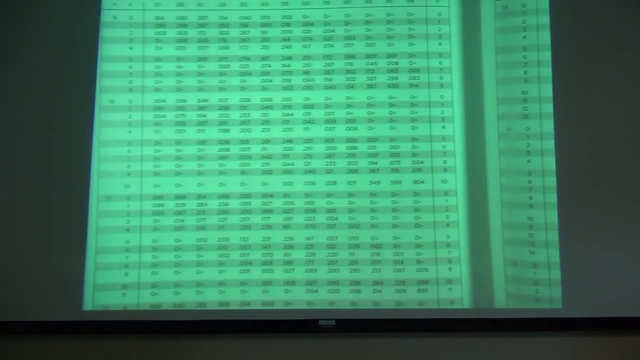 we're going to look for the number of successes that we were trying to find now in our situation. we were looking for how many successes exactly? and its for eight successors. that's not zero. we're 8 successes and the Then the probability of each success was how much. 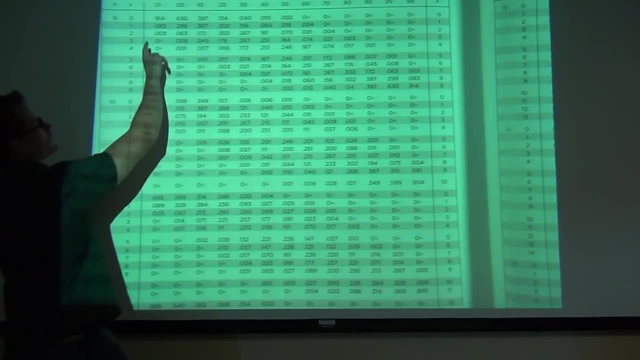 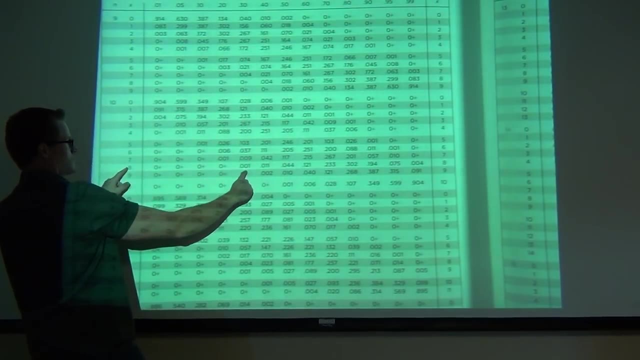 Anyota, thirty percent, okay. so what we're going to do? probably success. we're finding that. we're finding n ten, eight successes. we're looking for that. see where those things cross: point zero, zero one. we were more accurate, weren't we were point zero, zero one. four: 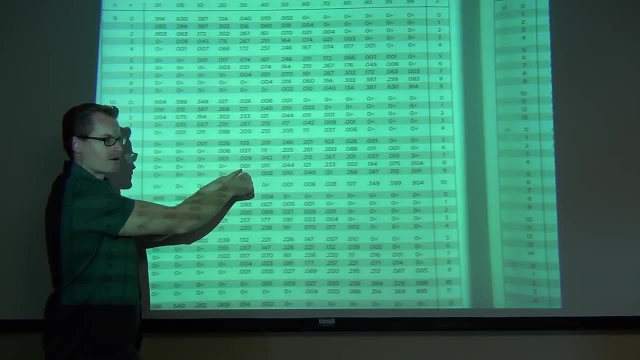 But tax Inflation is correct, so we still down to zero. That's the same value. that's what the guy found. He just rounded it to three decimal places. So we can find that value- .001, just by looking at a table. 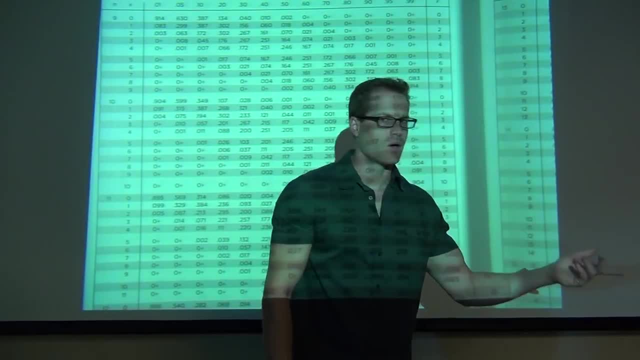 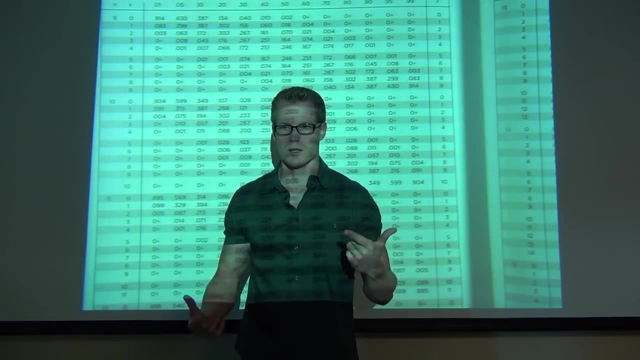 Now, why are we doing this? We could just do the formula. Well, when we are looking for the probability of at most- oh geez, at most- eight, that means zero, or one or two or three, and we would have to do the formula. 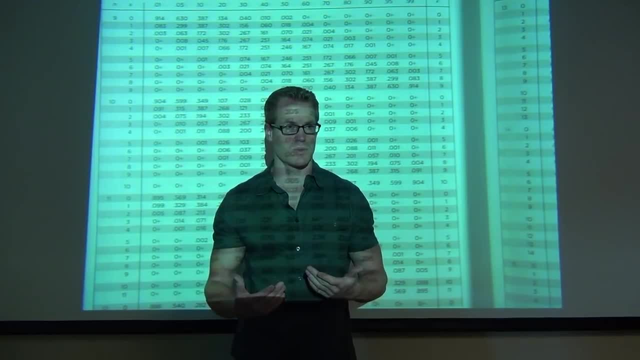 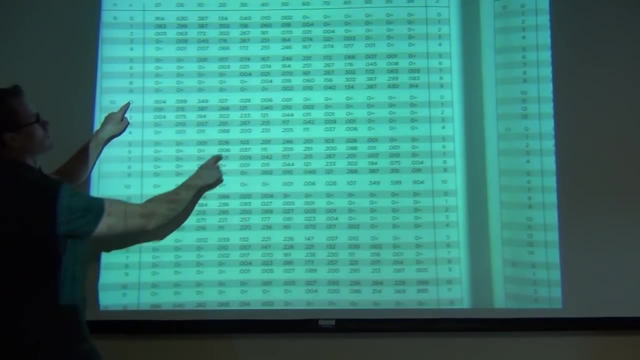 nine times to find out at most eight successes. Remember that. Can you find the probability of zero successes just by looking at this? It's right here that one. It's .028, that's great. How about the probability of one success? 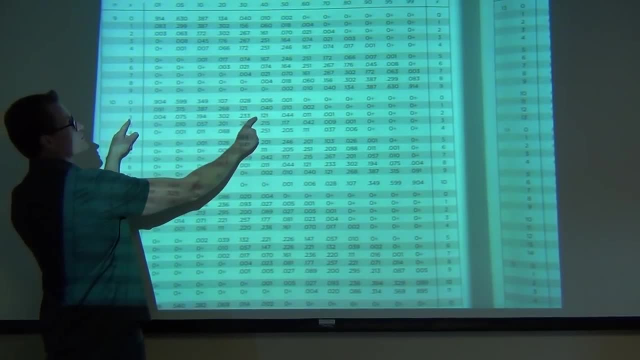 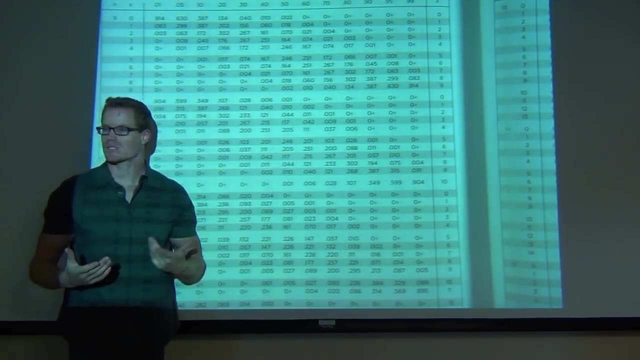 Oh, it's 1.21,. someone's already done the math for you: Two successes .233,, three successes .267.. How can I find the probability of at most eight successes? What am I gonna do with those values? I was just reading to you. 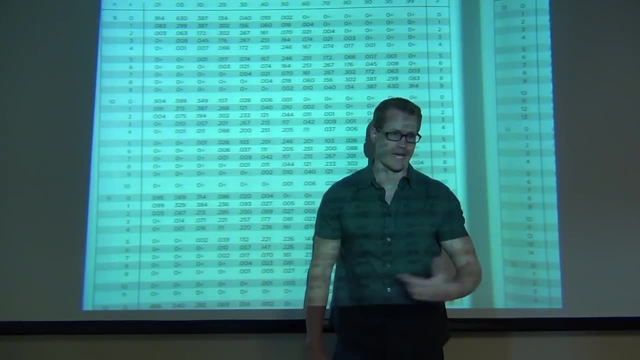 Let's just add them. We know that this was addition rule, right. So what we had up here on the board was the probability of zero plus the probability of one, plus the probability of two successes, plus three, four, five, six, seven, eight. 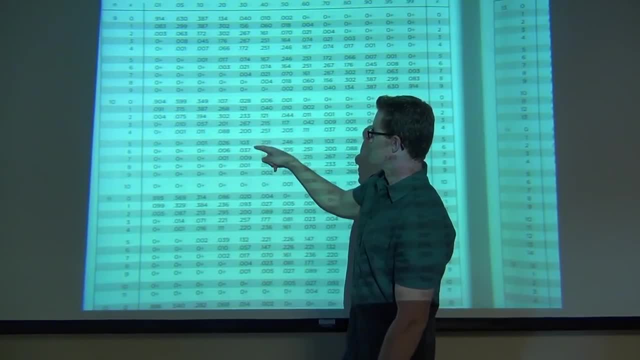 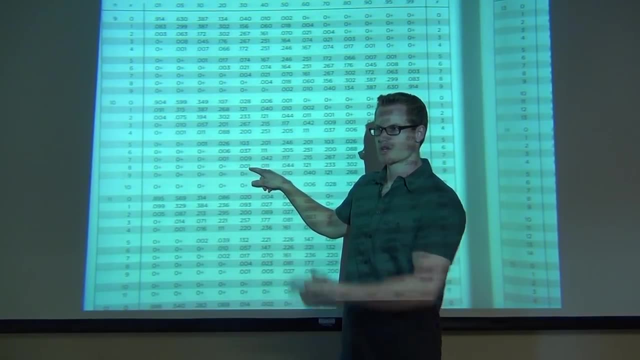 Let's just add from here down to and including the eight. Here's what you have to be good at. okay, Everybody's gonna know to do this, It's not hard. You just go to your n. the x is listed for you. 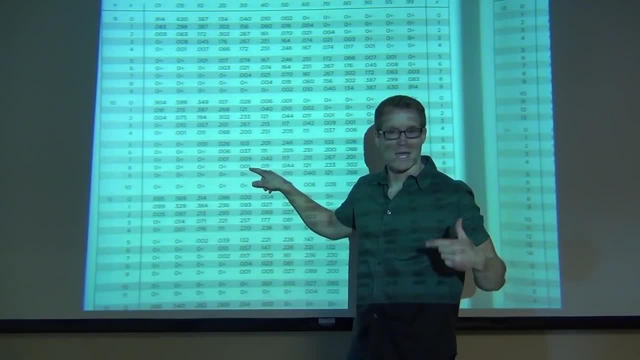 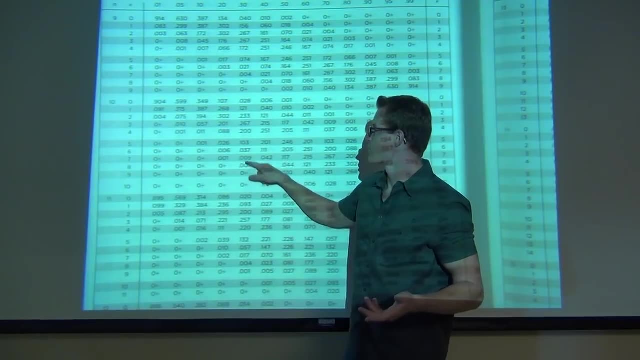 I mean even letters. are there the p's listed for you. You just have to know what at most means, at least means more than and less than. You have to know, basically, whether to include this eight or not, whether to add up all these or all these. 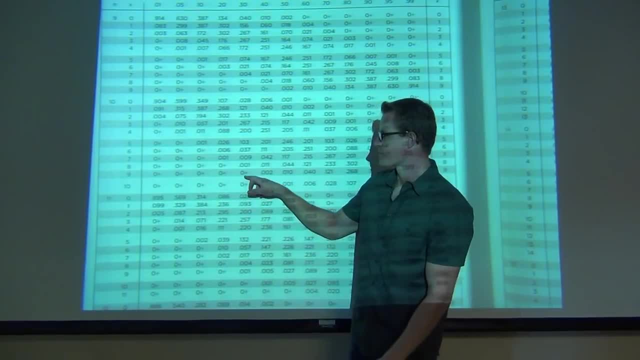 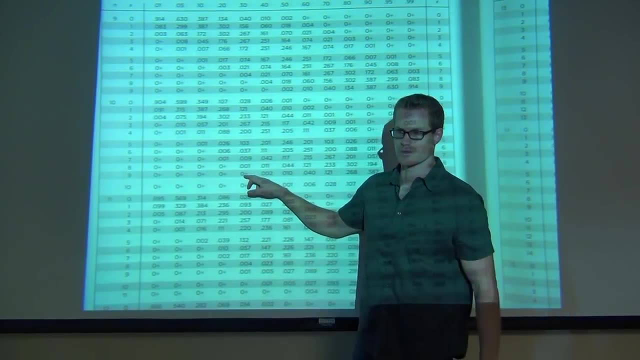 That's what you have to know. Also, one little piece of information: the zero plus. just use zero for that. Zero plus means less than 1,000th, so .000, something. that's what that means. So you would be able to find that on a calculator. 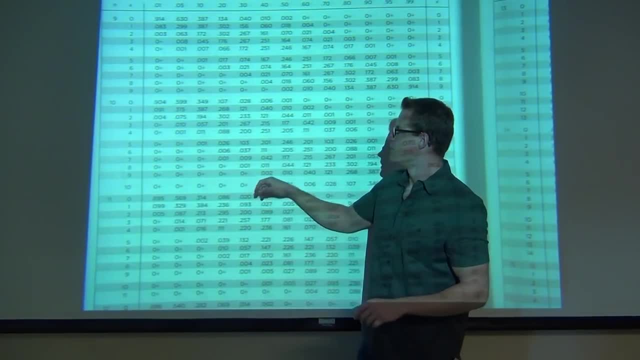 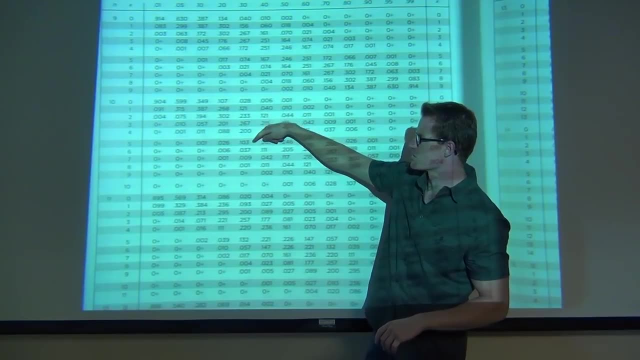 This won't let you do that, So you have to use zero for that. So for us, let's go ahead and do that. Let's write these down: .028, .121,, .233,, .267,, .200, and so on until you get to the eight, okay. 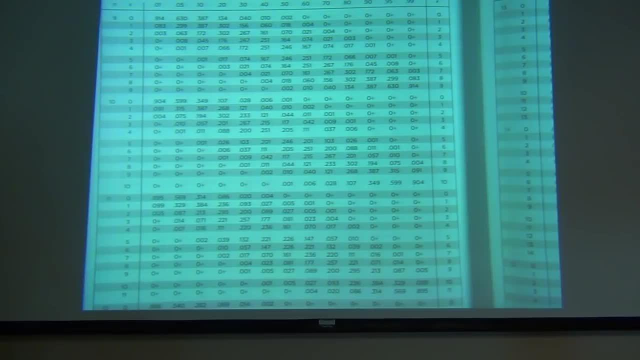 Write those down, because I'm going to show you how to do this on a calculator. Did you do it? .999.. Yeah, you should add like .9999.. Almost exactly what I thought. Good, What now? .999?. 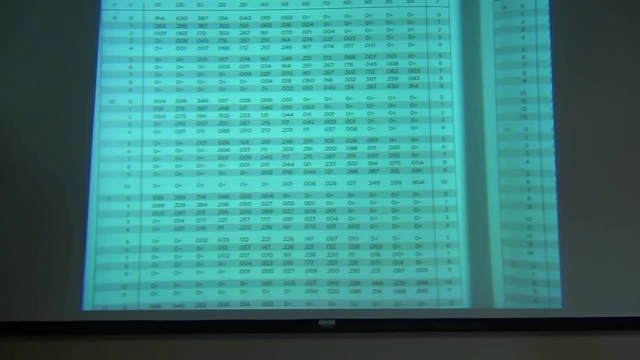 Yeah, Oh yeah, .999.. Do you have all those written down? Does anybody have all those written down? Okay, good, I'll write them in just a second. I'm going to close this book. I'm going to show you how to do it on a calculator. 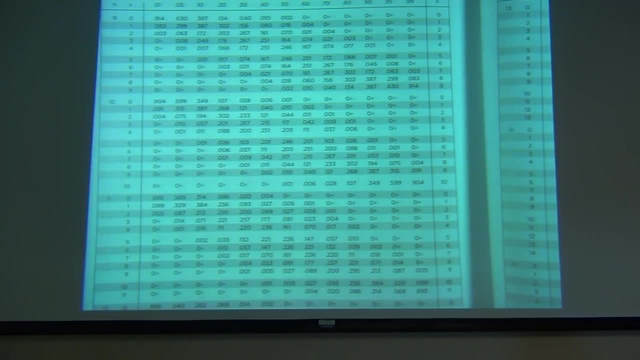 So hopefully you have those written down. If not, we'll do it in like as it was wrong. Yeah, write all those down and add them up. You should get .999.. Okay now, calculator people. there you go. 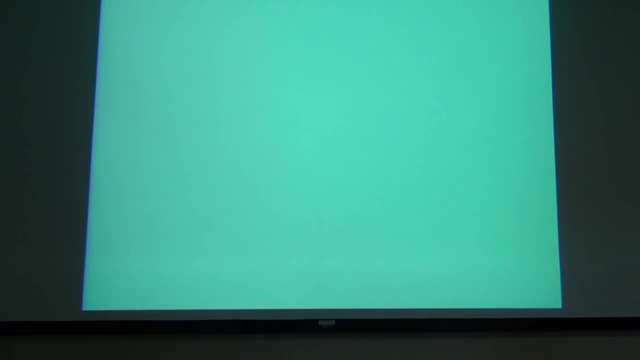 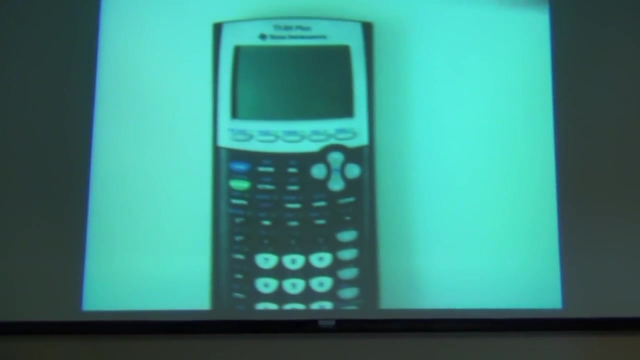 Your scientific calculator will not do this, but this fantastic graphic calculator will. What you're going to do is turn on the calculator. We are dealing with the binomial, what's it called Probability Formula Formula, And it's based on the probability distribution. 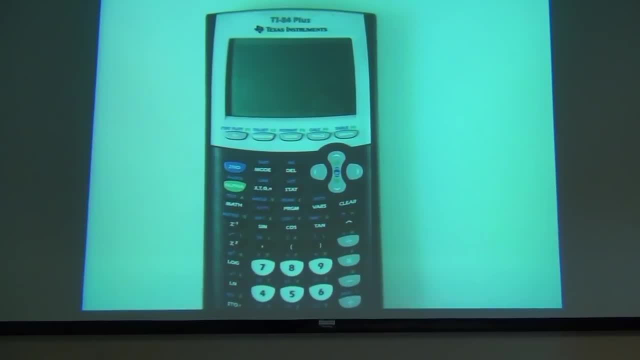 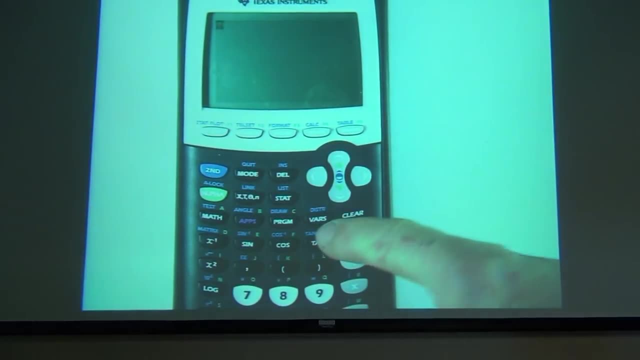 We're under a distribution, so look real careful. You should have a distribution button. It's the dis-ter. We're going to go to the dis-ter. Go to the distributions. right above the variables button. right there It pulls data on the screen. 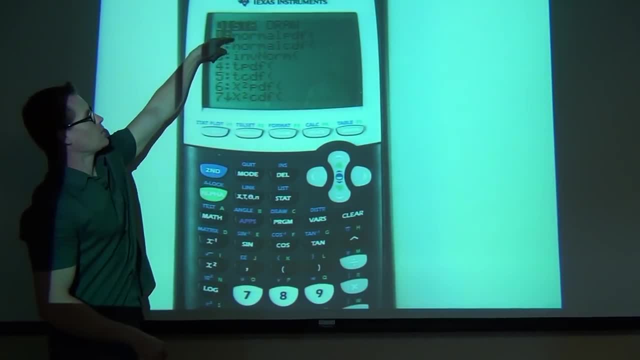 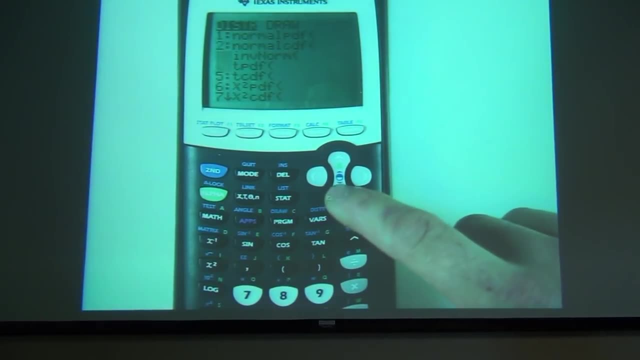 Now, eventually we will actually be dealing with all of this stuff right here, maybe even this stuff, But scroll down a little bit, would you Scroll down a little bit, and you're going to see the numbers 9,- I'm sorry- 10 and 8.. 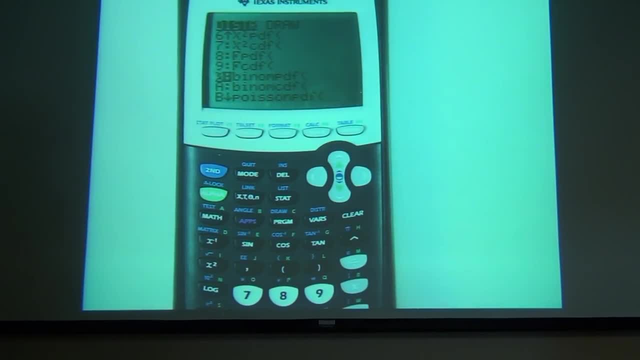 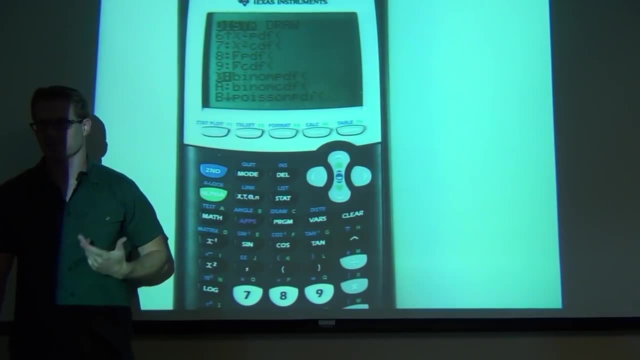 Those say binomial PDF and binomial CDF. Don't go into the poison. You don't want poison, That's poison actually. But don't go to that one, You'll get sick. We're just going to go here. 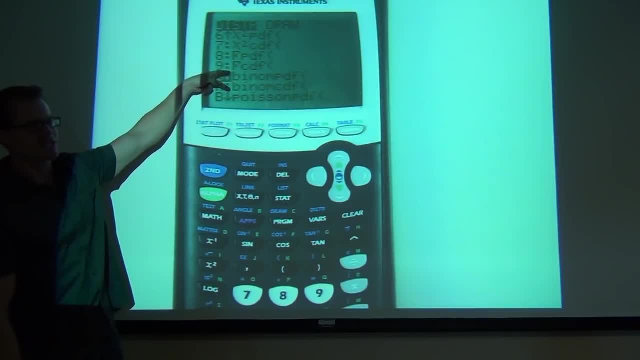 You go to poison, you go too far. Go to binomial PDF and binomial CDF. This is a point. probability, This is a cumulative probability. Here's how this works. Watch carefully If you want to find out an exact value. 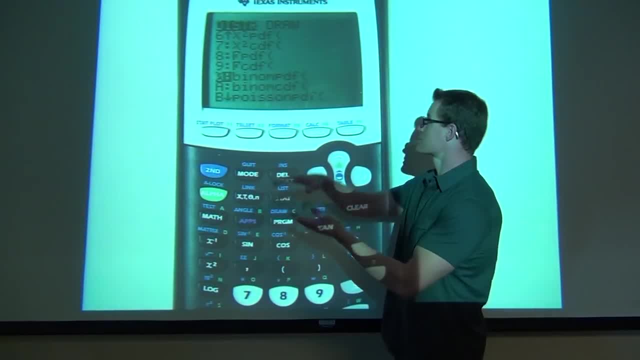 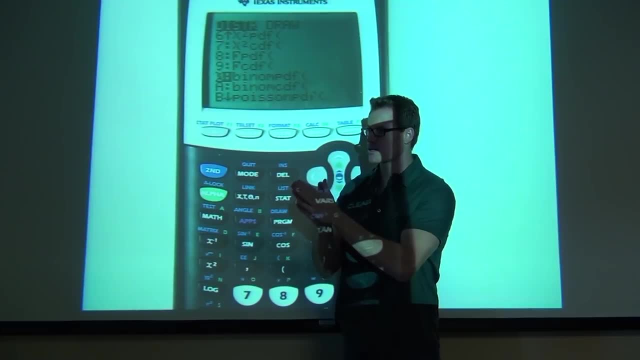 exact number of successes. that's considered a point probability. That's going to be your PDF. This is what's so cool about your calculator If you want to find out up to and including something that's cumulative. So if I want to find at most something that's up to. 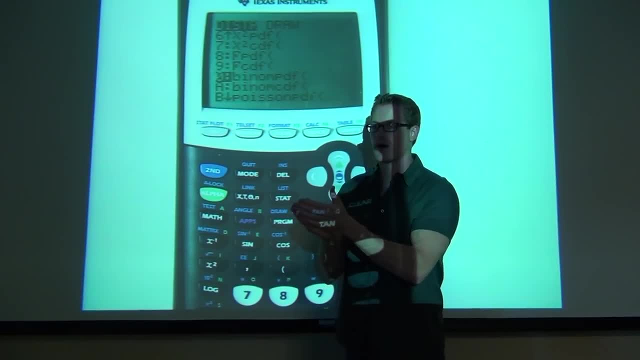 and including 8, you with me on that. If I want to find less than I'd go up to, but not including, So I'd punch it. not 8 here, but 7. One less than that? Does that make sense to you? 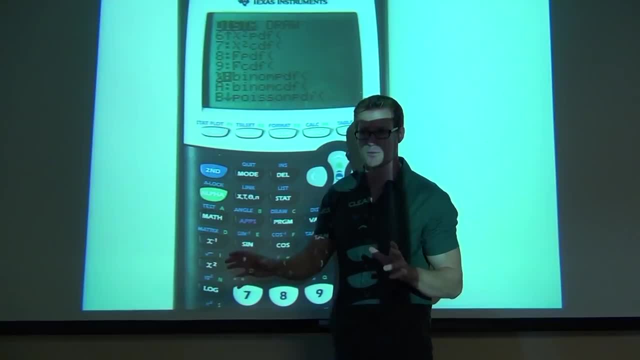 So you've got to be smarter than your calculator is. You've got to punch in the right numbers, But it will do the math for you. Here's how, What you're going to do. let's try the exactly 8 first. 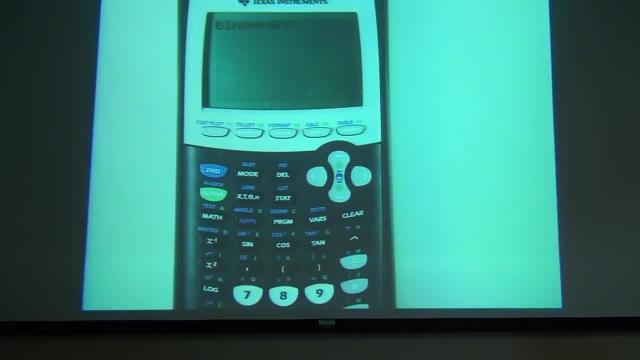 Exactly 8, you're going to punch in the number of trials you have first. So right now the number of trials is how many? Then put a comma, Then put in the probability of success for those trials. In our case it's .30.. 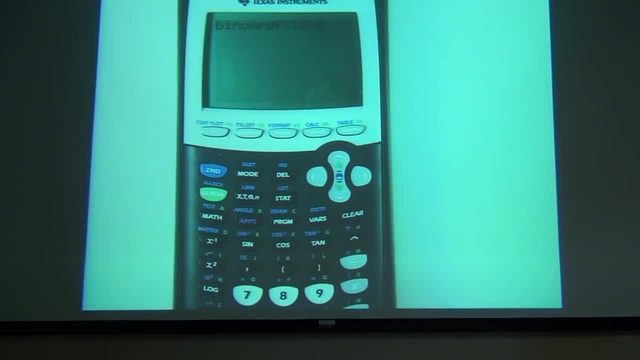 Comma's above the 7. Then you put .30, that's the probability of success, And then you put how many successes you want. So, comma, that's right here, I want how many successes 8. You don't have to even put the end parentheses. 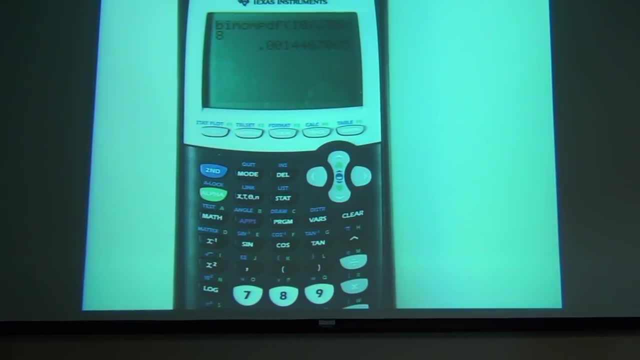 Just press enter .0014467,. that's exactly what we just calculated, with all that work with the formulas. Now, if you want to find up to and including- up to and including- I have to do this kind of quickly, we're running out of time. 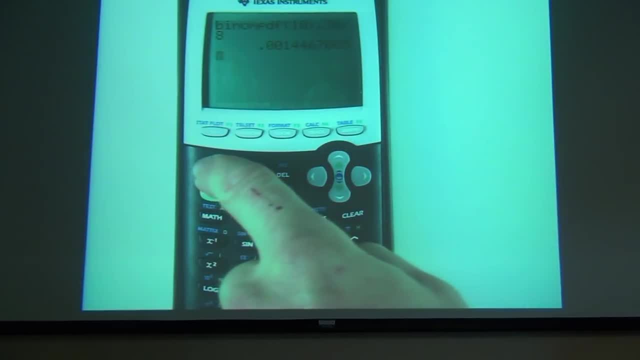 But I'm going to go. you can watch this on the video again. Go to distribution again. Go down to binomial CVF. press enter What this will do. you have the same information, but what this will do, it will add up all the probabilities. 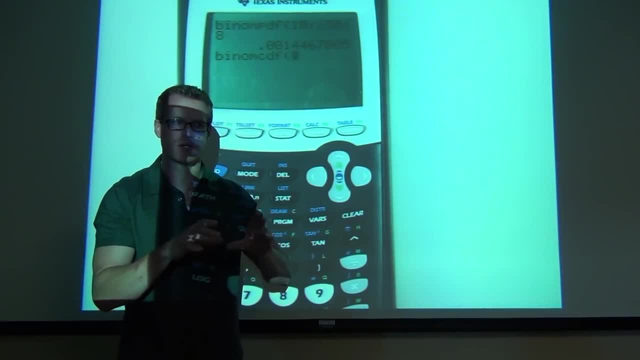 up to a certain number for you and including that number. So you have to be good at knowing whether you're supposed to include that number or not, Because if you put it, it's going to include it. If you want less than something, you go one less. 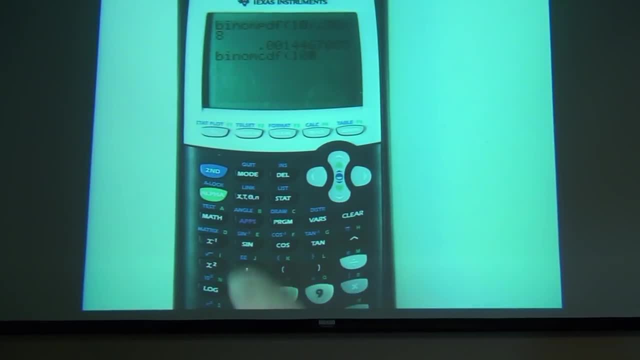 than that number. So we'd go 10 trials, probability of success is still .30.. We want- here's what you're saying here, folks- You're saying: I want up to and including 8 successes, .99985.. That just added everything up to you. 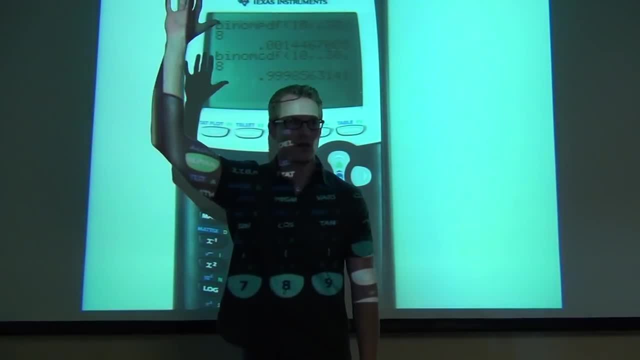 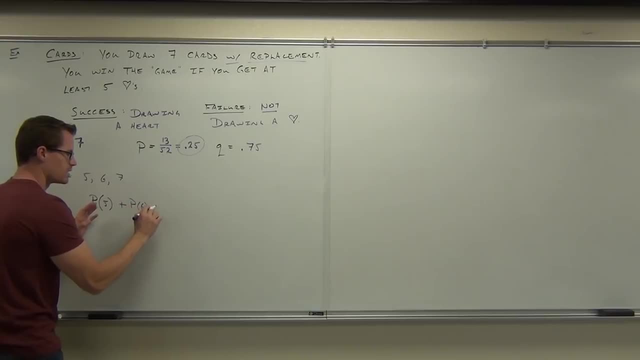 and it's more accurate than your table. How many of you understood that? Okay, watch that video again If you didn't quite catch how to do that on a calculator. this is very, very useful for you. Hearts plus the probability of getting 7 hearts. 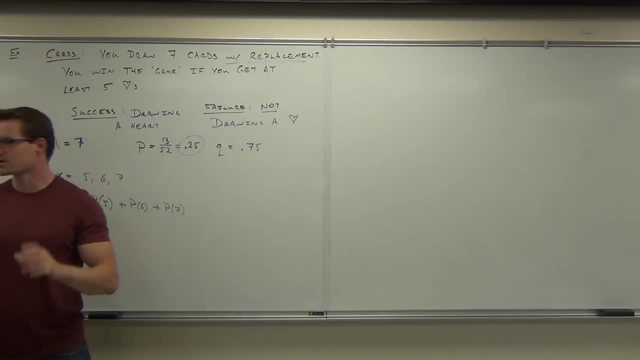 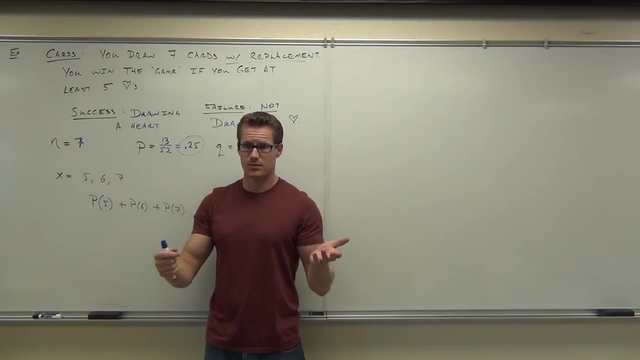 would accomplish my game. If I get 5 hearts, 6 hearts or 7 hearts, I win. true, If I pull out 7 hearts in a row, do I win the game. If I pull out 6 hearts, do I win the game? 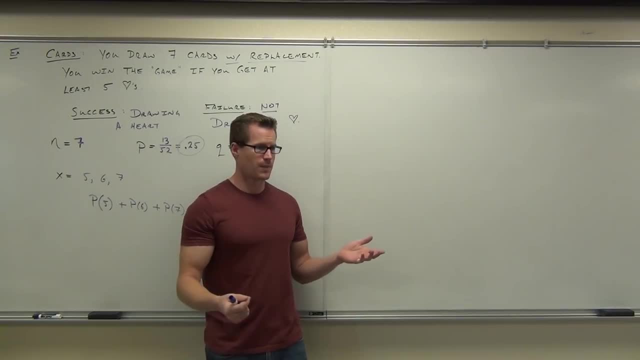 If I pull out 5 hearts, do I win the game? How about 4 hearts? No, I failed the game. So those right there, this right here, this would be the only ways that we can accomplish winning our game. This is the probability of getting at least 5 hearts. 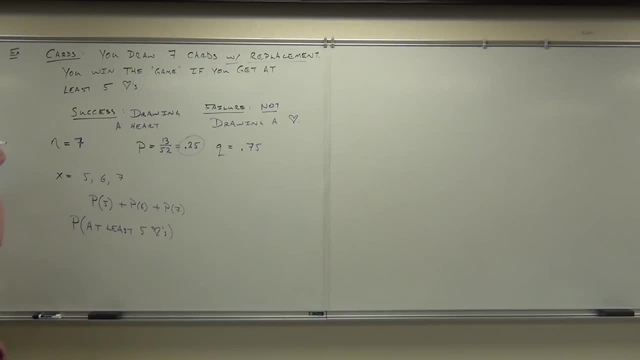 That's the worst art I've ever drawn. I don't even know what that looks like: Kind of like a fish tail actually going in the water, Doesn't it Like a whale tail? Anyway, whatever Art, And last time I showed you a couple ways to go ahead. 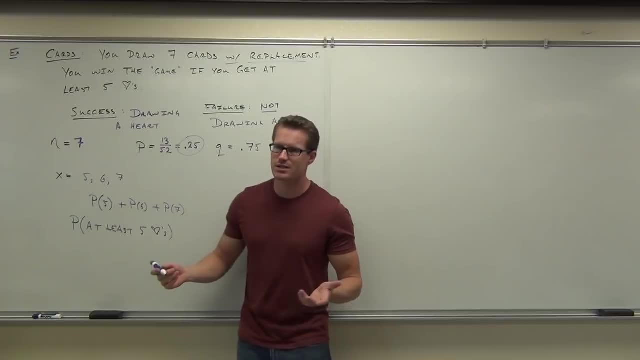 and find this without doing a whole lot of work, because, honestly, you're not going to want to do the formula three times, are you? The formula is kind of horrible. I mean, it's not bad for finding one, but it's kind of horrible to find more than one. 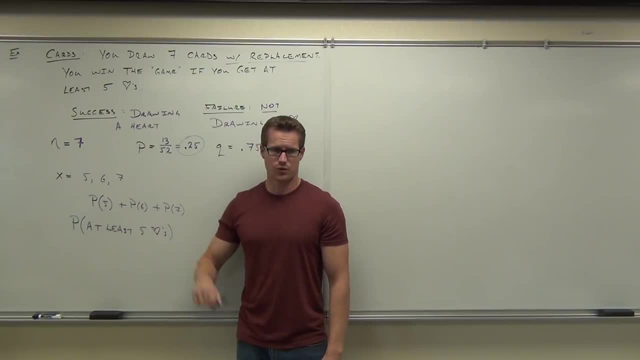 Even one takes a long time. You have a table that works for you. You also have a calculator that works for you. Before we go ahead and do that, we'll show you how to find all those things. I want to determine a couple other ideas. 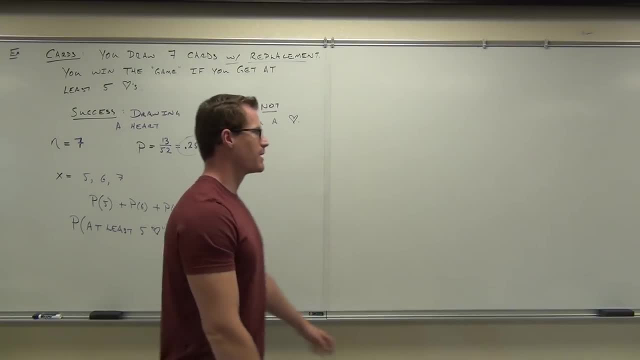 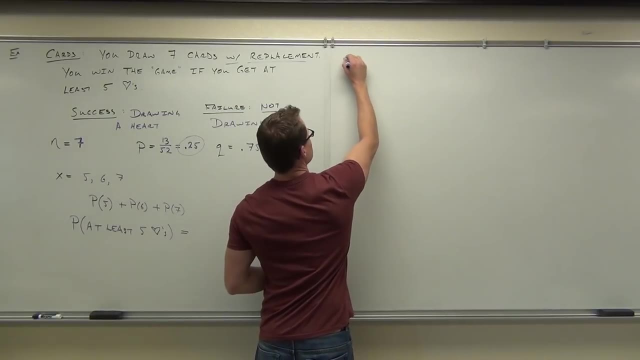 We're going to change our game a little bit. OK, Firstly, let's say that this is our first game. We're going to figure this out. We're going to figure this out in just a bit. Let's say that the next game is: you win the game if you get. 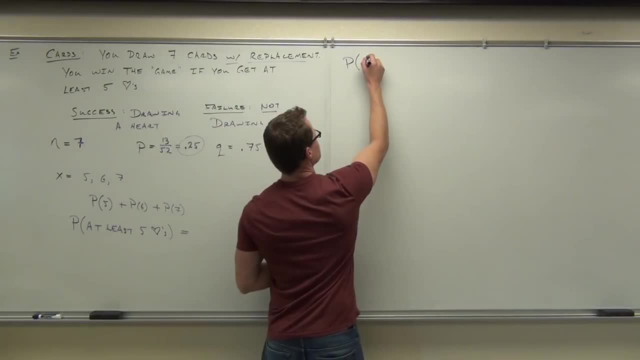 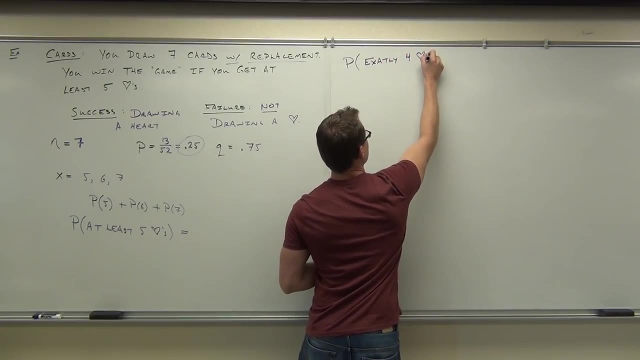 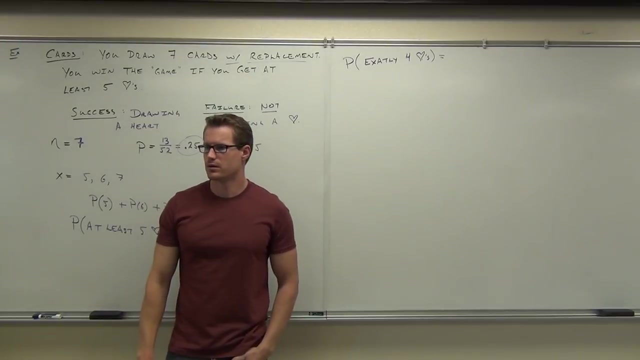 exactly four hearts, Exactly four hearts. How many successes are we looking for there? How many successes, if I'm getting four hearts, One, One success? How many hearts am I? Success is a heart right. How many hearts am I looking for? 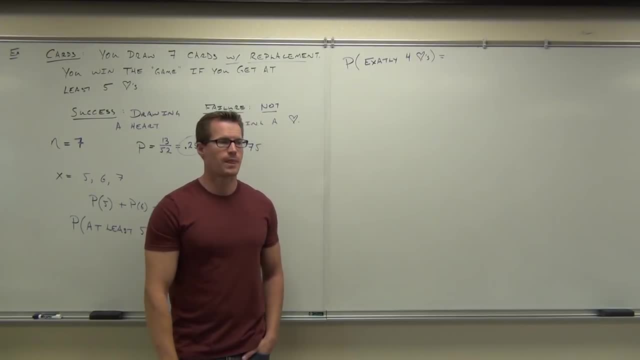 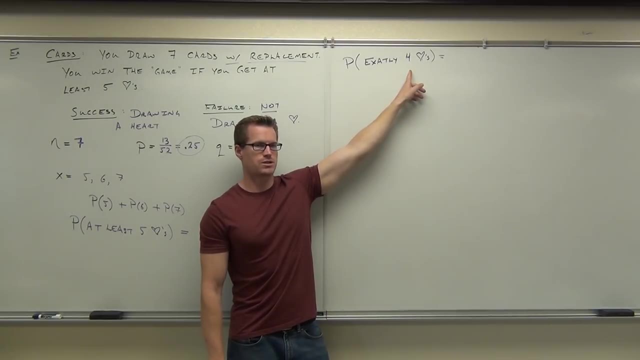 Four, There'll be four successes. Hey, tell me something. Would five hearts work for this? You'd lose. Would three hearts work for this? You'd lose. OK, so in this situation, you would have to draw exactly four. 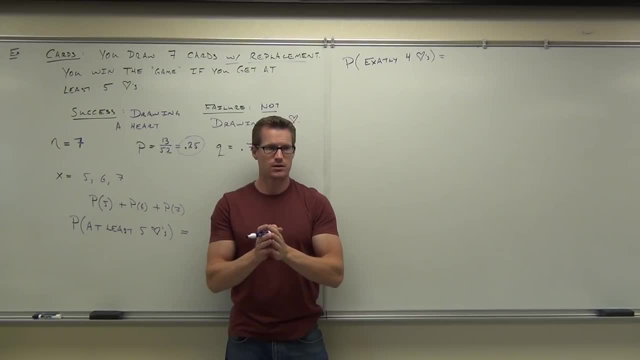 no more, no less. Is that hard to do? do you think It'd have to be like one of these combinations: No heart, no heart. Yes heart, Yes, heart, no heart, Yes heart, Yes, heart, no heart. 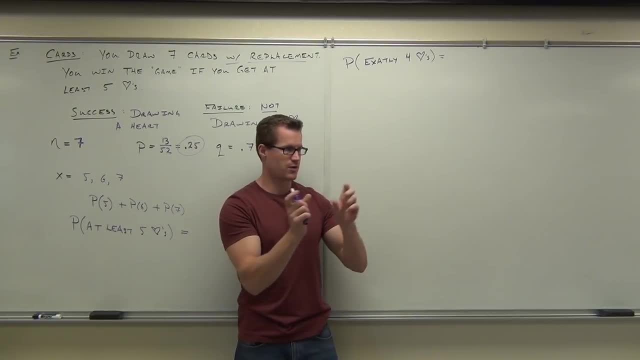 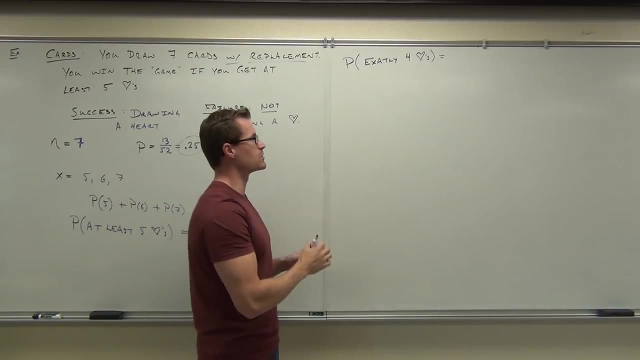 That'd be one combination. That's hard to do right. Every combination would have to have only four hearts in it and everything else would have to be a different sum. So that's one more game. I want to do this. What's the probability? 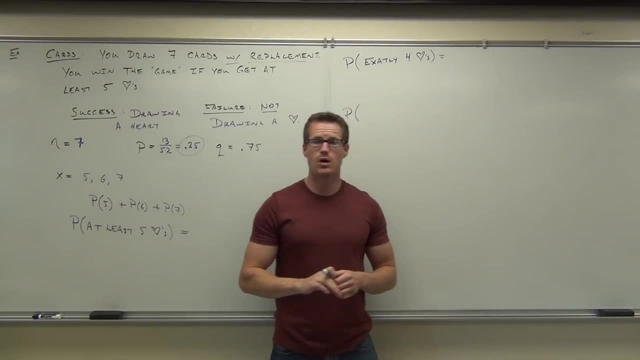 Let's say: this is our game. now. Our game is: you can have at most three hearts, At most three. So let's see how that game would work out. If you drew a card at most three, Could you draw no hearts? 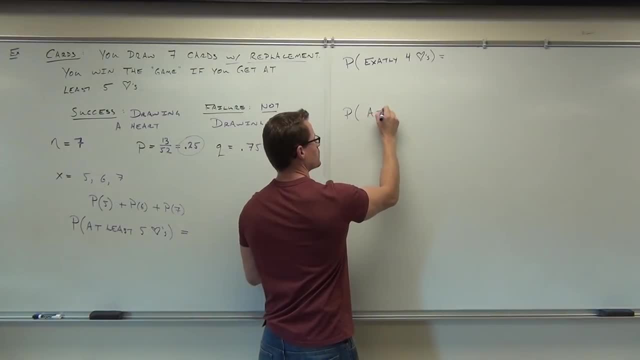 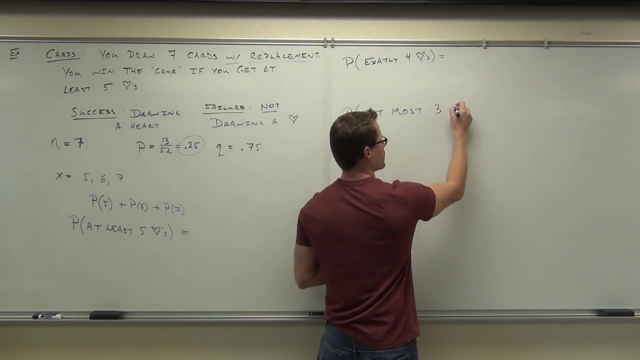 How would you win that game if you could get at most? Think about this as I'm writing it down: How would you win this game if you only could win if you got at most three hearts, No hearts, one heart, No hearts would work. 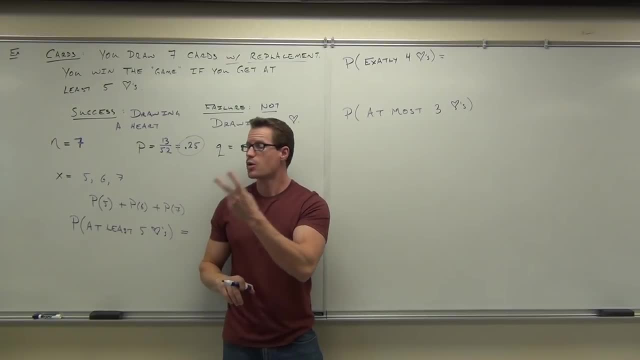 Sure, what else would work? One heart, One heart, two hearts? Would three hearts work? Yes, That's, at most three. How about four hearts? Five, Six, Seven? How about eight? Would you even consider eight? No, because it's outside of our range. 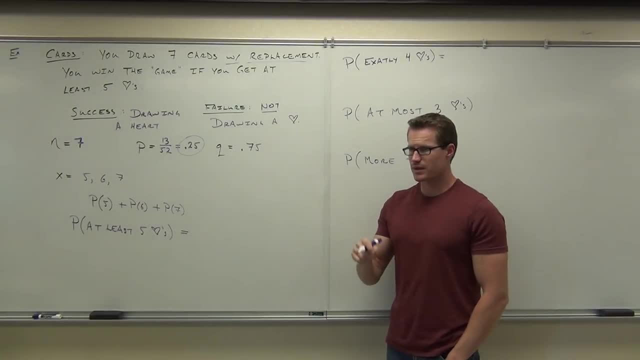 How about this? You have to win the game. In order to win the game, you have to have more than five hearts. Five, Five. I'm already using five. Let's say you have to have more than two hearts. In order to win the game, you have to have more than two. 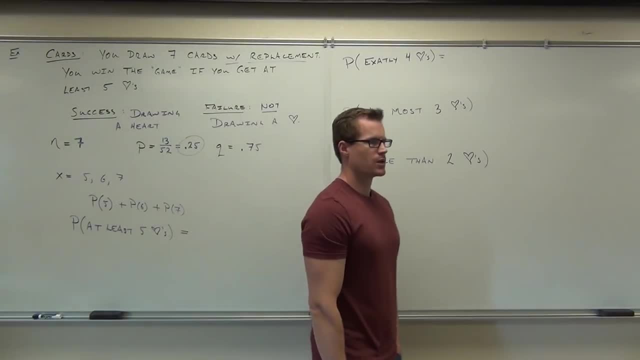 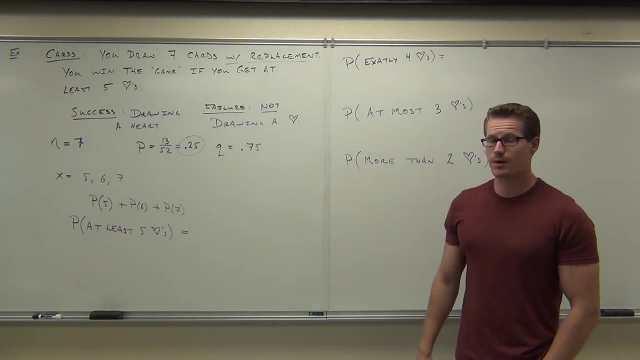 hearts. Give me the scenarios for winning this game. More than two hearts, Give me the scenarios for winning Three. Three, okay, How about two? No, Why not two? You need more than two, More than two, More than two. 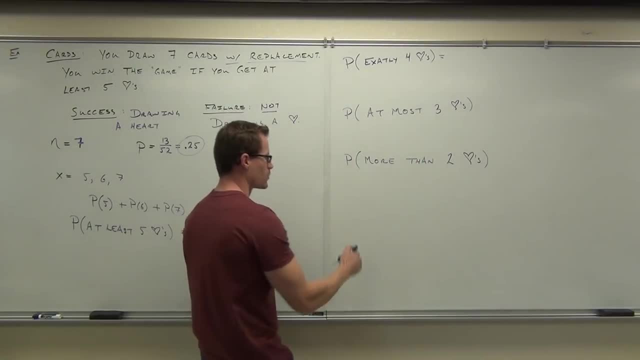 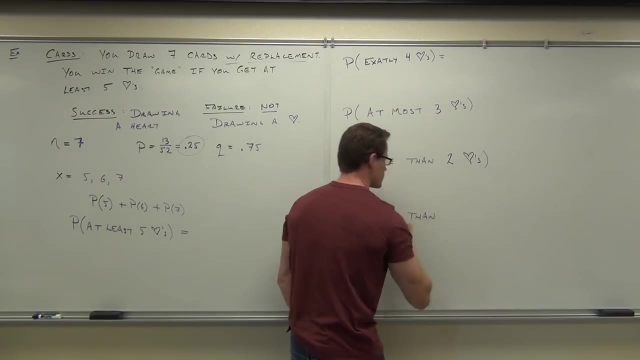 So three, four, five, six, seven. Okay, One more. In order to win the game, you need less than six. You need less than six hearts. Oh, that's one of the better ones I've ever drawn. That's pretty good. 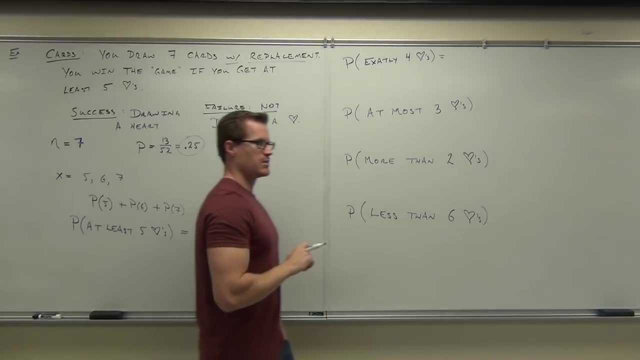 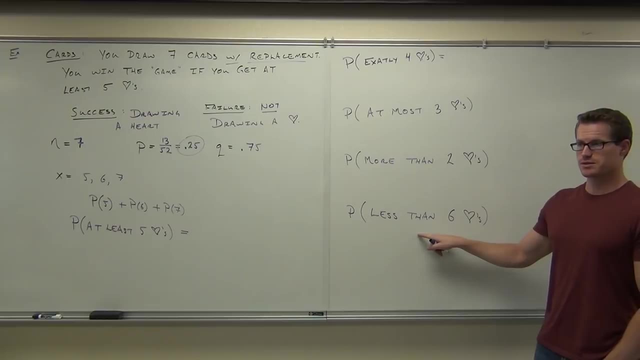 Five, Less than six hearts. Remember, in order to win the game, you need less than six hearts. So let's look at that. What wins for less than six hearts? Zero, Zero wins. That's less than six. One, two, three, four, five, six. 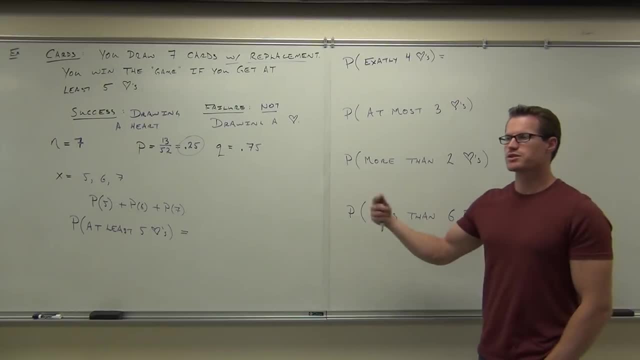 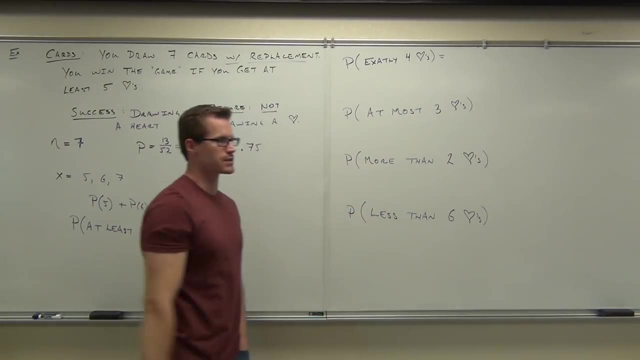 No, No, that's not less than six. These are most of the scenarios you're going to see. Most things we see are at least exactly, at most more than less than Those are the scenarios. So now we have one, two, three, four. 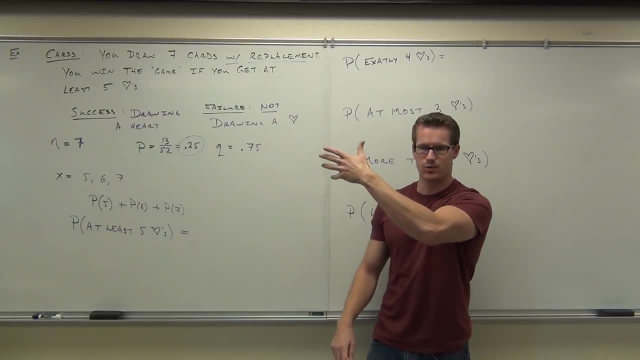 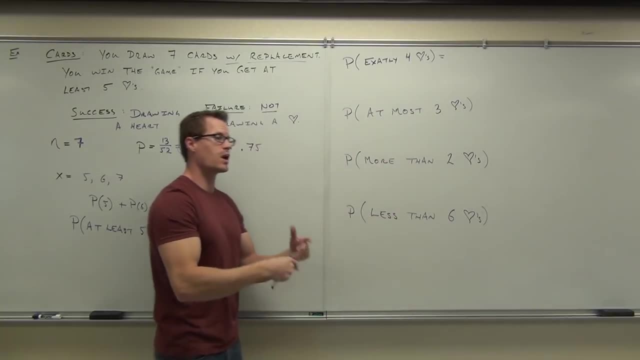 We have five games we're going to play with this one example. okay, So I have your cards. We're drawing one, Put it back. Drawing one, Put it back. Drawing one, Put it back. We're going to do that seven times. 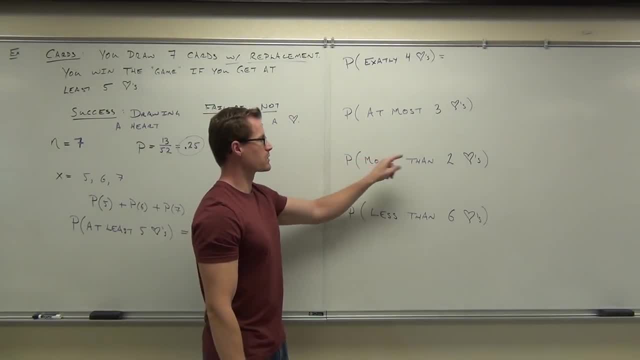 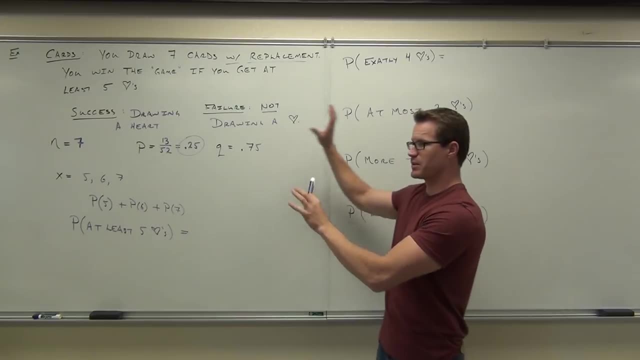 What I want to do is find the probability of getting at least five hearts, then exactly four at most. three more than two less than six. Are all the probabilities going to be the same? No, You're way off. You're going to be in completely different probabilities. 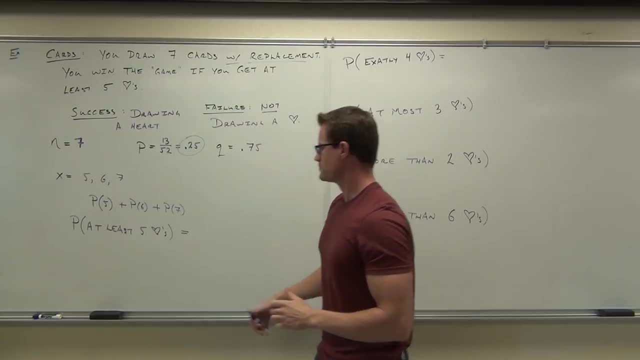 So the chances of winning are going to be different for every single game that we play. I'm going to show this to you on the table. We're also going to do this on the calculator. Do you see? a couple of ways of doing that? 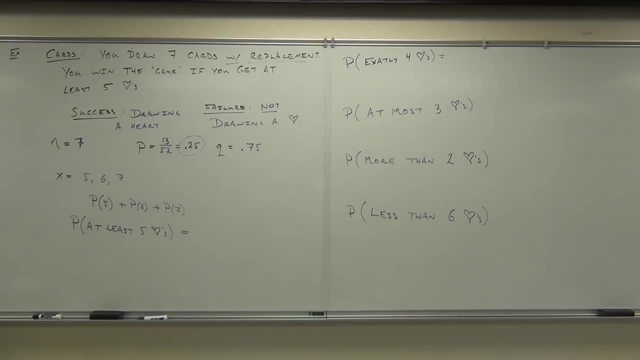 Did you guys bring your tables today? You should probably bring them, so you know we'll be doing this from time to time on your tables. 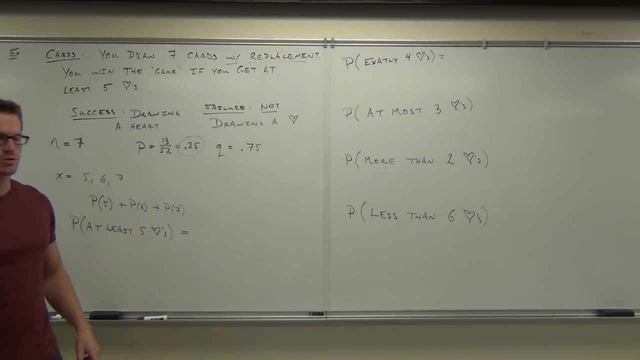 For now, we'll look at the table that I have up here in just a bit. Also, do you have your calculators? Yeah, I'll give you this table, the appropriate table, for your test, when the time comes to it. 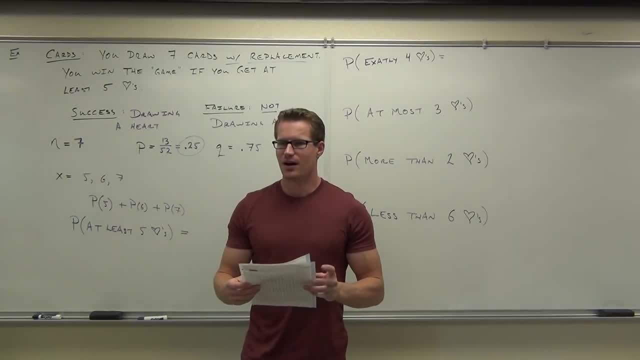 so that you have at least the information there. So I can't say like, yeah, memorize this whole thing, Ha ha, ha, ha ha. Okay, that would take your life. You don't want to do that. 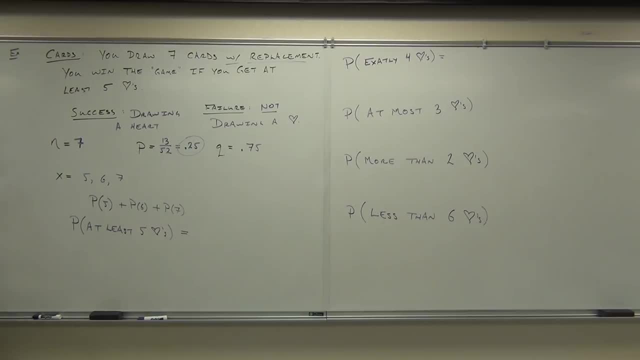 So let's look at the probability of finding at least five hearts. You have to memorize those, by the way, or have these written down, because we're going to do this on the board. well, the white screen, Actually, can you see it when it comes up? 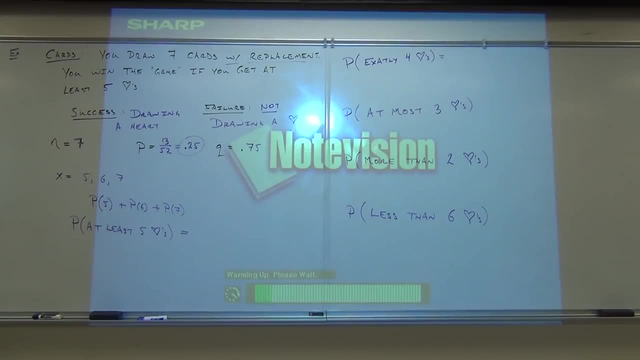 Probably not. Okay, Do you remember how to use this table? What is this column for? And so, in our case, in our game, what N are we using? So we're going to be down here. It's below our screen right now, but I'm going to move this up. 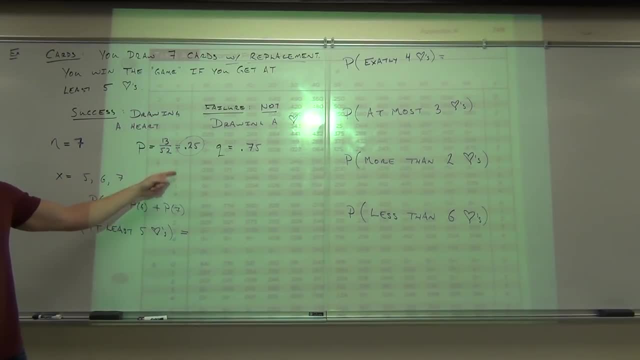 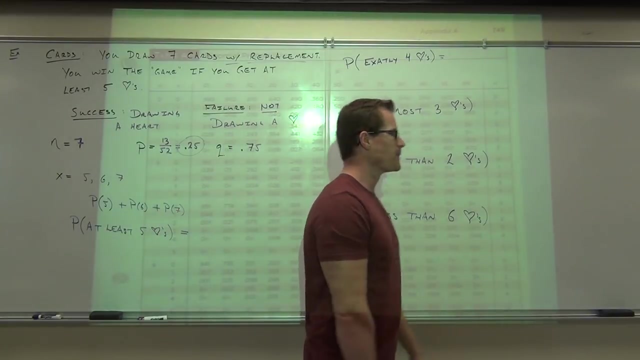 What's the X stand for? Number of what now Successes? Yes, successes. This is how much successes. What's this stand for Probability for each success. Notice how that has to be based on success by success, trial or trial by trial basis. 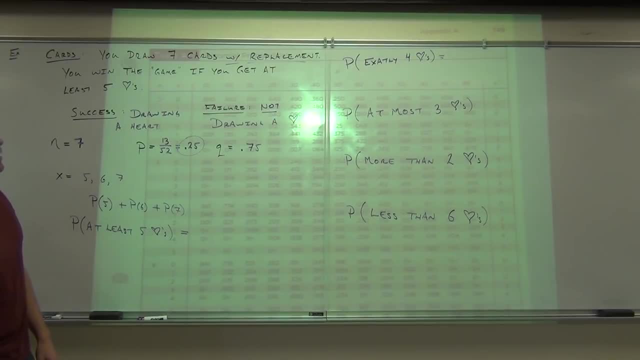 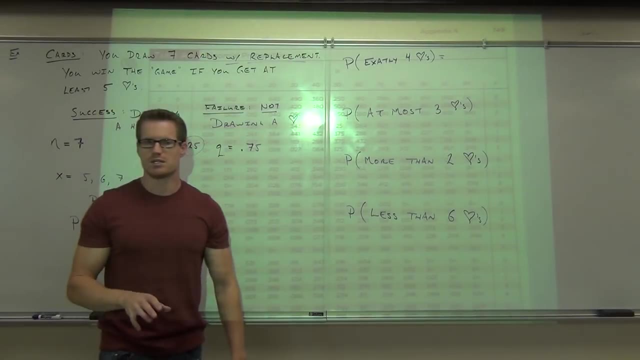 So what is our probability here? Whoa, wait a second. What are we going to do with that? It's right in the middle of that. This table isn't going to work exactly perfect for us. in this case, You're going to have to use your calculator, use the formula. 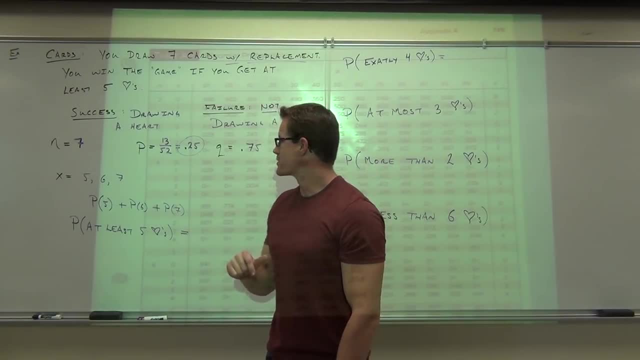 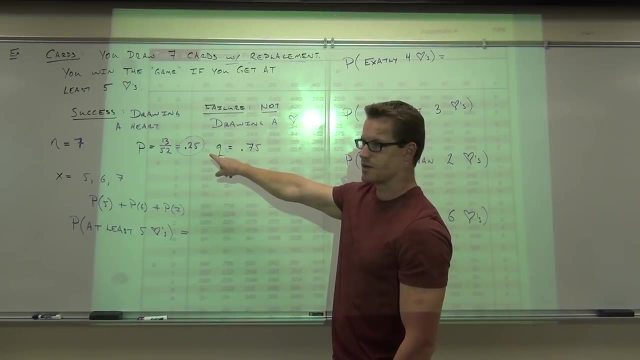 or you're going to have to guesstimate there, which is not going to be the best for us. So just to make this a little bit better, can I fudge that for a second? So you can use that. I'm going to fudge it for a second. 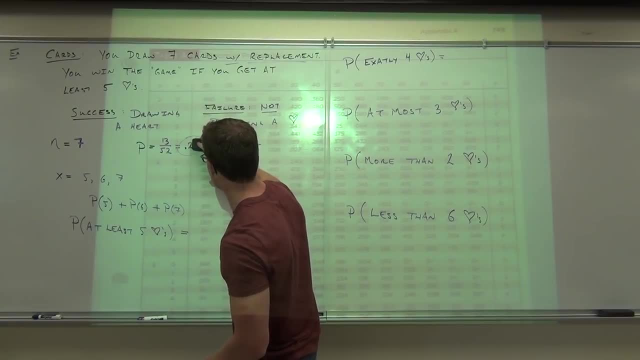 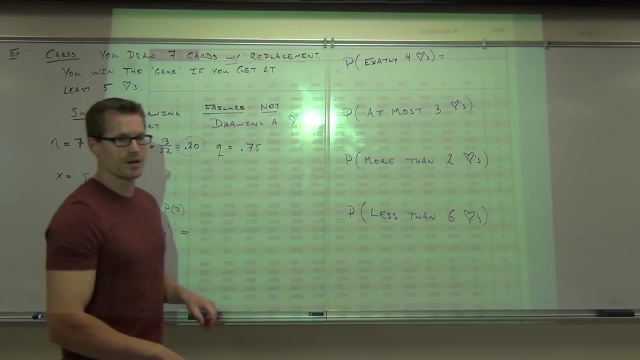 So our probability is going to be a little inaccurate. Let's say that we have .20.. So I'm lying here. Yes, I know I'm lying, but I want you to be able to use that table and get some appropriate answers out of that. 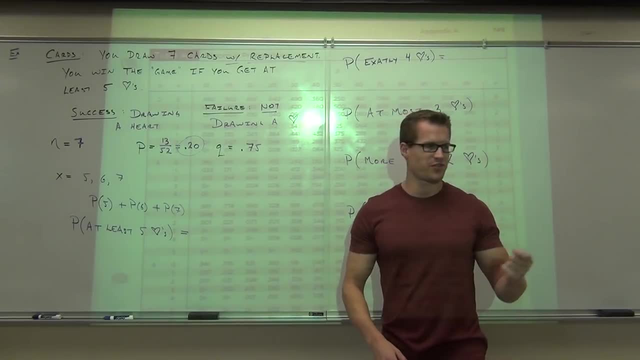 Your calculator, by the way, will use the .25 just fine, with no problems whatsoever. The table obviously has some drawbacks to it. We can do the 1,, the 5,, the 10 percent, the 20 percent, but then it goes up every 10 percent. 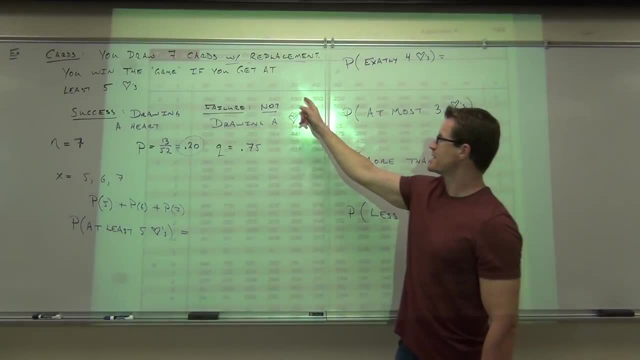 and we're done. So we're going to have to use the formula for that until you get to the 95 and 99.. So this range we'd have to go right in between those, just guesstimate between our .2 and our .3.. 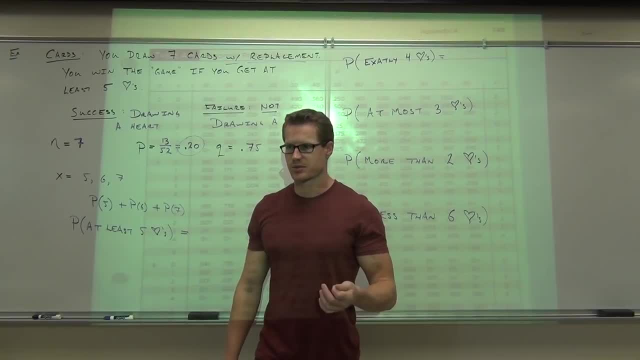 It wouldn't be the best case for us. Are you guys with me on that? So all you can expect on your test, on your homework, they might give you some of that. On the test, you can expect that one of your probabilities will be in one of these columns. 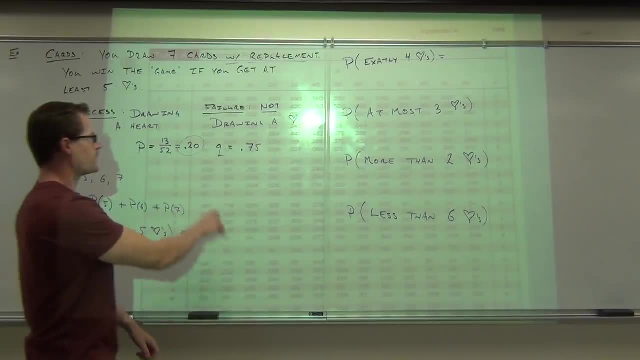 Okey-dokey, Okey-dokey. So we're going to fudge this a little bit. I know this is not accurate, but we're going to say it's .20.. Let's find the probability of at least 5 parts. 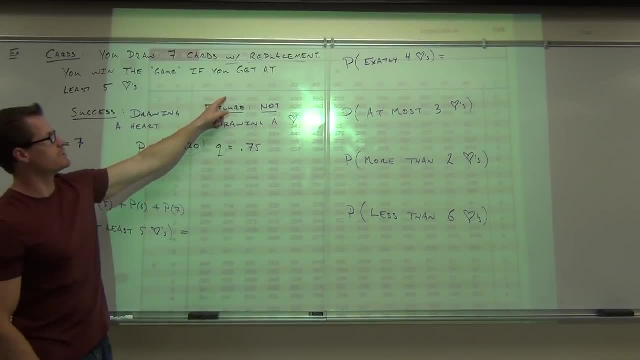 If we do at least 5 parts notice, we're going to be in the 1,, 2, 3.. We're going to be in the 4th column the whole time. Are you with me on this 4th column? let's move it on down. 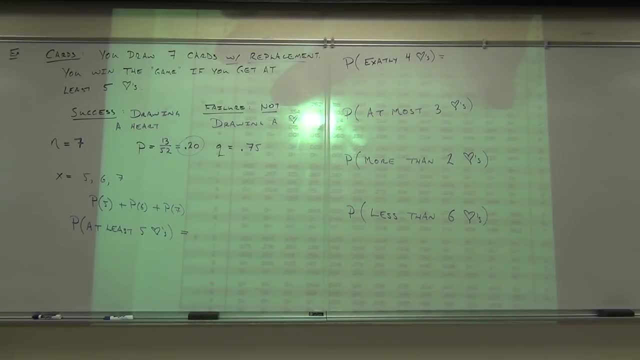 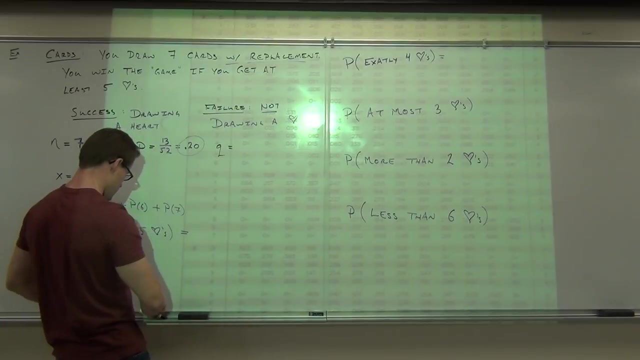 Don't you have to change the Q since you changed the probability? Yeah, of course I do. Fortunately for us, the Q is really not on this table. So if I did, then, yeah, that would be a .80, now .80.. 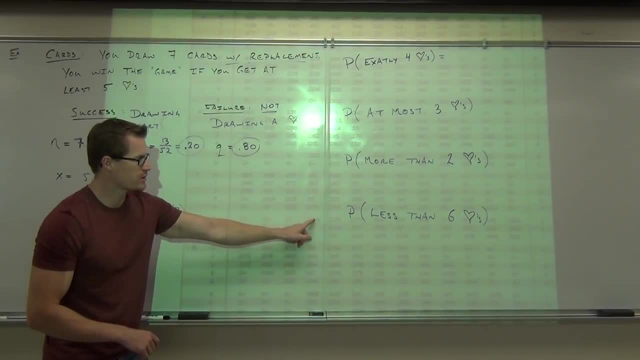 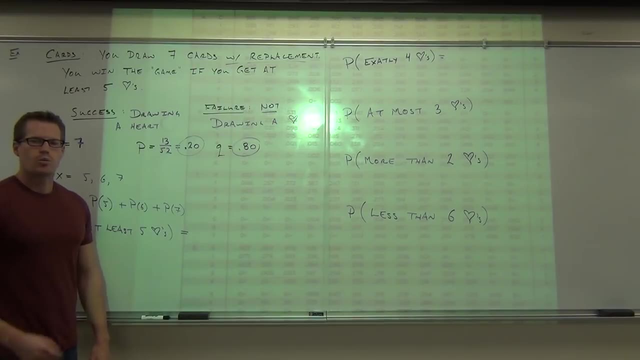 So let's check that out. I've moved it so that this is our 4th column. We know that this is a .20.. What we're looking for is, right here, the probability of at least 5 parts happening. What accomplished the probability of 5 parts? 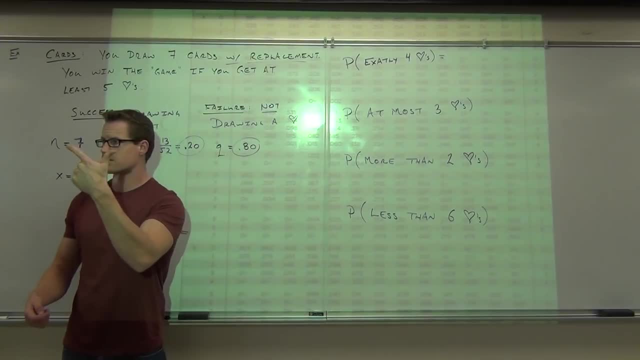 We already went through this. We could get 5,, 6, or 7,. true, 5,, 6, or 7, those three situations. Let's look at that. Here's 5 parts. This is the probability of exactly 5 parts coming out of this situation. 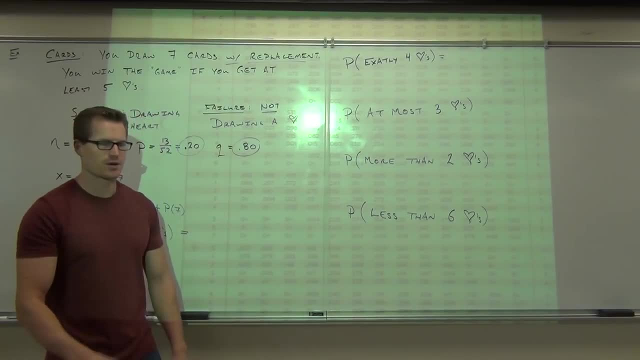 Here's 6 parts and here's 7 parts. So if we added all that together, remember we treat this as pretty much a 0.. This is less than .001, so this is going to be how much altogether? .001.. 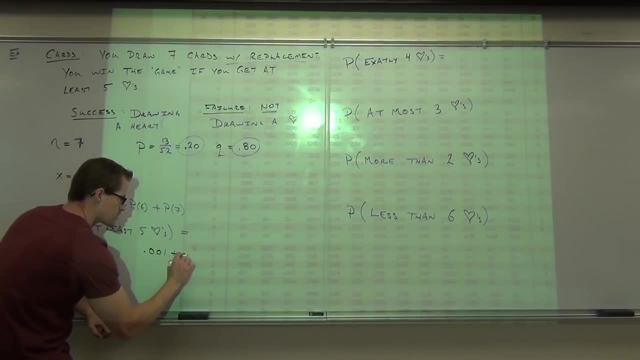 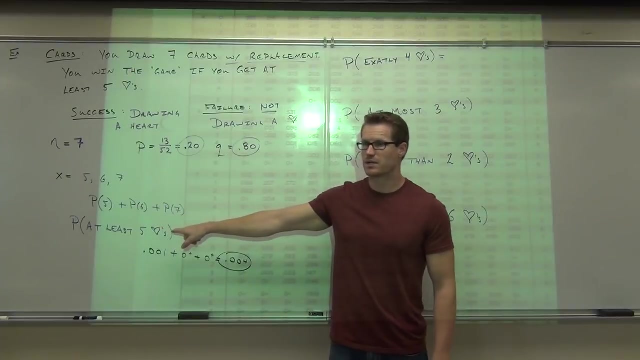 How you'd show that. you'd say .001 plus 0, plus You're going to get .004.. So the probability that you're going to win my game: is it good or not for this particular one getting at least 5 parts? 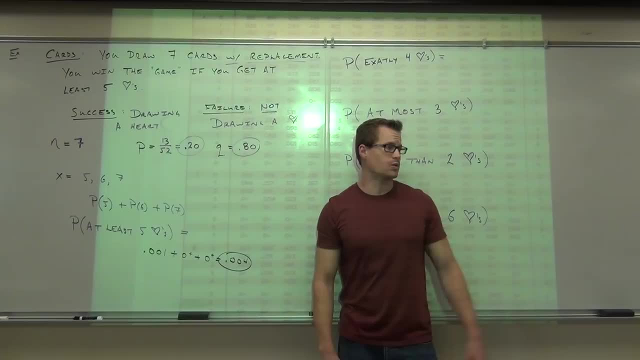 Is that good? Why is it unusual? It doesn't fall under .05.. Yeah, It's not above .05, so it's less than or equal to .05, so that would be very unusual to win this game. Why would it be .001?? 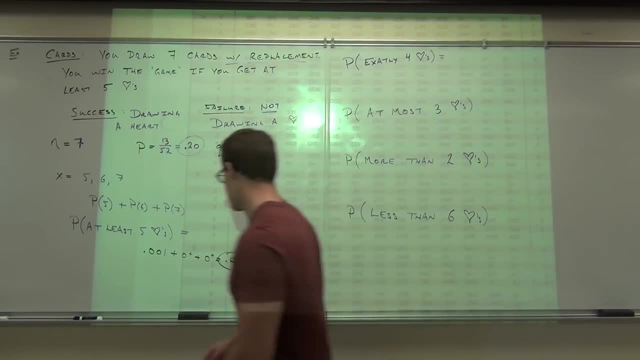 What did I say? Oh, I don't know. I made a mistake. It doesn't happen often does it, But it does happen. Just kidding folks, I made a mistake. I did the .01.. I should have been .04.. 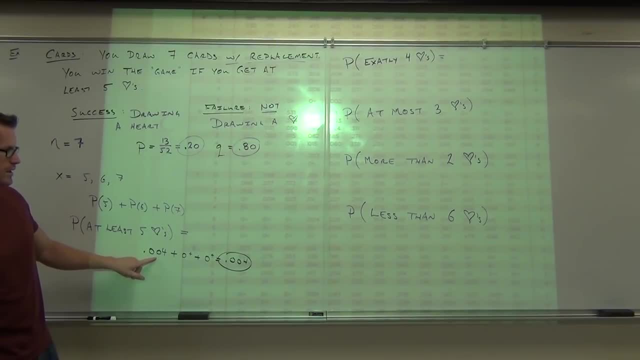 Yeah, .004 plus 0 plus 0 is .004.. So the probability is still not very good. I mean, we needed this to be a 5 right there. This is way less than that. So this is an unusual, unusual win. 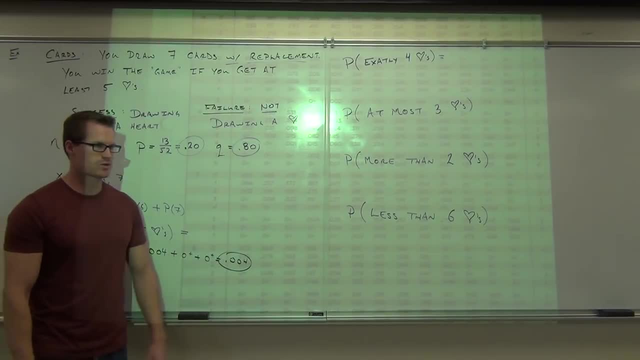 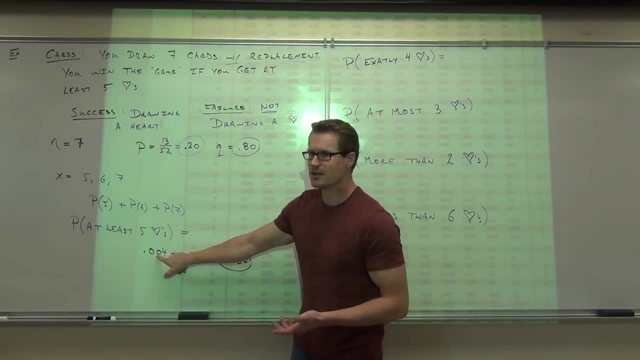 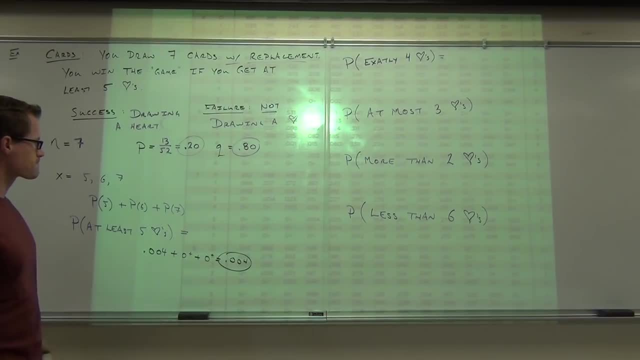 We did it And we're OK with that so far. OK, good, Let's find the probability of getting exactly 4 hearts, Exactly 4 hearts. So let's look at that: Exactly 4.. So I see 4 right here. 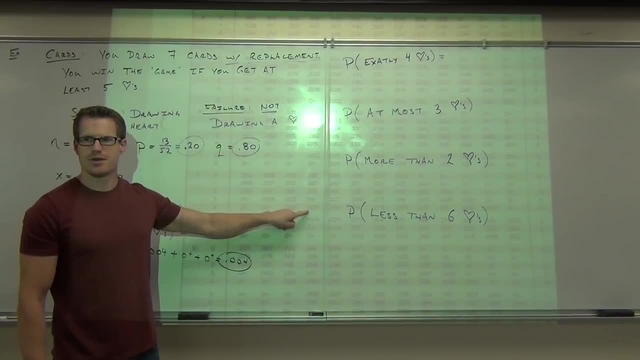 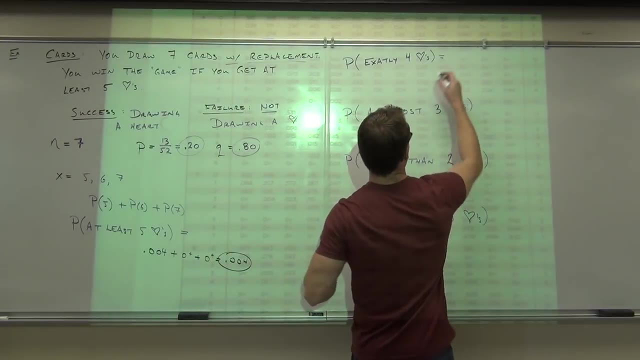 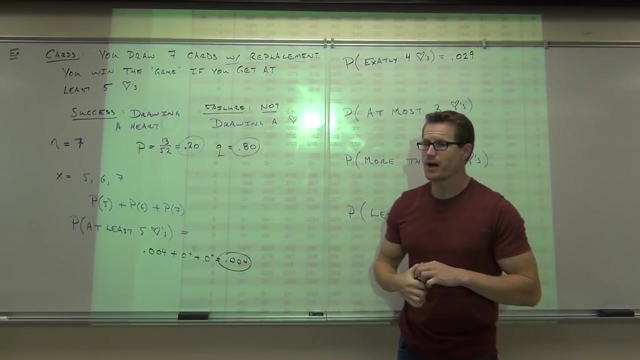 I know I'm in this column. Do I need to add anything on to this number? if I'm looking for exactly 4 hearts, So this is .029.. Which game would you rather play? .004.. Getting at least five hearts or getting exactly four hearts? 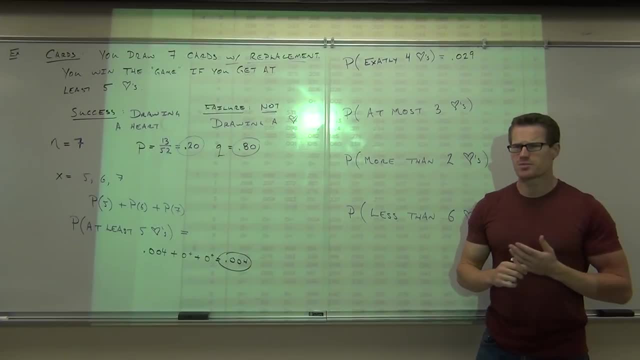 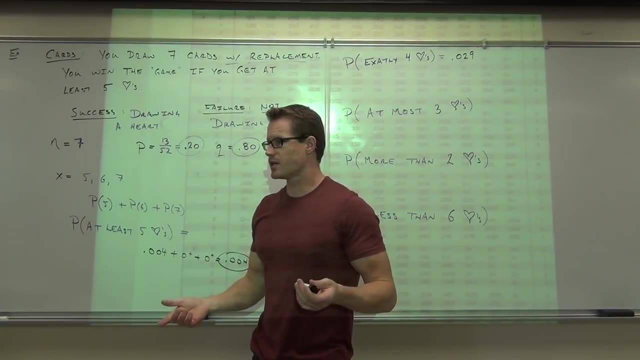 So if you get to choose between those games, you'd probably say I'd rather play the getting exactly four hearts, Even though the probability still sucks of you winning. it's still unusual, isn't it? Less than 5%, Still unusual. 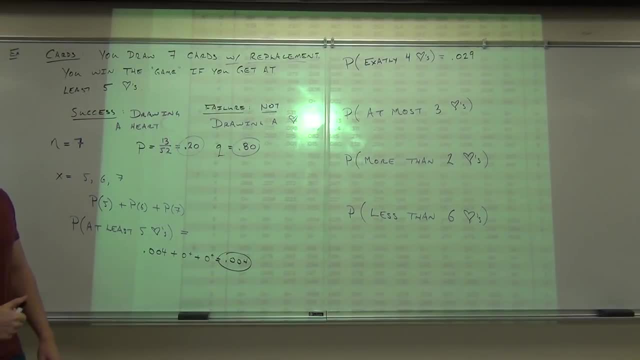 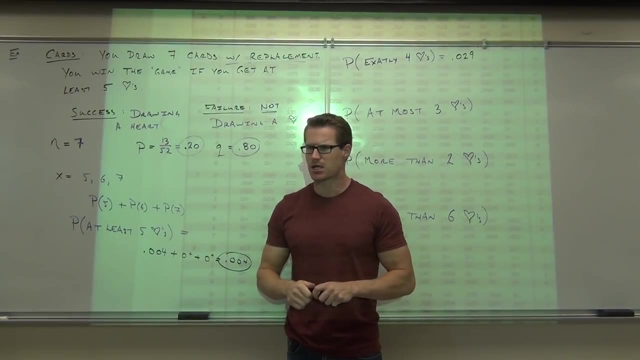 It's better than this game. Let's look at at most three hearts. At most three hearts. If you had at most three- we already said that was what was it most three again: Zero, Zero would work. 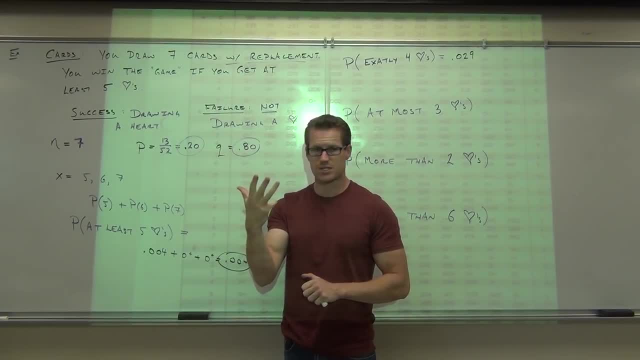 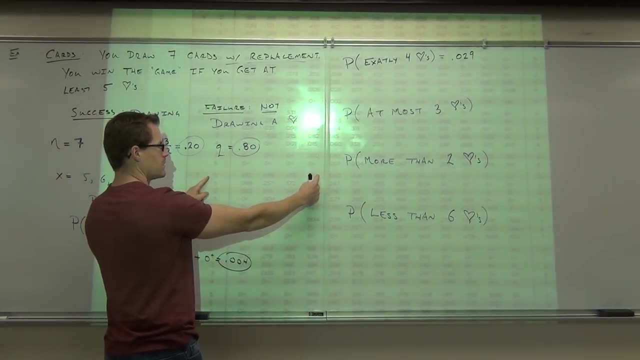 What else would work? One, Three is included in that, At most three. So we'd go back over to our column. We'd go: okay, zero hearts works. Okay, One heart works. Two hearts work All the way to three. 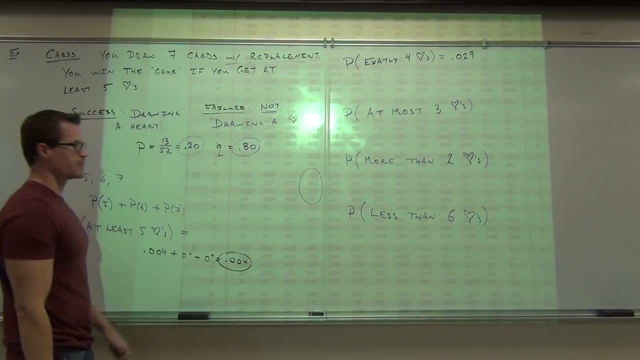 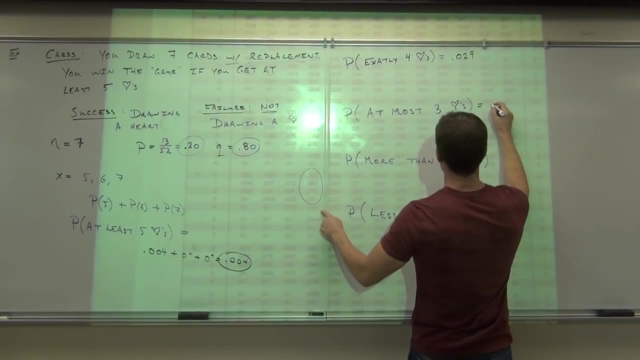 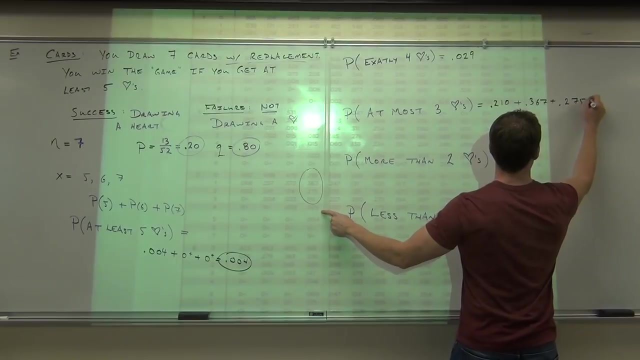 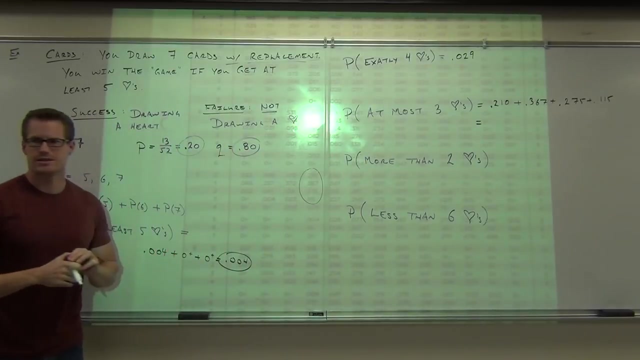 So we're looking at those four numbers right there, Zero, one, two or three inclusive. So we're going to add all those things up, So .210, .368.. .27, .275, .115.. Can someone add those for me and tell me what you get out of that? 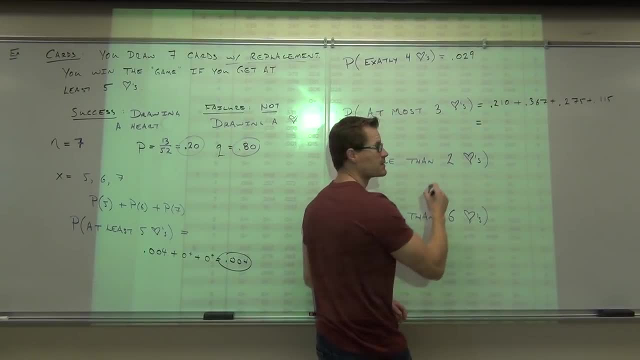 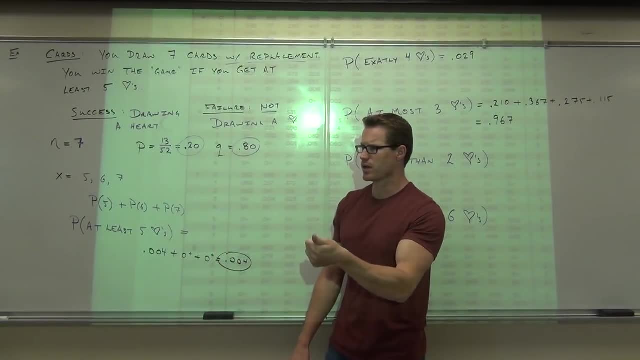 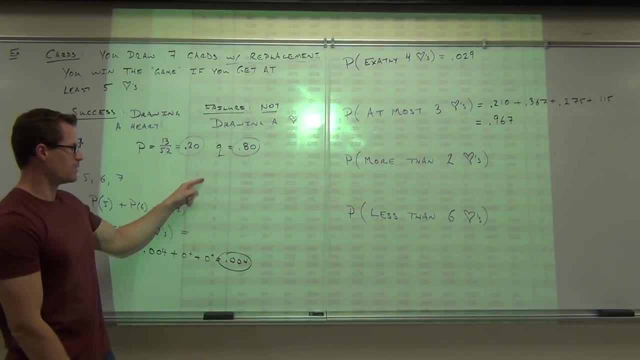 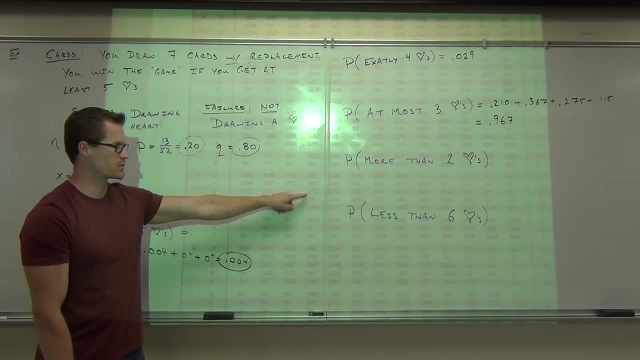 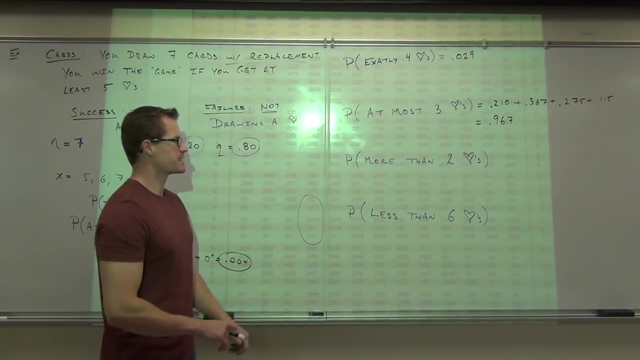 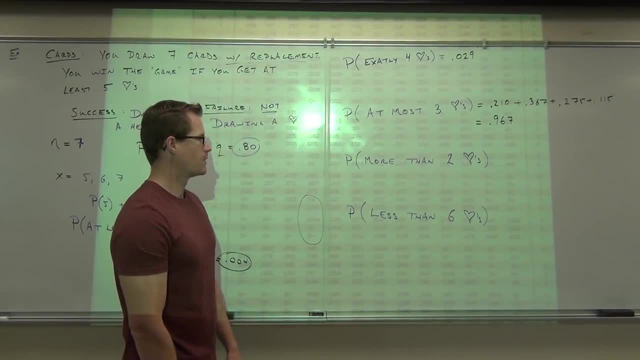 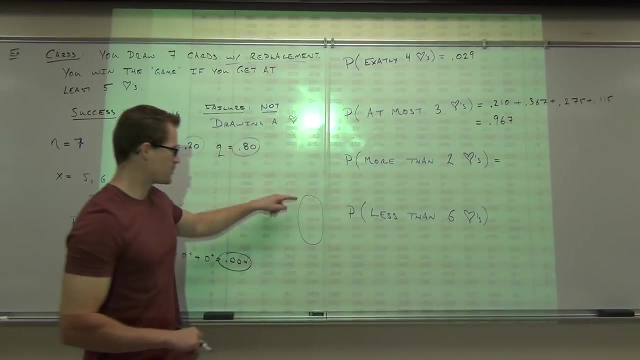 Are you guys getting that? Yeah, Yeah, Also, the same as at least 3.. So add up that column, We do the .115, .029,, .04, and then these are considered 0.. How much is that? .148.. 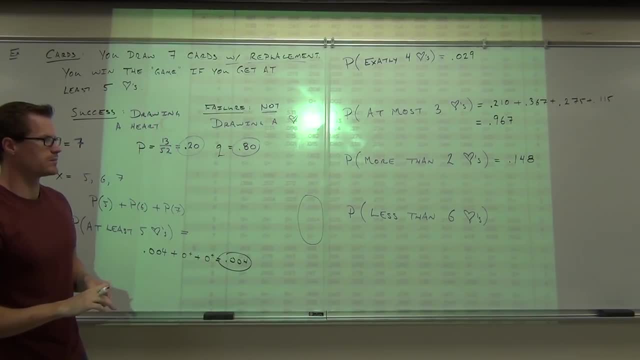 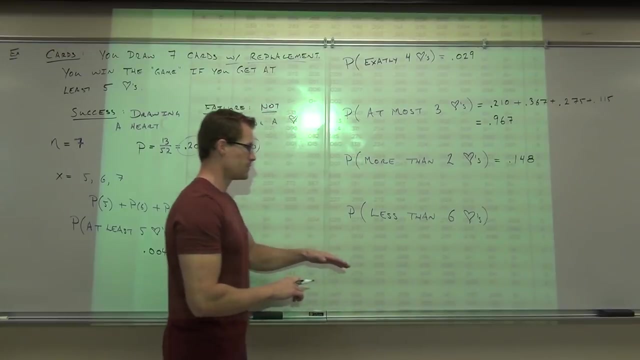 .148.. .148, so we add them. how about the less than 6 hearts? less than 6 hearts: here, What counts as less than 6 hearts? 5.. So 6 is not included, so we'd have to do 5 or less. 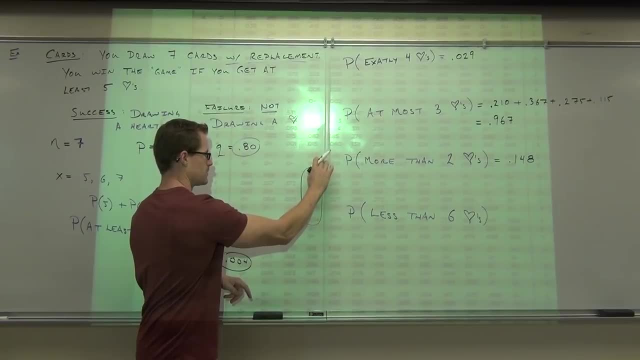 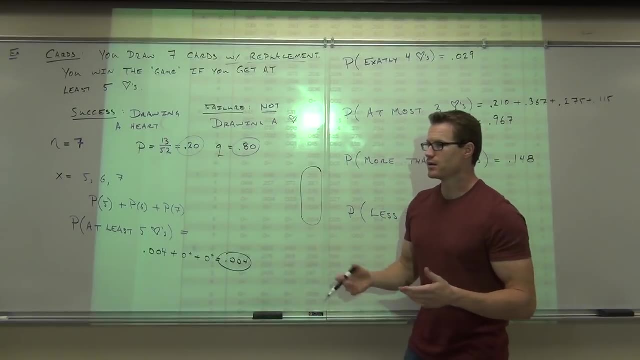 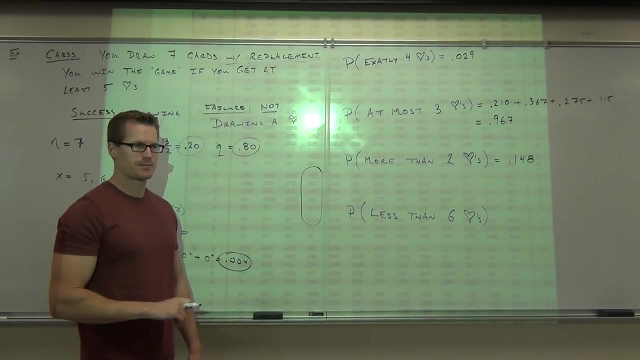 Oops, not that much. So less than 6 is 5 or less, or at most 5, it's the same thing. If you add all that up, how much are you going to get? How much are you going to get there? 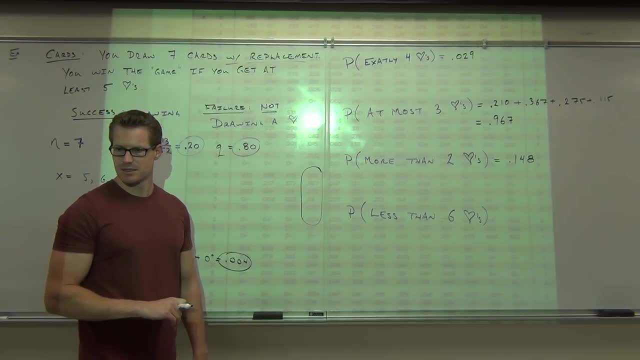 It should be pretty close to 100%, like .999,. how much One? One, exactly one, No, Okay. so this is a little bit off because this cannot be 1, but it will round to 1.. There is some probability here, so I'm not going to put 1 for you. 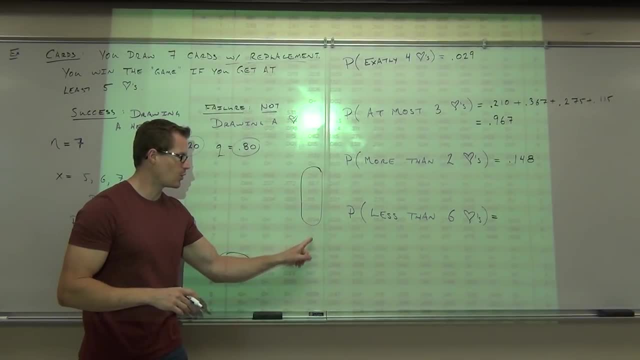 If you ever get this case and you add up- and you haven't added the whole column, here's what you know about this- The whole column will equal 1.. There's 1.. There's a 100% probability you're going to land in one of these cases. 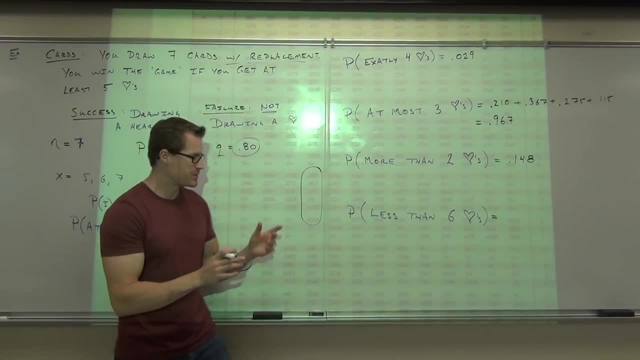 However, there is some probability here. it's just rounded. In this particular case, these round in such a way that when you add them up, you get 1.00, right. So if you ever get that and you haven't added the whole column, don't do 1.00,. 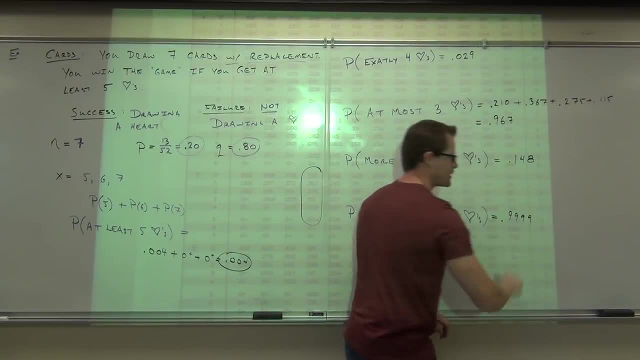 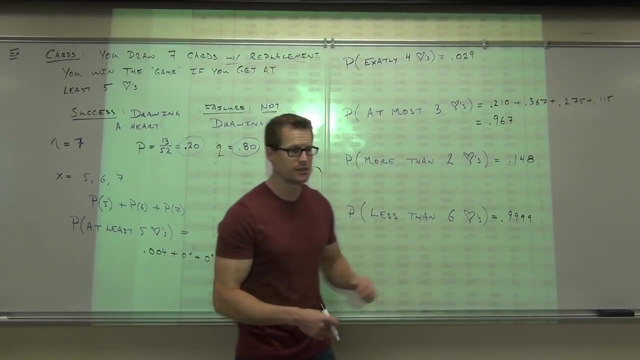 just do like .9999, give me an extra 9 on there. I don't know if this 9 is going to be accurate, but it's definitely not 1.00.. I need you to know that. Would you raise your hand if you're okay with this? 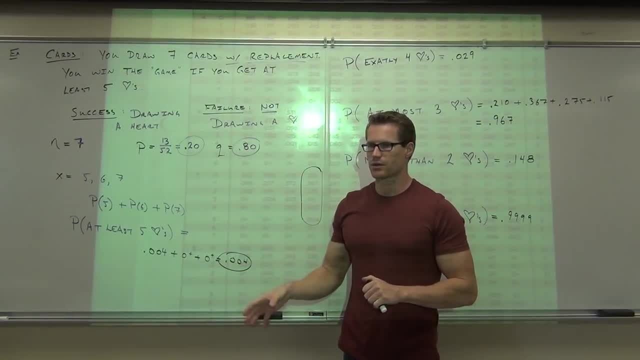 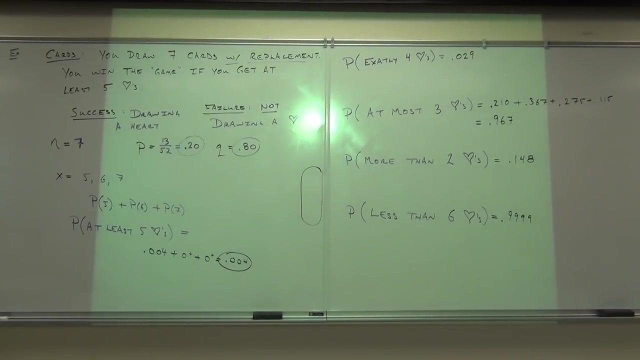 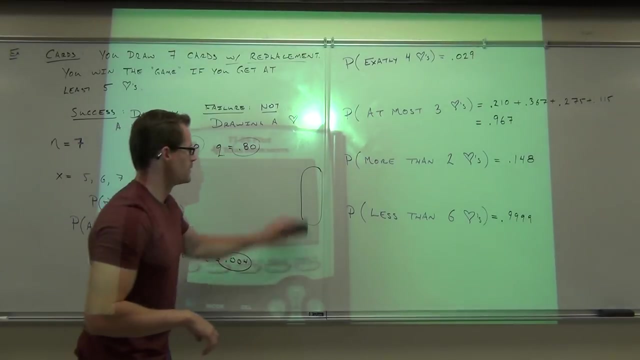 I'm okay with this so far. Now would you like to see the way to do this on a calculator? Yes, Okay, let's do that. One of my tables. You see that, okay, Okay, so you're going to have to remember what buttons we have to press. 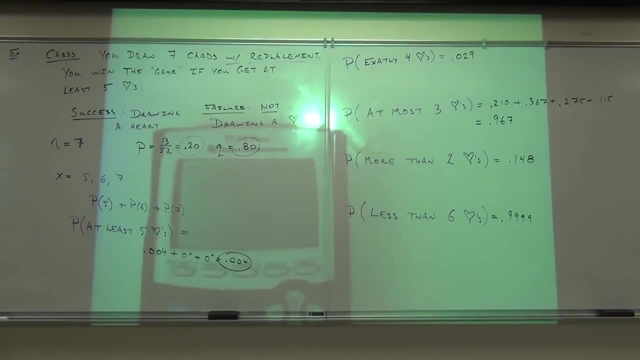 You're going to have to remember which buttons are pressed. Now I want to keep this zoomed in, so you'll have to remember what buttons we are pressing. Firstly, where did we go to deal with the binomial distribution? Not math. 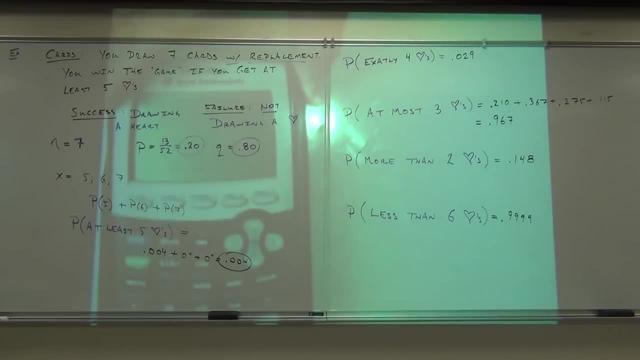 We're now in. can you see it down there? We're in a distribution, so we're going to use second. that's what I just pressed. 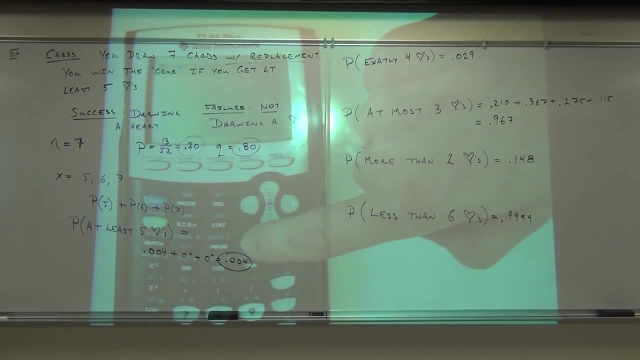 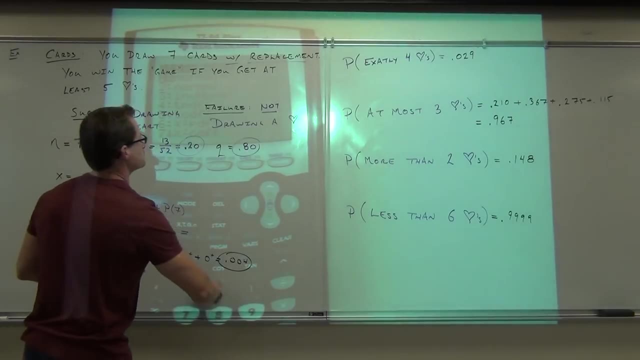 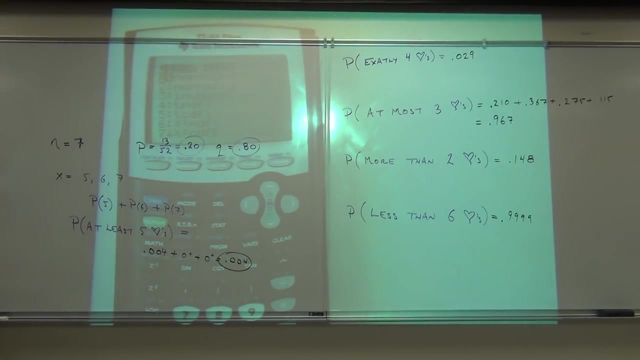 And distribution is right there by my finger. So we're going to press the V-A-R-S button That brings you to your distribution There. that'll work a little bit better. So we're looking at our distribution. which distribution are we going to go to? 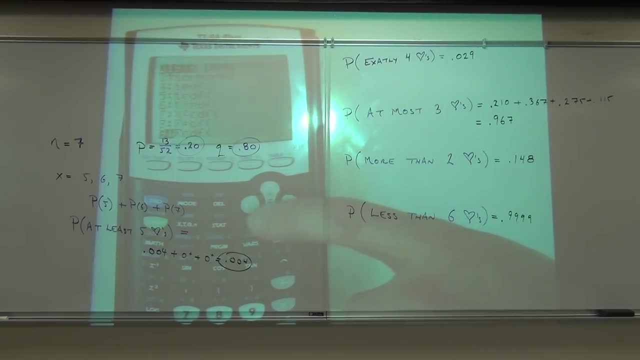 That's way down here. pass our chi squared, pass our t, pass our f Down here to binomial. you have two choices. you have the pdf and the cdf. Which one of them works for a single value, the p or the c? which one? 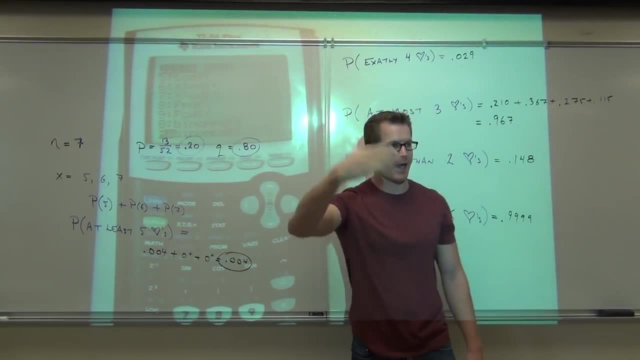 The p is for a point, one single point. The c means cumulative. it'll add them all up for you. You put in the information the same way. so you really need to know. You need to know which case you are working on. 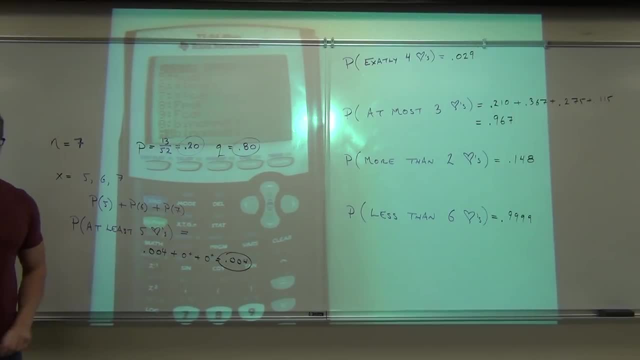 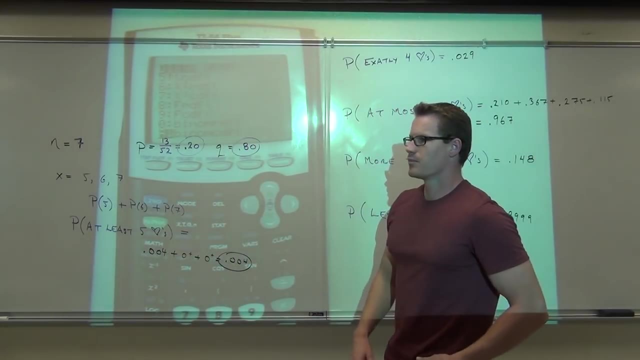 In our case, for at least five parts. at least five parts. which one are we working on? Are we working on a c or a p C? Now, here's the problem with this. maybe I'll come back to this one. I want to work on a couple of these other ones first. okay, 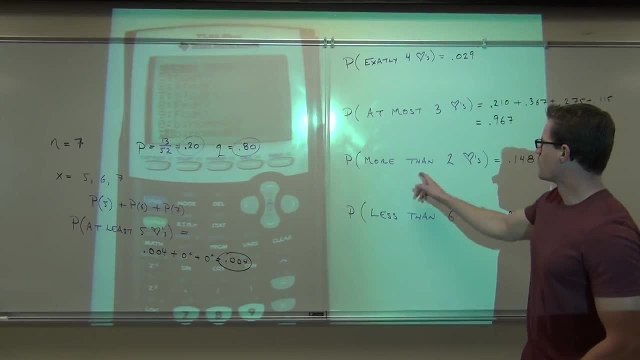 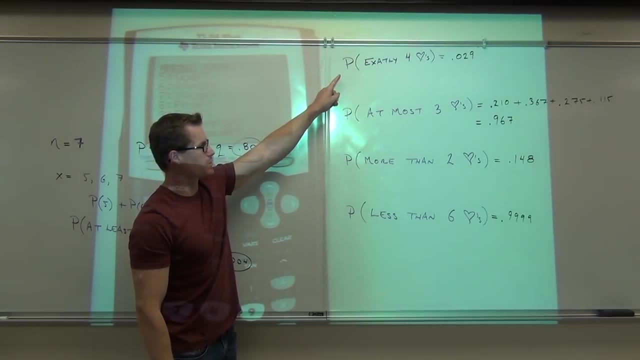 I'll show you the at least. I'll show you the more than, and just a little bit. I want to show you the exactly first. then I'm going to go through the at most, the less than I'm going to do those other two. 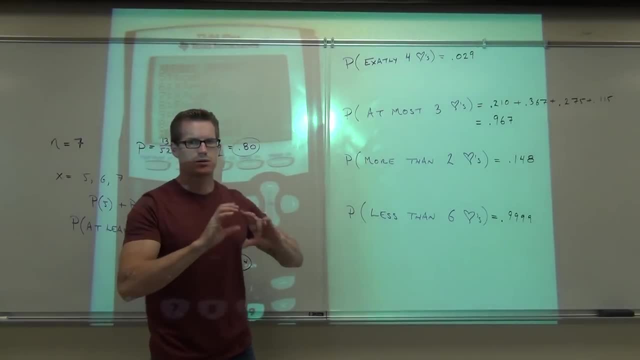 So let's work on exactly for right now. for example, are we going to be on the p or the c? P? Okay, for at most, are we going to be on the p or the c, C, C. For the rest of them, we'll be on the c. 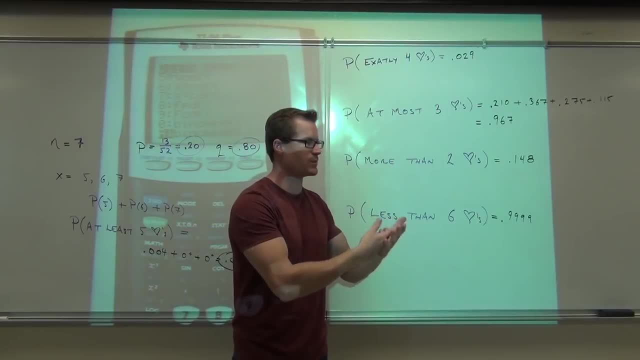 We'll be on the cumulative, because we're talking about, at most, less than more than all that stuff. If it says exactly, it's the p, If it's anything else, it's the c. Dr Henry, are you okay with that? 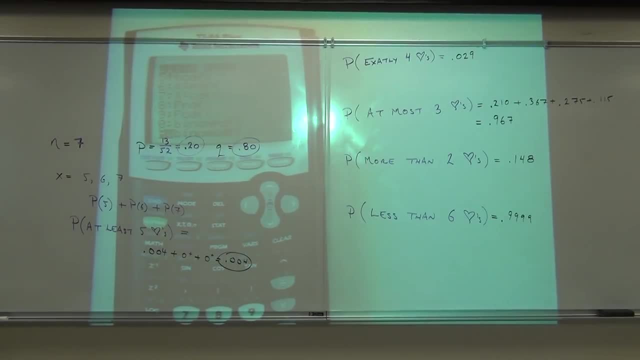 So let's do the exactly for, For, exactly for. do you remember what we plug in first? So now I'm going up to the p, I'm going to highlight the zero, I'll press enter. That should be on our screen right there. 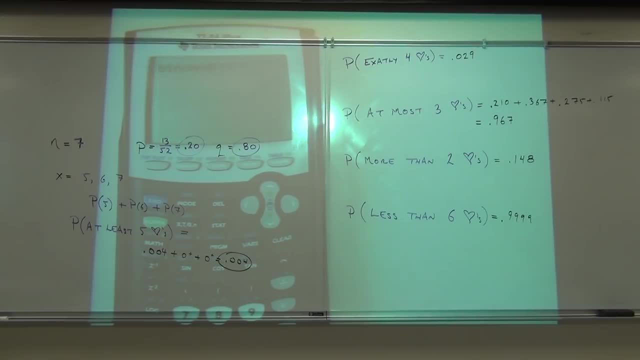 What do we plug in first for that? The, not the x, it's the Seven. Seven. What's n? what's? I'll just give it to you. What's the n stand for? N stands for seven. Yeah, it's the seven. 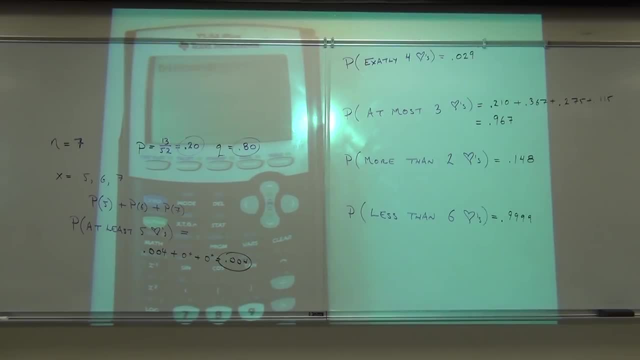 That's our n, Then we find our comma And we put in what next? X, Not x, The probability. You put in The probability, The probability, Sure, Put in the probability. Okay, The probability, The probability of what? 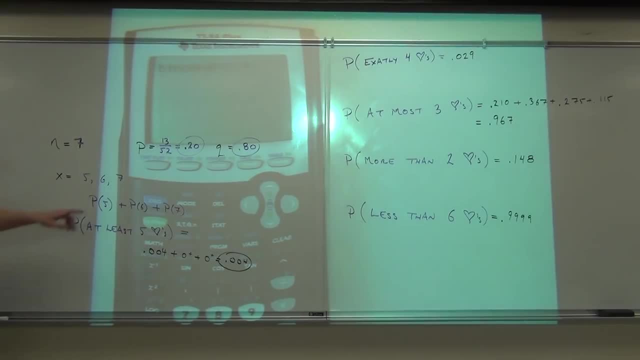 This example. We put in this Right there. Or if you want to do the previous example, you can do that right now. you put in 0.25 right now. Now we're, we're, we did this so we could use the table. 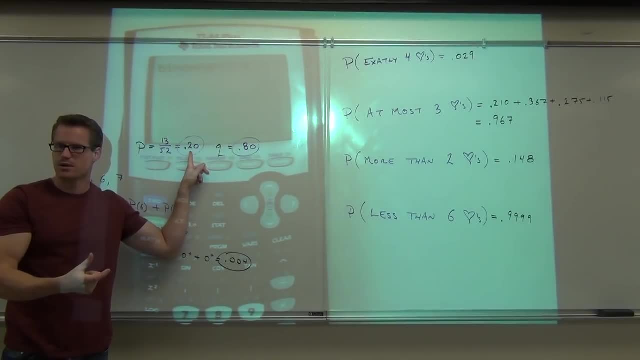 Of course, the realistic example would be 0.25.. You with me on that. I want to show that to you, so you know that your table doesn't work perfect in every case. Right, It doesn't have everything. If this was a 0.28, you certainly wouldn't be able to use the table at all. 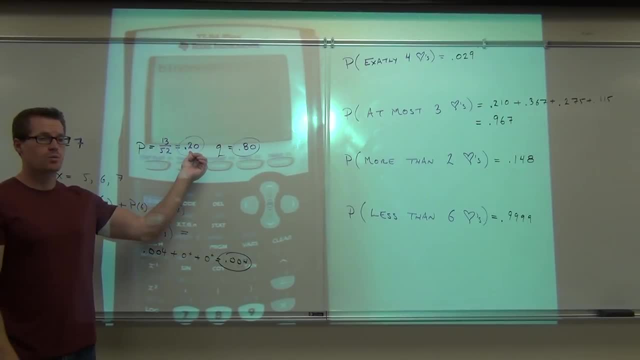 It'd be very, it'd be awful. So here our 0.20,. we're going to use this so you can see the. the numbers do match up or pretty close to match up on this. So 0.20, that is our probability of success for each trial. 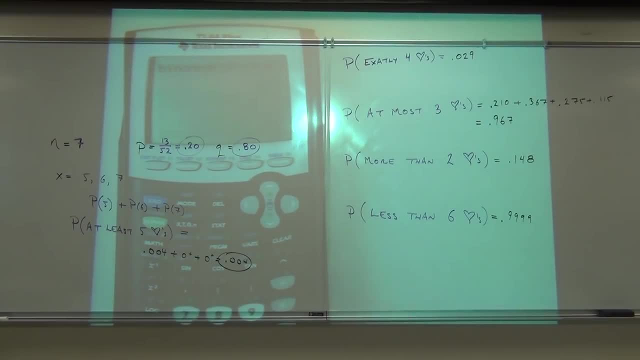 0.2.. What's the next thing that we plug in? X? Now comes our x. So with the calculator you do an n, then your little case, letter p and then whatever x you're looking for In our case, what's our x? ladies and gentlemen? 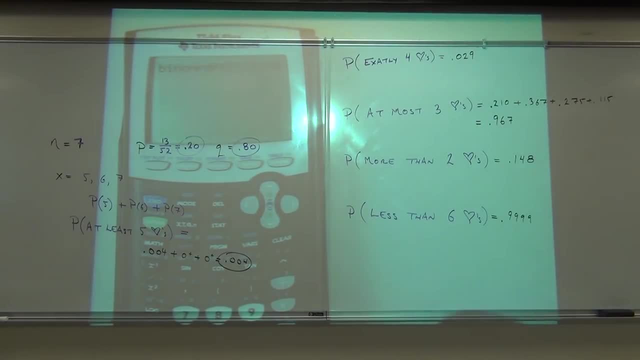 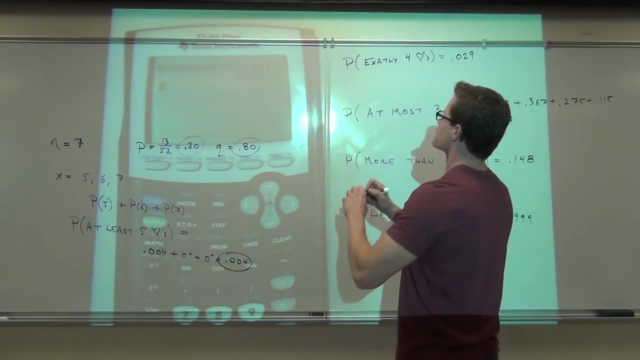 We're over there: 4. 4., 4. 4, maybe 7, 0.. 0.. 0.. 2. Three, Oh, it's 10. 0.. 2. One, 1.. 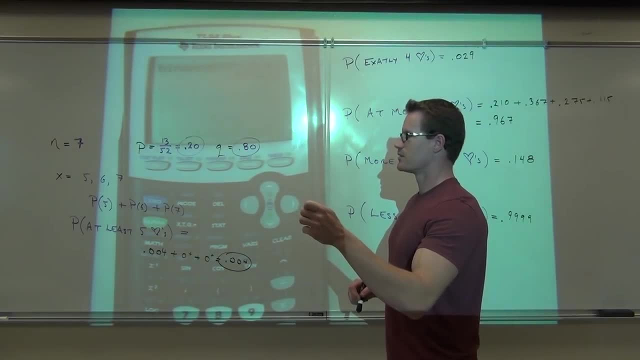 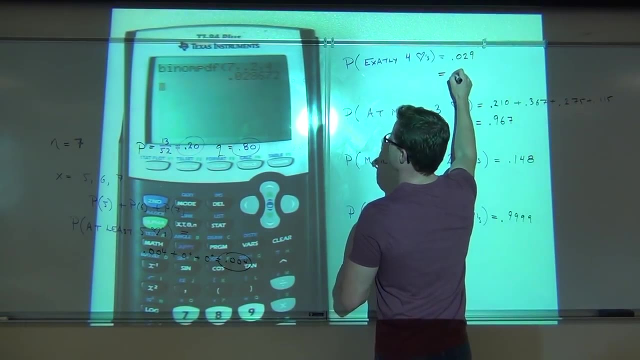 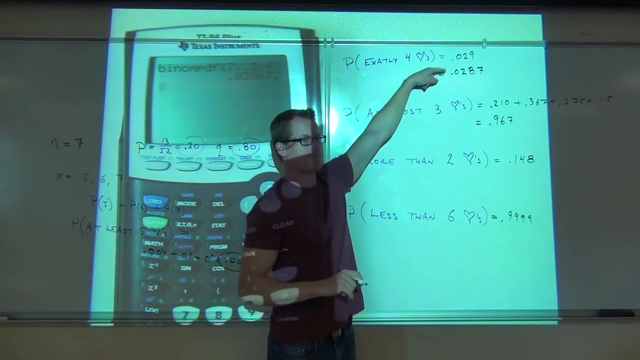 1. 1. 2. One, 2. 1., 1. 0. 0. 1. 0. 2. 0. 0., 1. 2., 1. 1.. 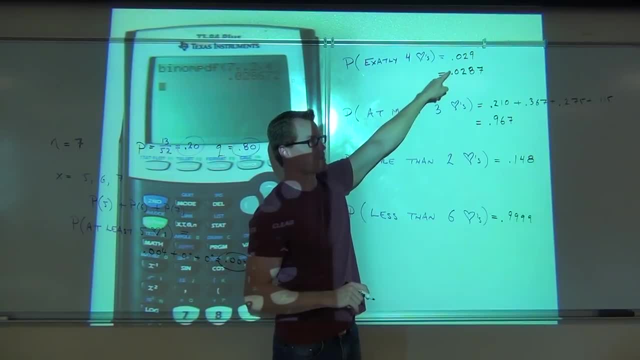 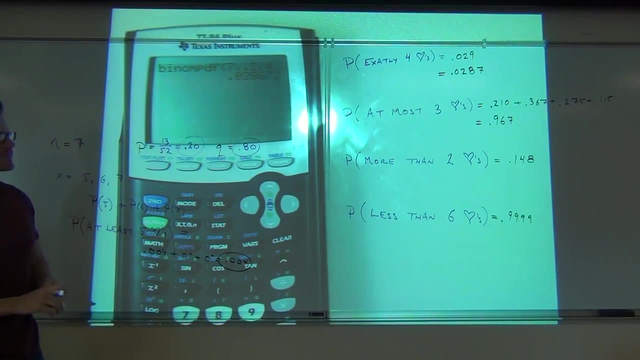 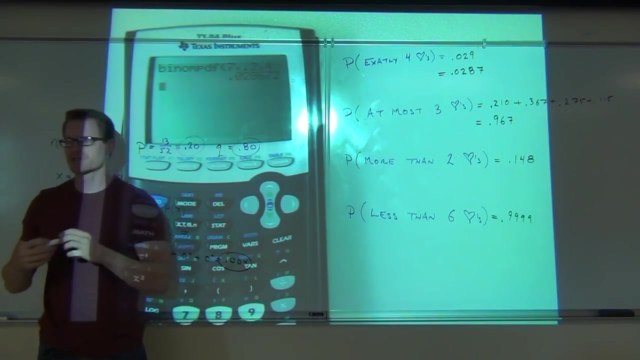 1. This one's actually supposed to be this one. It's just rounded. It's rounded more to fit on the table, Are you guys okay? so far, All right, let's do the at most three parts. If you have at most three parts, stick with me here, ladies and gentlemen. 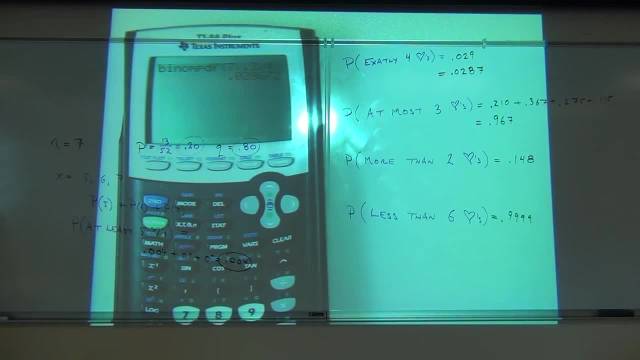 If you don't have a calculator, it's good to refresh your memory on how to do this. At most, three parts. are we going to be in the P or the C? once again C. So I'll go back to my distribution. 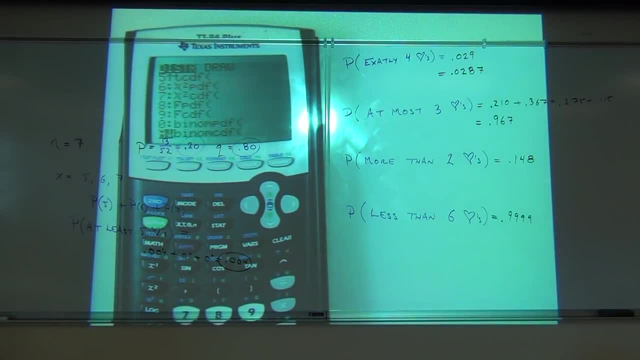 I'll go down to the binomial CDF. I'll press enter on the CDF. That's the A. Did our trials change? Did our trials change? No, We still have seven. Did our probability of success for each trial change? 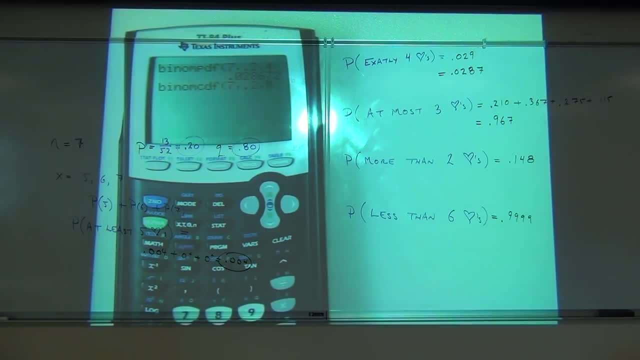 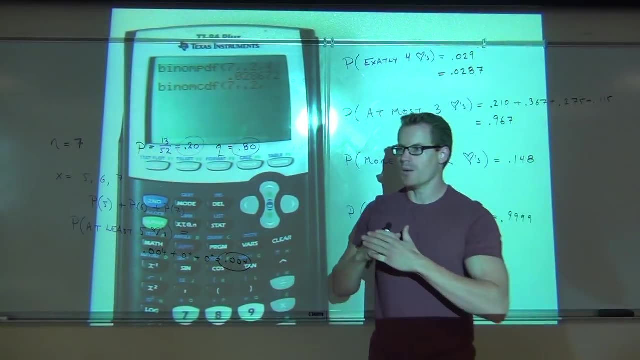 No, We still have .20 or .2.. Now did the Xs change? Yes, Now you need to know what at most three means. This is what I'm talking about. Do we want to go up to three non-inclusive or up to three including three? 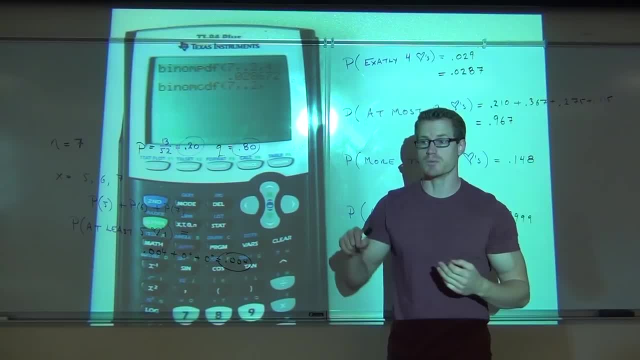 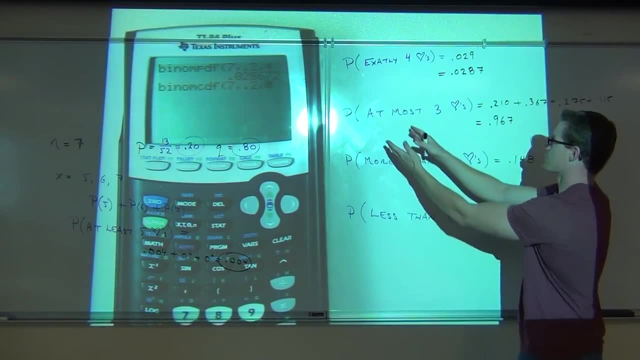 Including three. Listen, if you want to include the three, you put the three. If you don't want to include the three, you put the two. Does that make sense? So we want at most three. that means 0,, 1,, 2, or the three. 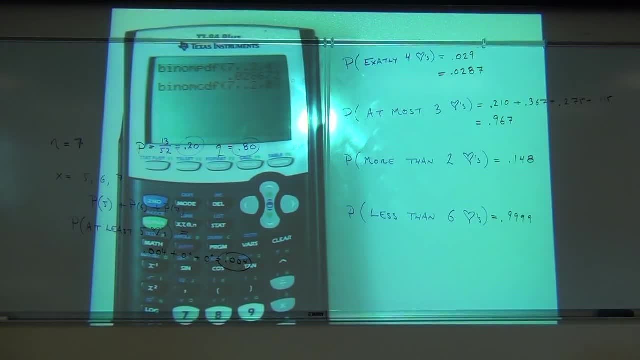 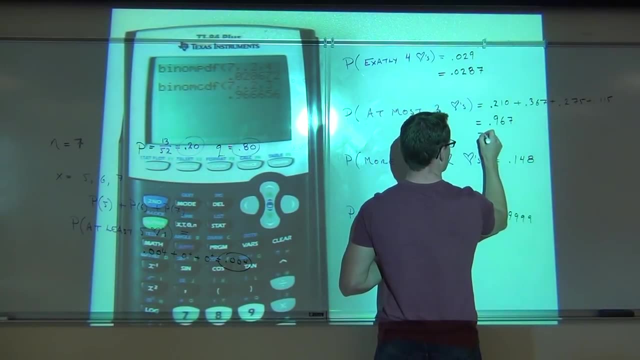 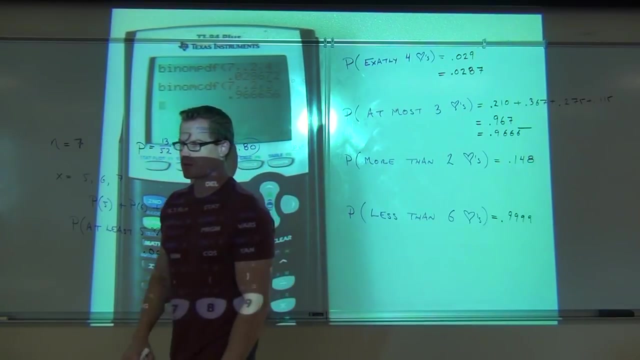 We're going to put the three. This is going to add up to the three, including the three, and it's going to give you .9666.. Yes, Does that round to .967, like your table suggests? Yes, Absolutely, Oh show. 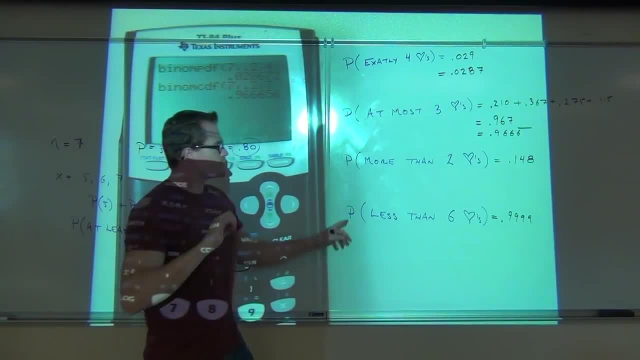 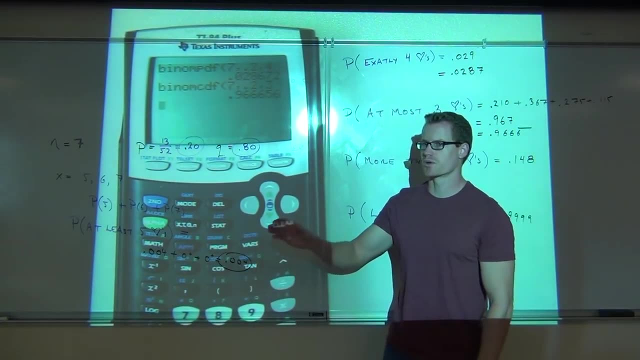 Okay, so we've got .9666 forever. Let's do the less than six hearts. Less than six hearts. What works for less than six hearts? Does the six work or not? Does the six work for less than six? Ladies and gentlemen, I need you with me. 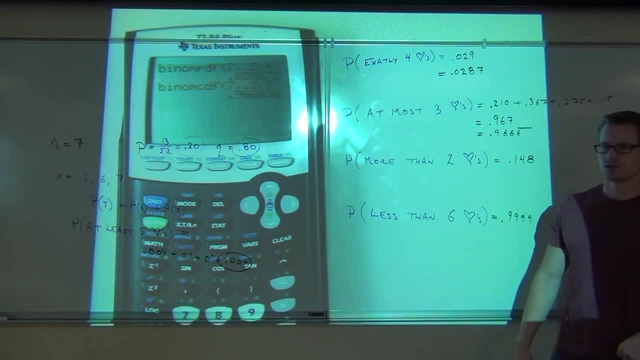 Does the six work? No, What works? Five, Five or less? 1,, 2,, 3,, 4, or 5.. 0, 1,, 2,, 3,, 4, or 5.. 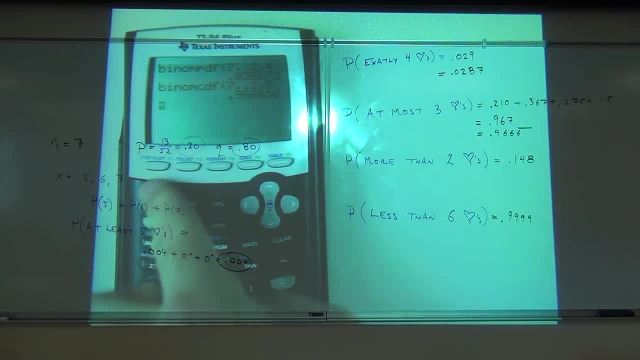 So when you do this one, you've got to go back to your distribution. We're still on the CDF, but I want you to watch what I'm going to do here If we're going to do less than six. be smarter than your calculator. 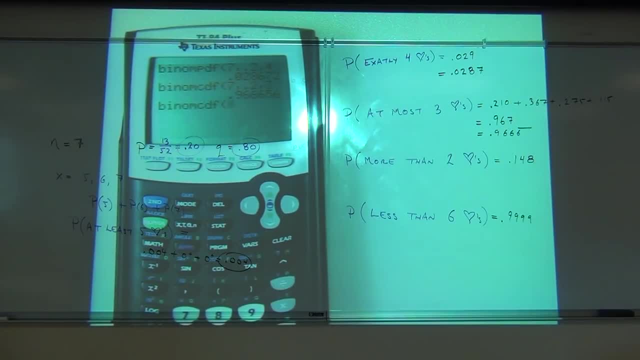 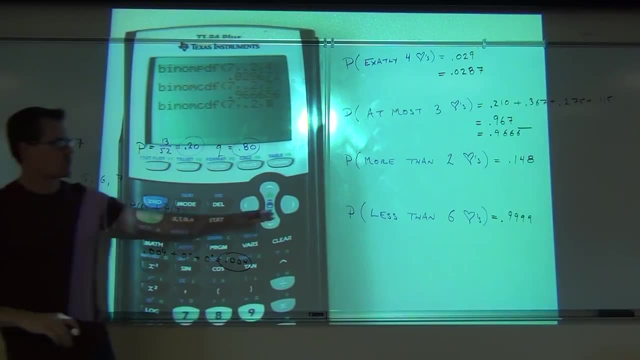 Your calculator doesn't really know what you mean. It just says: I know you're bugging number 7.. You've got to be smarter than the problem in your calculator. You've got to know that what I'm really talking about is five or less, including the five. 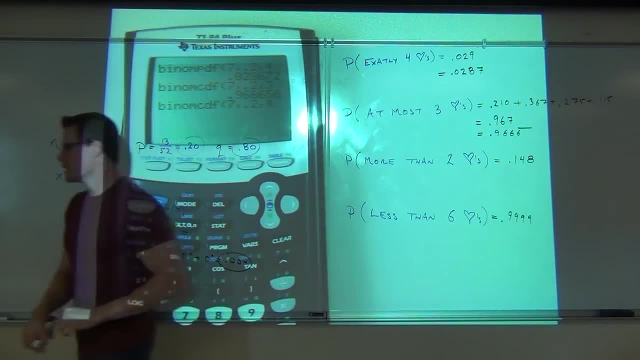 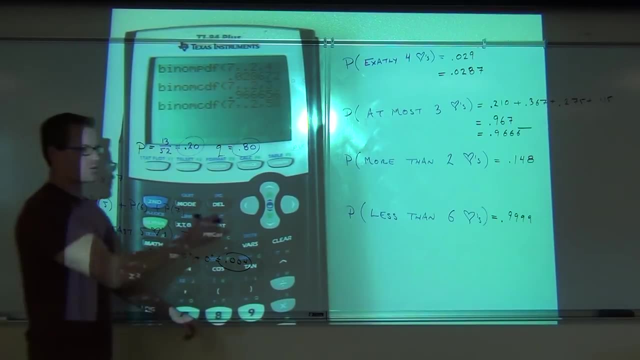 Less than six is five or less. Those are the same thing. So I'm going to put it in Not six, because that would add to six. I'm going to put it in five because I know that really, the only way that I can accomplish this is 0,, 1,, 2,, 3,, 4, or 5.. 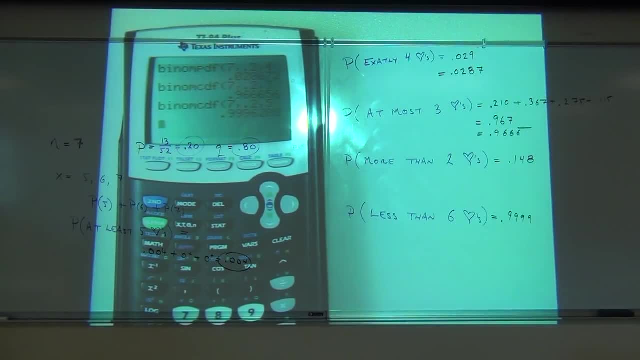 I put in the five there, I press enter 0.9996.. I was a little off: 0.9996.. According to the calculator, that's what we're going to do. Let's see what we get. Okay, I need you to raise your hand if you're okay on finding what we have just found so far. 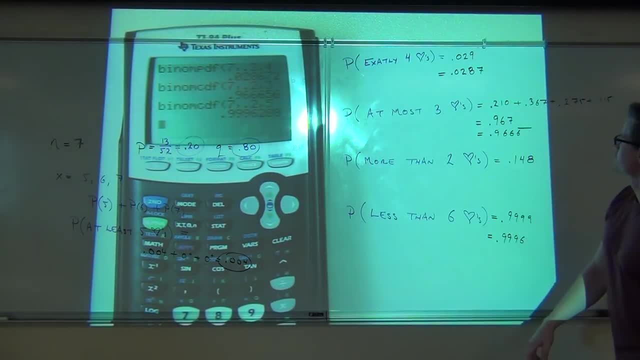 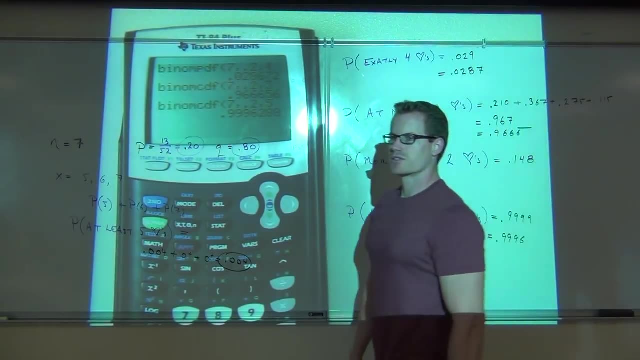 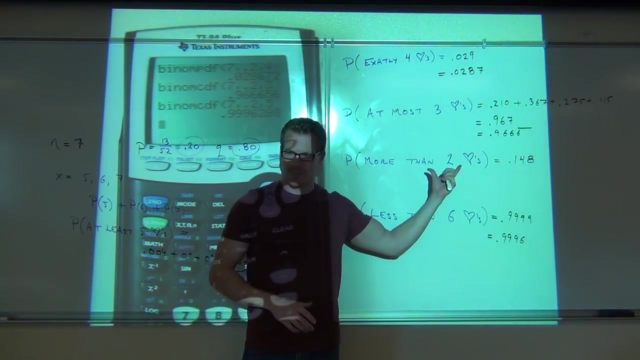 Cool, Now the next ones We're going to do. which ones have we done? The more than two hearts or the at least five hearts? All right, Here's the deal. It's oftentimes a lot easier to find out a complement of this thing in the calculator. 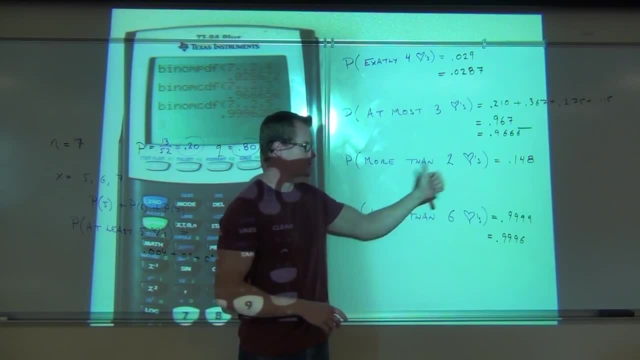 because your calculator won't directly give you this. If you plug in two, You know what It's going to give you: 0,, 1, or 2.. You've seen that right, That's what these gave you. It's going to give you 0,, 1, or 2.. 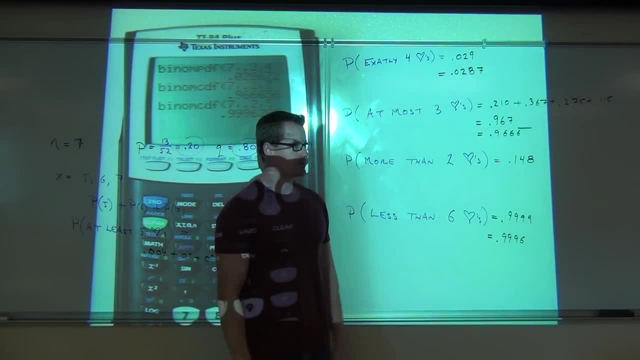 If you plug in one, it's going to give you 0, 1.. If you plug in three, it's not going to give you greater than that. It's going to give you 0,, 1,, 2, or 3.. 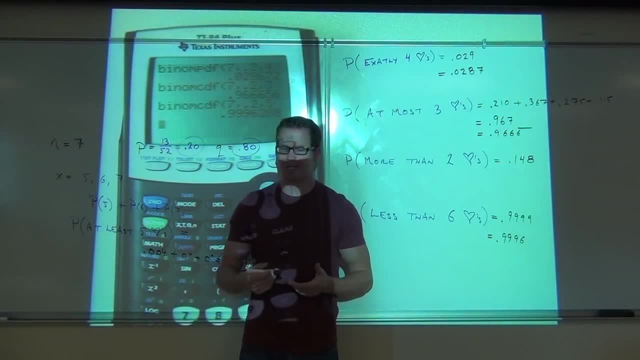 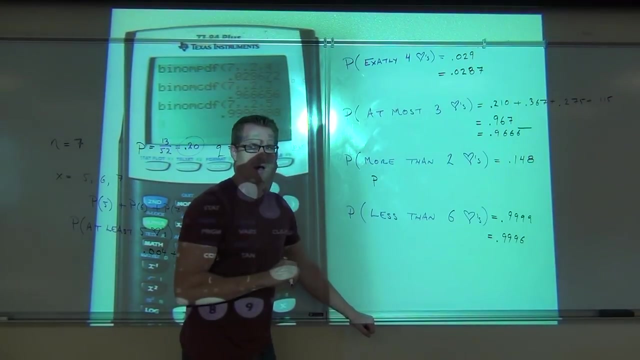 So here's the idea: In order to use your calculator effectively, you need to understand the complement of what this is. So you need to understand that, if I want more than two hearts, what we should be doing is finding the probability What's the opposite of more than two hearts? 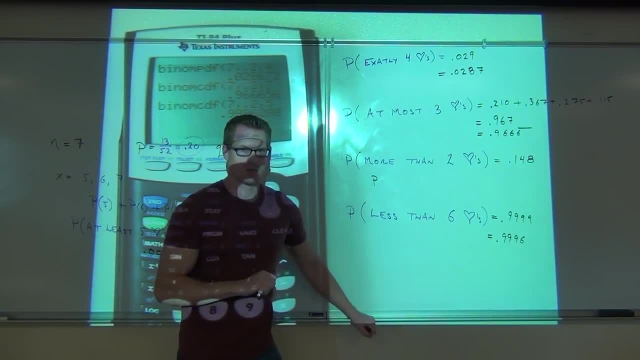 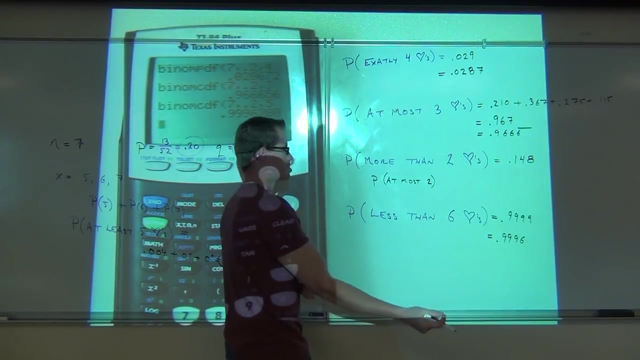 What's the opposite of more than two? At most two, At most two, Or less than three, Or probably at most two would be the best way to think of that. So the complement of more than two hearts is at most two. Why are we doing that? 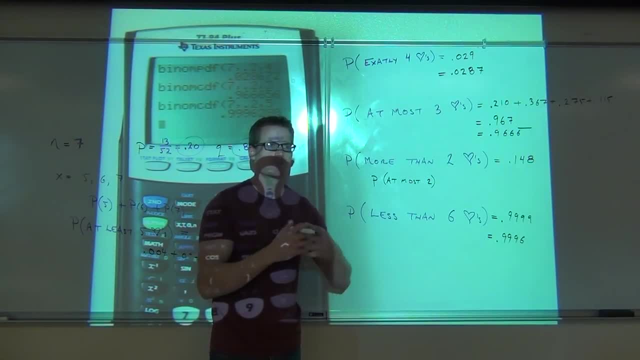 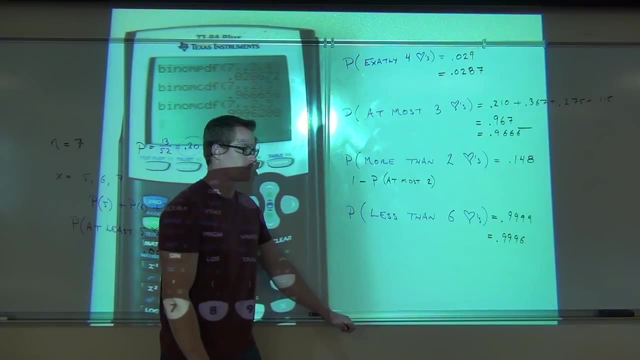 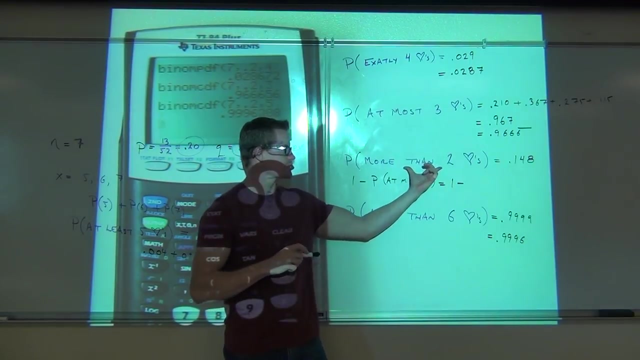 Well, we know one thing about complements: Complements have to add up to what number? One minus one? Let's just take this as one minus at most two, One minus at most two. Check it out. Aren't these things complements? 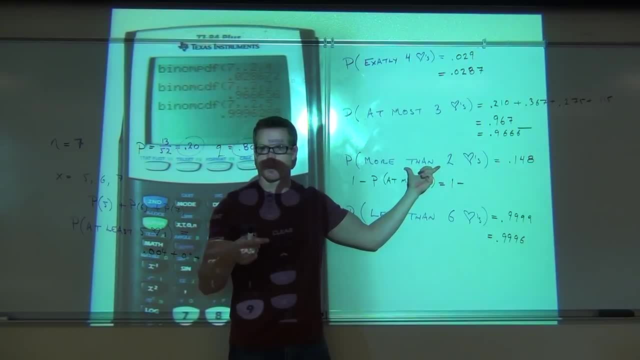 More than two, and at most two More than two. Think about more than two. Can you please think about more than two? for me, What's more than two mean Three, four, five. What's at most? two, Three, four, five. 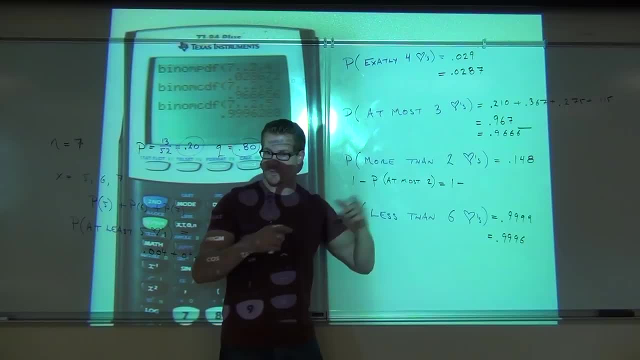 What's at most two mean Zero one, two. Zero one Are those things complements? You're either three, four, five, six, seven or zero one, two. Those things are complements, Instead of going for this one directly in the calculator. 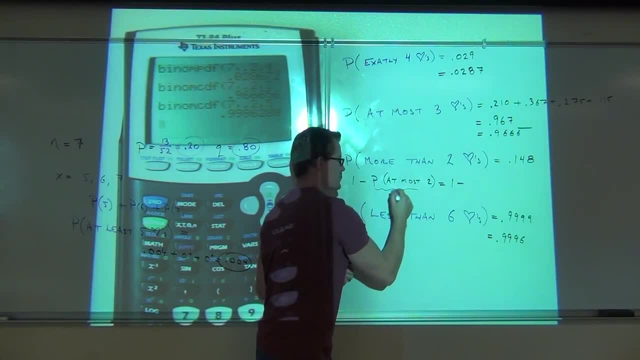 you've got to take one minus the complement. This would be our complement here. So let's look for at most two. Subtract that from our one We'll go to our distribution button, We'll go down to the cumulative again, We'll plug in the second. 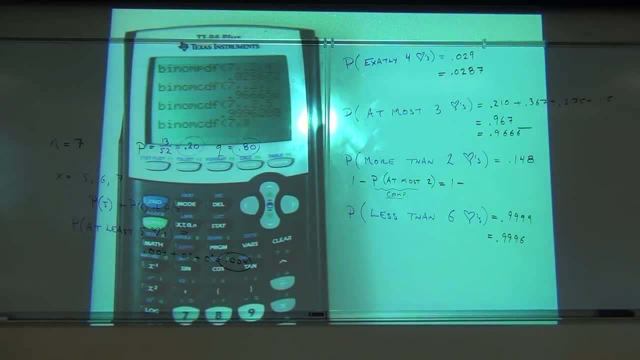 We'll plug in the .2.. We'll plug in what's the next number. we're going to plug in Two, Two. Now, when you're plugging in the two, remember what this is giving you right here when you do the two. 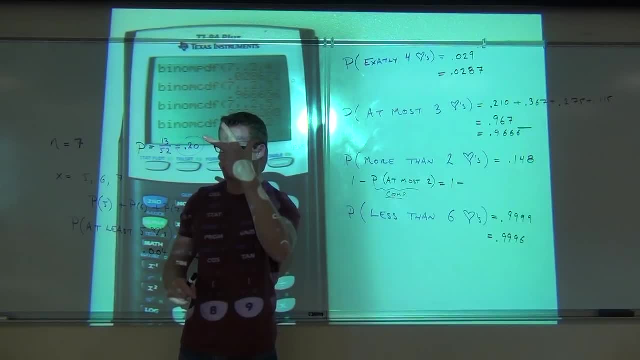 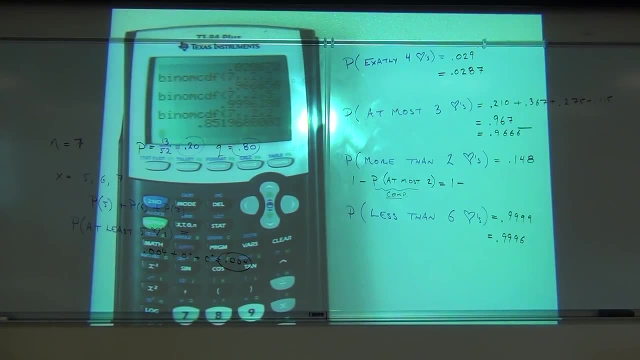 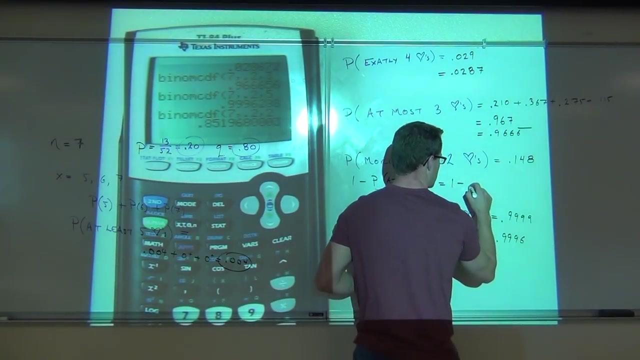 That's giving you zero or one or two. Does that make sense to you? Yes, It's not giving what you want, It's giving you the complement of what you want. Go press enter. That's giving us .8520.. Well, I'm just doing the math in my head. 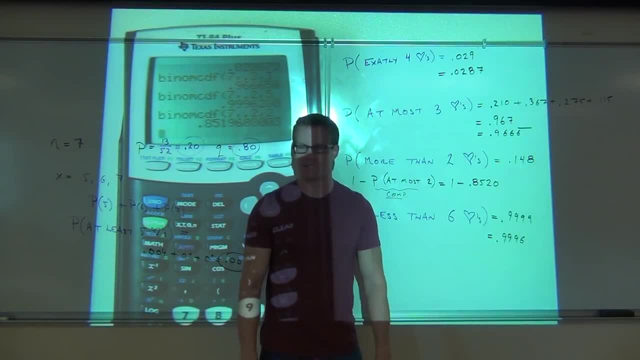 Are these things equal? Take your calculator. if you don't believe me, Take 1 minus .8520.. Is it the same? Yes, Exactly the same as that one. That's kind of cool. Hey, nod your head if you're with me on that one. 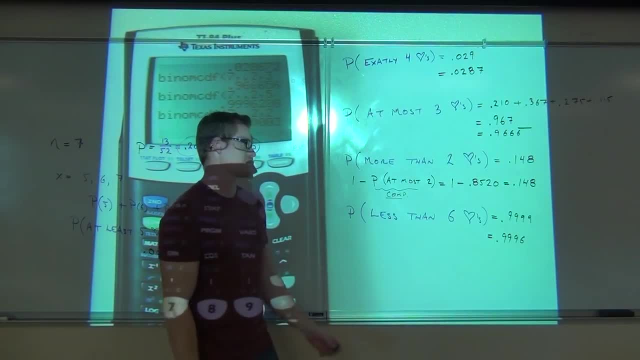 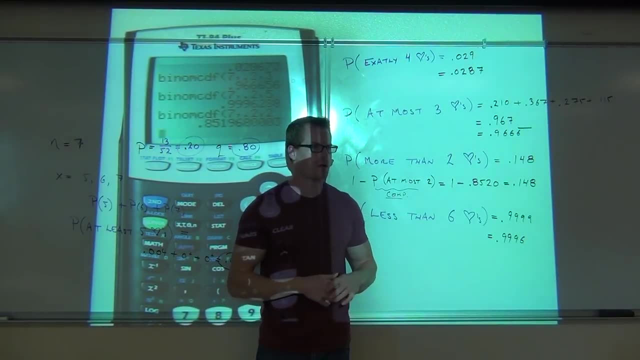 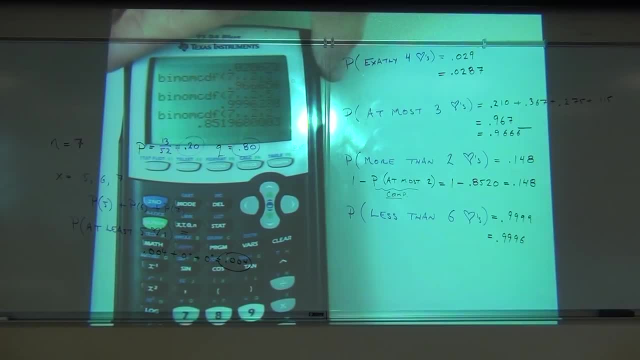 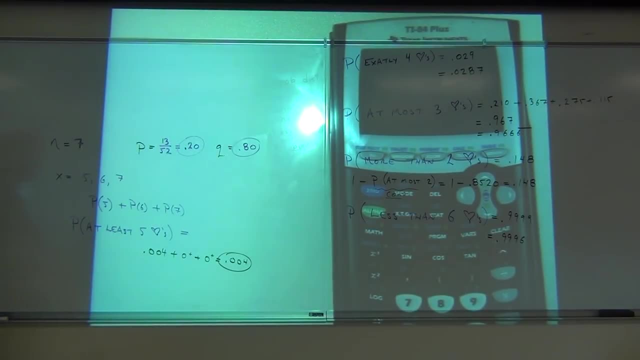 Change my sides. Change my sides. here. We want the probability of at least five hearts. At least five hearts means what? What does at least five mean to you? At most four, Okay, The compliment would be at most four, but what's at least five mean? 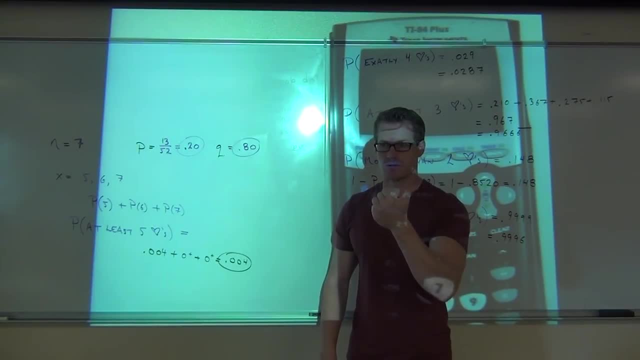 At least five. Five, Does it include the five or not? Yes, Five, six, seven. What's the opposite or compliment of five, six seven? Zero to four, Zero to four. So we want at most the opposite, or the compliment of at least five hearts is at most four hearts. 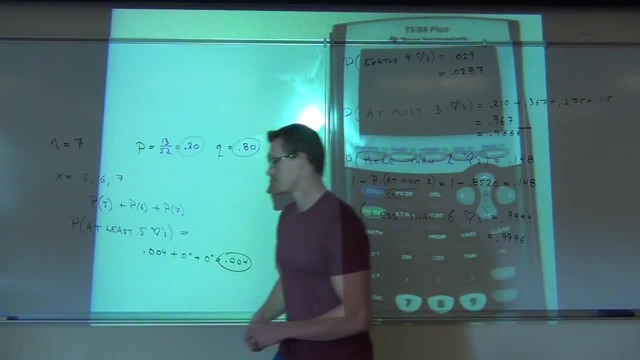 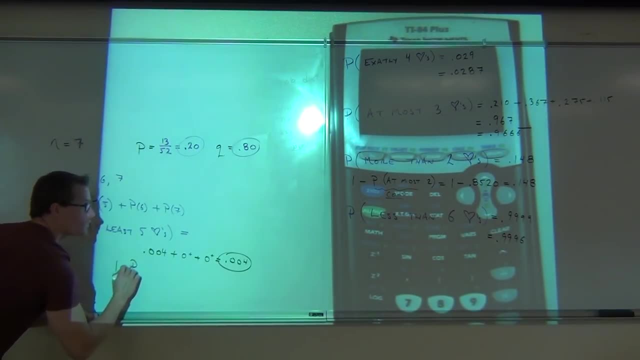 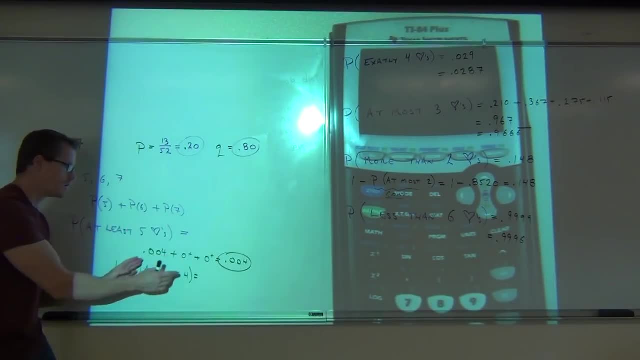 four of hearts. Those are complimentary events. We know they have to add up to one. So by saying probability is zero, one, two, three or four. subtract that probability from my one, I get the probability of five, six or seven. 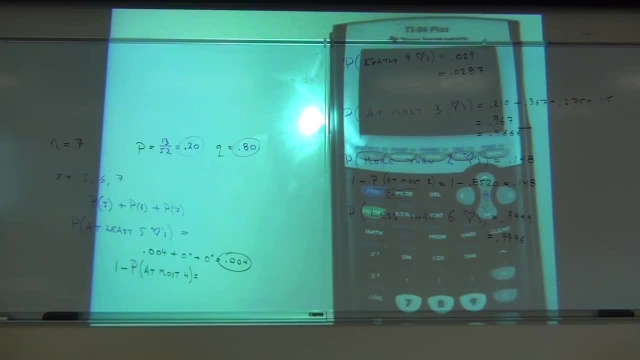 palm Knife Topics. To vid the bottom line – And we're gonna go for now. what number are we gonna plug in after that, Say 11?? Yeah, we'll do our four. We want up to and including four, 0.9953..